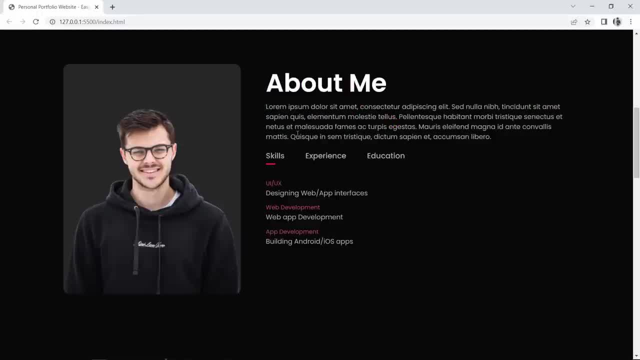 text and then we have three tabs. in the first we can see the skills over here. then if i click on the second tab link, which is experience, if i click here it will display the work experience of the user and if i click on education it will display the education of the user. so this tab is also 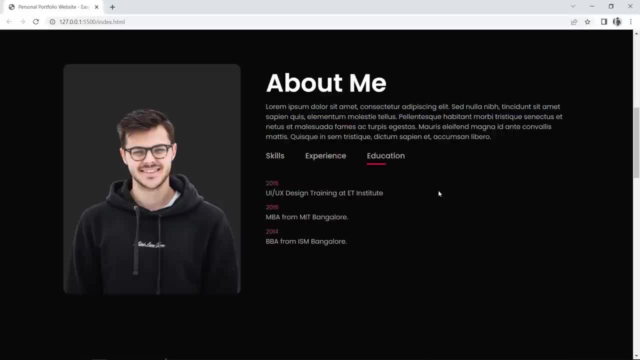 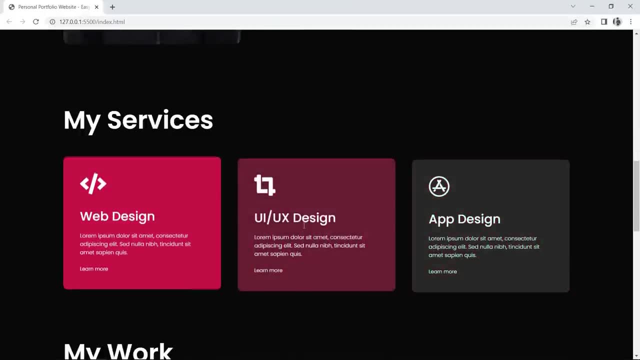 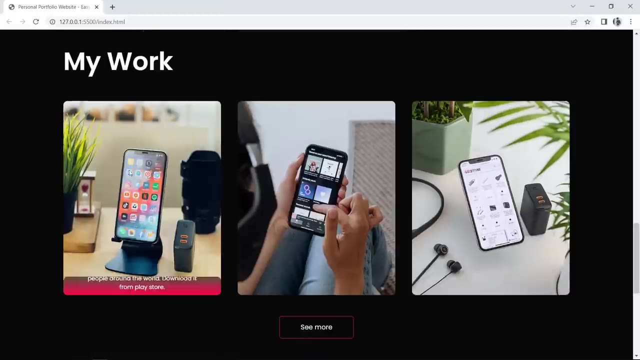 looking good. then let's scroll this website again. in the next section you can see my services. here also you can see this hover effect. if i take cursor, the background color is changing and it is moving up by some pixels. and let's scroll, then we have the my work or portfolio section. here you can see. 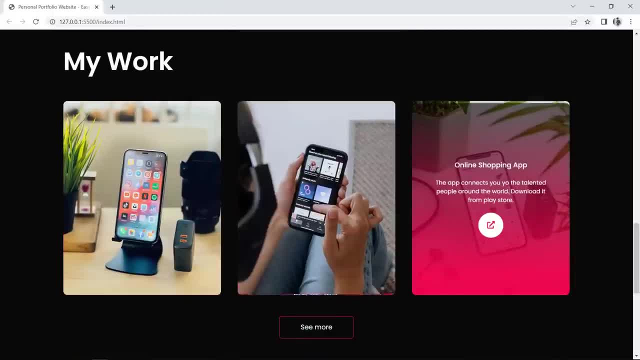 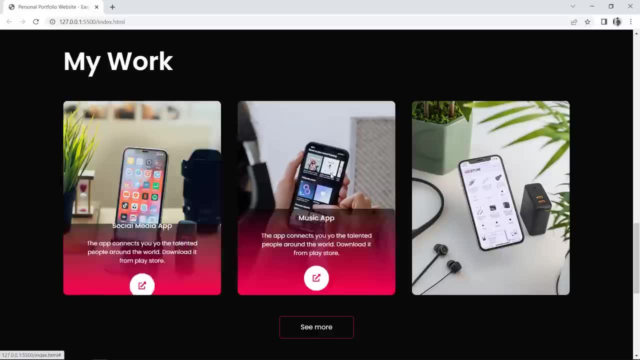 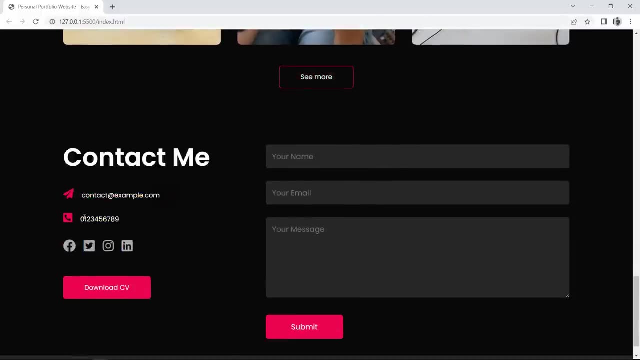 beautiful hover effect. when i take cursor, the background image gets zoom in and then we have these text coming from the bottom and this external link. then we have this button with hover effect and then we can see the contact information, like email id, phone number, social media icons. 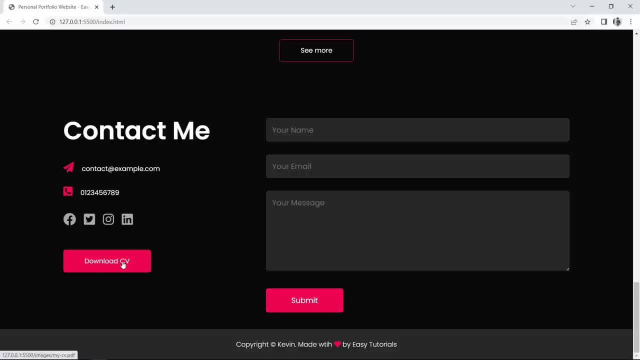 then download button where you can download any file. if i click here, you can see it will start downloading the attached file. here i have attached the pdf file, so it will start downloading this one. then we have this contact form here at the bottom. you can see this. 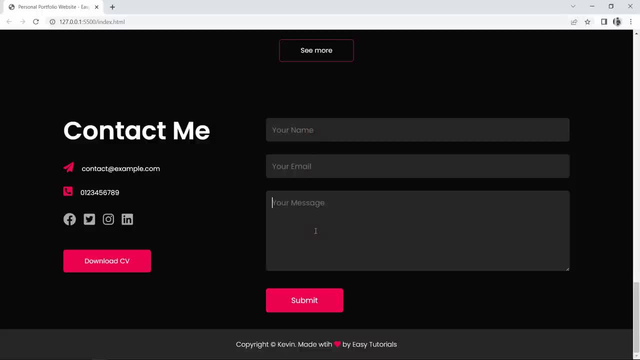 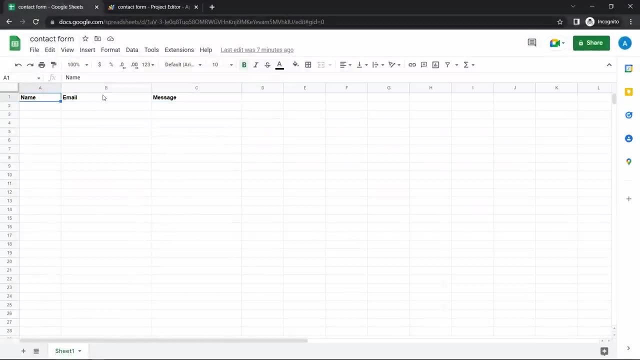 copyright message made with love by easyTutorials and in this contact form. if user will enter, any will receive the contact information on your google sheet. let's try this one. if i come to my google sheet, you can see right now it is blank. we have the fields name, email and. 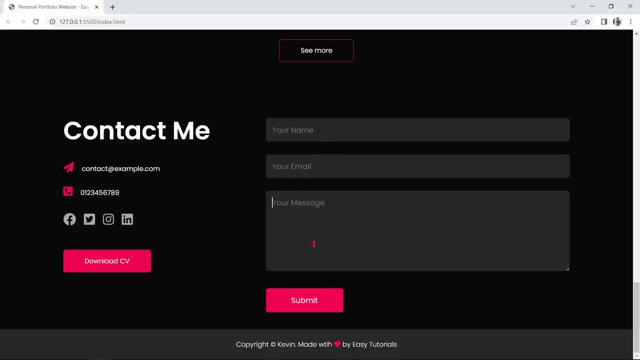 message. let's come back to the form. here also you can see name, email and message. let's write anything here. if i will write avinash, then email id and write any message here, just a test message. so we have added the name, email id and message and if i click on the 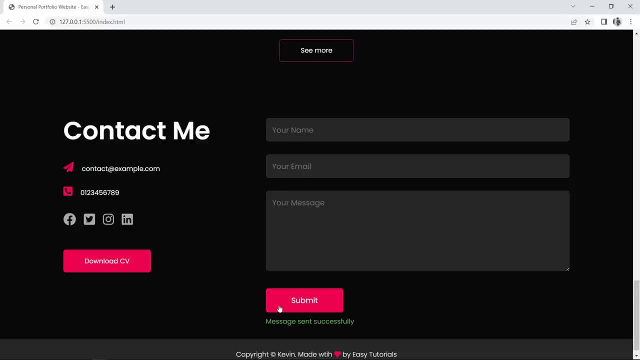 submit button. you can see we will get the success message here. message sent successfully and it will disappear after five seconds and the form get reset you let's check our google sheet. you can see we got the information here: name, email id and message. so this is how you can receive this contact form information on your google sheet if i click here. 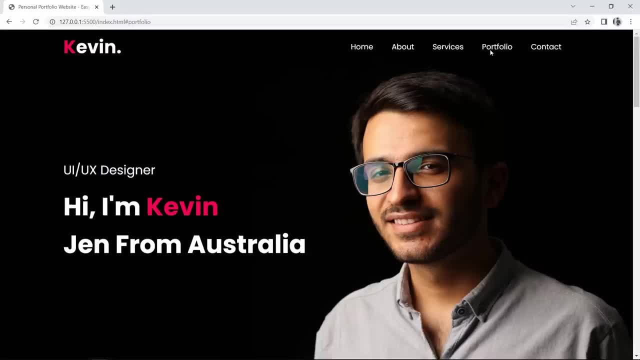 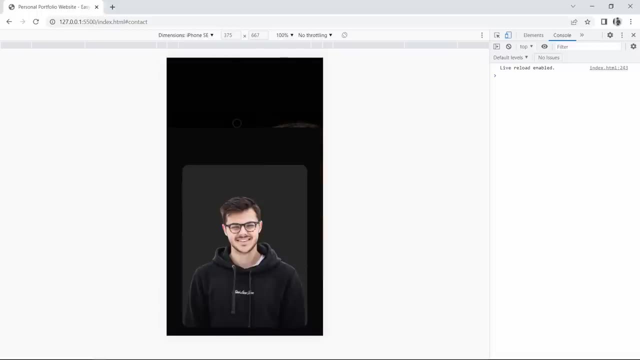 on this about, it will scroll the website to the about section. if i click on this portfolio, it will scroll the website to the portfolio section. and if i click on the contact, it will scroll the website to the contact section. let me open this website in smaller screen here you can see this. 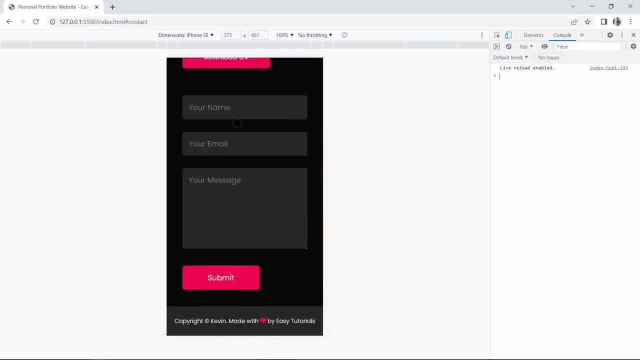 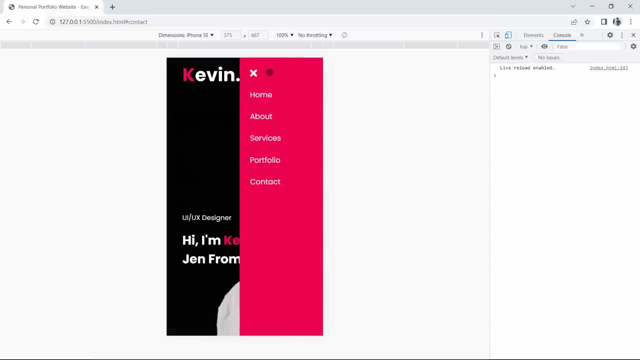 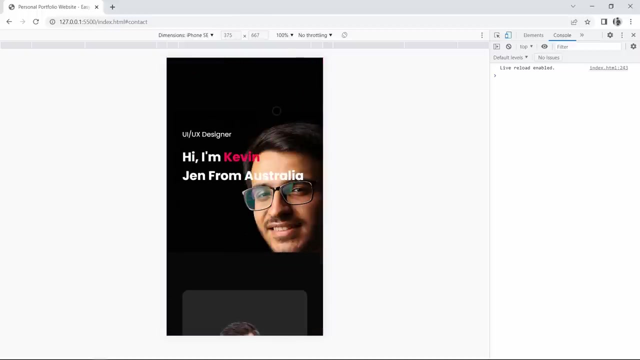 website is completely responsive for a smaller screen. also, this is how it will look on your mobile devices. if i click on this menu icon, it will open the menu from right side, and let's click here on this cross icon, it will close this side menu. so it is very good. now let's scroll this one, you can. 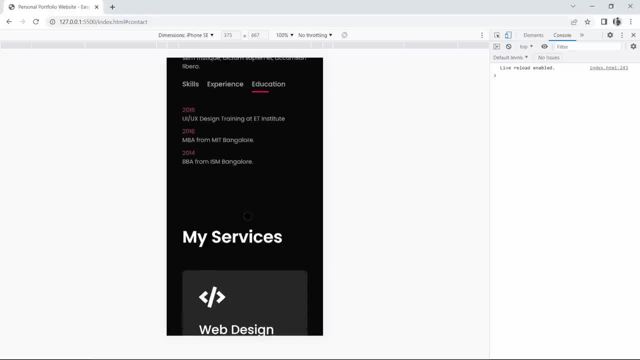 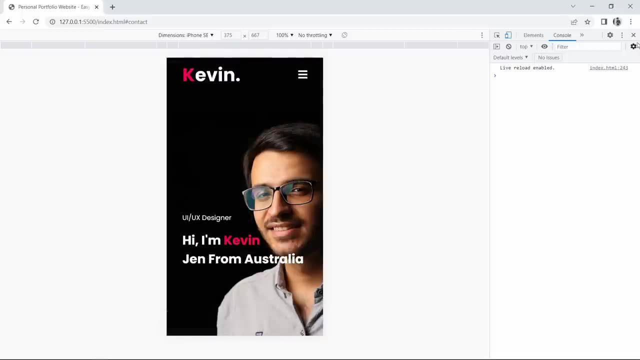 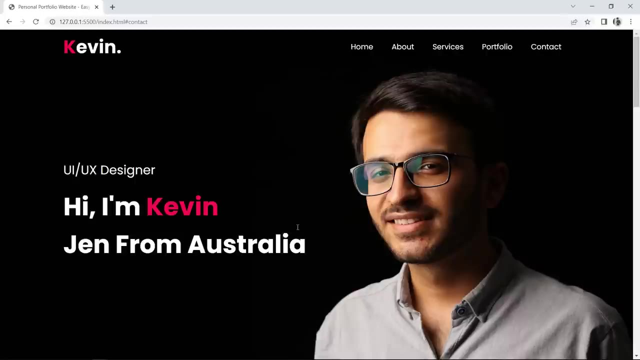 see, we have the other sections here, which is also perfect in a smaller screen, so we will make this website completely responsive for a smaller screen. we will create this portfolio website using a HTML, css and javascript. if you are beginner, you can start with this video also, but i will. 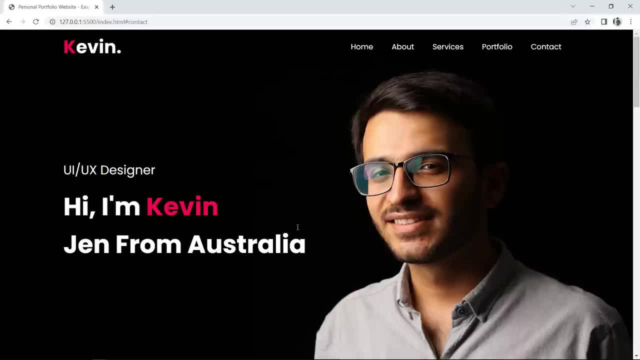 recommend you to at least watch my HTML and CSS beginners tutorial first, where i have explained all the HTML and CSS properties in detail. i will provide that HTML CSS beginners tutorial link in the description. after learning the basic HTML tags and CSS properties, you can start with this video. so now let's start making this personal portfolio website step. 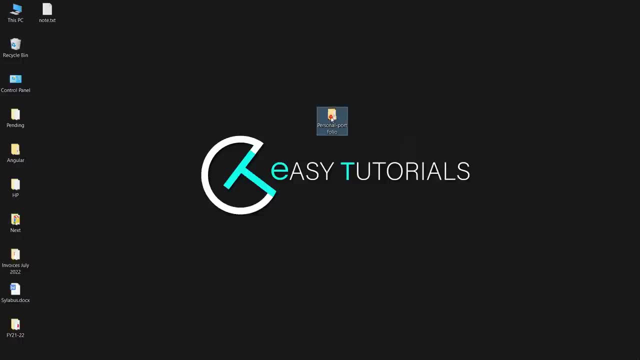 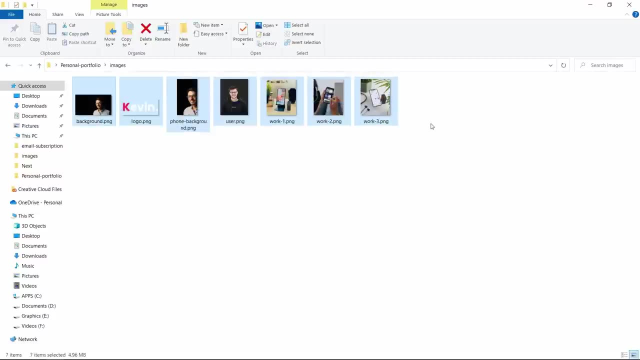 by step here. i have created one folder and in this folder you can see i have another folder called images and in this one you can see some images that i will be using on the website. you can find all these images download link in the video description, so just download these images from the link given in the description. 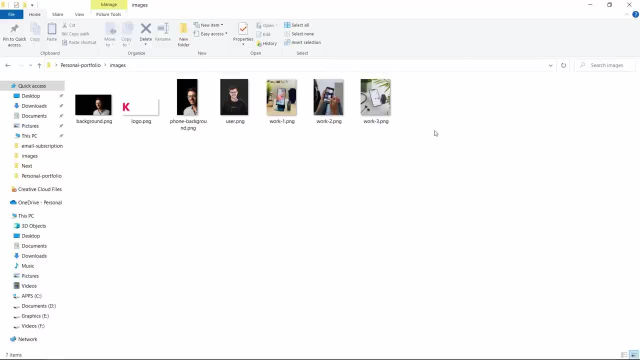 and start building your own portfolio website along with this video. now let me open this folder with my code editor, which is visual studio code. you can use any code editor here. in this left side, you can see this image folder and in this left side, you can see this image. 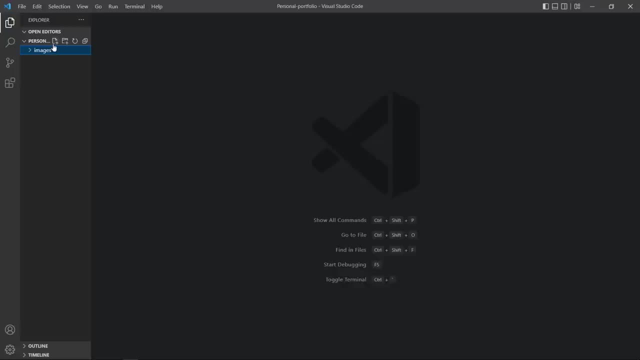 images folder and these images. here we have these icons to create a new file. just click here and create a new file, or you can click here on files. select new text file. click here and now save this file file and save. save this file in the folder that you have created. 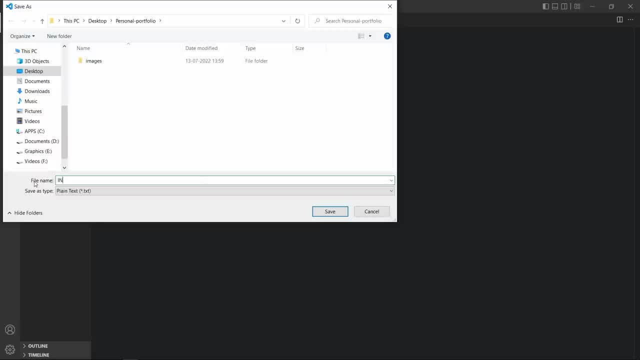 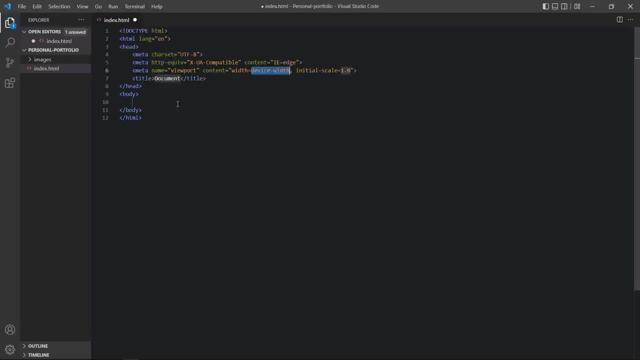 in this one i will write the file name indexhtml. so this is the html file. here we will add the basic html restructures. so let's quickly add this. here we have the html open and closing tag, then head. after that body: open and closing tag. in this head we have these meta and this title. let's create. 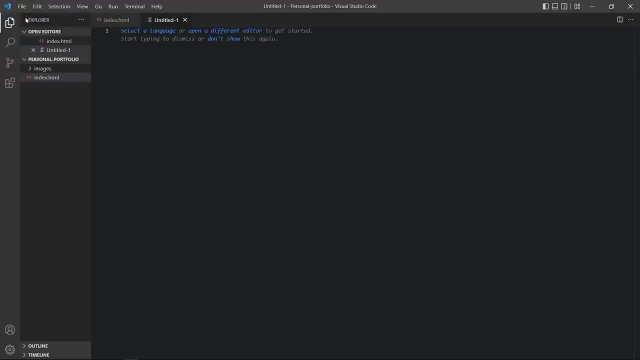 another file again. go to files new and save this file. i will save it as stylecss and in this one let's add star margin zero, padding zero, then font family and box sizing. next we have to connect this css file with the html file. so in this html file, before closing. 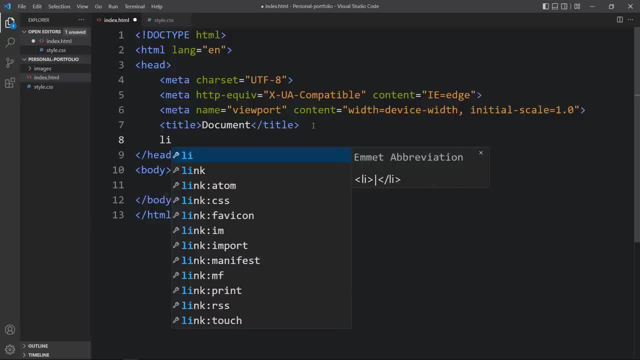 of this head tag. here we will add link rel, stylesheet, href and in this href write the file name of the css file, which is stylecss, so it will connect the html and css file. here in this title we can write our website title. so let me add: 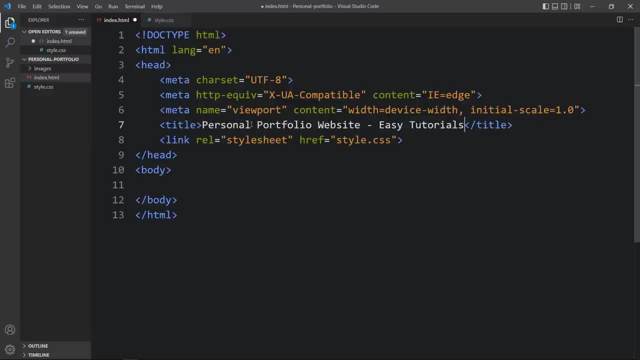 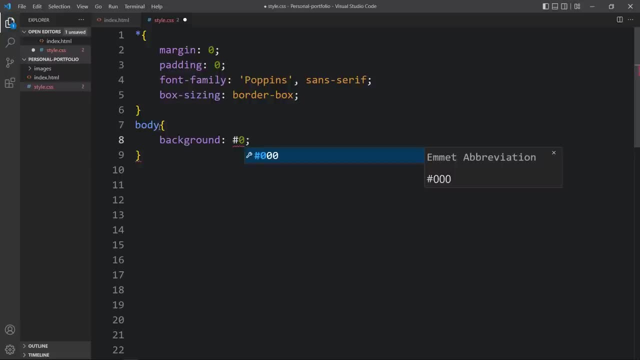 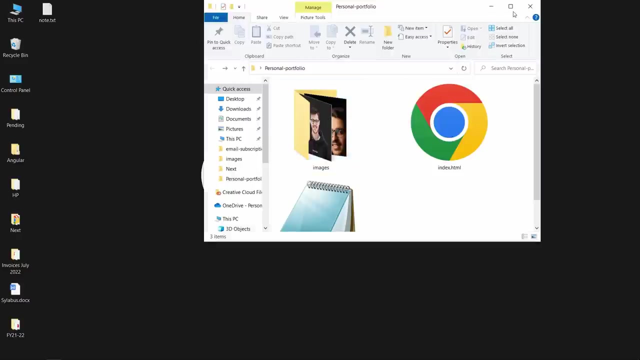 adding one color code for the dark color and then write color. it will be white. that will be the text color. after adding this, let's come back to the folder and in this folder here you can see the html file and css file that we have just created using visual studio code. 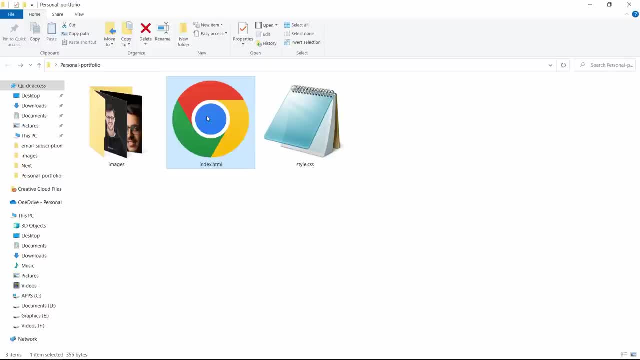 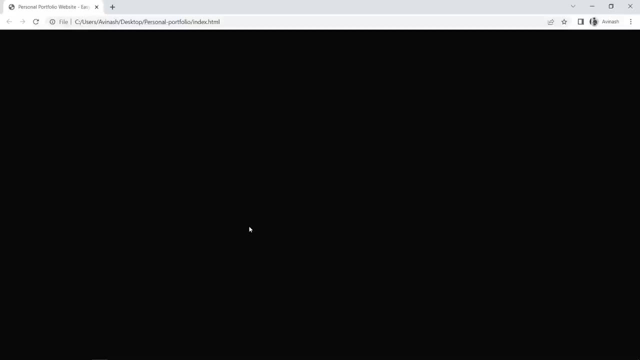 so let me open this html file with any web browser. you can right click on the file and select open with your browser. i will select google chrome so you can see this dark color, because we have added dark background for the body. now let me close this browser and. 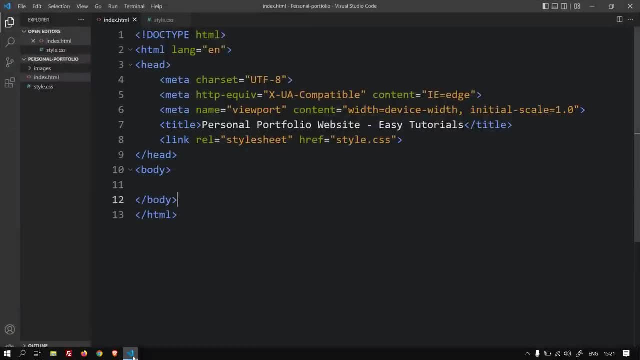 there is an another option to open this browser. let's come back to the visual studio code, and in this visual studio code i have added one extension called live server. you can see in this extension list i have live server installed in this visual studio code. so now, 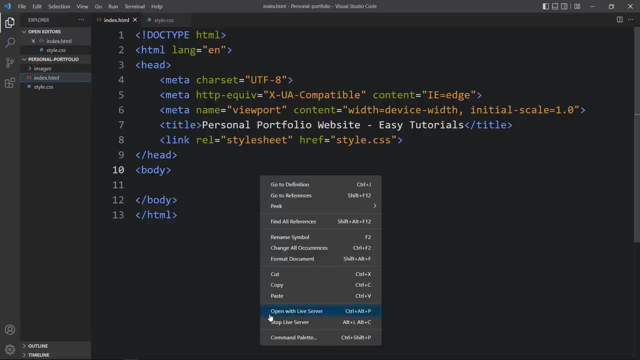 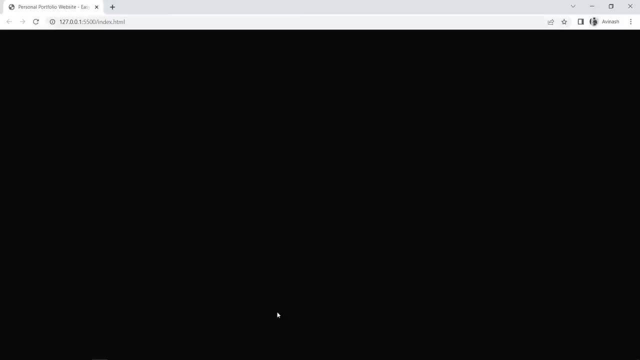 i can open this web page with the live server, right click and select open with live server, so it will refresh the website automatically whenever we will add any changes in the code file and then save the code file, so you can see the same web page, but the url has been changed. that's it. so now let's come back to 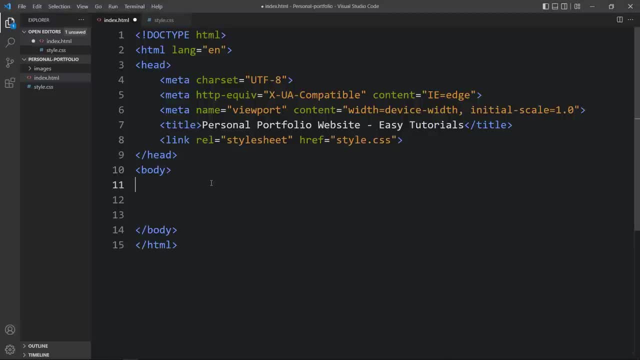 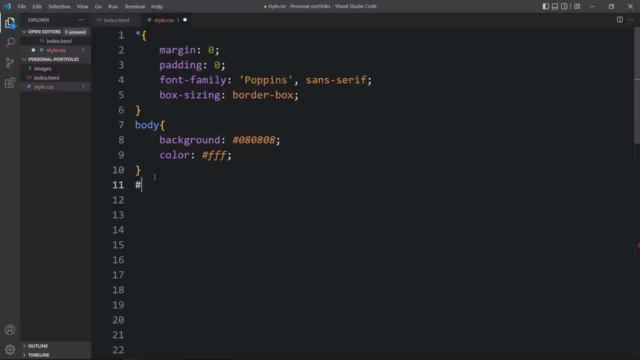 the html file. so in this body let's add one div and we will add one id for this div, which is header, like this: now in this header we have to add the background image. so write this header over here with the hashtag, because it is an id. so in this header we will add the width and height. 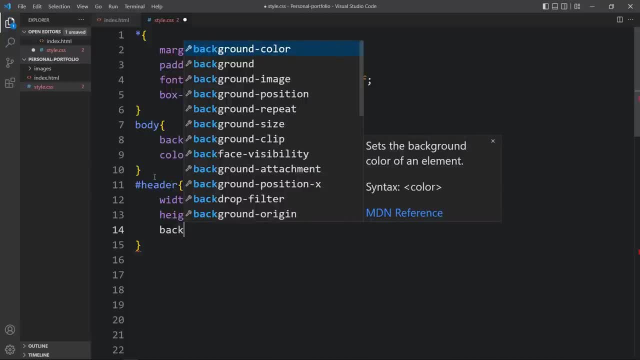 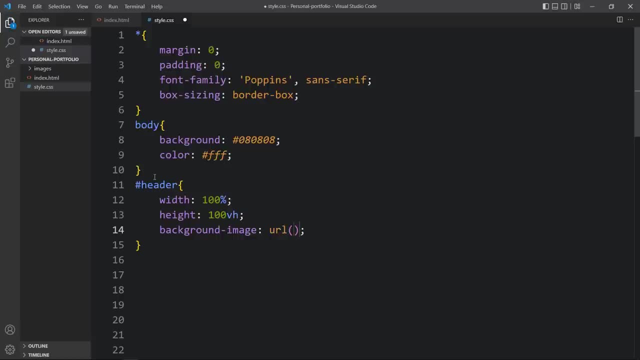 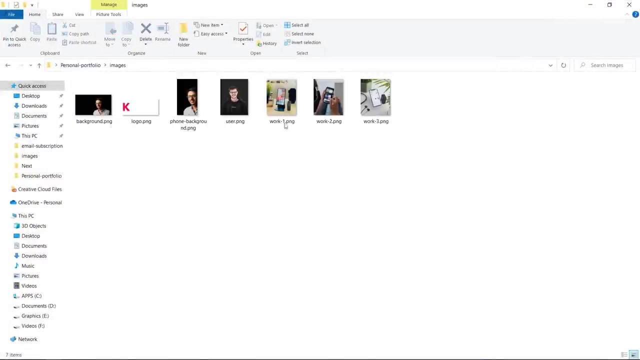 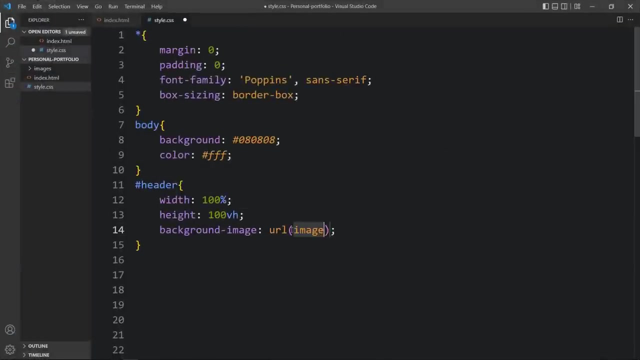 after that we have to add the background. so here let's add the background image url, and in this url i have to add the file path of the image. so you can see the image is in the images folder and the file name is backgroundpng. so here we will add images, which is the folder name: slash file name, which. 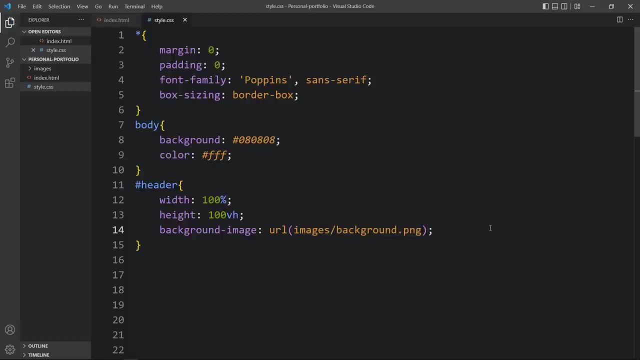 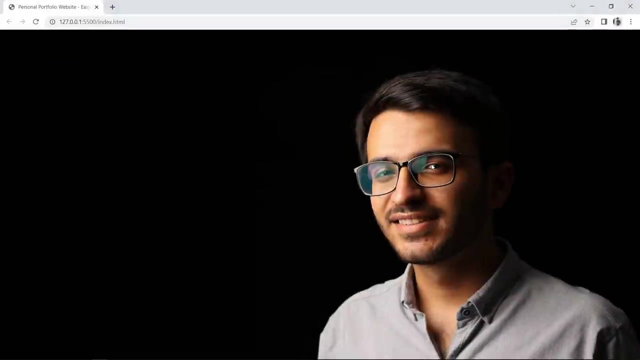 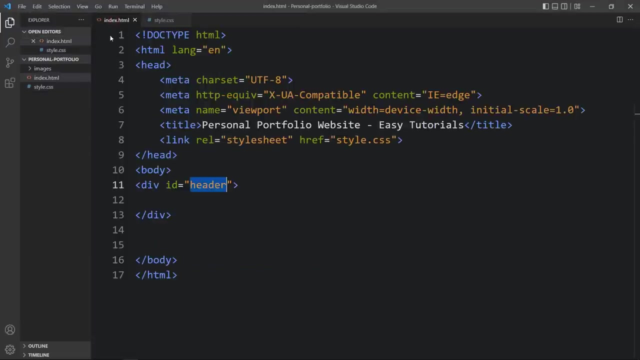 is backgroundpng, then we will add background size and background position. after adding this, let's refresh our website again so you can see this image in the background of this webpage. next we have to create the navigation var, where we will add the logo and some menu. so let's come back and in this header first, we will add one another div with the class. 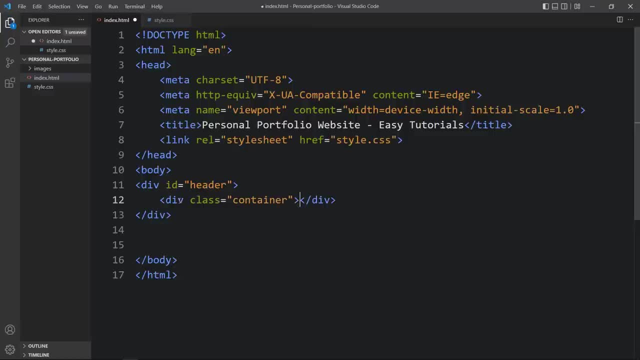 name container. so for this container we will add some padding. after that we will add nav tag and in this nav there will be one logo. so right, i have a logo. so i am going to add this logo. so i am going to add this logo. so i am going 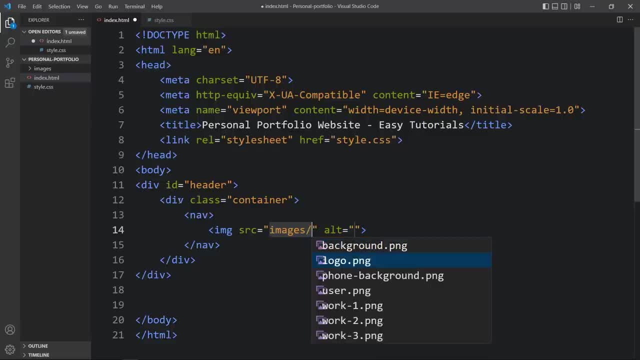 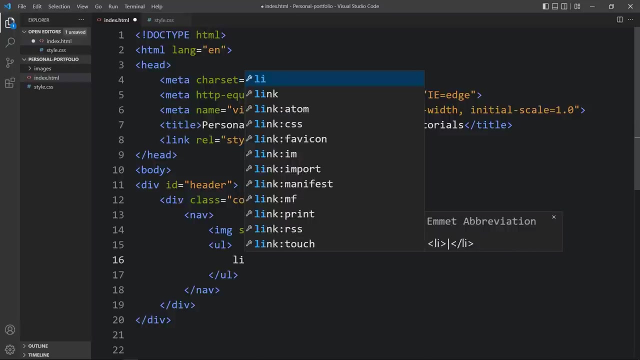 to add. this is ng tag to add one image file path of the logo- images slash logo- and we will add the class name also it is logo. after that we have to add the list of menu, so we will add ul and li for unordered list. in this li we will add a tag so that it will be a 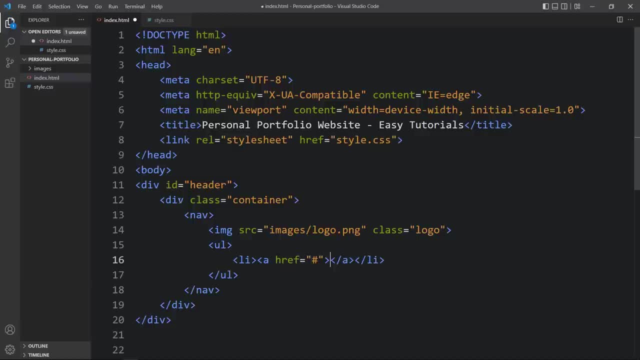 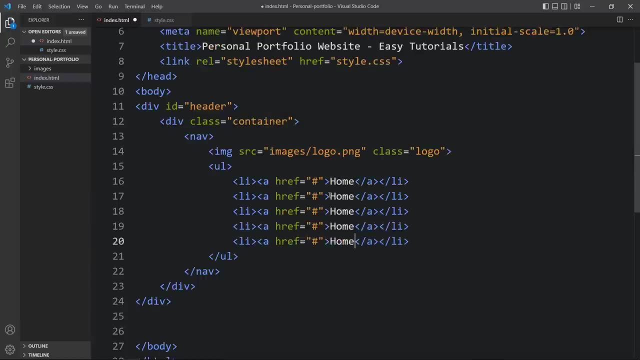 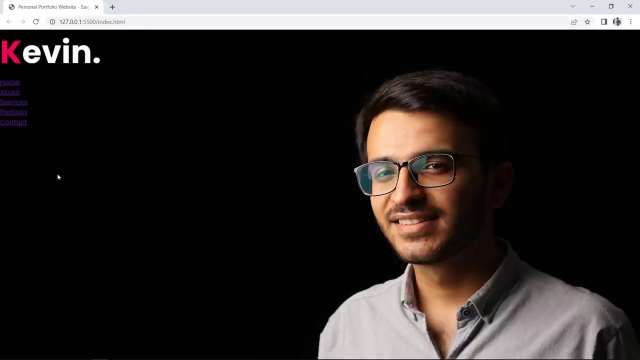 clickable link and write the link text. it is home. just duplicate it print. change the link text. so let me add the another link text. let's come back to the webpage again. here you can see this logo and this link in the top left corner. now we need some space from the left side, so let's come back and first we will add: 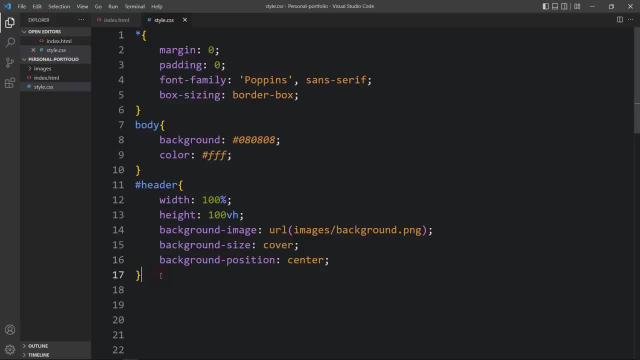 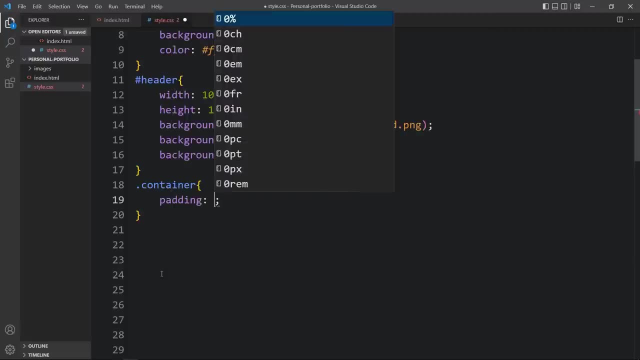 the CSS for this container, write it here in this CSS file. so in this container we will add some padding. it will be 10 pixel from top and bottom and 10% from the left side and right side. so you can see we have some space in the left side. 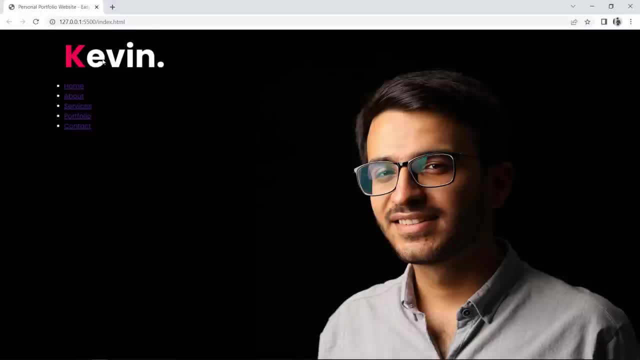 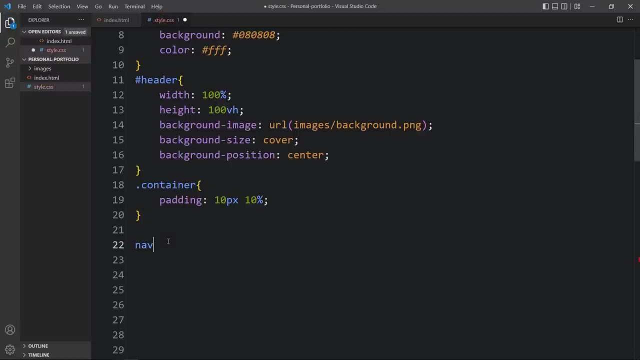 and 10 pixel space from top. next we will add the CSS for the nav tag, where we have added the image for the logo and these menu link. let's come back and here you can see we have the nav tag. so let's copy this one, write it here in this CSS file. so in this nav we will add: 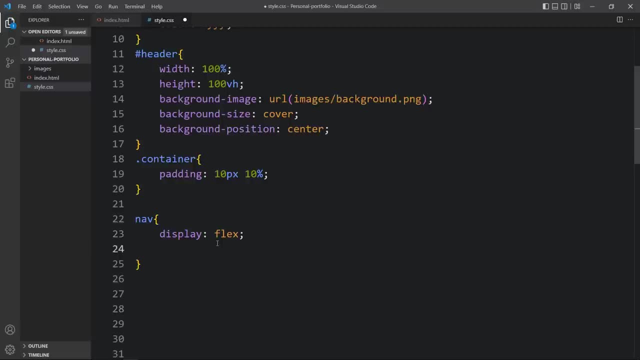 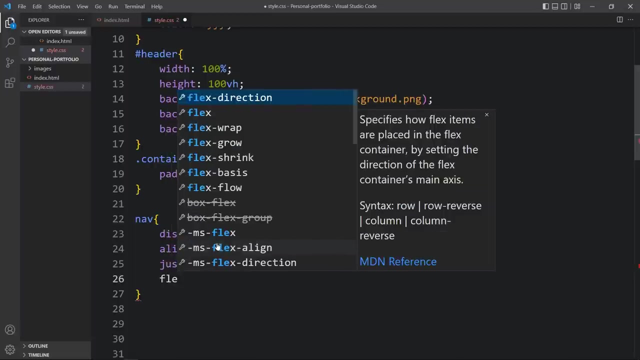 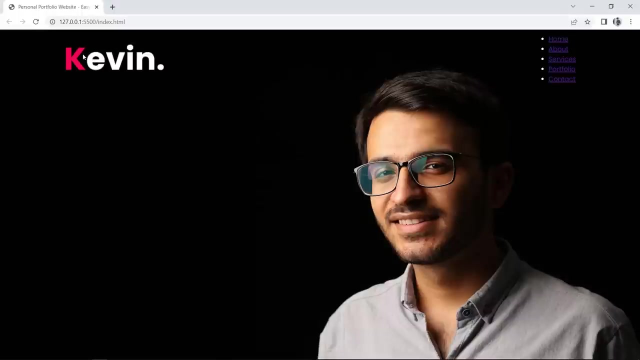 display flex so the image and links will be side by side. align items will be center and justify content it will be space between wrap will be wrap. now you can see this logo image in the left side and these menu links on the right side. still, we have to change the size for this logo and then we will change the alignment. 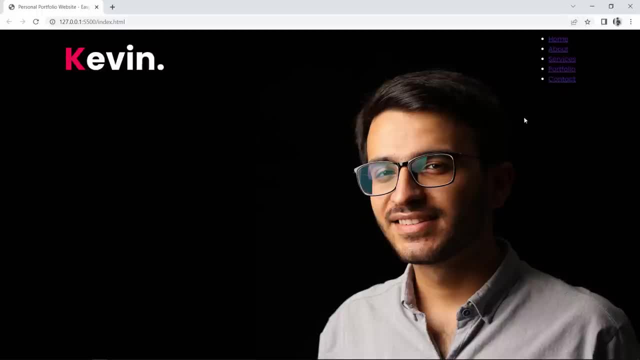 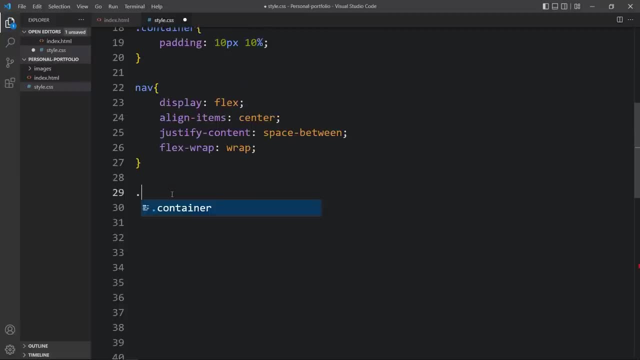 for these menu links and we will change the color. so let's come back and here you can see we have added the class name logo. so we will add the CSS for this logo. write it here, and here we will add the width for this logo. it will be. 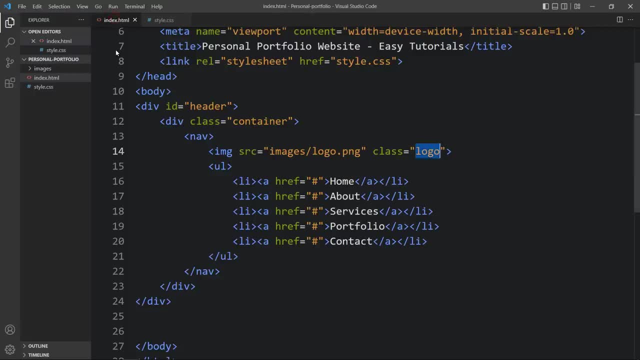 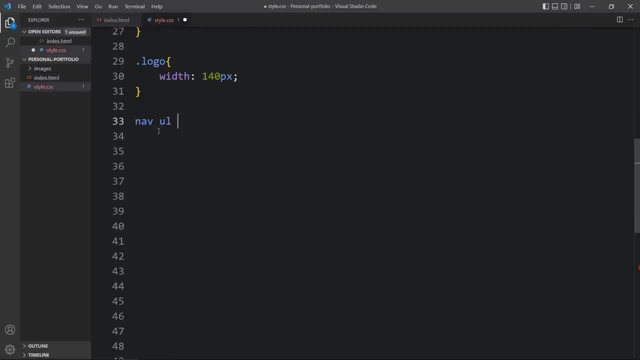 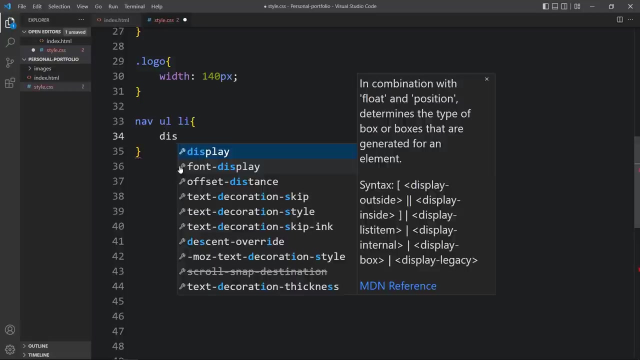 and this: it will also be 1 and it will be x writing. so this a will be 14 and it willau a. it will be expressed as context장을, it will be 140 px, and after that we have the link text in uI, al and e. so first we will scanbrokerphp visual as method forizard. 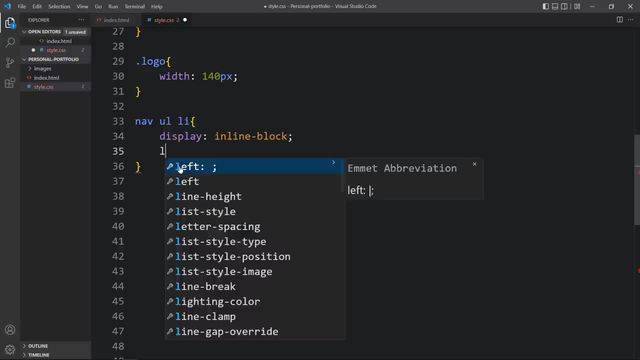 abnavul AMD a li. so for this l I we have to add the display. so right, display inline block, so it will be horizon yazillian lists style will be none, and after we will add display alignment block, so it will be horizontally aligned list her style will be none, and after that we will add the displaylow disabilities will not be insufficient- and into a archive event, so to that we have a hybrid of this SnapShj estrella, and then after that we will 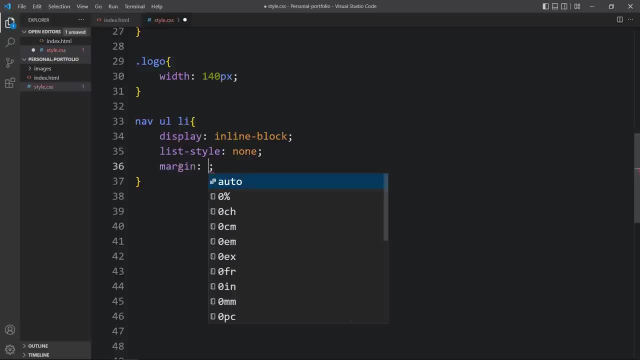 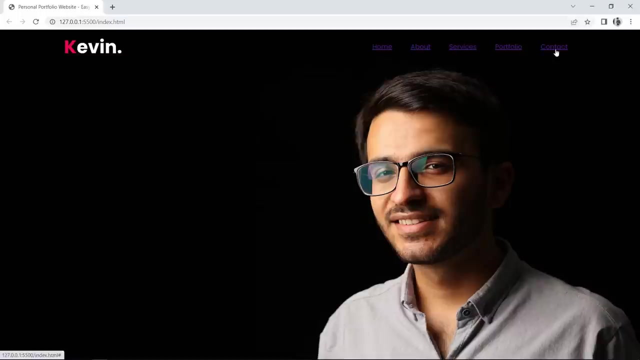 add margin so we will get some space between all the links. it will be 10px from top and bottom and 20px from left and right side. now you can see these links are horizontally aligned. next we have to remove this underline and we will add the white color. so let's come. 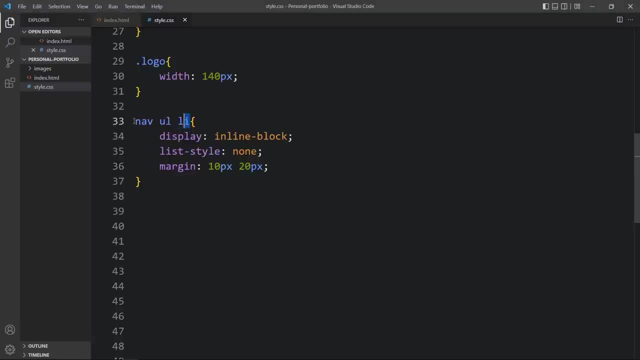 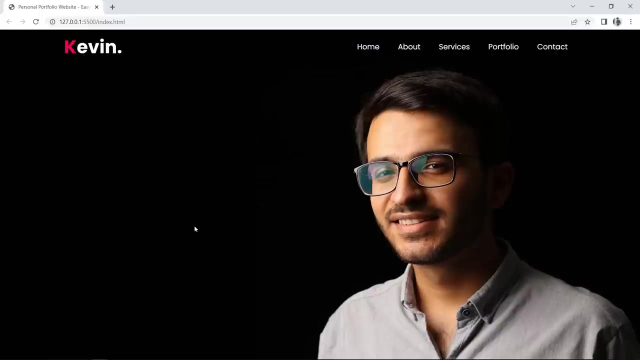 back and here we will add the same thing, then write a, so for this a tag. we will change the color, it will be white. then remove the text decoration: it will be none, so it will remove the underline. now we will add the font size: it will be 18px. so these menu links looks. 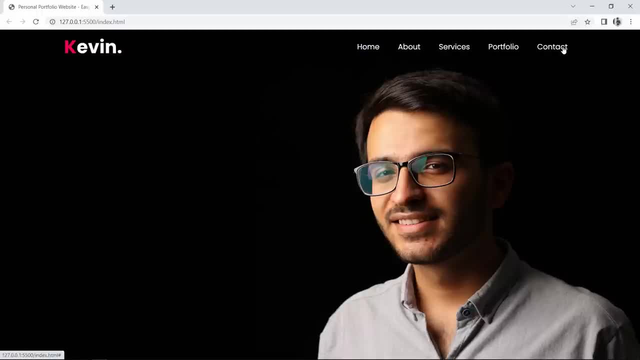 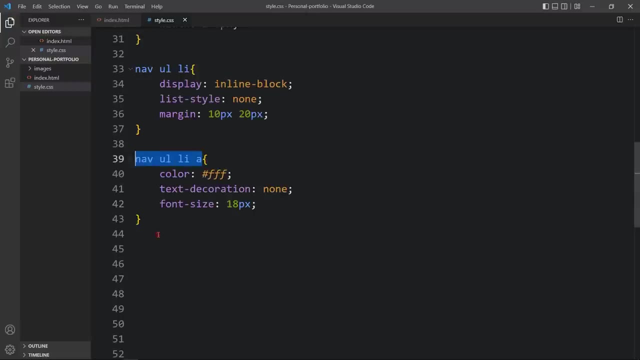 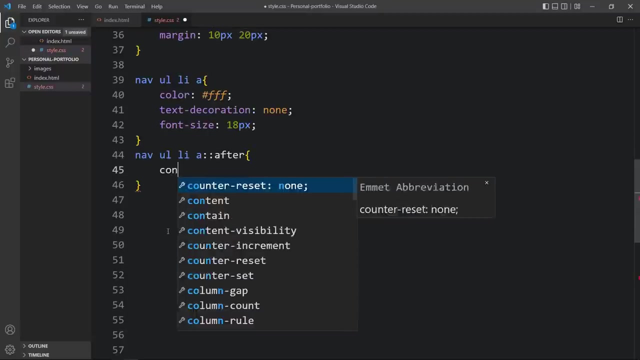 good home about services, portfolio and contact. next, we have to add the hover effect on these links. for that let's come back. so, and here we will add this one- then write double colon after. in this one we will add content. content will be empty. then we have to add the width. width will be 100%, then we will. 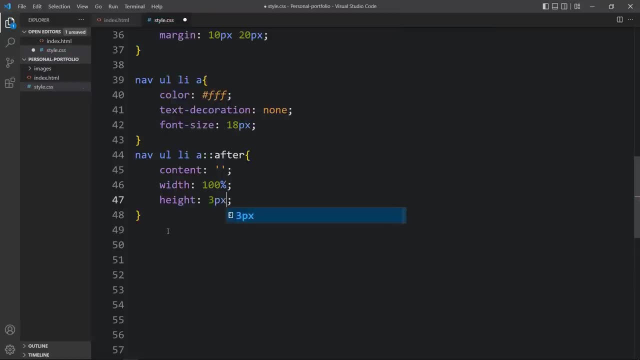 add the height, 3px and background. in this background we will add one color code after that position. position will be absolute, left it will be zero and bottom minus 6px. and here we are adding position absolute. so in this a we will add position relative. 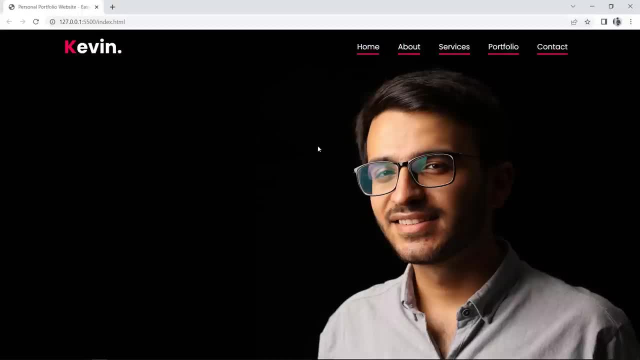 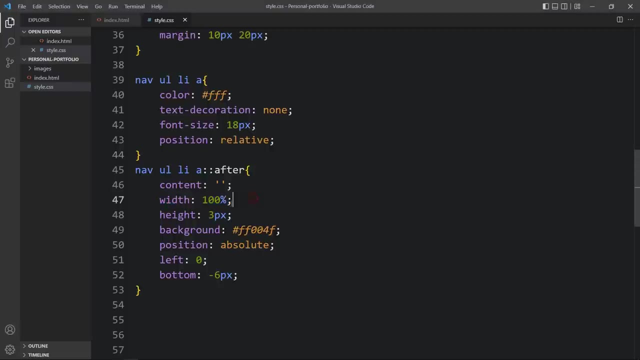 after adding this. so this HOWCAL WE АрWING OF SERVICES, let's refresh the website again. now you can see this colored line in all the menu links, so we have to hide this line and it will be visible whenever we will tick cursor over any menu link. for that, lets come back, and here you can see we have added the width 100%. 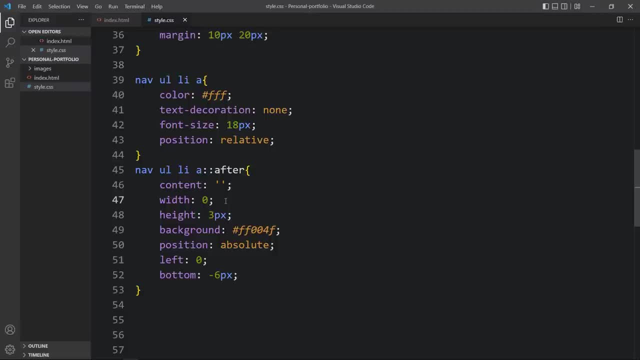 so we will make it 0, so it will be hidden. now we have to enable this line whenever we tick cursor. for that, let's copy this one, write it here: write hover and double colon after, like this, and here we will add the width 100%. so whenever 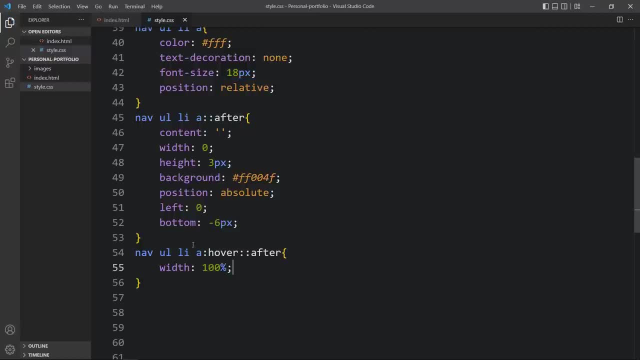 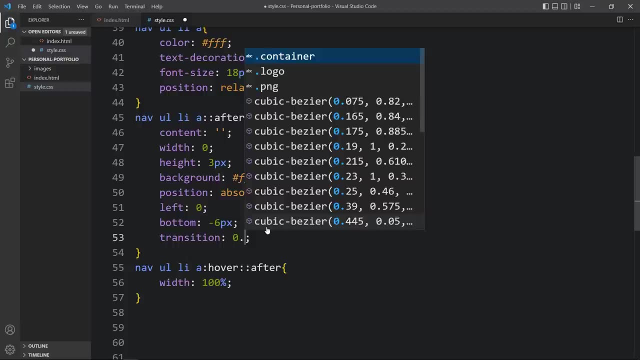 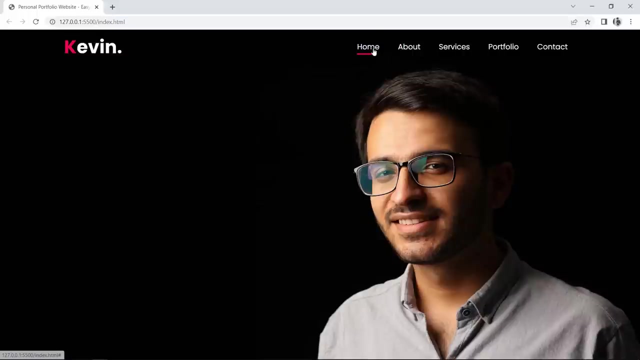 width will be 100%. it will be visible and in this after we have to add the transition, so it will be 0.5 seconds. after adding this again, come back to the website and here you can see, if i tick cursor, this colored line is coming at the bottom of each menu links. 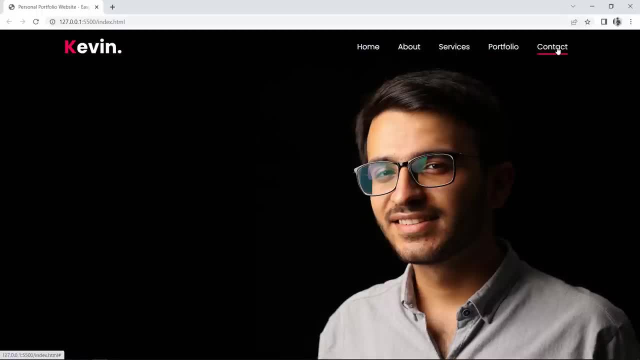 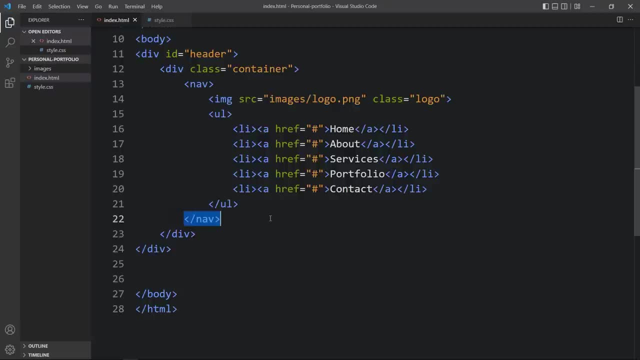 so this animated hover effect looks good. next we have to add some text and title on this screen. so let's come back in this html file. after closing of this nav tag, we will add another div with the class name header text. now we will add one small text in p tag. then we will add another text in h1. that will be the main title. 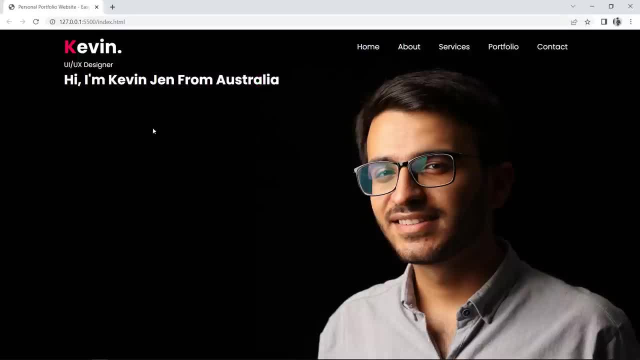 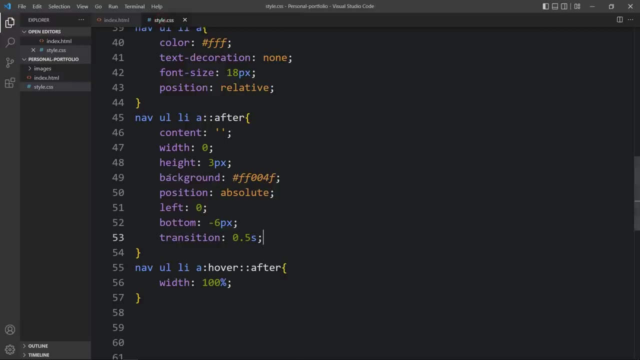 after adding this text, let's refresh the website again. here you can see this a small text and this large text. now we have to change its position and we will change the font size also. so let's come back and copy this class name header text. write it here in this header. 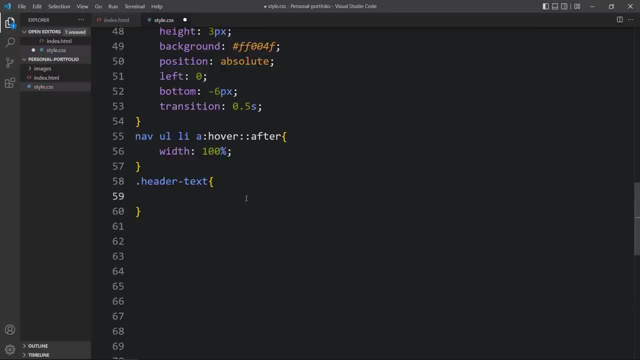 text. we will add the css properties. so first we will add summer space from the top, so margin top it will be 20 percent. then we will change the font size, it will be 30 pixel. next copy this one, then write h1, because we have another text in h1. so here we will add the. 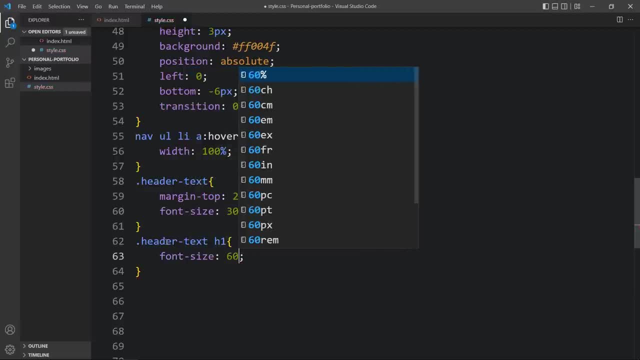 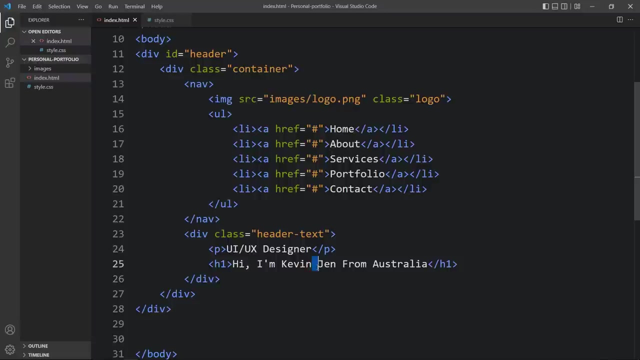 font size. it will be very large- 60 pixel, and some margin from the top- 20 pixel. so this text is very long, so we have to add one line break over here. so let's come back in this html file and after this text we will add br to change the line. so it will add a line. 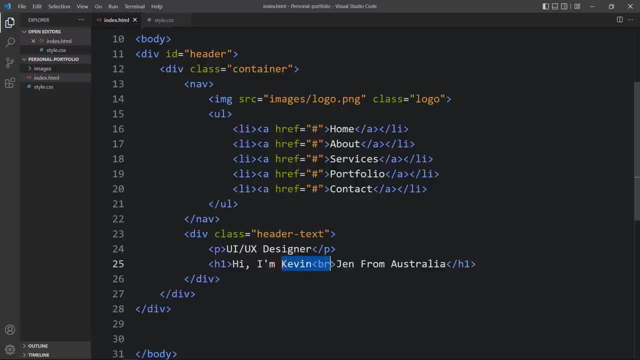 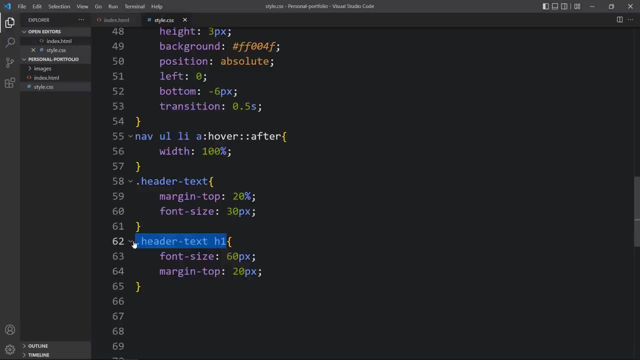 break here and for this cabin we will add the color. so here we will add span open and closing tag. span open tag here and close it after this text like this, so you can see this text in two lines: let's come back to the css and copy this one, then write span. 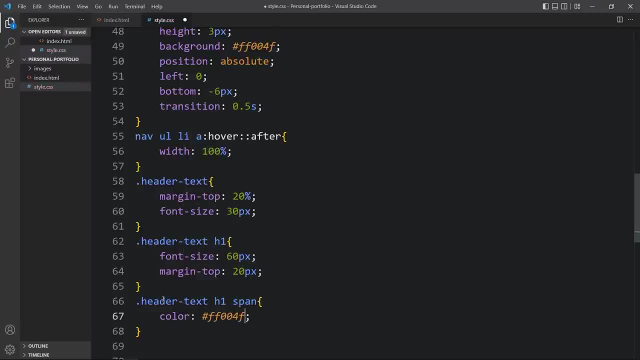 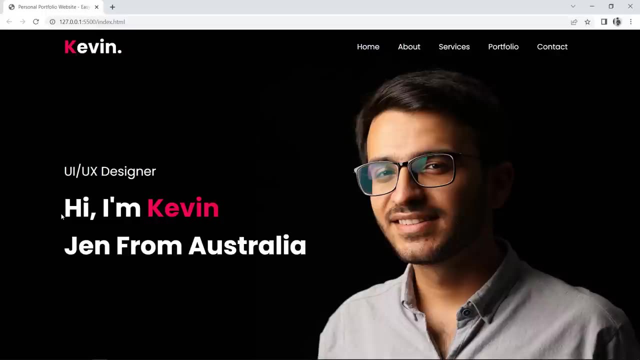 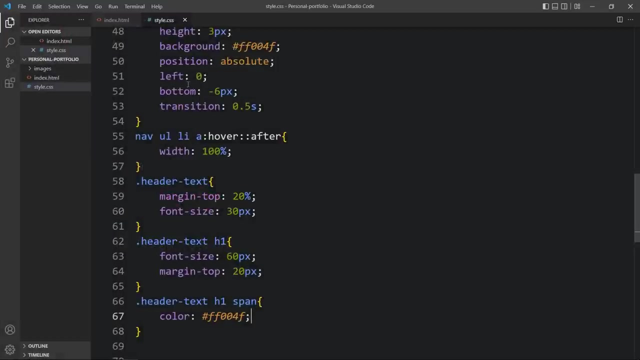 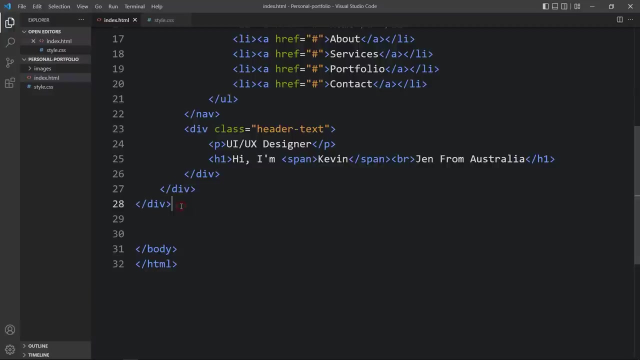 and write the color, this one, so you can see this color in this text. so we have completed the header section of this personal portfolio website. now we will create the about section. to create the about section, let's come back to the html file. and this header section is closing here, so here we will add another div with the id. 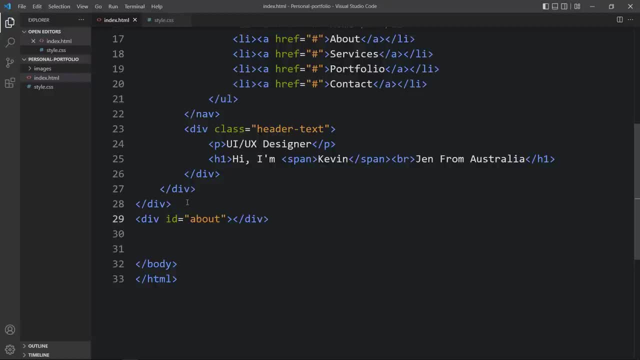 about div id about in this one. again, we will add one div with the class name container and within this container we have to create two columns for that. we will add one div with the class name row and in this row we will create two columns. so first we 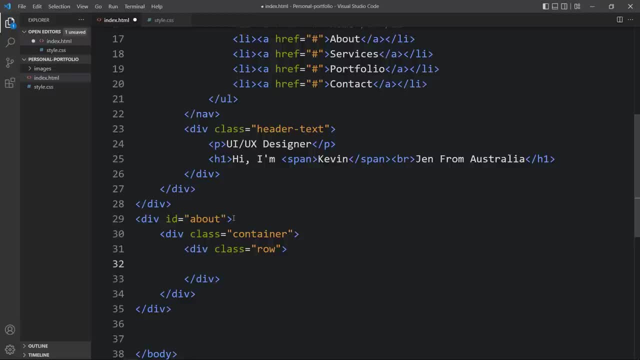 will add one div with the class name about call 1, which is for the first column. so this is the first column. let's duplicate it and write about call 2. that will be the second column. so in the left column we will add the image and in the right column we will add 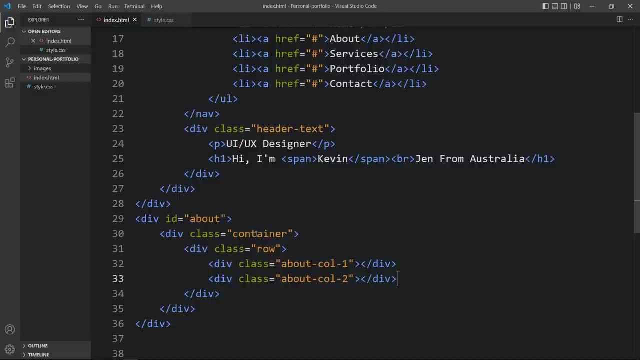 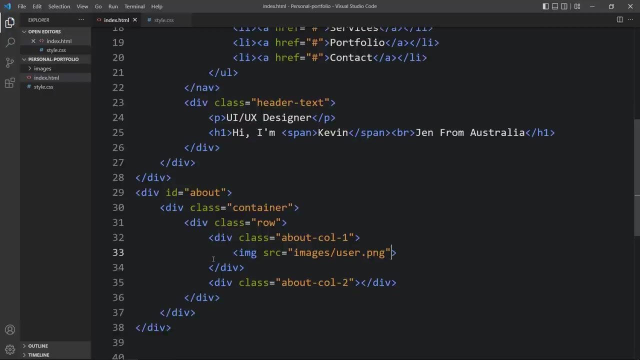 some text, so we will add one image in the first one. so here we will add one image with the img tag images slash file name, which is img userpng. that's it. and in the right side we have to add one title. so let's add one. 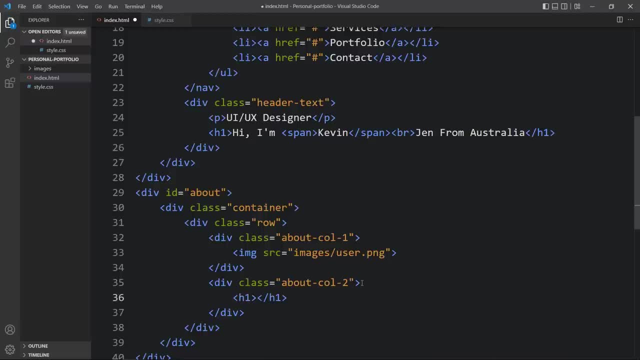 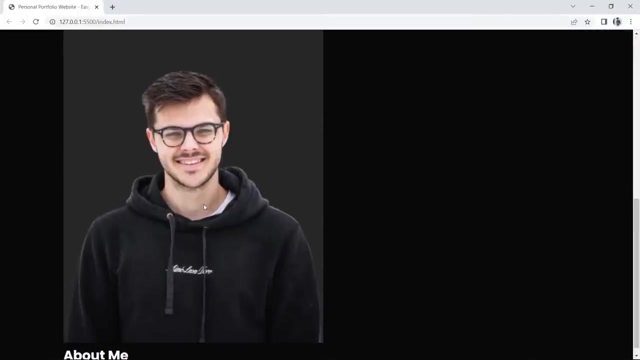 title in h1 tag and this will be the text about me, like this: after adding this, again refresh the website. you can see this image and this text below this image. so we have to align this side by side. this image will be in the left side and this about me text in the right side. so let's come. 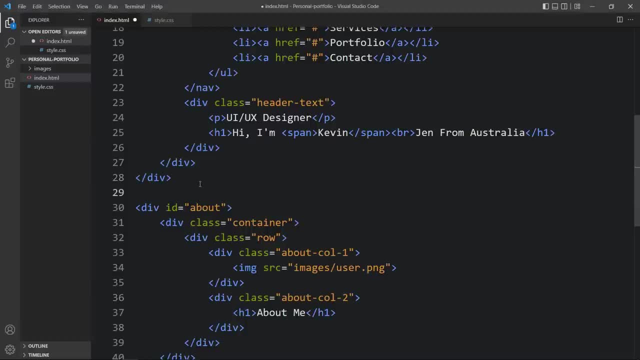 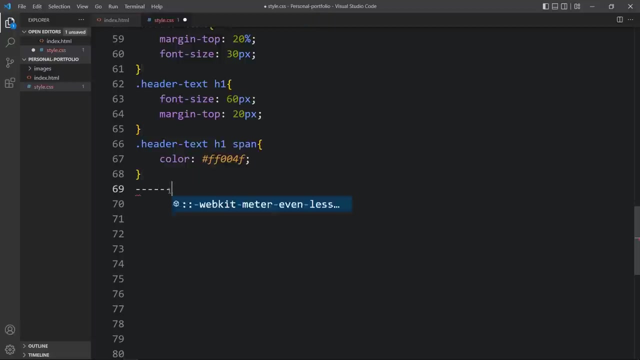 back. let me add one comment here, so it will be easy to read this code. here we will add about. come back to the css file. here also we will add one comment about css file, about, about, about, about, about, about. so here we have to add the css for the about section. so let me come back to the html file. 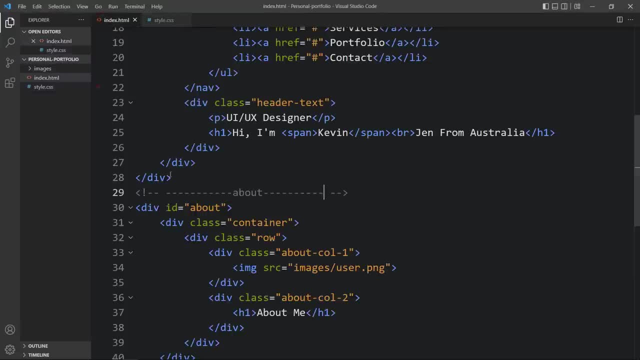 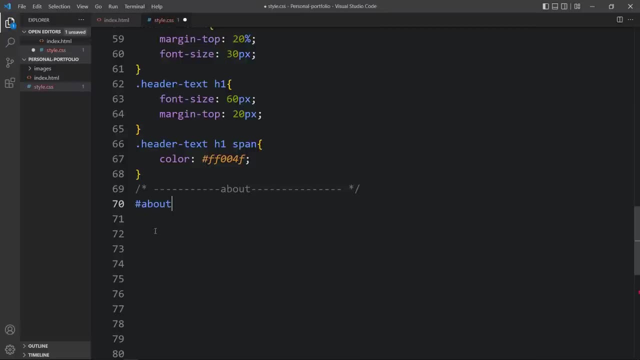 and here you can see we have added the id about. so let's copy this one and paste it here with the hashtag. let's add some padding. it will be 80 pixel from top and bottom and 0 from left and right. then we will add the color here. we will add different color for the text. 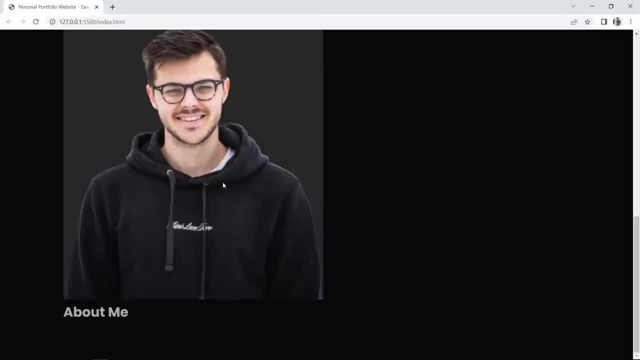 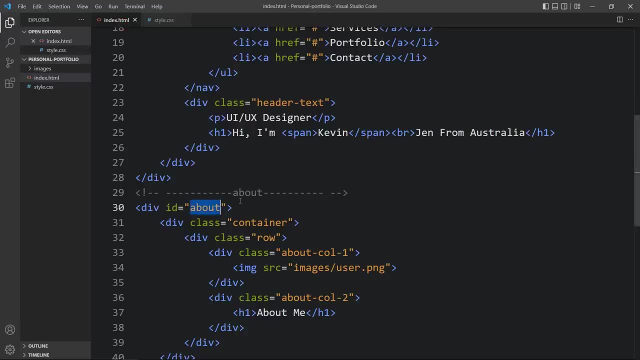 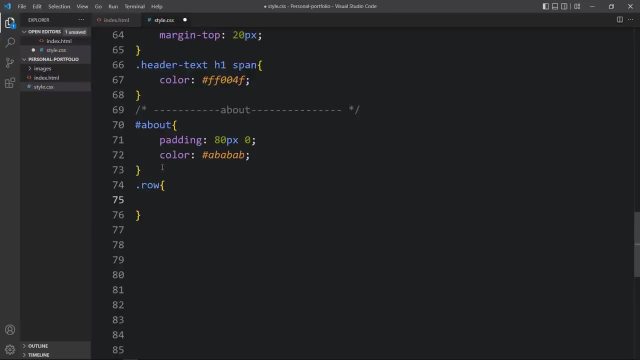 so you can see some space above this image and below this text, and the text color is also changed. let's come back, and here we have the class name called row. write this class name here, dot, row, and, and here we will add display. display will be flex, so we will get the contents side by side. 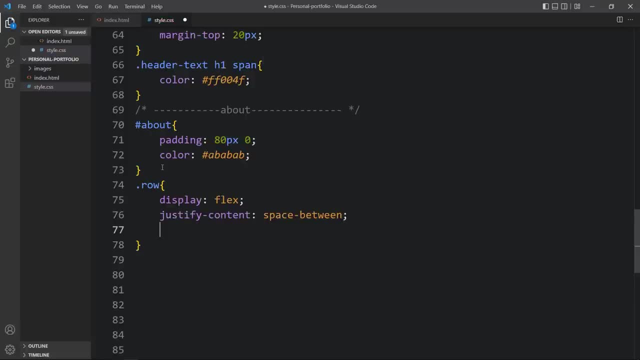 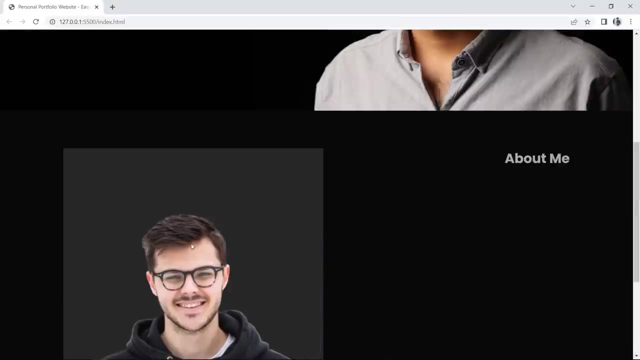 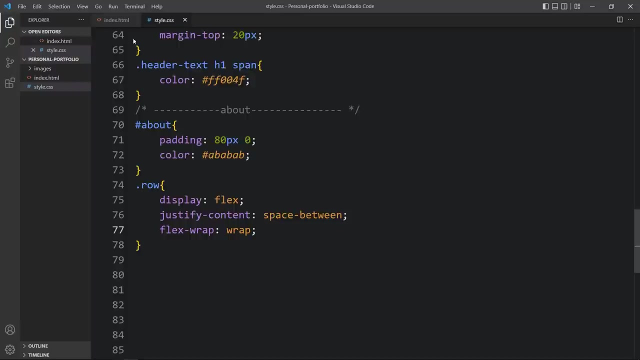 justify content. a space between and flex wrap, wrap. so you can see this image left side and this text in the right side. now we have to decide the width for the first column and the second column. so let's come back and here you can see we have the class name for the column about: call one and. 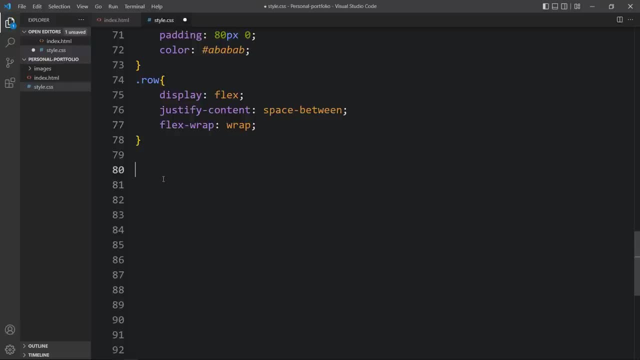 about call two. write this class name in the css file. so for the first column we will add flex, basis 35. it means the width of the column will be 35, and in this one we have the image also. so write the same class name, then img. so in this image we will add the width, it will be 100, then border radius for the image. 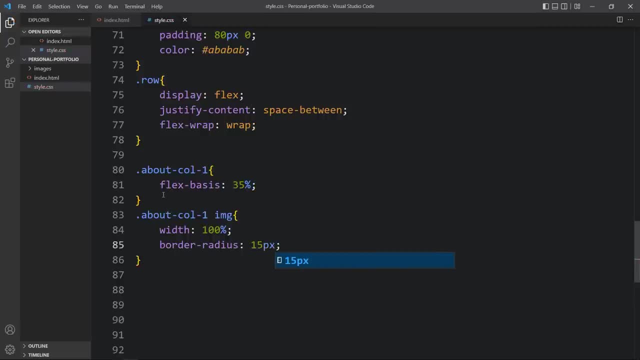 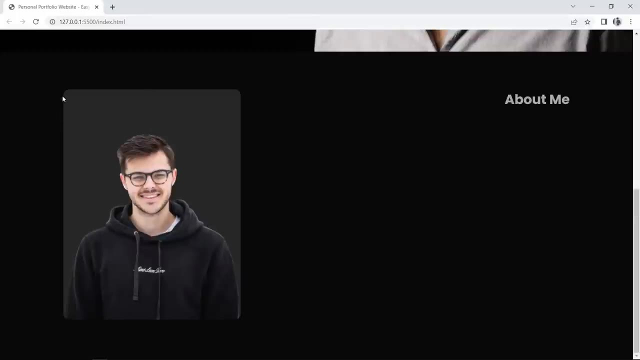 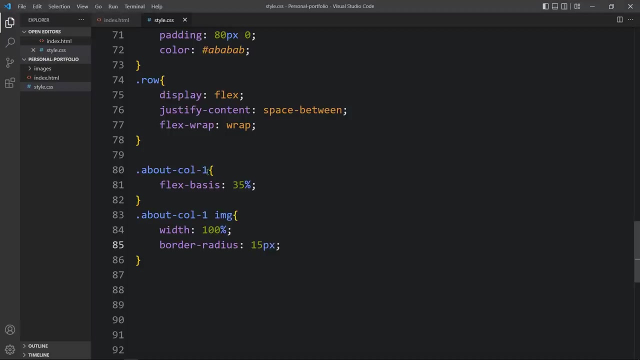 it will be 15 pixel, so the corner of the image will be round. so you can see the perfect size for this user's image and the corners of this image is round. now we have to fix the width of the right column. so again write this class name and change the class name. it is column 2, so for 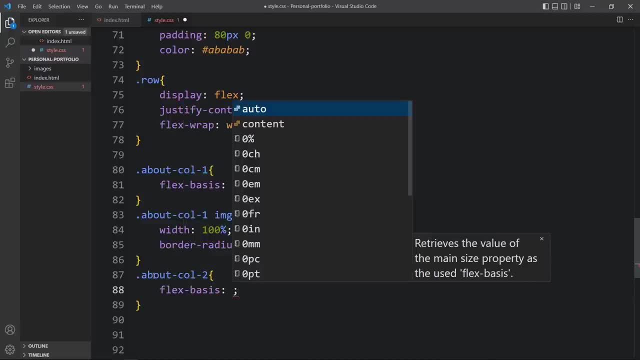 the second column, flex basis will be 60%. so you can see, in the first column we have added the width of 35% and the second one width of 60%, so we will get the 5% space between both the column. you can see the second column is starting from here and we have some space. 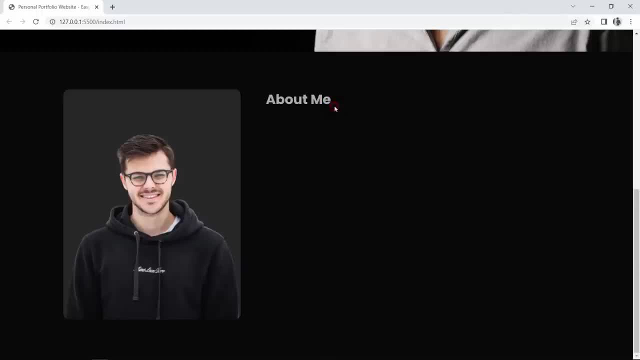 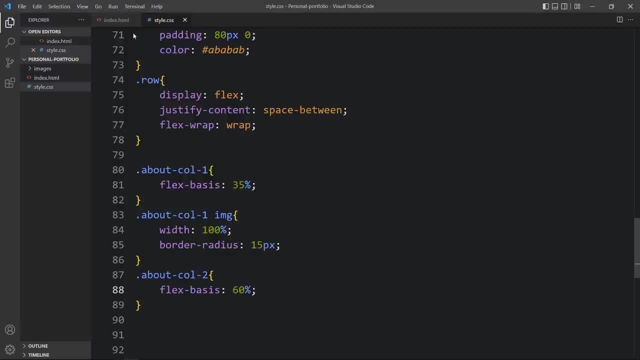 between the 1 st and 2 nd column. Now we have to change the font size and color for this text. so lets come back and here in this H1 we will add a class name. so we will add an Calendar jámbric Inside the collection. do we have got a single bar列? Just a write. 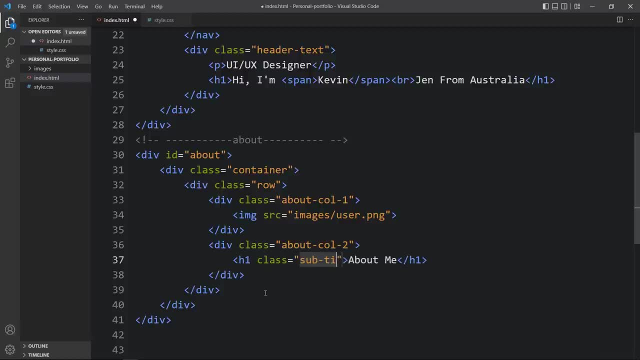 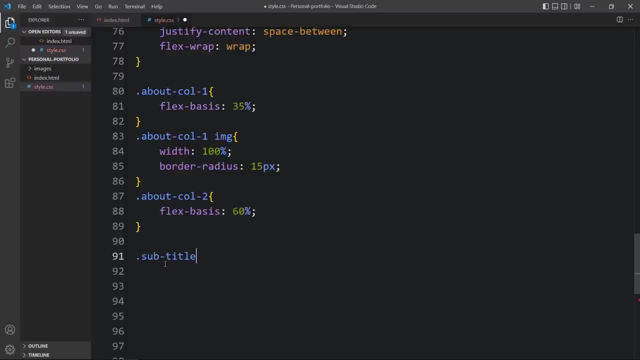 an teenagers: Ramji Br Barnes. This color first field will be. the background head is entered. add a class name subtitle and copy this class name subtitle. write it here. for this subtitle, we will add the font size: it will be 60px, then font weight 600 and color will be white. 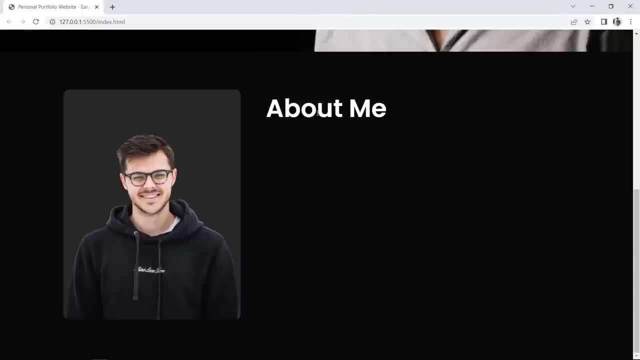 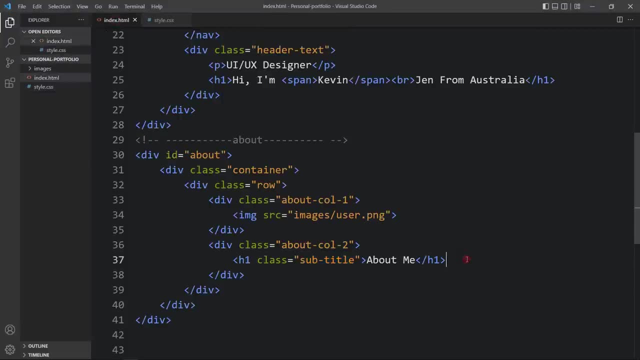 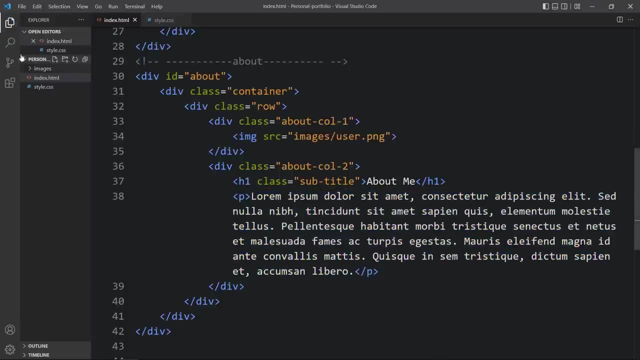 so you can see increased font size for this text. after that we have to add some description in this second column. so lets come back to html file and here, after this h1, we will add text in p tag. we have added this text using p tag. you can see the text on the web page. 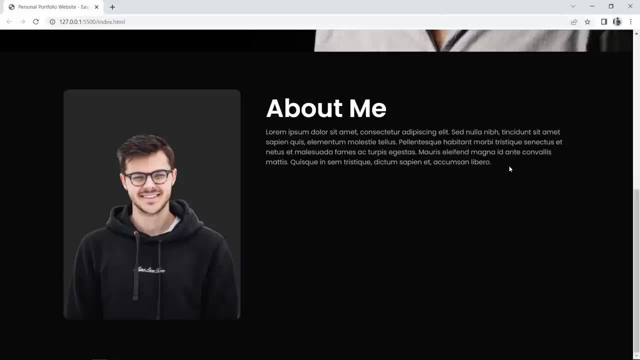 next we have to add 3 tabs, and in each tabs we will add different content. here we will add three tabs. in the first one we will display the skills, and in the second one we will display the experience, which is work experience, and in the third one we will display the information. 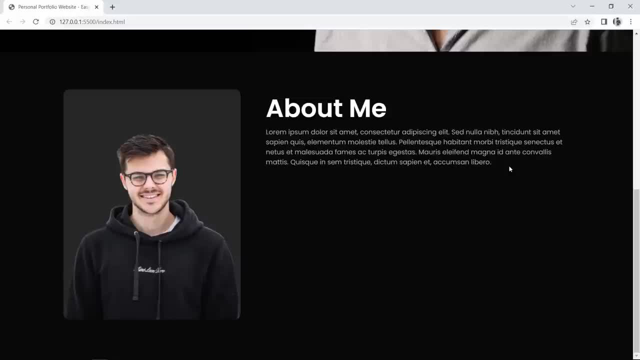 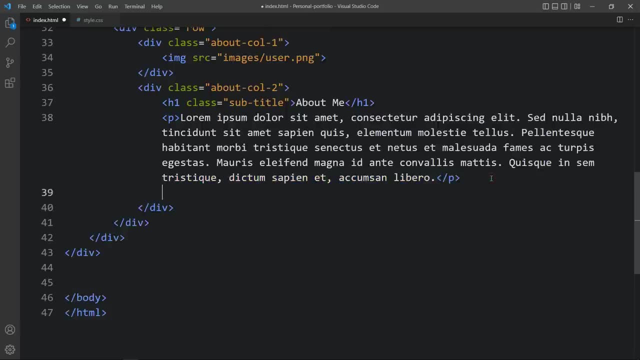 about the education. so to create the tabs, let's come back to the html file and after closing of this p tag here we will add one div with the class name, tab titles, and in this tab titles there will be three title. so let's add one p tag and in this p 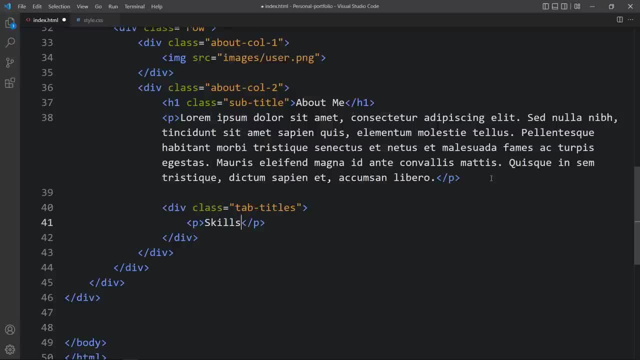 tag we will add the title skills, like this and with this p we will add a class name. so let's add the class name of tab links like this and let's duplicate it here. we will add another title, which is experience, and in the third one, education. you can see it is like this: skills. 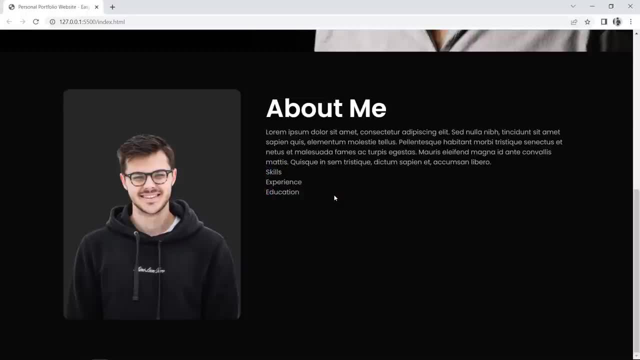 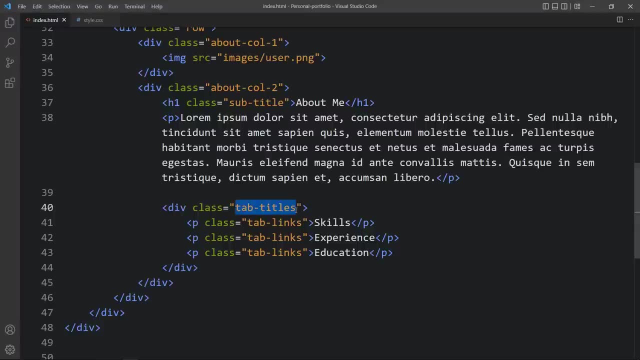 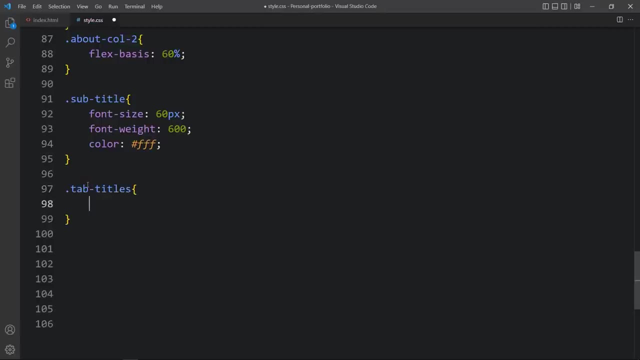 experience and education. now we have to align it. so let's come back and copy this class name tab titles. write it here in this css file. for this tab titles we will add display. display will be flex, then margin: it will be 20 pixel from top, zero from left and right and 40 pixel from the bottom. 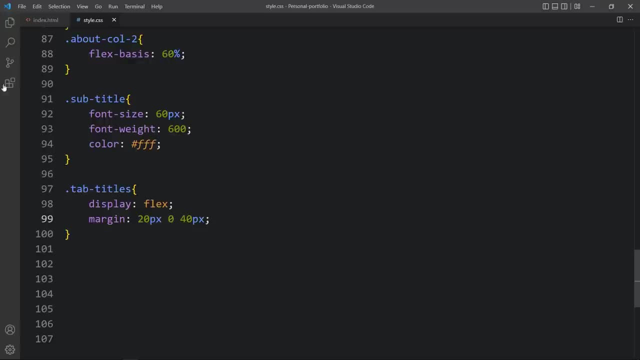 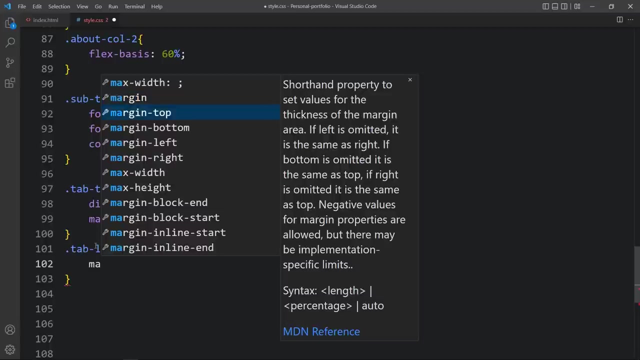 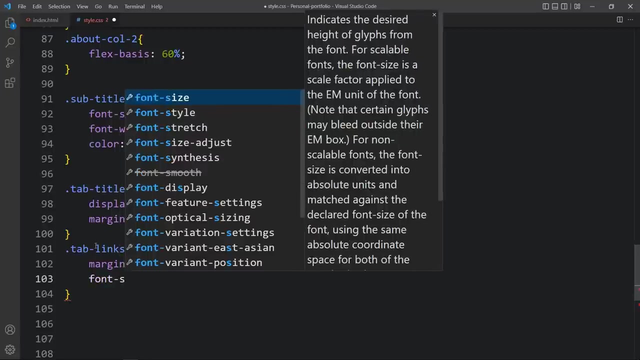 and in this one we have the class name called tab links for the individual tab titles. so write this class name: tab links. here we need some space from the right side margin. right. it will be 50 pixel, then we will add font size. it will be 18 pixel, then increase the font. 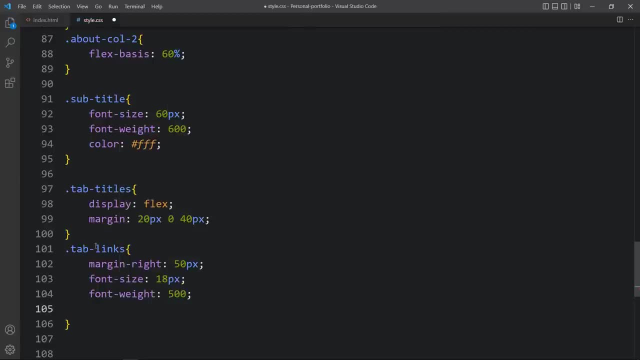 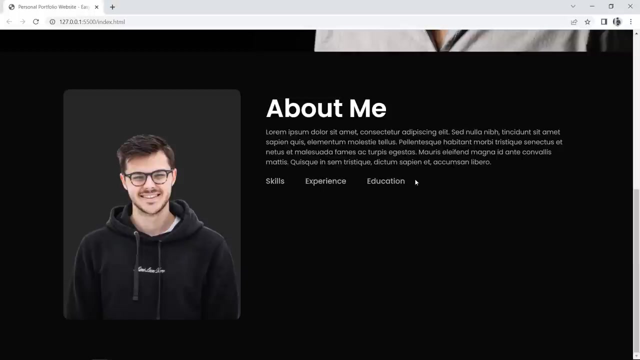 weight cursor will be pointer and we will add the position relative so you can see it is horizontally aligned. we have the bold font weight and we have some space between each tab links or tab title. next we have to add one underline in this tab title. so we have to add one underline in. 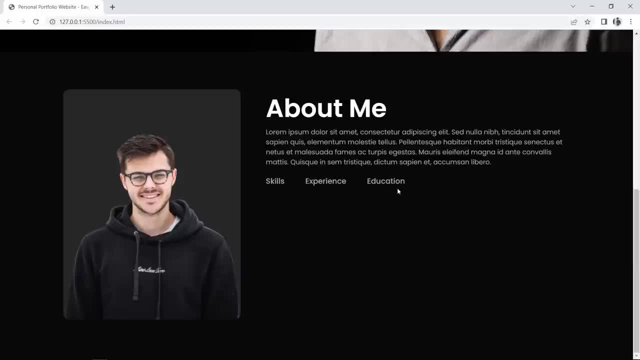 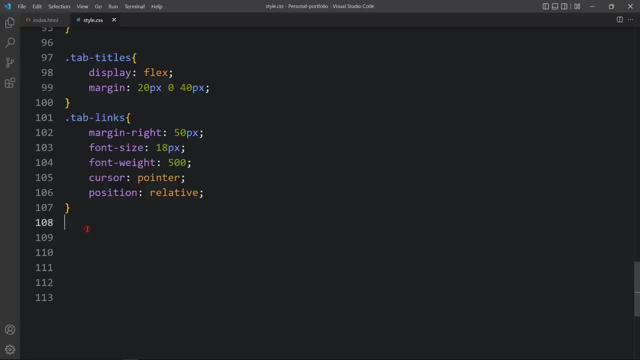 this tab title. next, we have to add one underline in this tab title. so we have to add one underline in the first one and it will be visible in other also whenever we will click on anyone. so for that let's come back and here we will add this tab links double colon after. 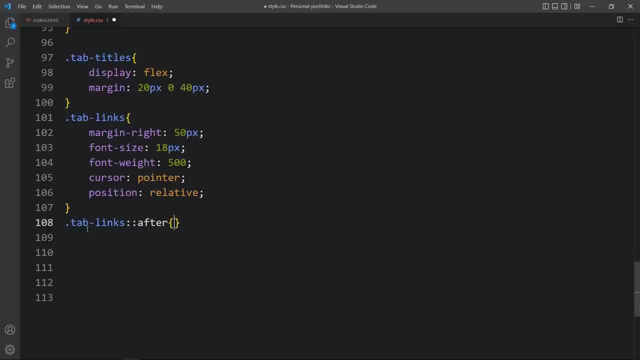 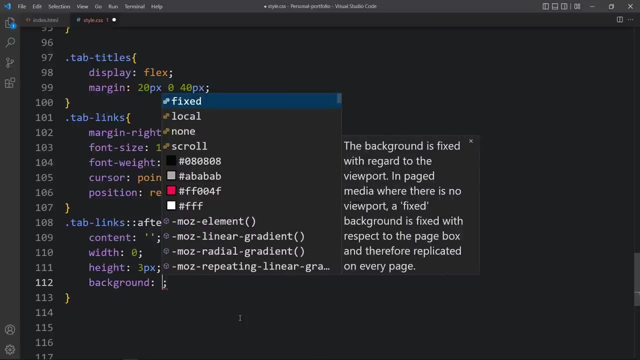 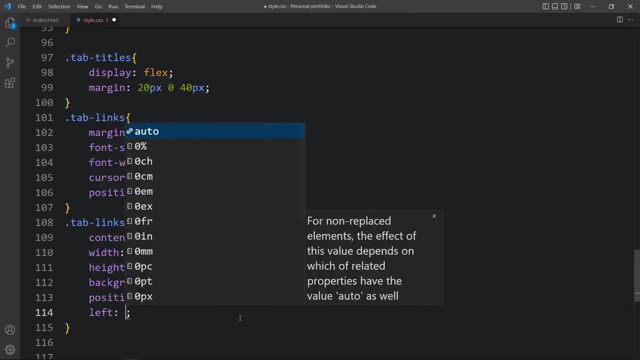 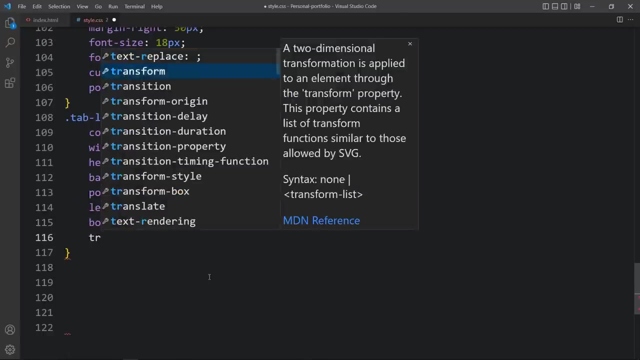 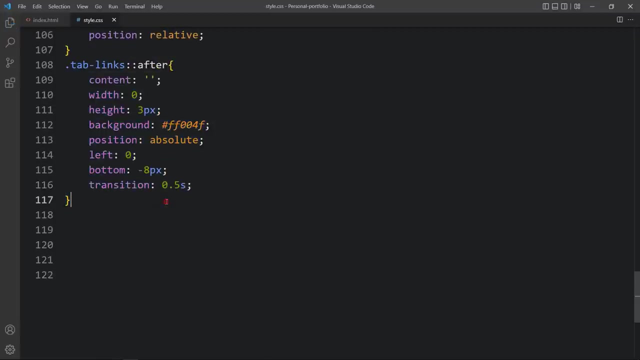 here also, we will add content: empty, width it will be zero and height, 3 pixel, as we have added in the navigation menu. then background: this color code position will be absolute, left will be 0 and bottom minus 8 pixel. then transition: 0.5 seconds. so right now it is 0, so it will be hidden, and now we have to add the width: 100%. so 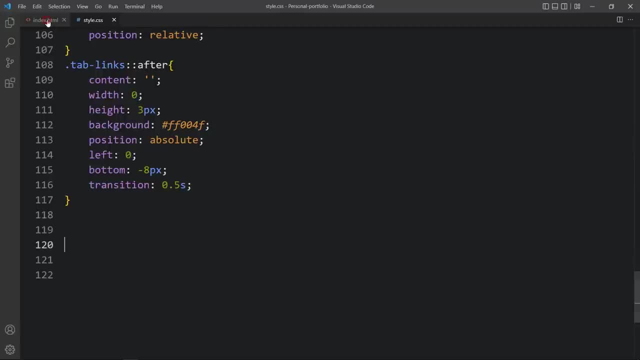 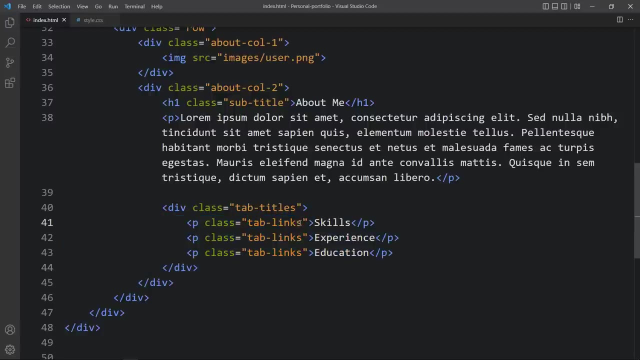 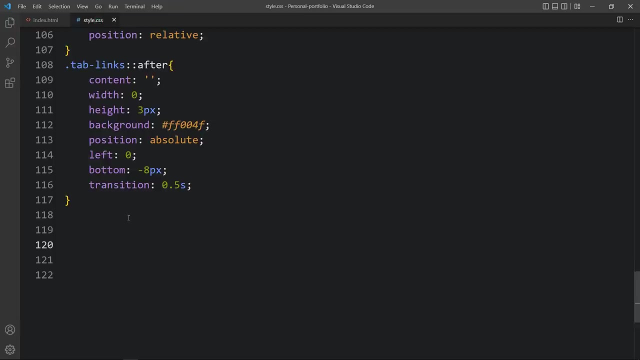 this will be 100% on the first one. so in this first link we will add one more class name. so let's add one space after this tab links. just add one space. and here we will add a class name active link. we have added this class name active link. let's copy this one. come back to the css file. 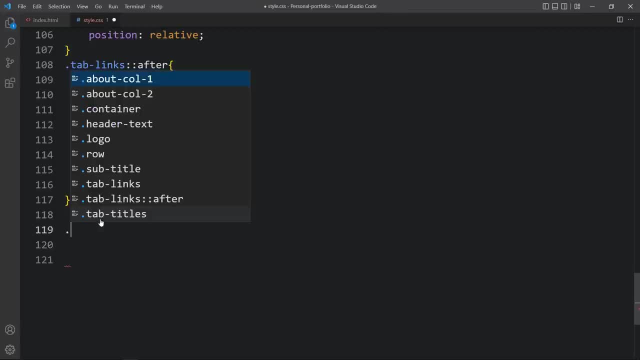 here we will add dot tab links, dot active link. there will be no space between these text. and here we will add double colon after and just add width 50 percent. so it will be visible in which way we will add the width 50 percent. so it will be visible in which way we will add the width. 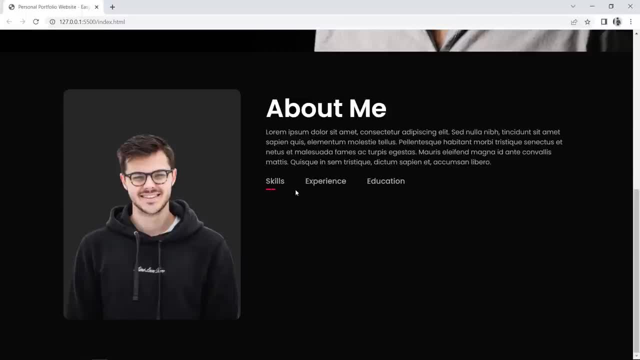 one we have the class name called active link. so you can see it is in the first one, because in the first title we have added the active links class name and it is hidden in the second one and third one. now we have designed this tab title. next we will display the tab contents. so let's come back. 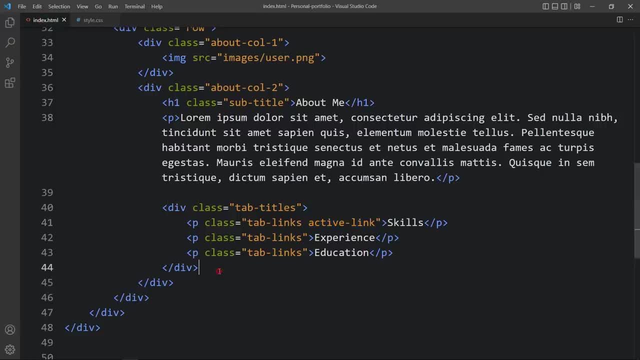 to the html file. after closing of this div, which is for the tab titles, here we will add another div with the class name. after closing of this div, which is for the tab titles, here we will add another div with the class name. tab contents. in this one we have to add the list. so here let's add ul li, and in this li we will add one title in. 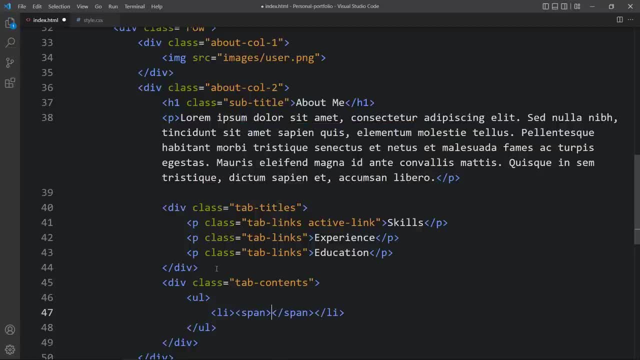 a span tag. it will be ui, ux, and i will add a title in the span tag and i will add a title in the span tag and i will add a title in the span tag. after this span, we will add br, to add a line break like this: pier, and after that we will add another. 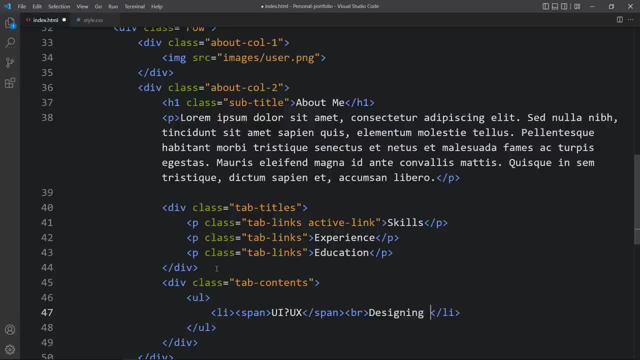 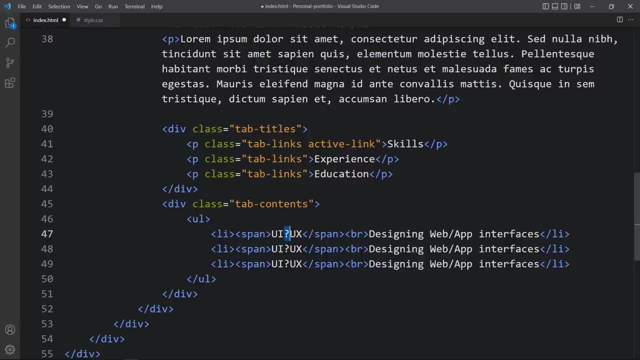 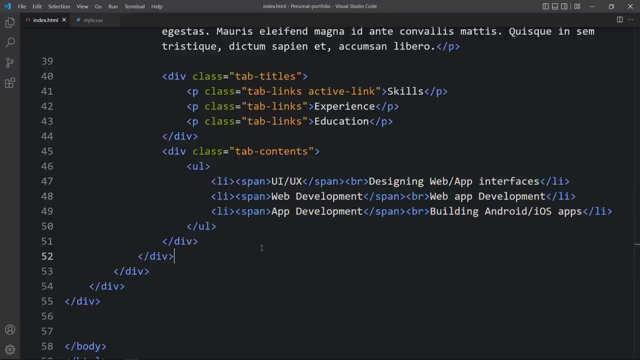 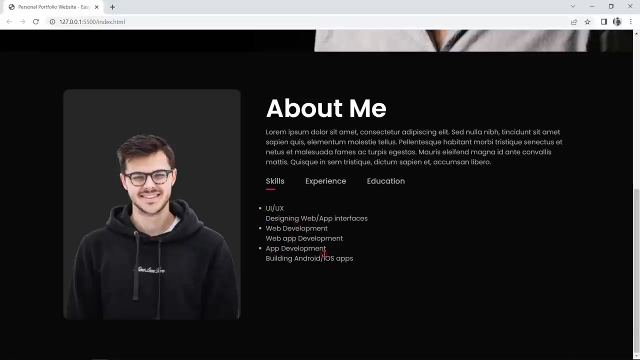 text: designing web app interfaces. so this is the first skill. let's duplicate it and here we will change the title. so here we have added three different list. let's come back to the website. you can see this list here under this skill: to design this one. let's come back to the html file. 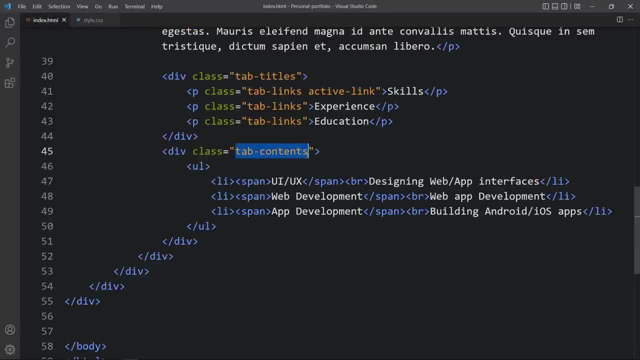 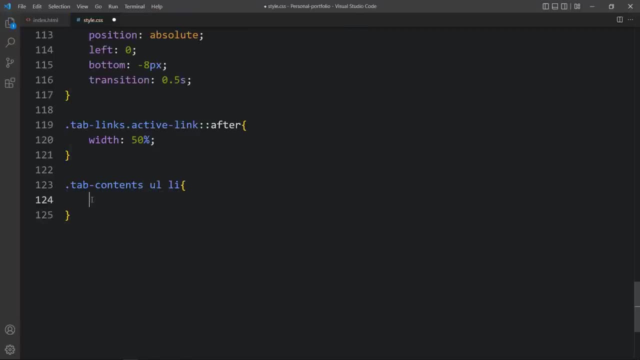 copy this class name tab contents, write it here and here. we will add ul and li list style. it will be none. then we will add the margin. it will be 10 pixel from top and bottom and left right, zero. in this li we have added the span tag, so for 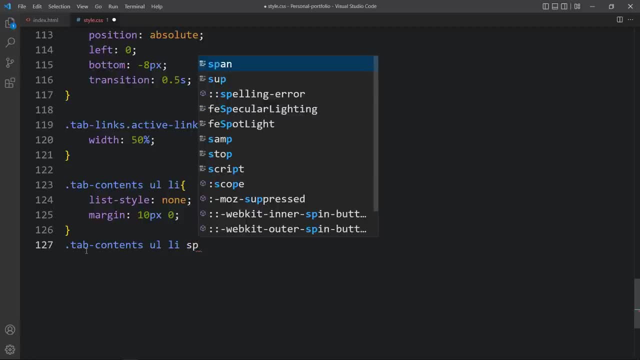 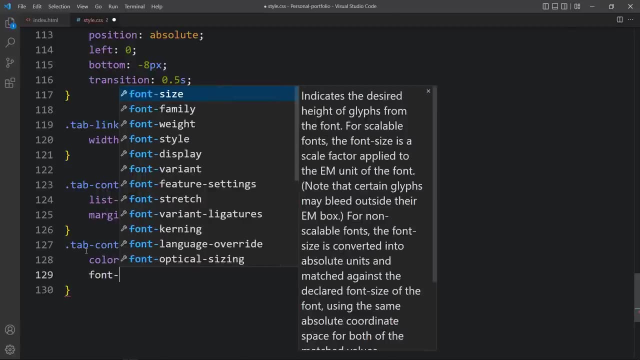 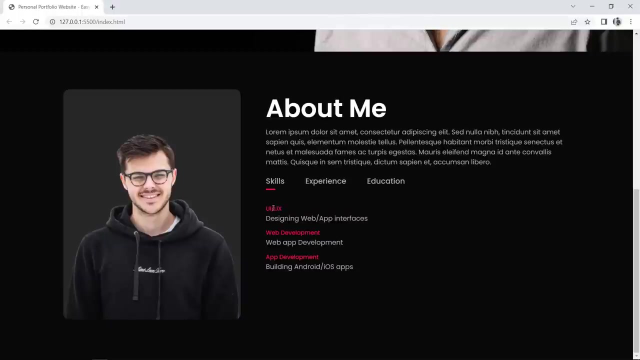 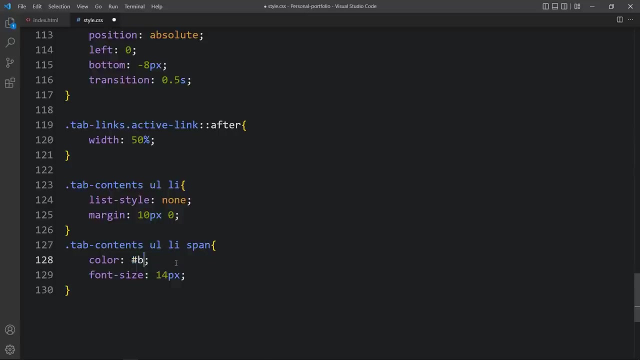 that span. we have to add the color. so write a span and we will add the color. then we will decrease the font size also. font size will be 14 pixel. so this looks good. let me change this color here. we will add another color code. now you can see here. you can see that text is here. now you can see the text is in this: 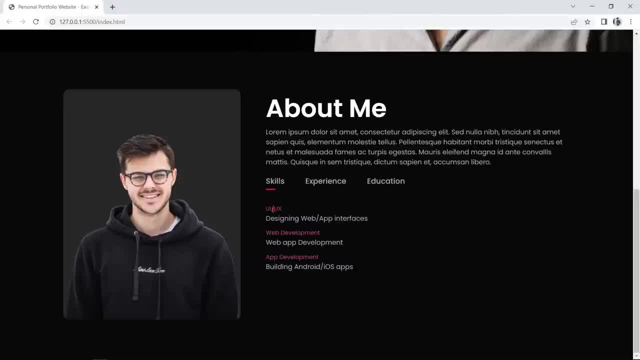 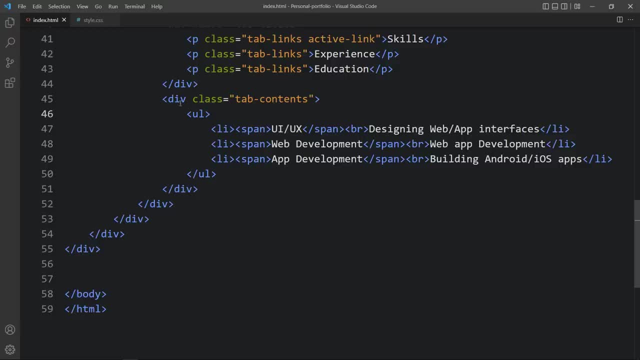 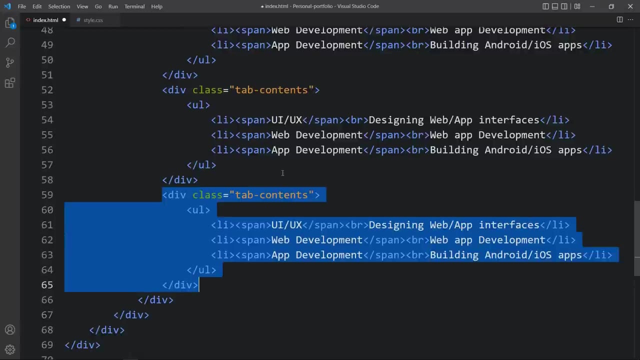 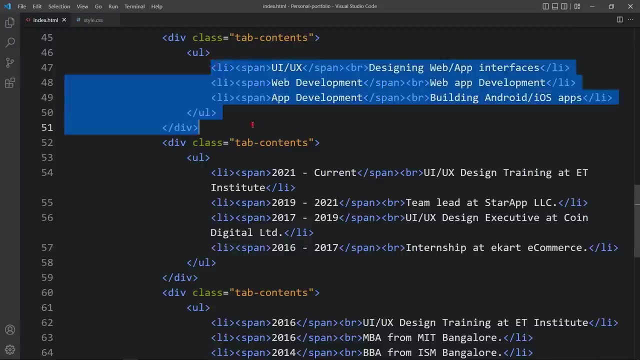 is looking good. next, we have to add the content for the experience and education. so let's come back in this html file and duplicate this type contents here. it is just duplicate this one and replace these contents. now i have replaced these text in the experience and education, so let's refresh the website and 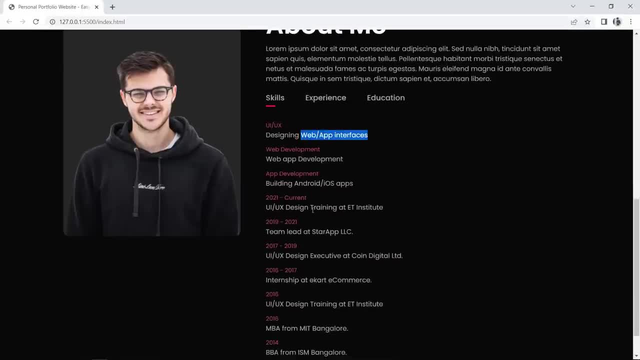 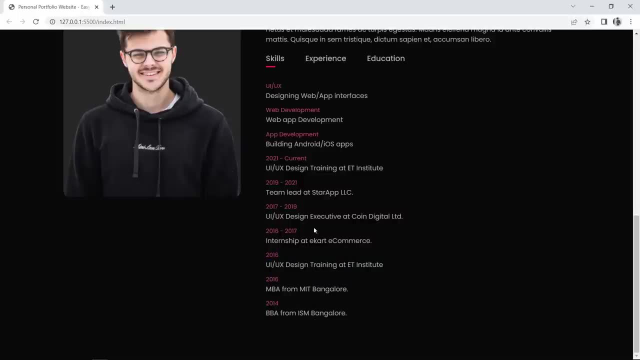 here. you can see, this is for the skills, this is for the experience and this is for the education. but right now, all these contents are displaying at a time, so we have to hide the experience and education. it will be feasible whenever we will click on this one. so let's come back. 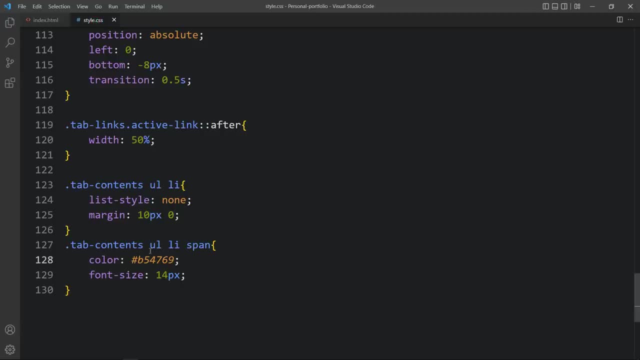 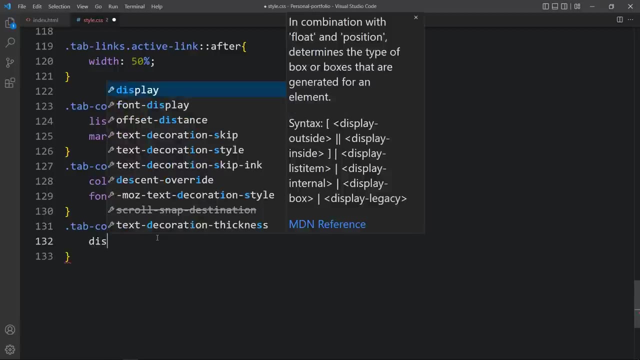 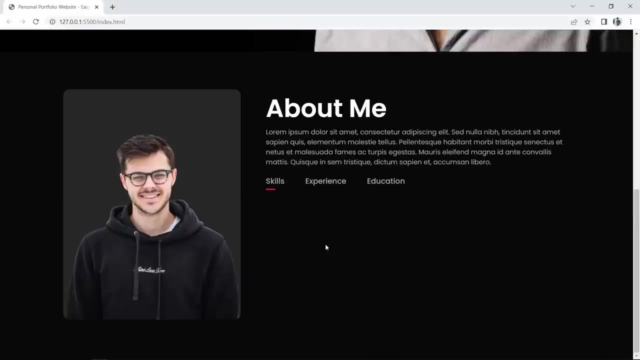 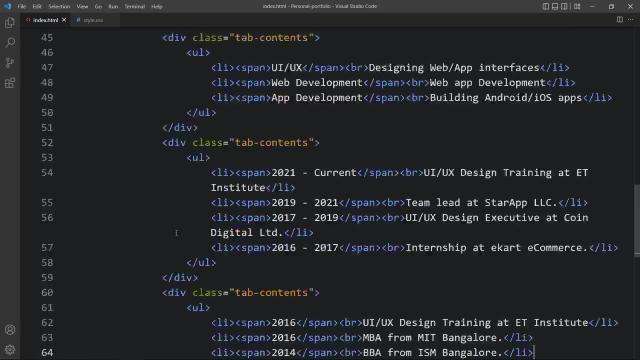 and come to this css file. here we will add this class name, tab contents. then we will add display none, so it will hide all the tab contents. you can see, all the contents are hidden. so we have to display the first one, which is for the skills. so let's come back and in this html file, in this first one, which is type contents. 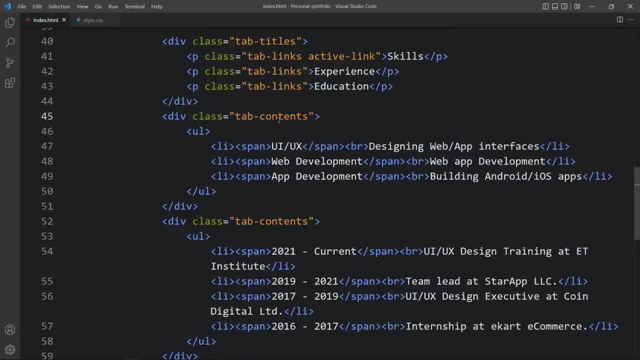 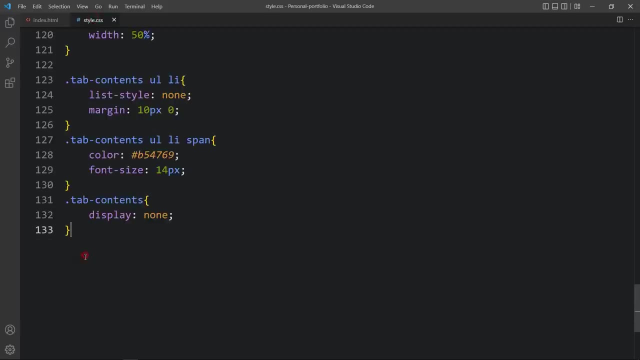 for iskils. here we will add some contents, one more class name. so after tab contents, class name, let's add one space and here we will add active tab like this. now just copy this one. come back to the css file. here we will add dot tab contents, dot- active tab. there will be no space here we have to add display. let's add the display. 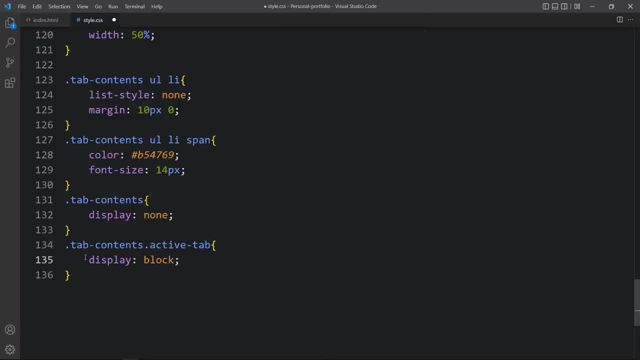 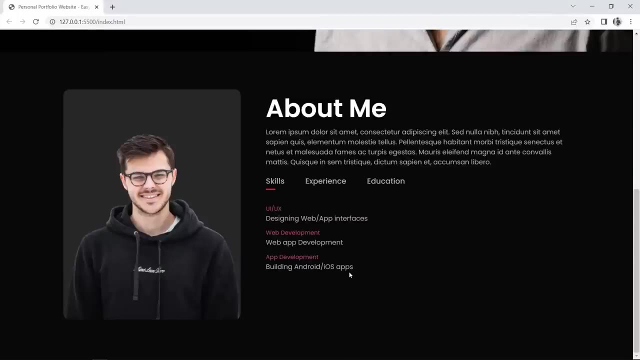 block, so it will be visible. now you can see the first one is visible here and the other, experience and education, is hidden. next we have to add the click feature. whenever we will click on experience, it should display the experience, and when we click on the education, it should display the education. 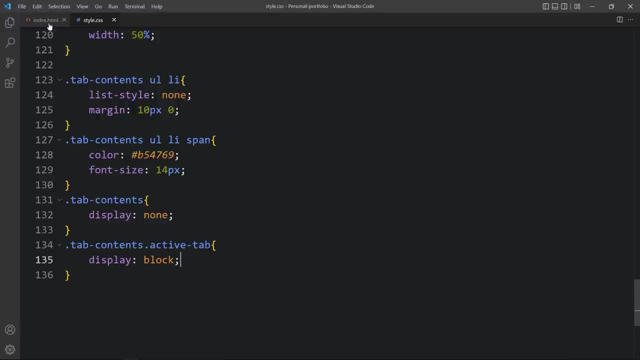 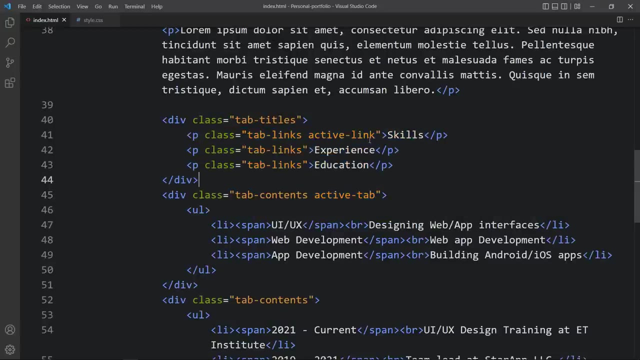 so for that let's come back and come back to the html file here here in this tab links we will add one on click events. so in the first one here we will add on click equal to write a function called open tab, and within this we will add one name. so it will be. 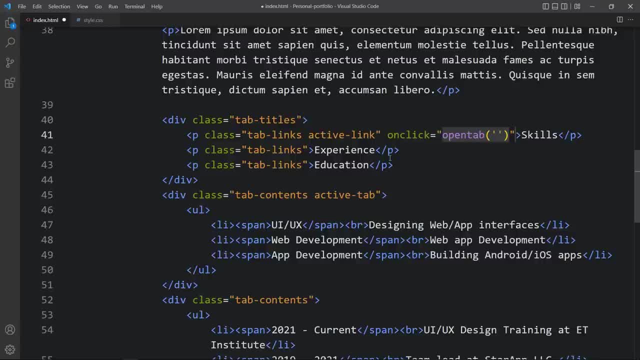 in single quote skills, just copy it and add it in the another one. add it here and here. here we will change. it will be for the experience and this one for education. so after adding this, in this content also, we will add one id. so in the first one let's add one id. 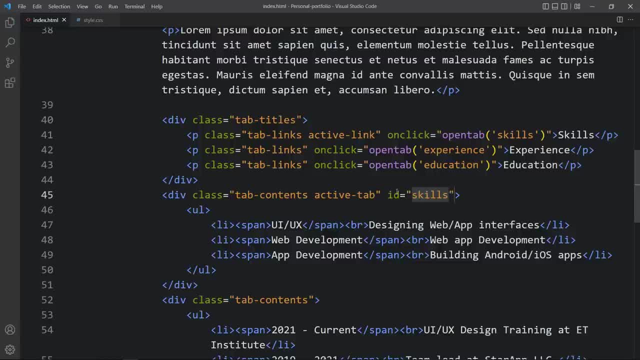 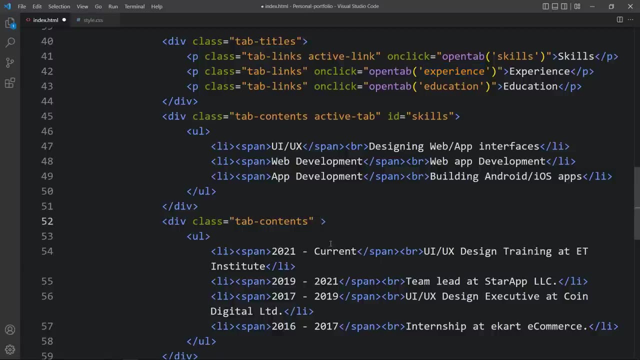 called skills. it should be same here. we have added skills. here also we are adding skills. it should be in the same upper and lower case. now copy this one experience add. add it here in the second one, id experience. and copy this education, add it here in this: 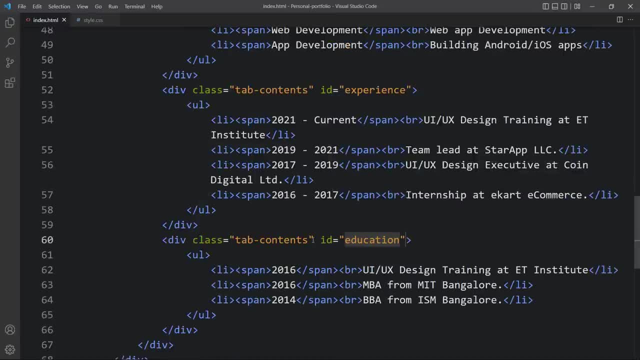 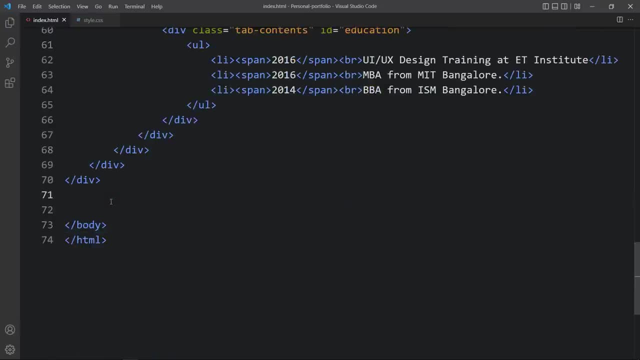 third, content id education like this: after adding this, let's come back to the bottom. just above this closing body tag, we will add a script tag, script open and closing tag. in this one we can add the javascript. so here we will add one variable where write tab links equal to. 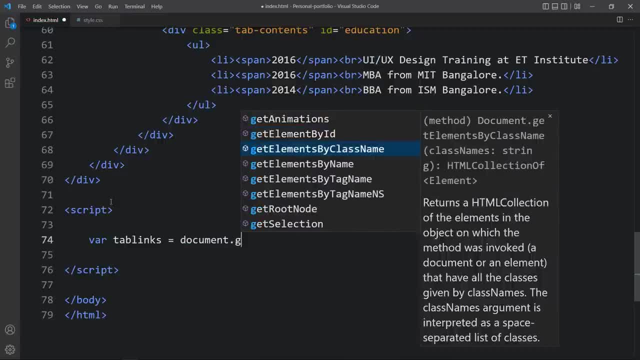 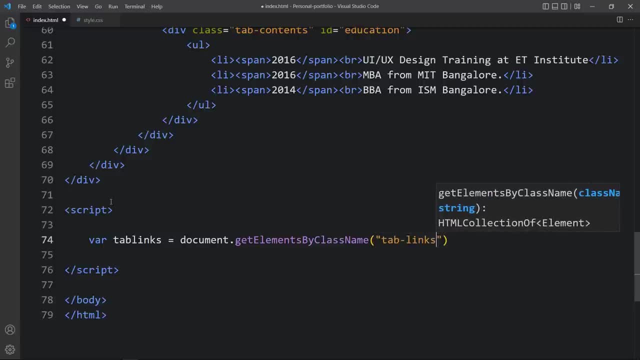 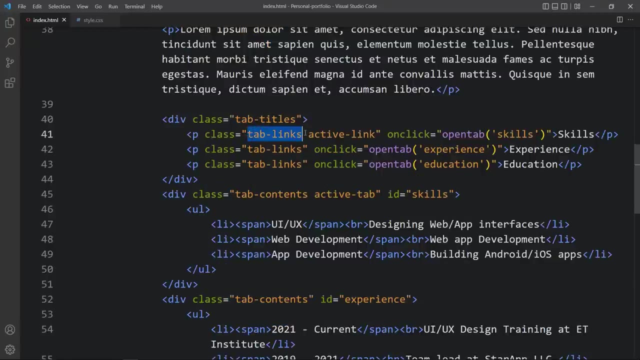 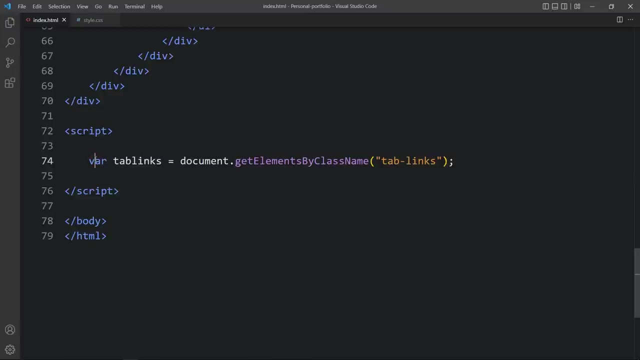 document dot. get elements by class name, and in this class name we will add tab links, because we have added the class name here, tab links. now we have the class name called tab contents. so here also we will add another line, duplicate this one and write tab contents like this one, and in this one we will add tab. 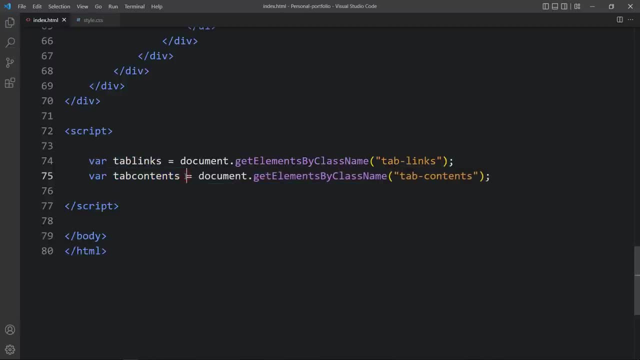 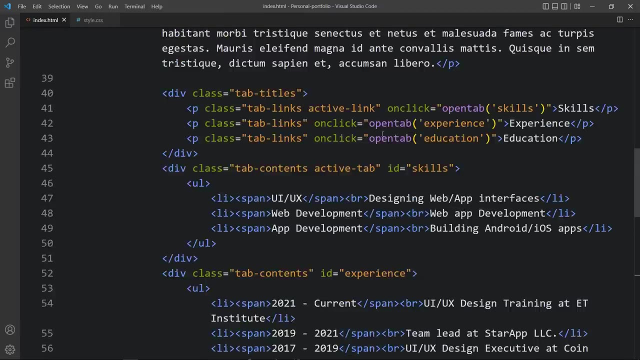 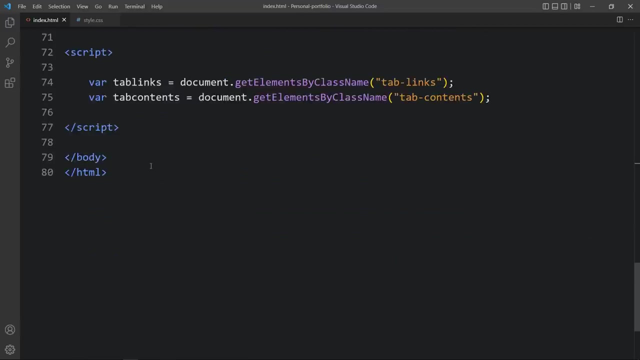 contents like this. now let's come to the tab, and here you can see we have added on click and this function open tabs. so let's define this function open tab. come back here, write function open tab. in this open tab it will receive one argument. so here we will add any name. let's add. 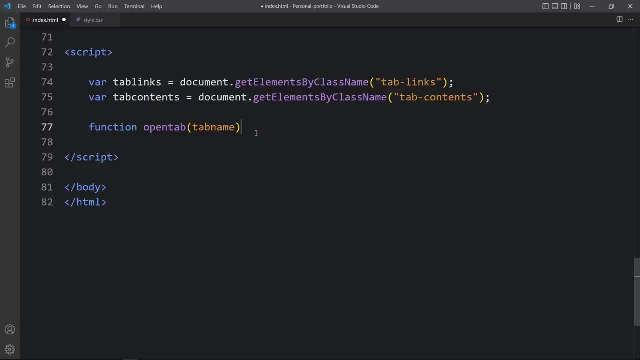 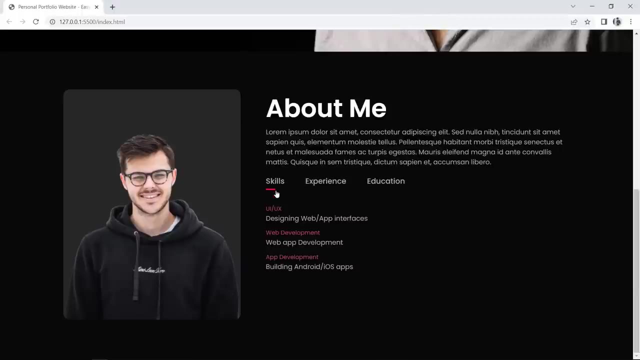 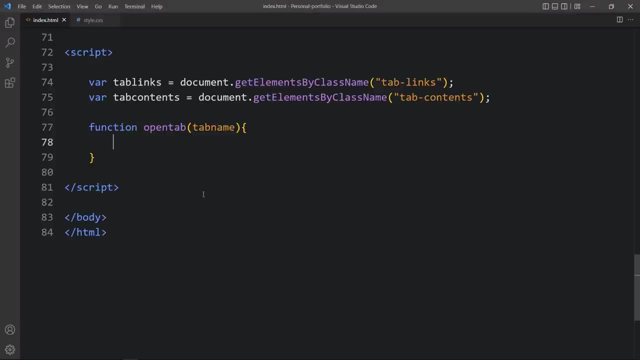 tab name like this. so whenever we will click on any tab link, suppose if i click on skills it should hide this one and it should also hide this underline for that. let's come back and write this for loop for tab links: write tab link, only tab link of tab links. 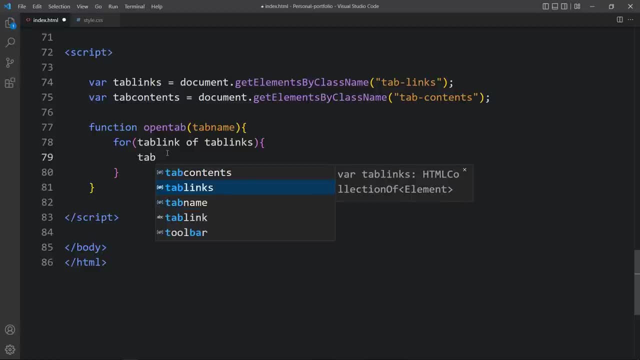 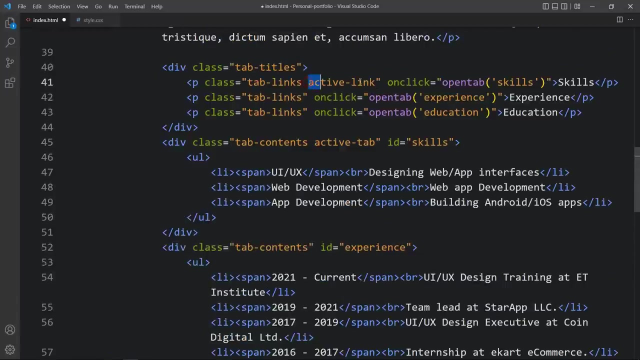 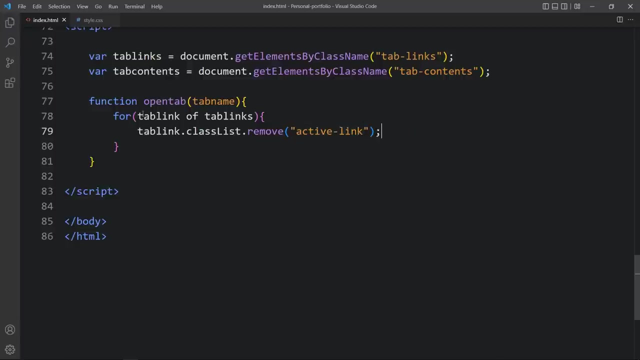 then tab link: dot. class list dot. remove what it will remove? it will remove the active class name. you can see we have added the active link in the first one, so let's copy this one. paste it here. it will remove this class name for all the tab links. now again, duplicate this one. 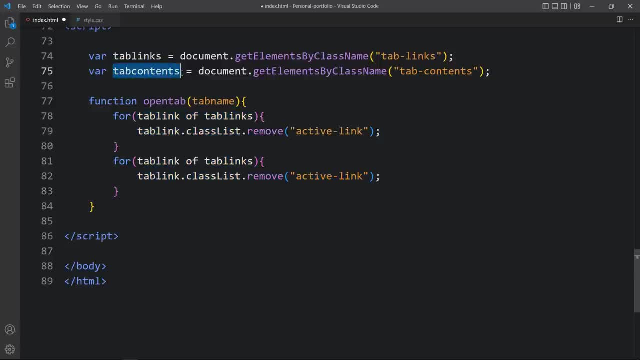 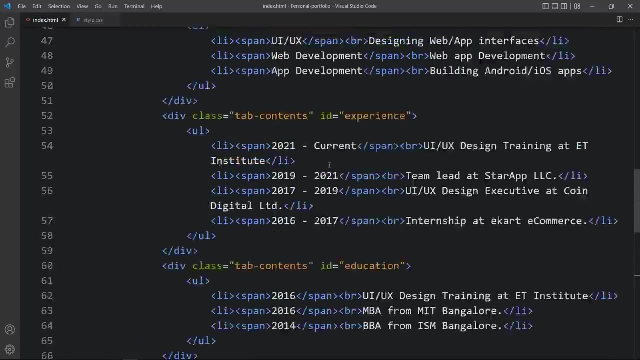 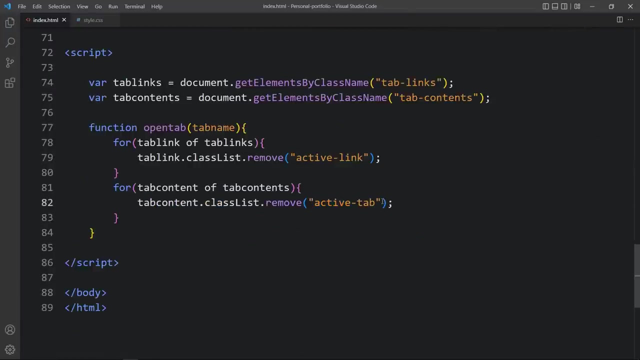 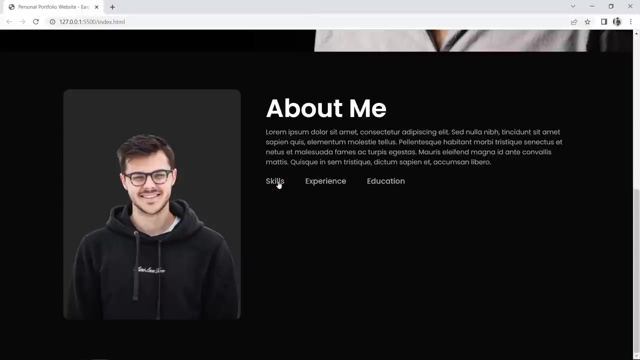 here we will add this tab contents: tab contents: remove s tab content only and here also tab content and this one another class name: active tab, like this. so, after adding this, let's come back to the website and you can see if i click on this skills: it is removing the description, which is the content, and it is also removing this underline. 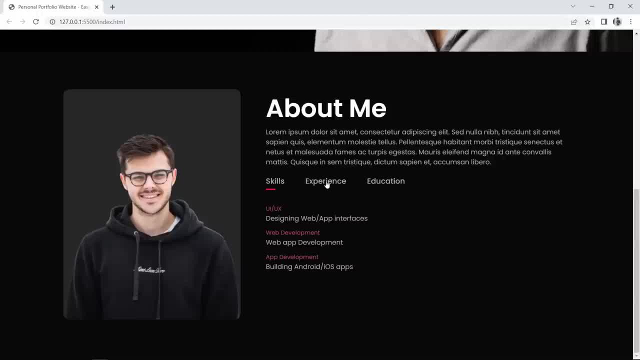 let me refresh the website and if i click on another one, it is doing the same thing. let's click on the third one. it is hiding all the content and underline. next, we have to display the title of education. if i click on education, education- and if i click on experience, it should display the experience content. so let's come back. 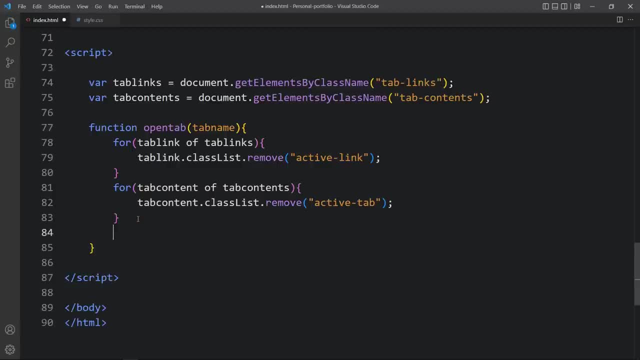 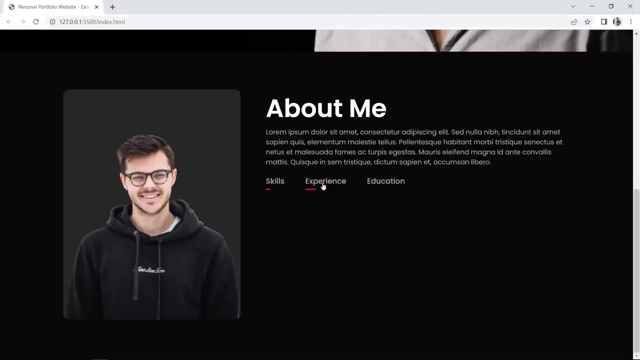 here we will add event dot, current target dot, classlist dot add and it will add this one active link. so it will add the active link and it will display the color. so let's check this one. if i click here, you can see the active color here. if i click here, it is displaying the active color. 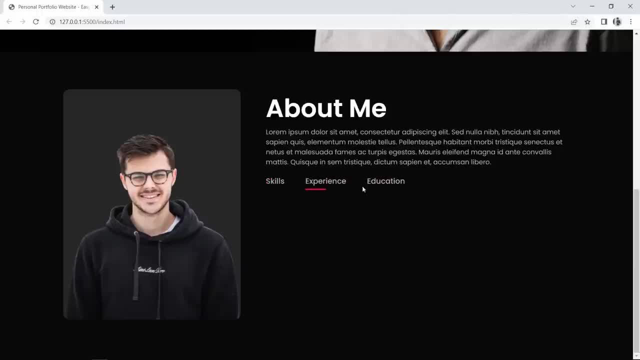 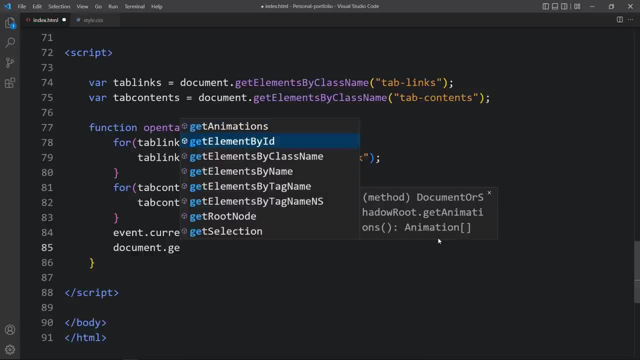 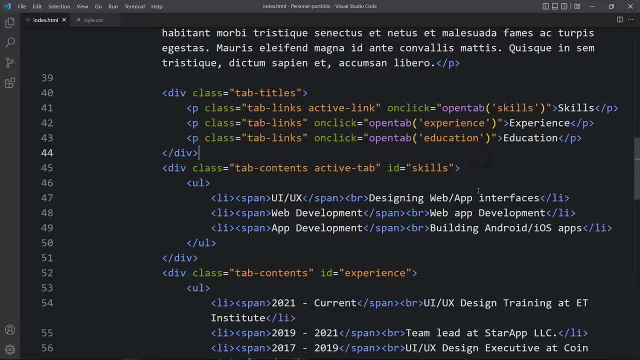 here. so this color is working. next we have to display the content. so let's come back here. we will add document dot, get element by id and in this id we will add this tab name. so if we will click on this education, it will send this education here in this tab name and it. 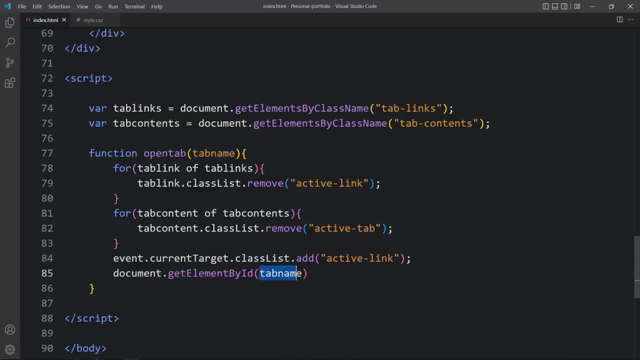 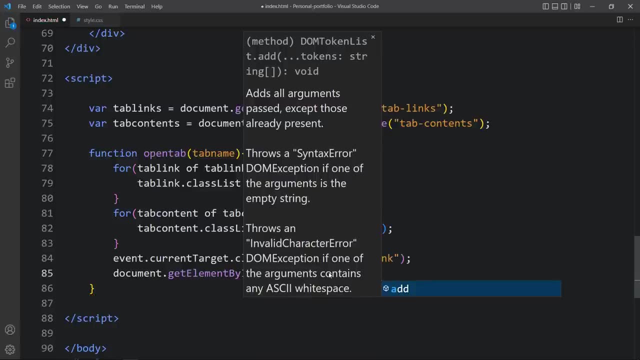 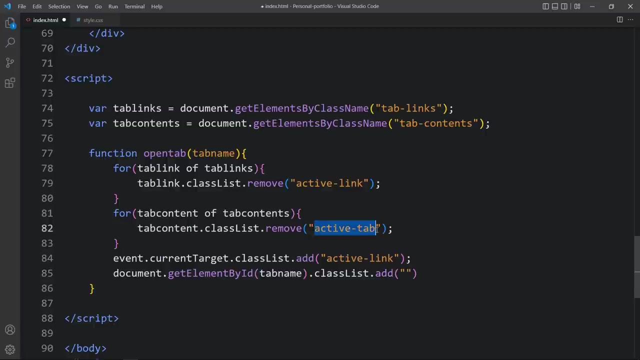 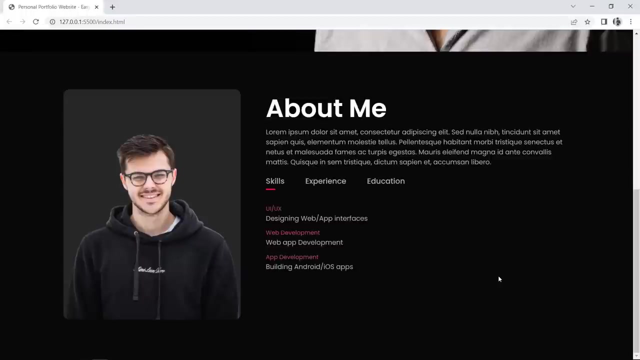 will search by document dot. get element by education dot. classlist dot. add. and what it will add: it will add that active tab. that's it now again. refresh the website. you can see, if i click on experience, it is displaying the experience here and if i click on education, it is displaying the education content here. 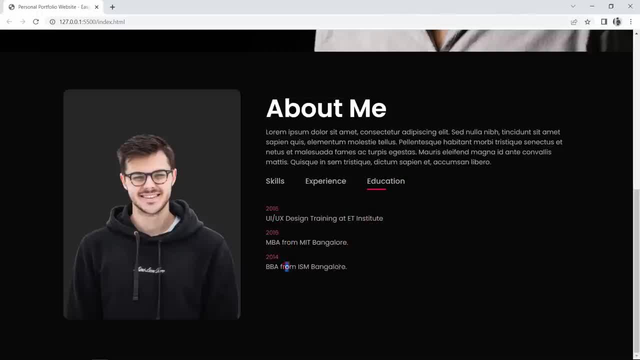 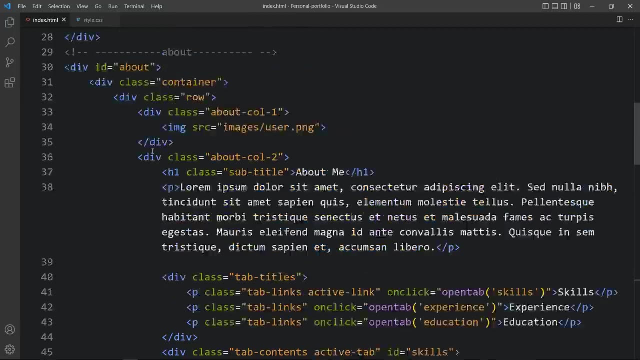 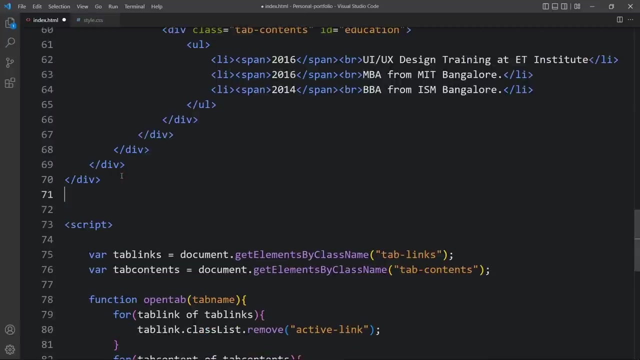 now we have completed the about section of our personal portfolio website. next we will design the services section. so let's come back to the html file. so we have completed the about section of our personal portfolio website. next we will design the services section. this about div is closing here, so after this div let's add one comment. 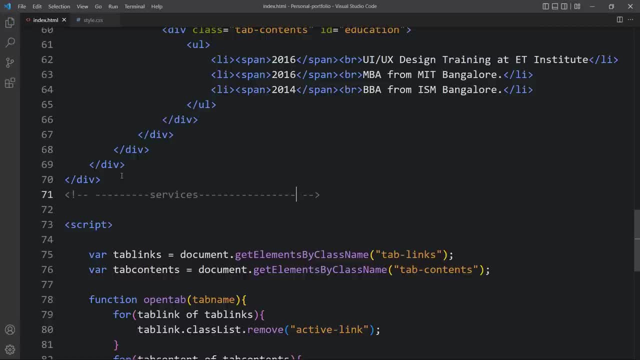 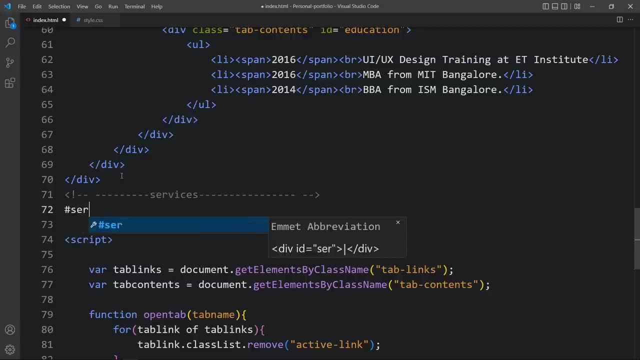 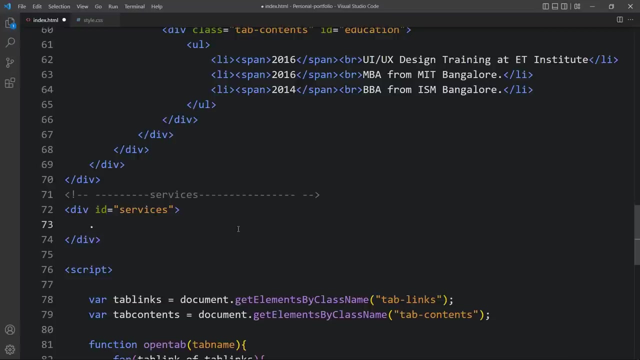 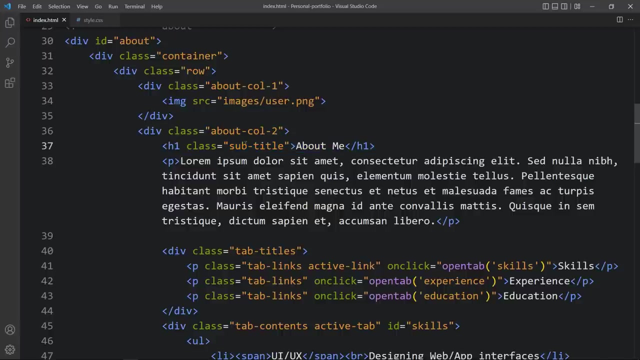 services. then we will create a div with the id services. in this one again we will add one div with the class name container and here we need one title. so let's come back here. in this about section, here i have added one title with the class name subtitle. so let's copy this one and 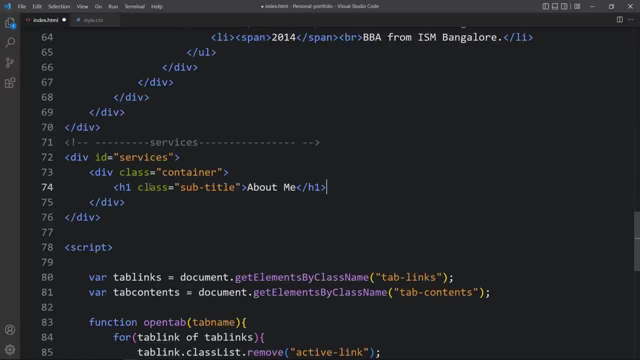 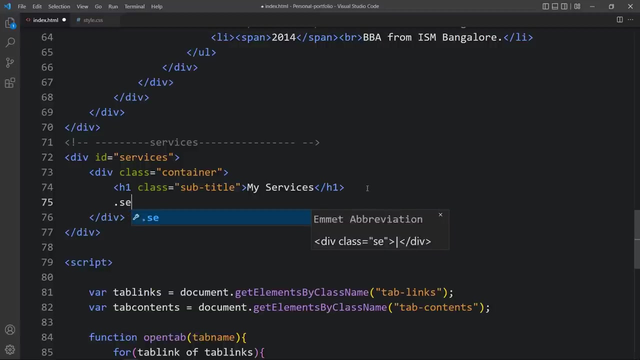 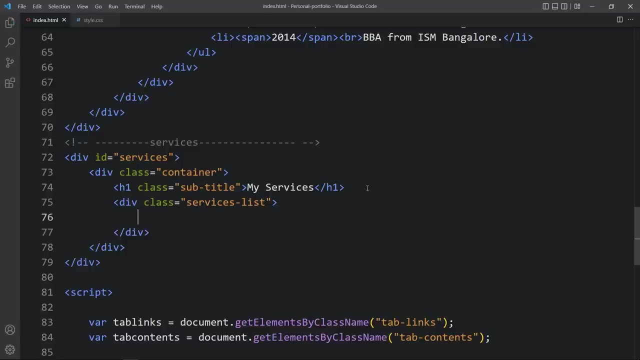 add it here in this services, and we will change the text here so it will be my services. after this title we will add list of services in three columns. so here we will add a div with the class name, services list, and in this one we will add multiple services. 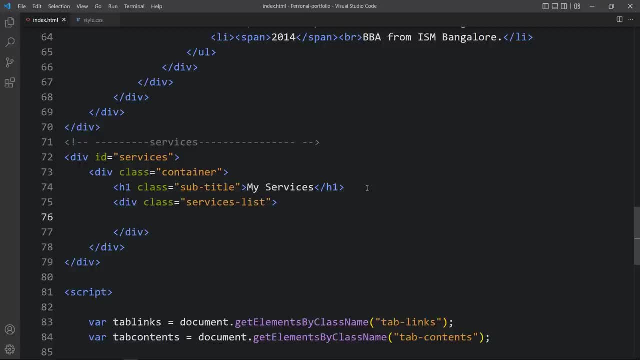 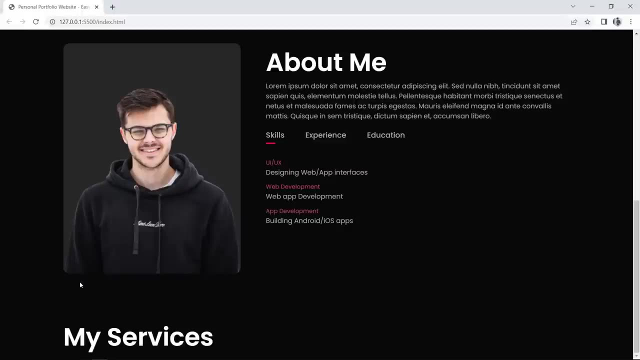 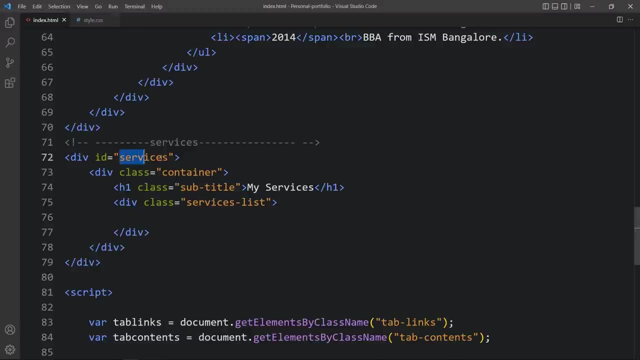 so first we will add some css for the class name and id that we have created right now. so let's come back to the web page right now and here you can see this text at the bottom. so now we will come back and here we have this services id. so let's copy this one and come back to the css file first. 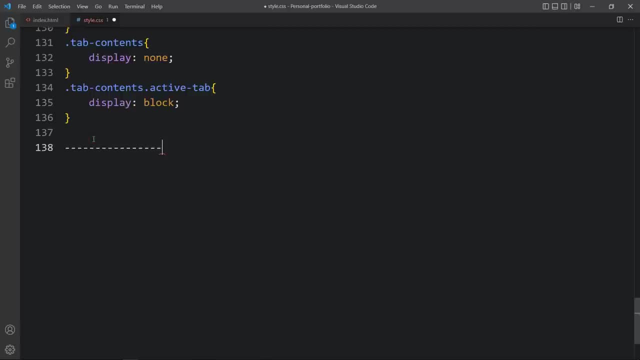 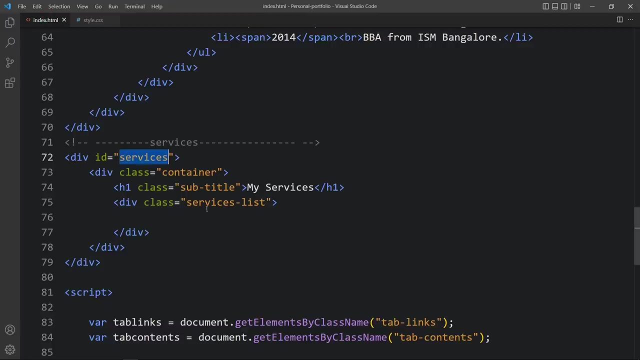 we will add one comment here and let's add this id with the hashtag services. so for this one we will add some padding. it will be 30 pixel and 0: 30 pixel from top and bottom and left right, 0. after that, we have added this services list, so let's copy this one and write it here in the css file with: 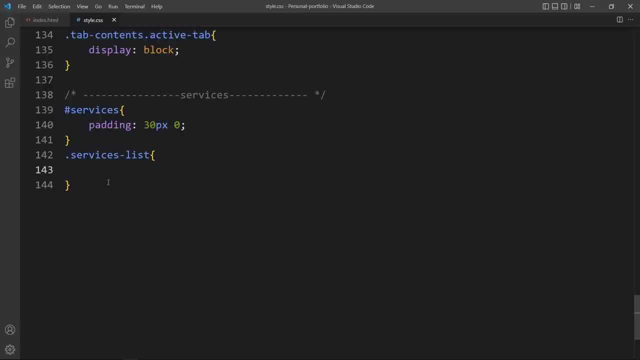 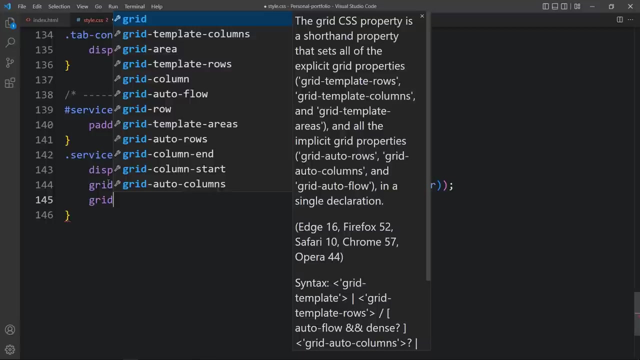 a dot because it is a class name. so here we will add display grid and grid template columns. it will be repeat auto fit comma min max 250 pixel comma one fraction fr. then we will add the grid gap. i have dedicated video about grid. you can find that link in the description. 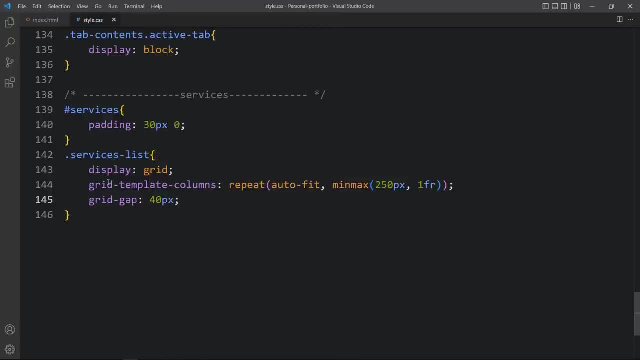 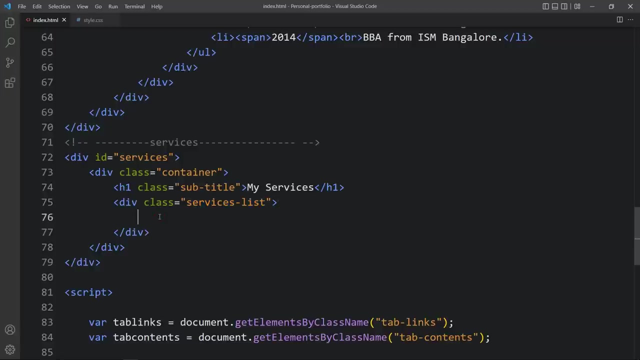 grid gap will be 40 pixel and summer space from the top. so let's add margin top 50 pixel. so we have added grid layout in this one. now we will add any div inside this services list that will be displaying as a grid. so we will add any div inside this services list that will be displaying. 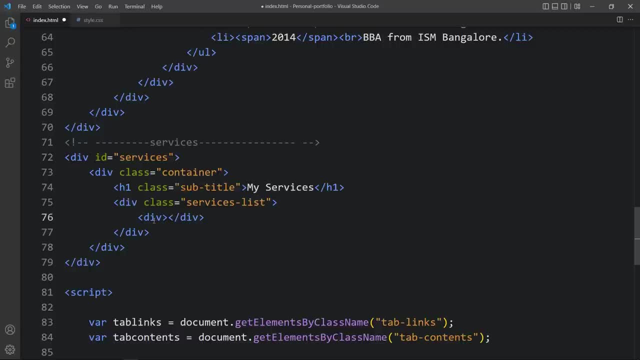 as a grid. so here we will add one div. there is no class, name or id. simply we are adding div open and closing tag and in this one we will add the services title and description. so let's add one service title, then we will add one description in p tag. 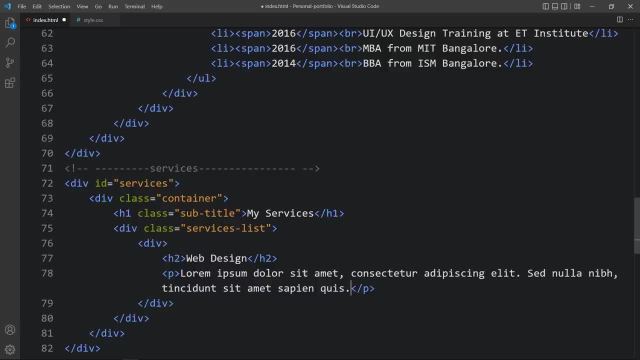 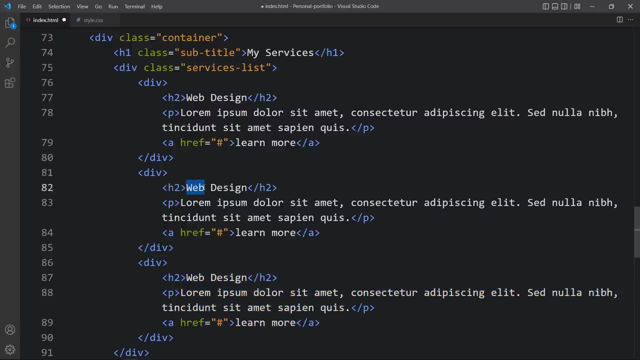 so this is the description for the first service, and after that there will be one link for learn more. so let's add one, a tag, and the link text will be learn more. let's duplicate this one and here we will change the title. now change the title in the third one. 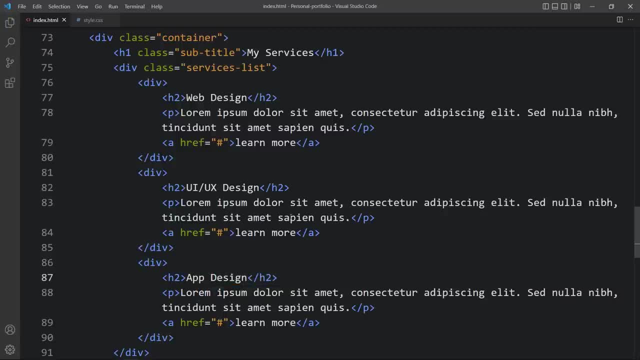 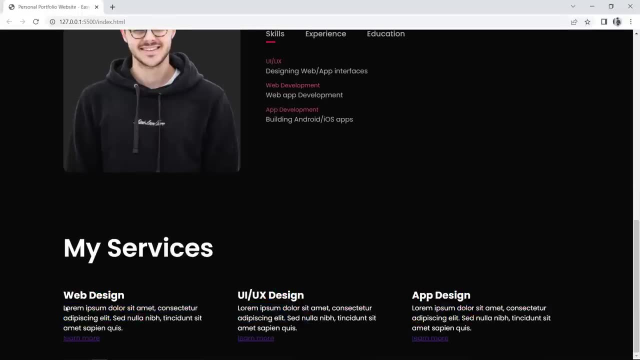 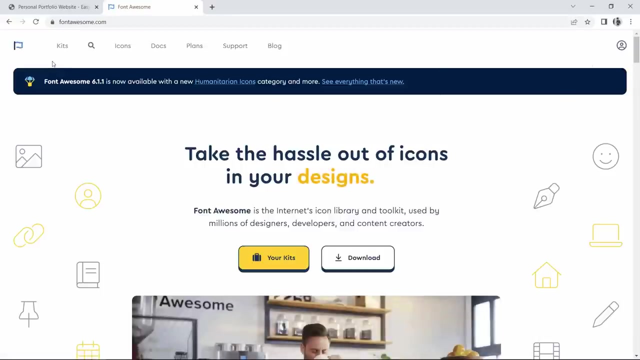 and we will add one description from this new design. after that, let's refresh the web page, and here you can see these services in three columns. next we have to add one icon also. to add any icon, we will come to the website called fontawesomecom. on this website, you have to create an account. it will be for free. 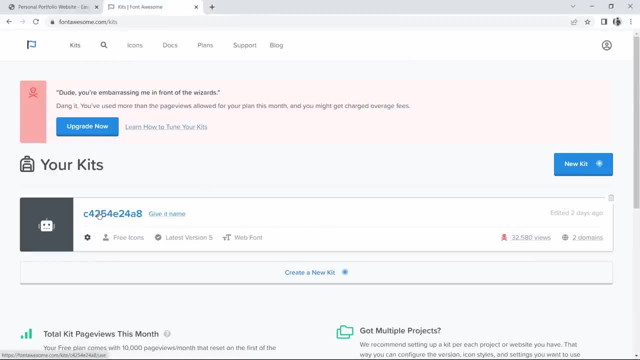 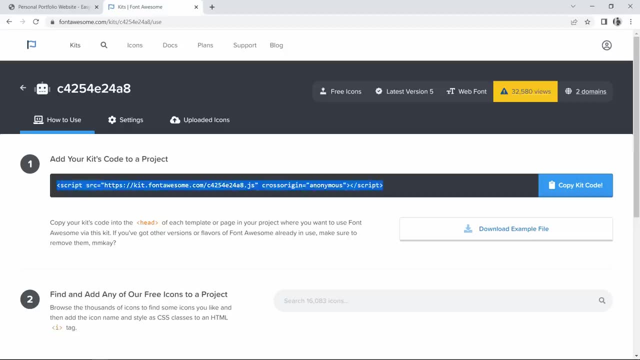 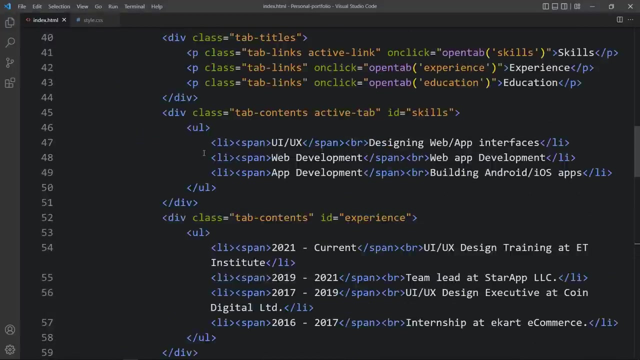 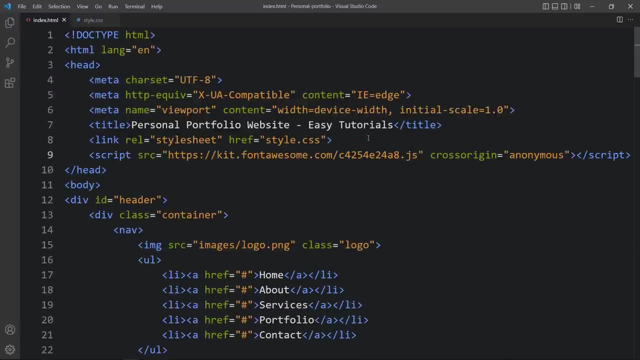 and click here, then you will get this type of script. it will be for one line script that you have to add in your html file. let me come back to the html file and add it just before this closing head tag. so i have added this font awesome kit script here you just add. 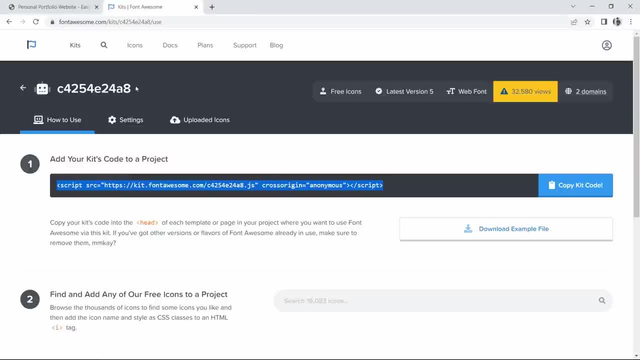 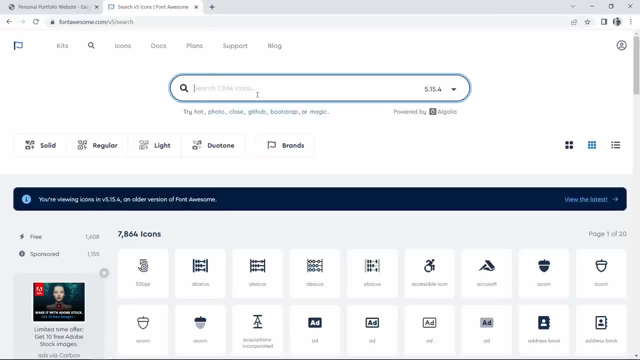 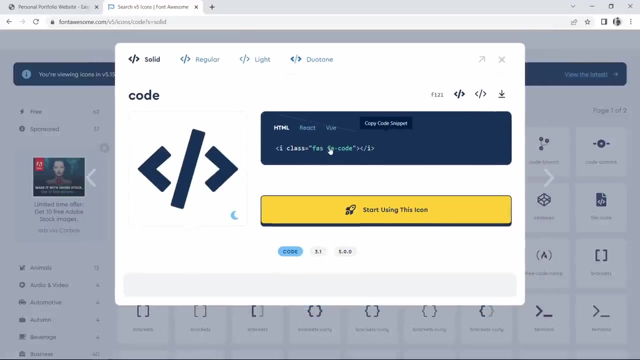 your own script. so let's come back and again. come to this website and click on icons here. in this search box, you can search for any icon that you want to use on your website. so let me search for code. let's click here. click on this code. it will be copied. so let's. 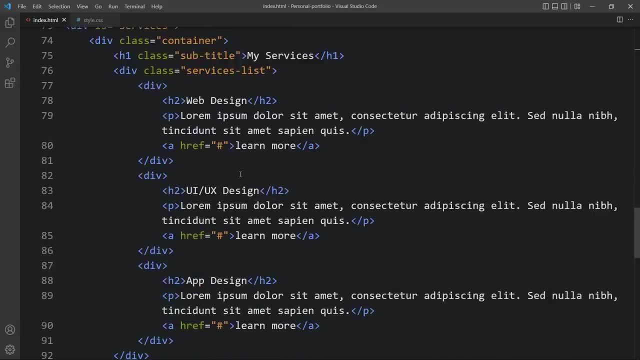 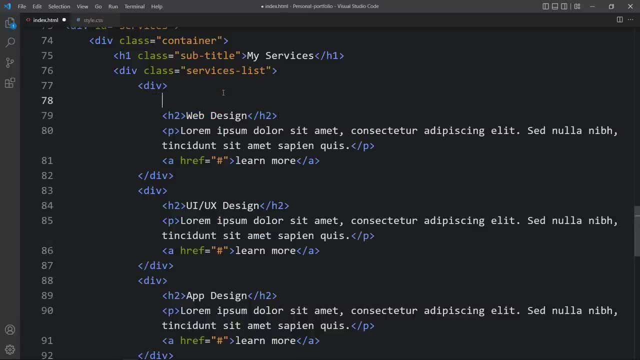 come back and add it here, where you want to display the icon. so we will display this icon in this first service, just above this title. so here let's add a space and add this one line of html code. so we have added one icon. let's come back and we will search for another. 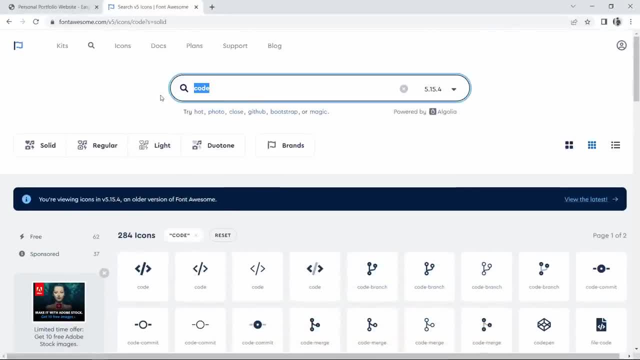 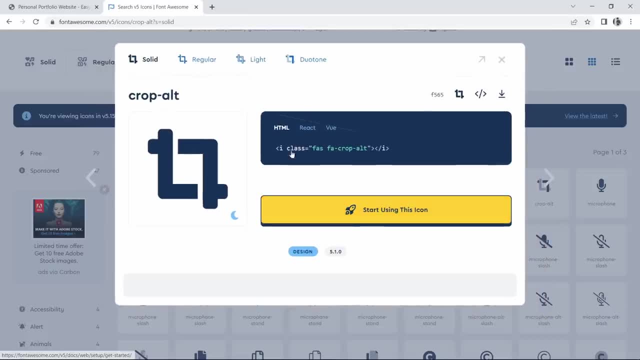 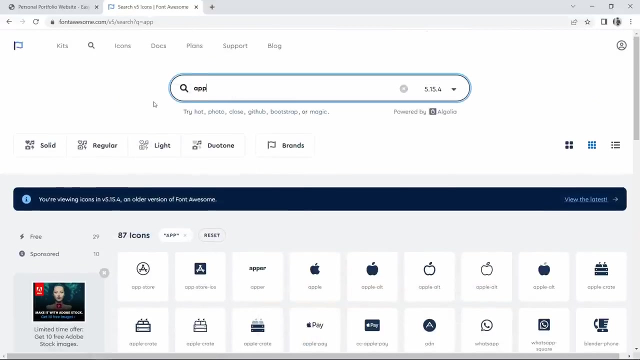 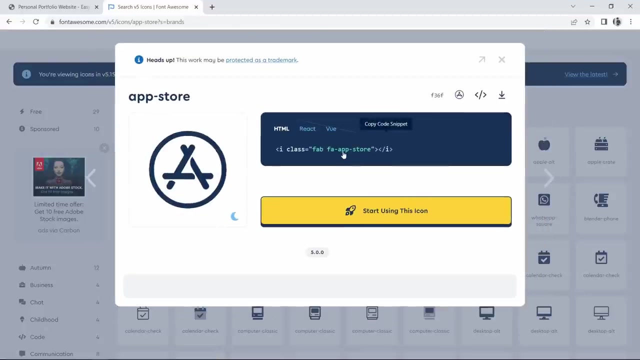 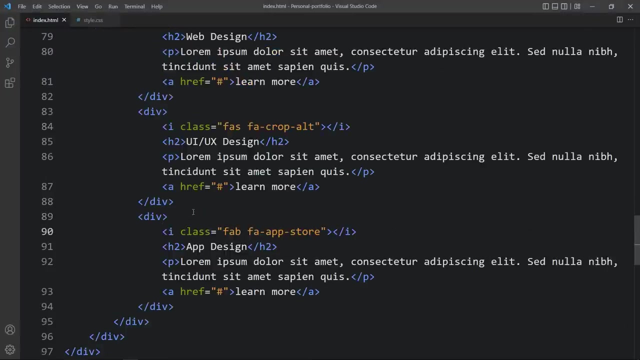 icon. so here we will search for another icon called crop. let me use this one. click here. now we will search for another icon. here we will search for app. let's click this one, copy this one and paste it here in this third service. after adding all the three icons, let's come back to the website again. 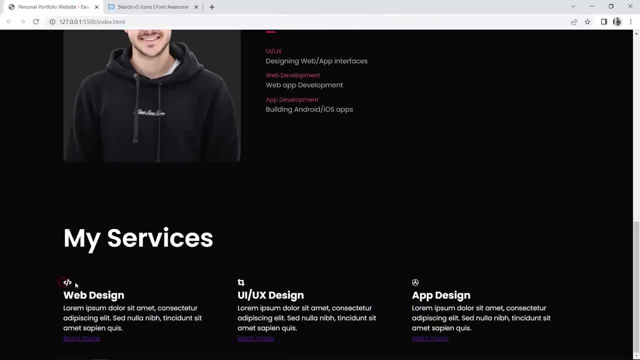 here you can see that lower left column is there. you can see official icon object c: l special name back desire is here and here. here you can choose again and click here. you can add this11M Continuing такой- these icons just above the service title. next we have to add some css to design this layout. 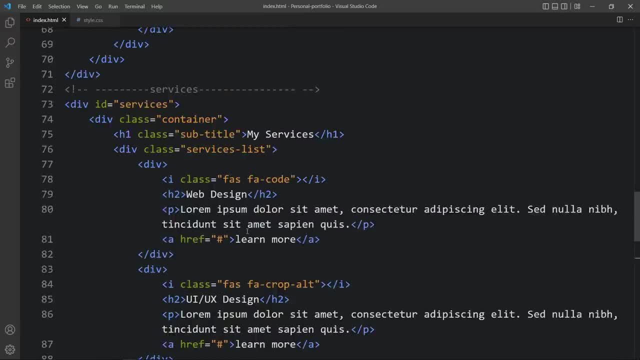 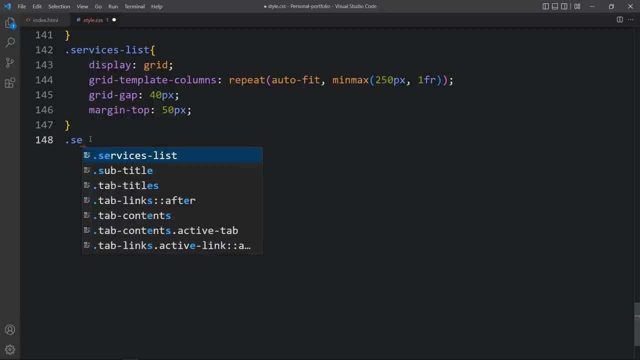 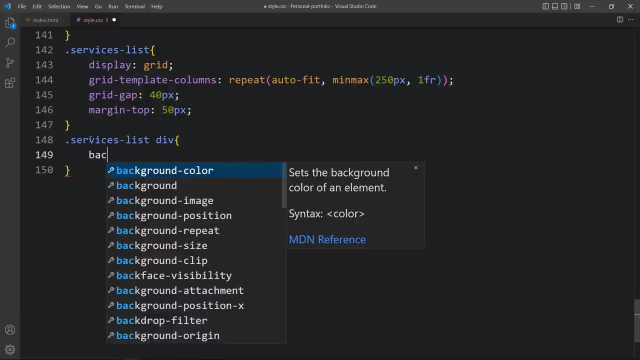 so we will come back to the html file and you can see we have added services list and in this one we have the div. so come back to the css file again. write this class name, services list and div. so for all the individual services we will add the background. write this color code. 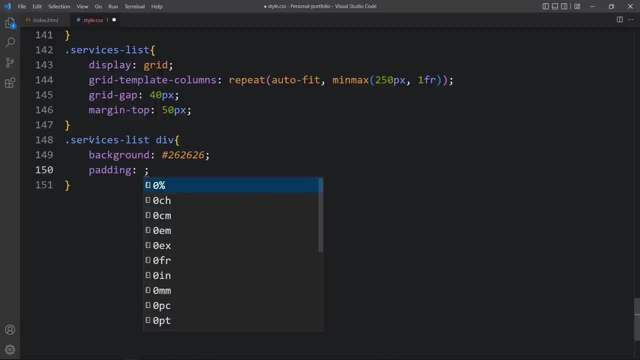 then we will add some space inside this box, so we will add padding of 40 pixel. then let's change the font size and font weight. now we will add the border radius so that the corners will be round. you can see, we have this gray color of box for all the services. 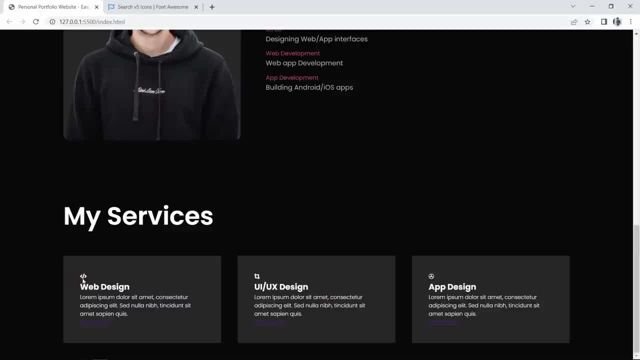 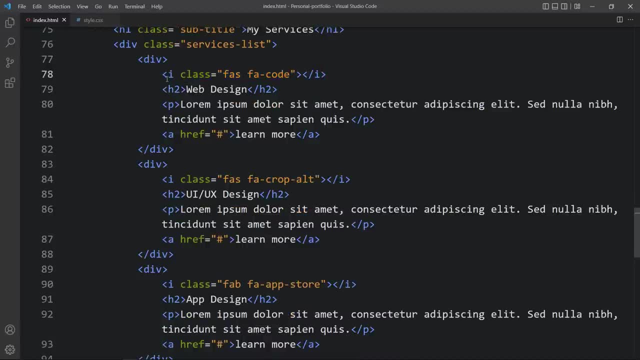 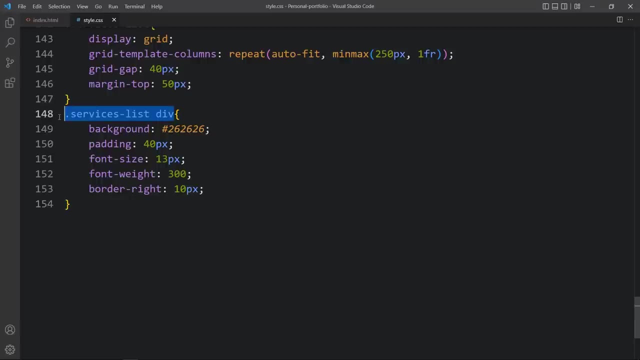 next we have to change the size for this icon. so let's come back. and here you can see we have these icons with the tag i. so let's come back to the css file. here we will add the same thing- services list, div- and then write i for the icon. in this one we have to increase the font size. it. 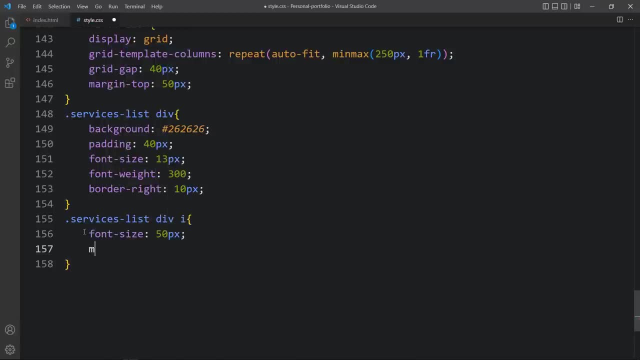 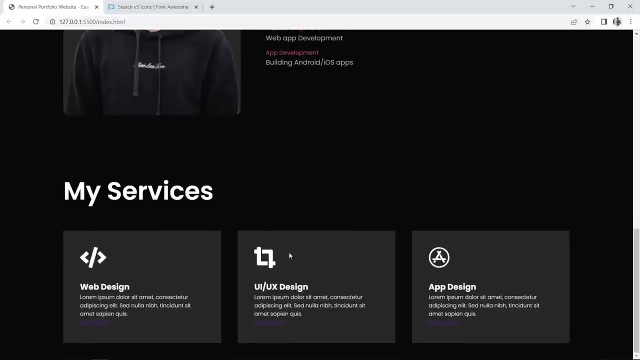 will be 50 pixel, then summer space at the bottom so you can see the increased size for the icon. next, we will add the css for the title, we will increase the font size for this title and we will also decorate these links, which is learned from this tutorial. 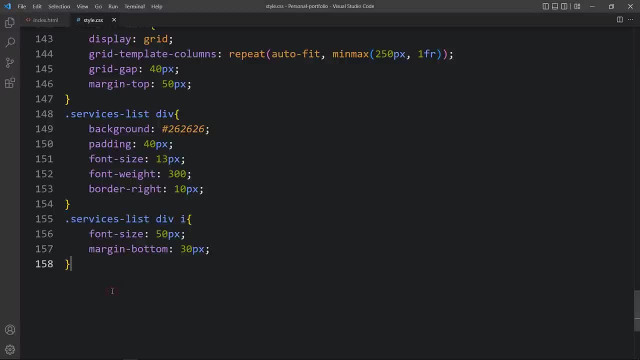 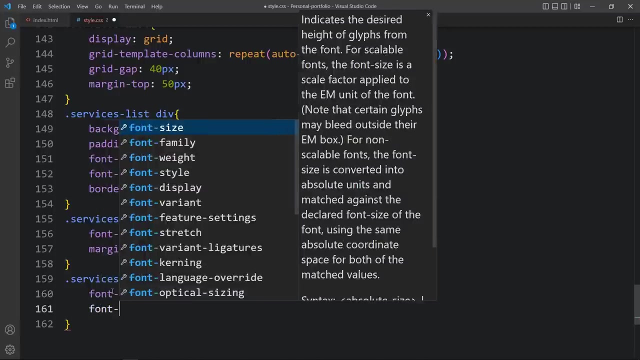 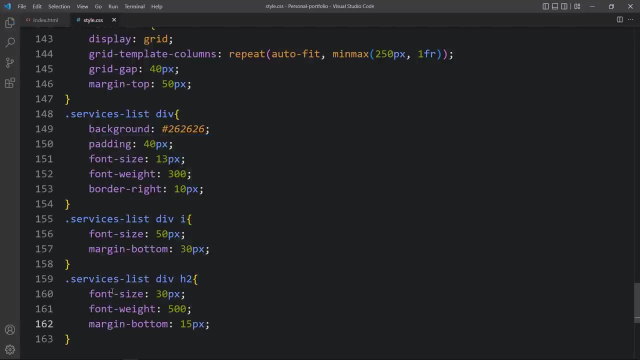 so let's come back again. copy this one, then write h2, because we have added the services title in h2 tag. so font size will be 30 pixel, then font weight- it will be 500, and margin at the bottom. after that we will decorate the link. so again write this. 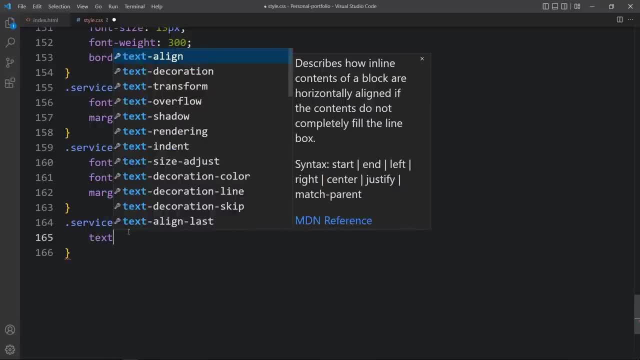 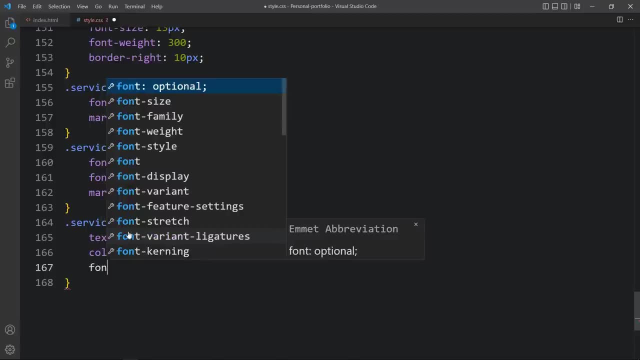 then write a and for this link we will add text decoration: none color will be white color. then font size: it will be 12 pixel, very small, and margin from the top display will be inline block. after adding this again, refresh the website. you can see we have. 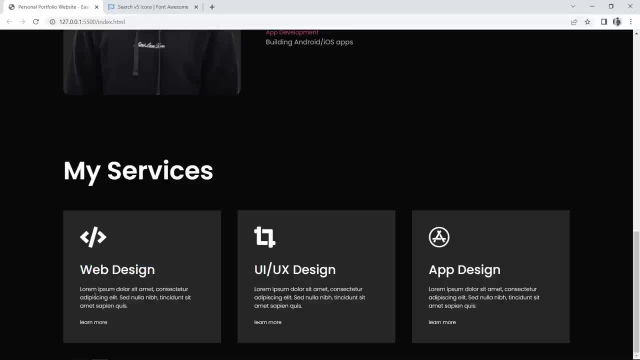 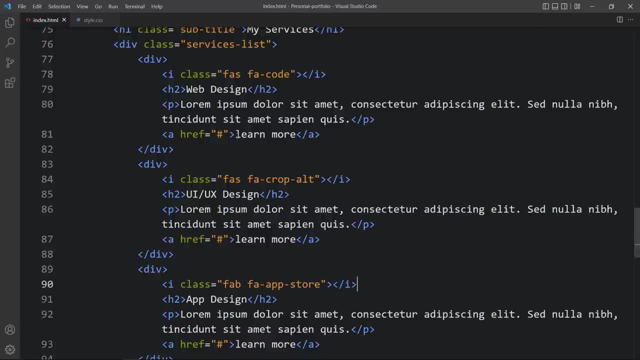 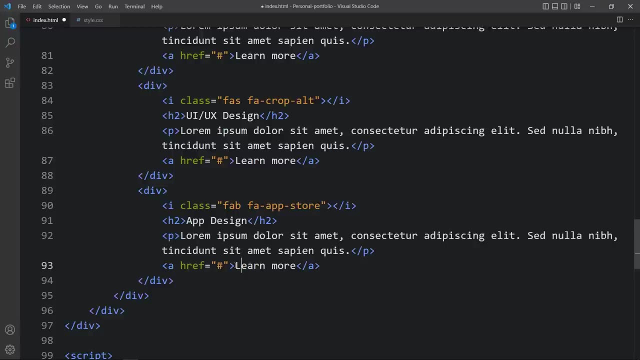 some space around this title and the font size for this title is looking good and this learn more text is also looking good. let's come back. come to the html file. we will make it capital l, so it will look good. so, after adding this, we will add the hover effect on. 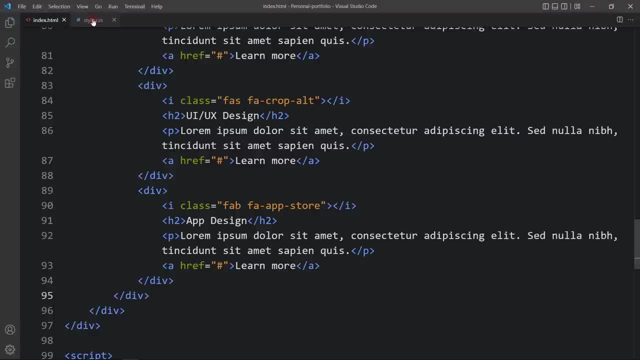 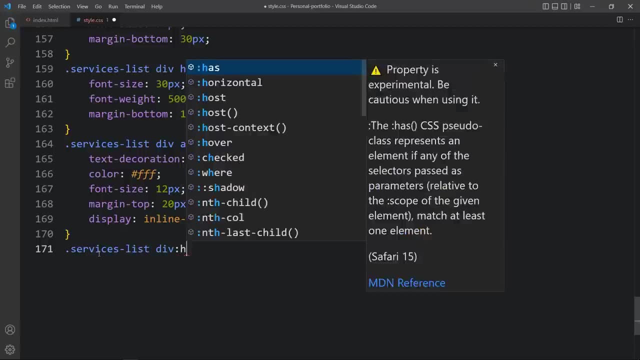 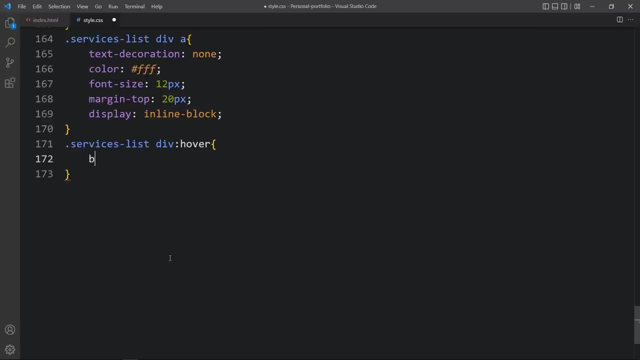 these services list. so let's come back and come to the css file here. just copy this one and paste it here. then write colon hopper. so whenever we will take cursor over any services, it should change the background color. so we will add background and another color code. 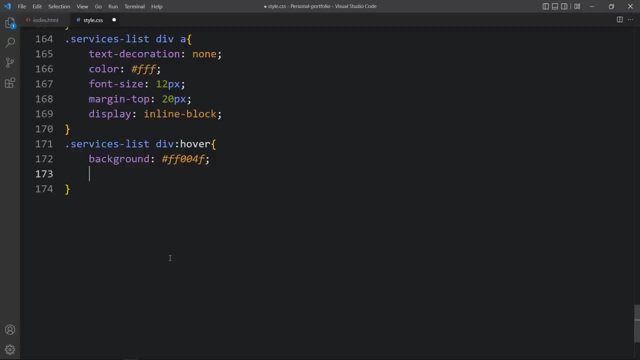 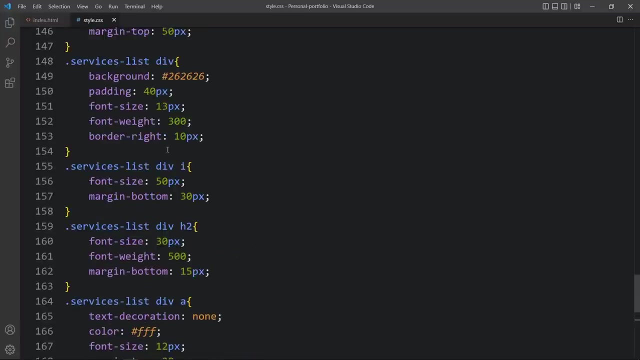 after that we have to move this services a little bit up. so let's add transform translate y minus 10 pixel, so it will move the box by 10 pixel. so in this one we have to to add some transition. so here we will add transition background. it will be 0.5 seconds. 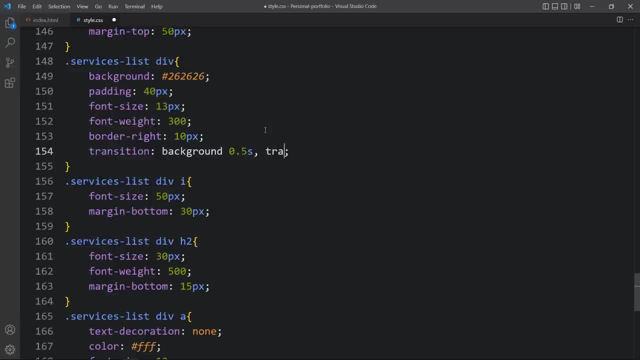 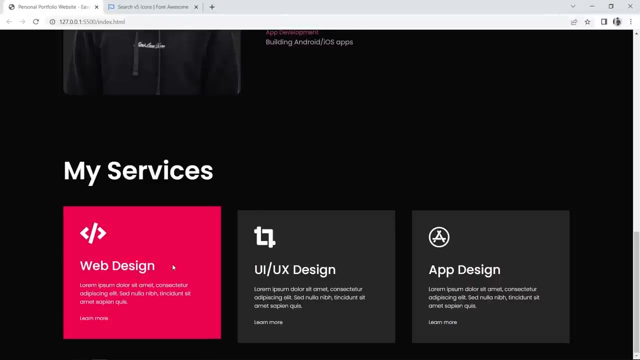 comma transform 0.5 seconds. after adding this, again refresh the website. and here you can see, if i take cursor, it is moving up and the color of the background is also changing. this border radius is not working. let's see here we have added border. right, it will be border. 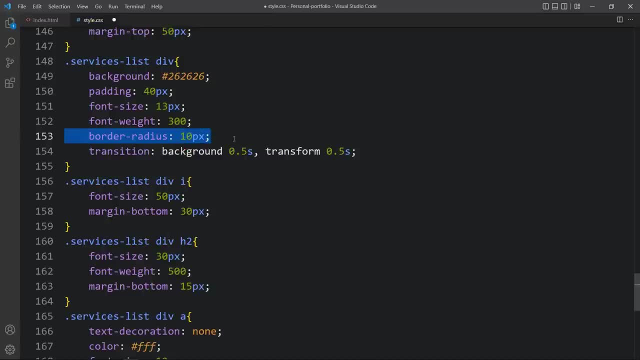 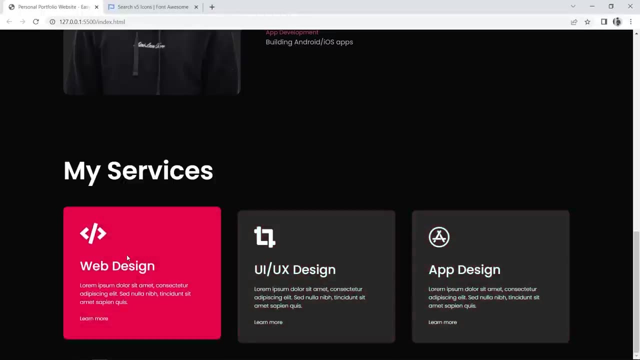 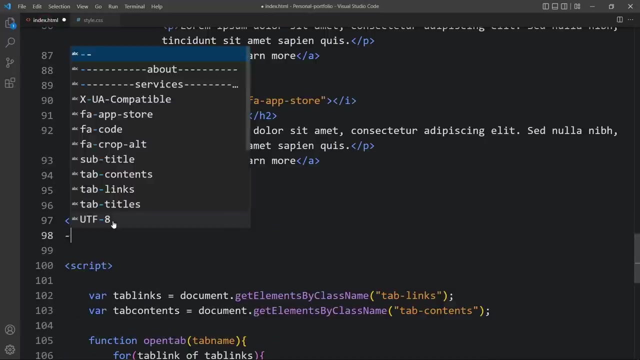 radius: 10 pixel. now you can see the corners are round. so we have added 3 services. after adding this services, we will add another section called portfolio or my work. so let's come back to the html file and here, after this div, we will add one comment. 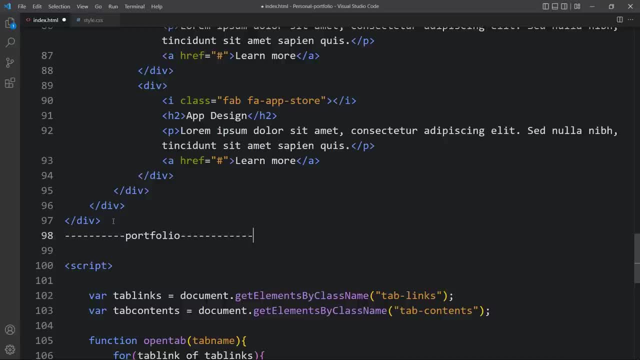 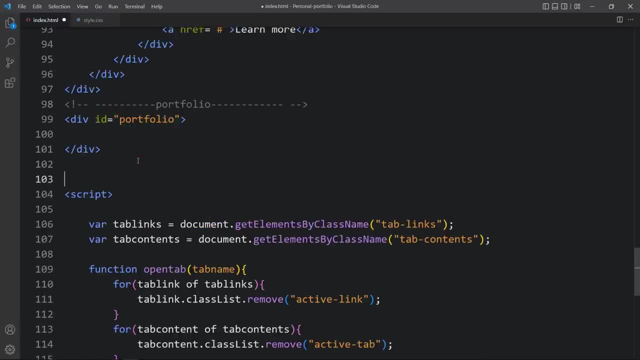 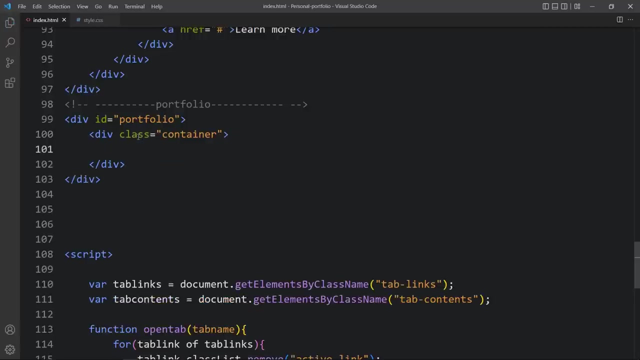 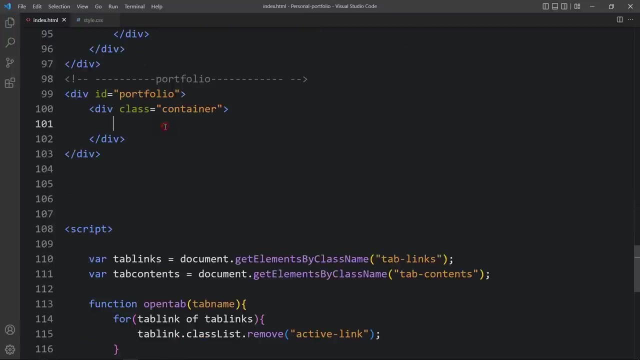 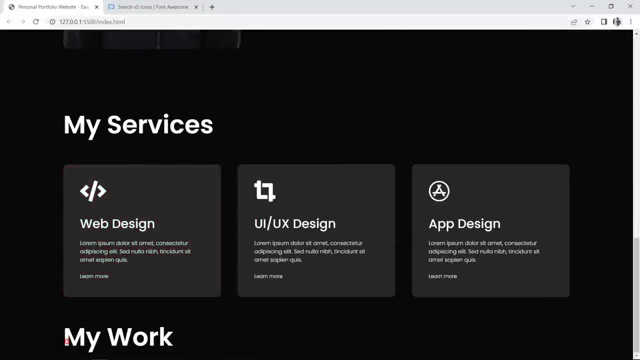 portfolio. then we will add one div with the id portfolio. in this one, again we will add one container and again we will add one subtitle. so let's copy the subtitle from here and paste it here. here we will change the text. it will be my work. let's refresh the website. here you can see this title called my work. next we need some. 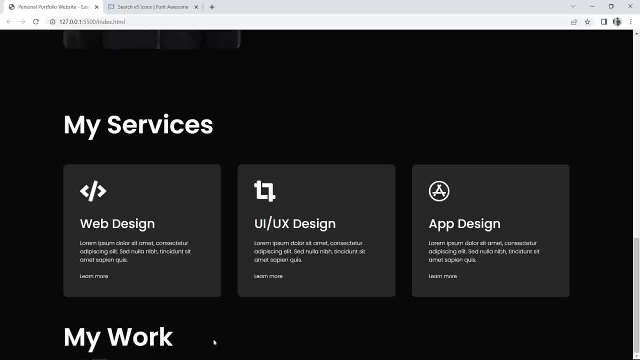 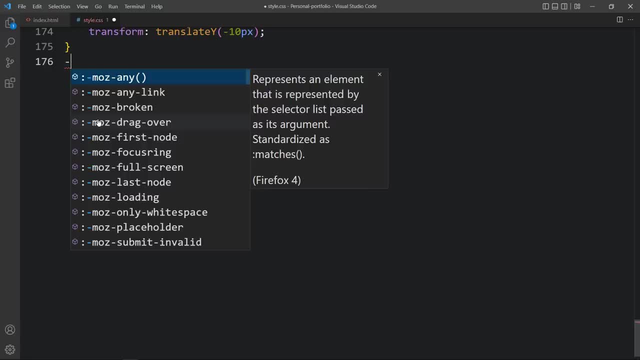 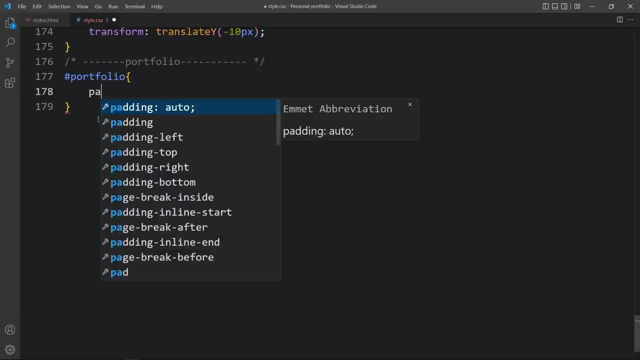 space around this. so let me come back and copy this id portfolio, write it here in this css file. first we will add one comment, then write this id with the hashtag and here we will add some space. so we will add padding, 50 pixel and zero. 50 pixel from top and bottom and zero. 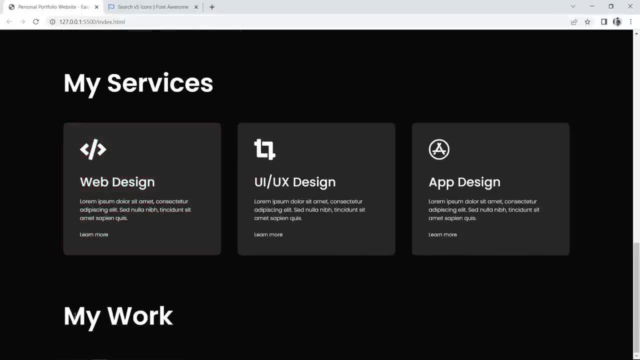 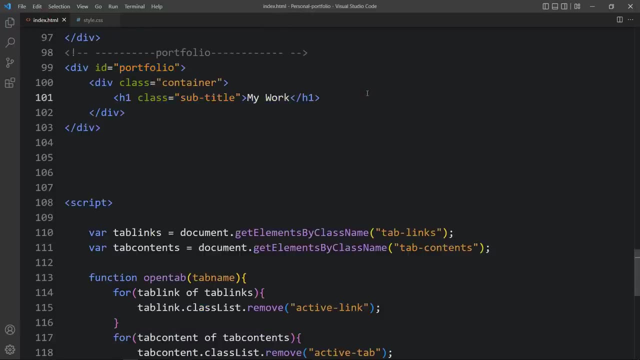 from left and right side, so you can see we have even more space around this text, which is my work. now again, we need grid layout where we will display the list of work. so let's come back and come to the html file. after the subtitle, we will add one div with the 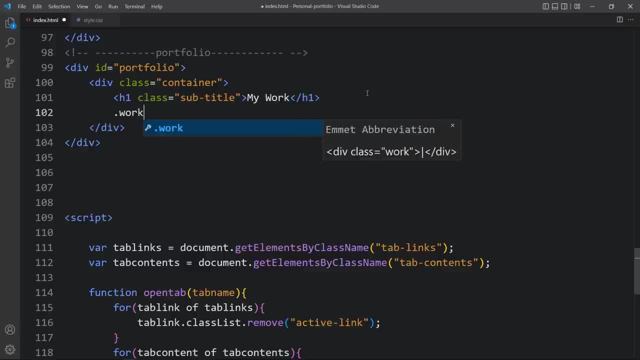 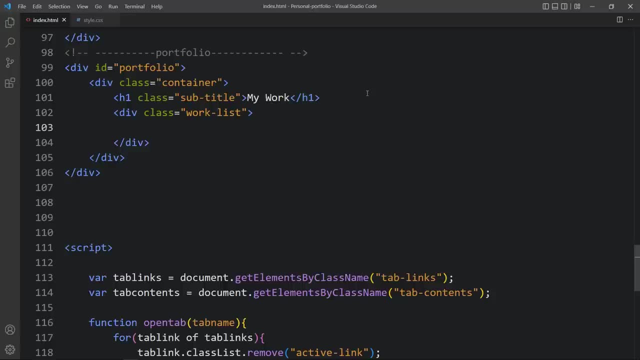 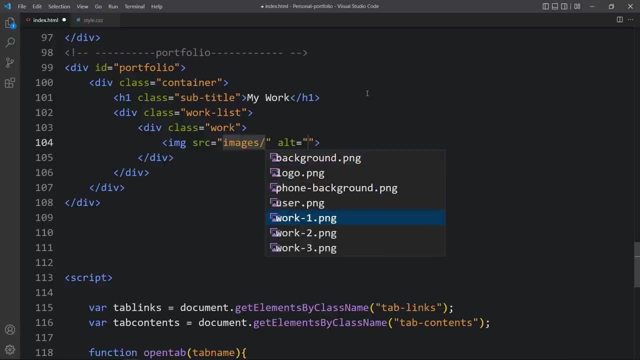 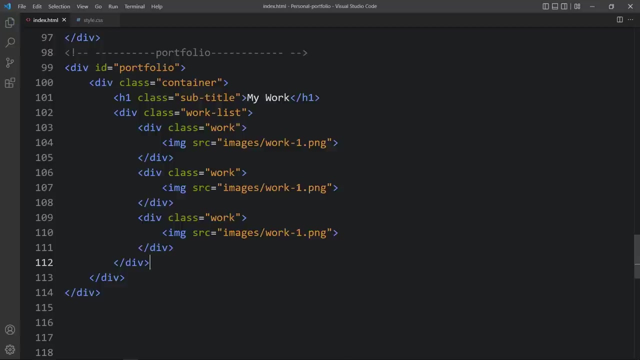 class name: worklist. in this one we will add the first work. so here we will add another div with the class name work. so first we will add one image. write the file path of the images. it is images slash- work one dot png. duplicate this one and change the image. it is 2 and 3, work 3. let's refresh the website. 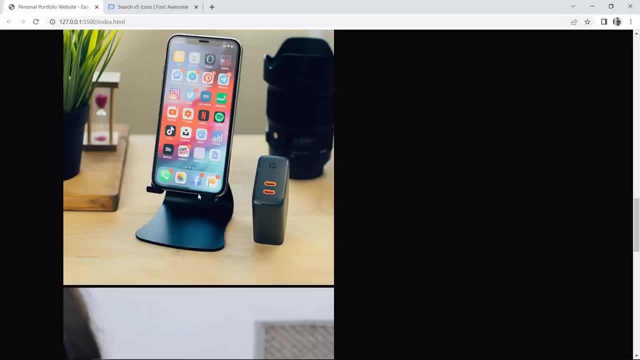 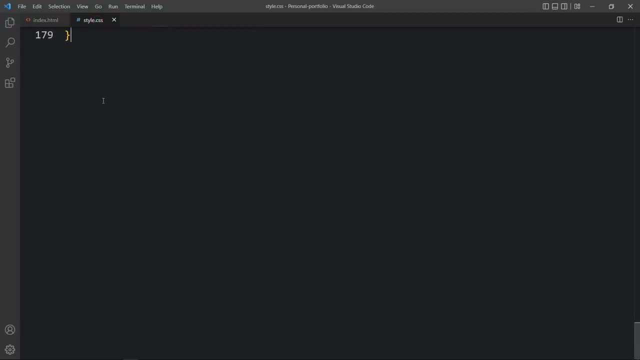 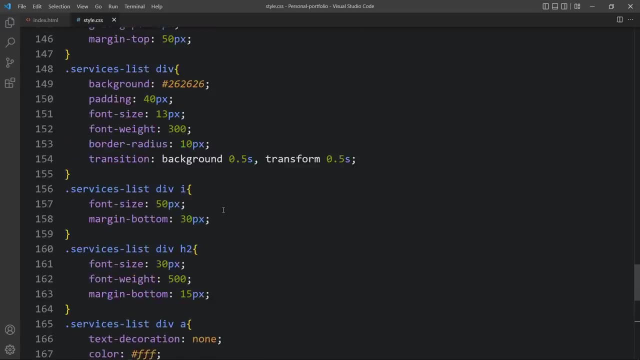 you can see 3 images here, so we have to arrange these images as a grid. so again, come back and copy this class name worklist, write it here in this css file and here also we will add the same css that we have added in the services. so let's see, here we have added display. 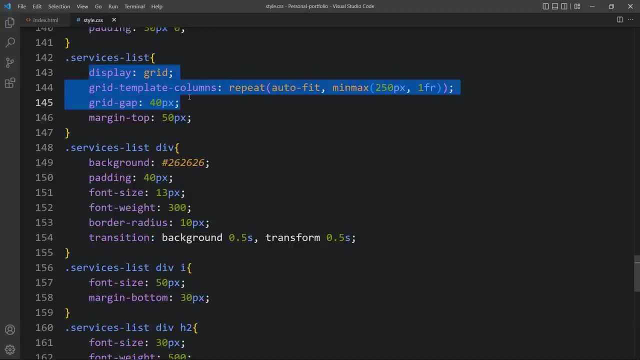 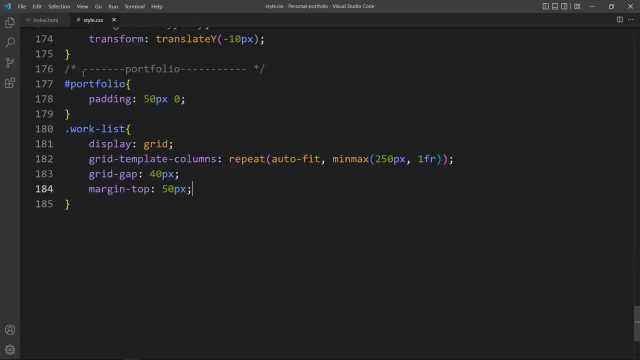 grid, grid template column and grid gap. so just copy this 3 line and we will copy this margin, also margin top. so paste it here in this worklist. after adding this, here we have the single work with the class name work. so right, this class name here work, and in this one we will add the 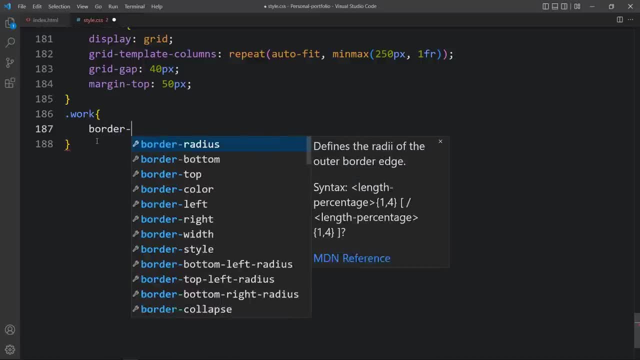 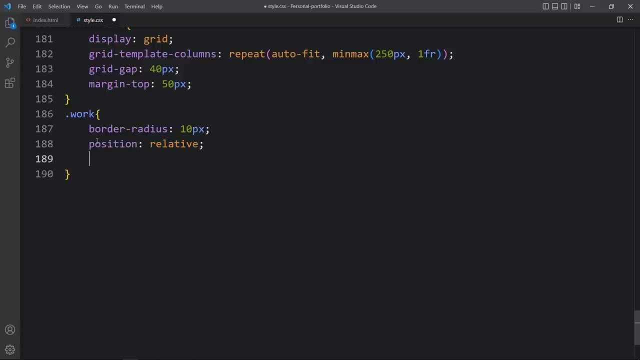 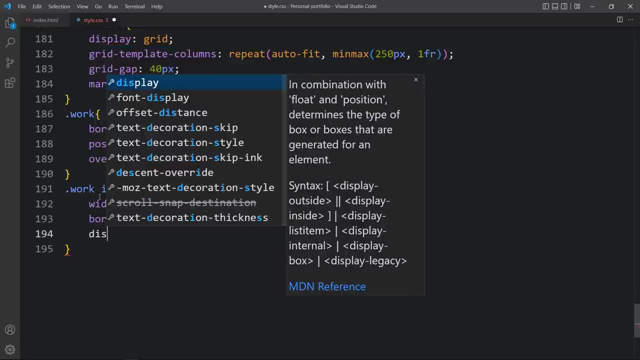 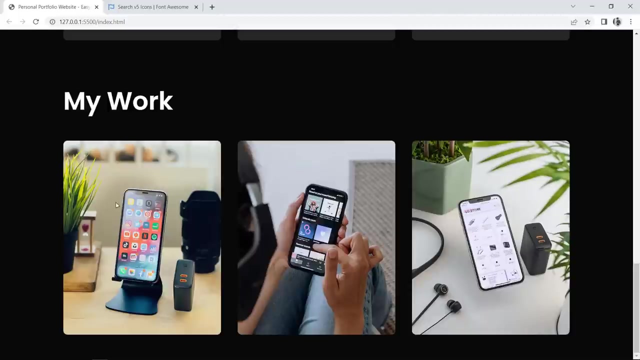 border radius: 10. pixel position: relative and overflow: hidden. again write this class name, then write img. in this one we have added the image, so we will add width: 100 percent. border: 10px display. it will be block. that's it. now you can see these images in grid layout next. 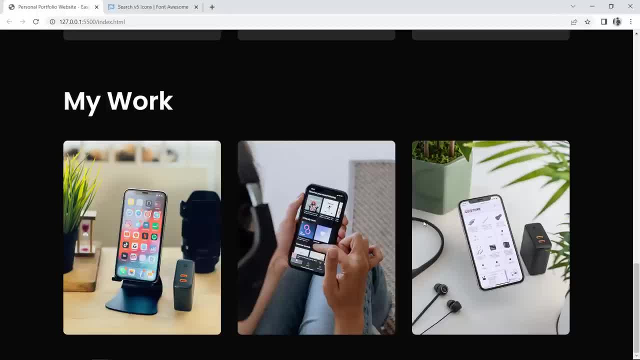 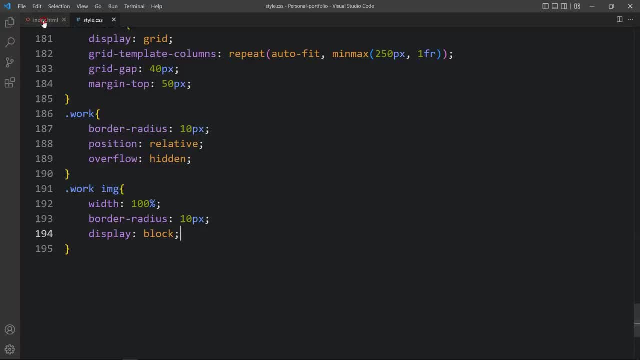 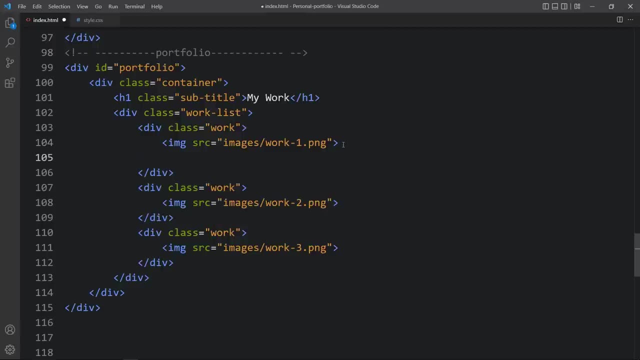 we have to add some information over this image, like there will be one title text and one link for that. we will come back to the html file and after this image we will add one div. so let's add space here, and here we will add one div with the class name layer. 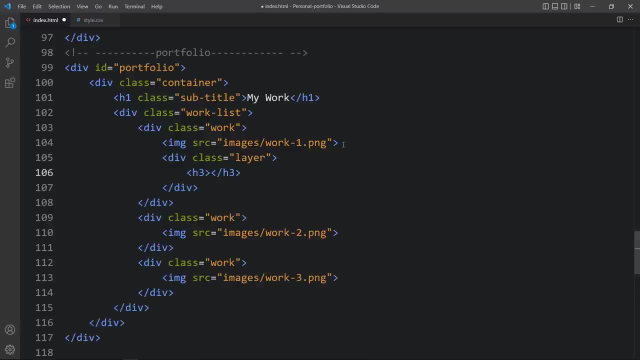 and in this one we will add one title. so let's add the title in h3. then we will add one description in b tag. so this is the description, and then we will add one link. so we will add a tag, and in this link there will be no text, we will just add one icon. so again come back. 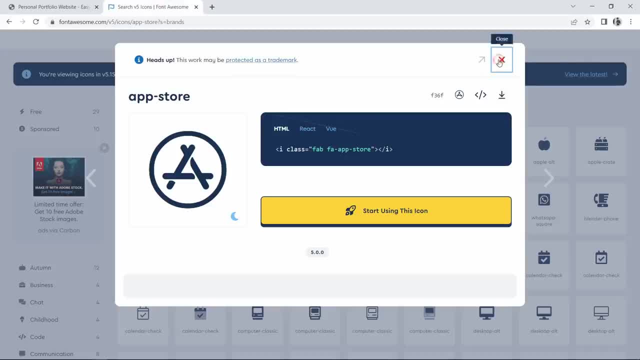 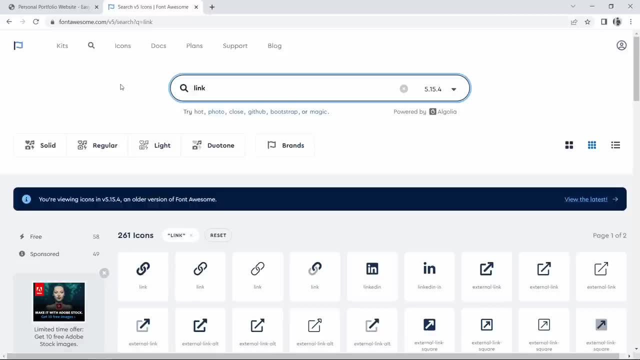 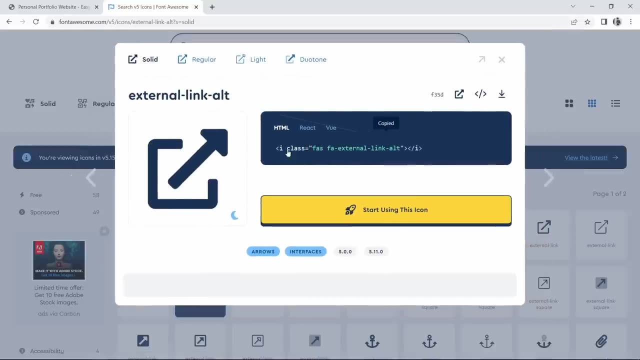 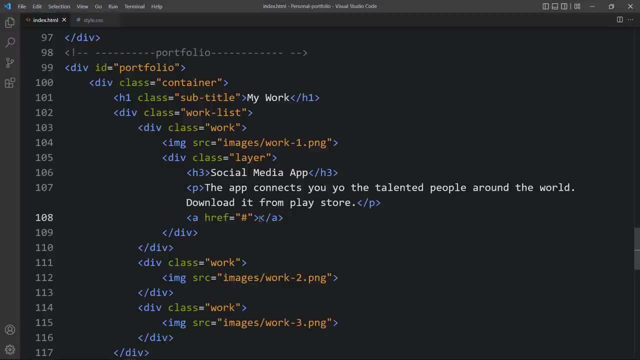 to the font awesome website and in this search box we will search for link. i will use this icon: external link alt. click here and click on this code and add it here in this html file within this a tag. so we have added this one. let's come back to the 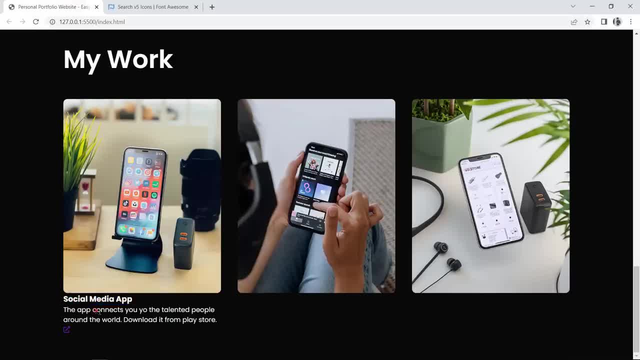 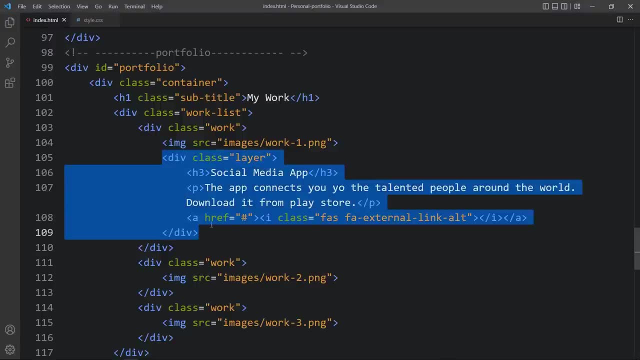 website again. you can see this text description and this link icon just below this image. similarly, we will add these things in all the work. so let's come back and copy this div, which is layer, and add it here in this second one, and in the third one we will change. 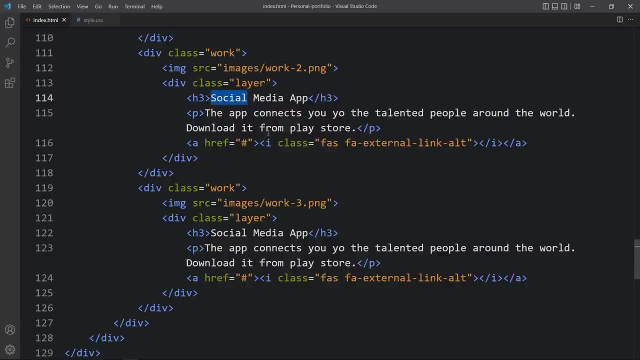 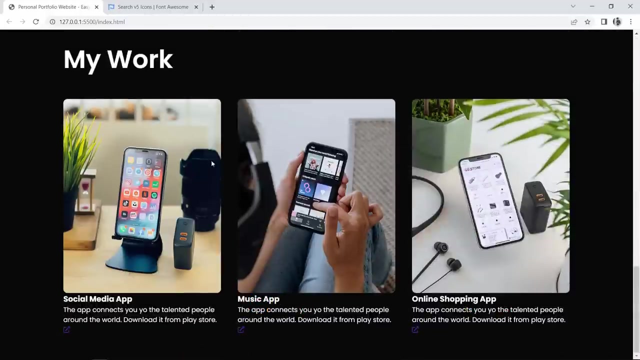 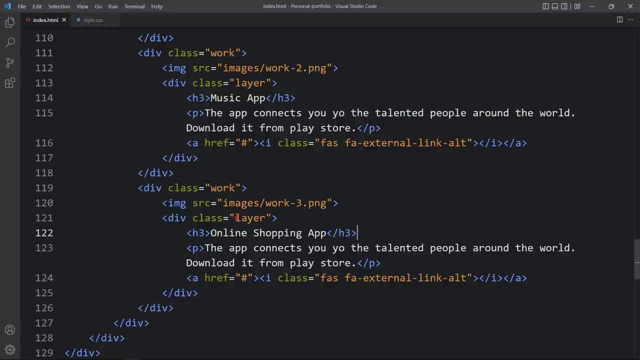 the text. you can see this title and description and link in all three work. next, we have to change its position and we will also add the background color. this text will be displayed over this image, so we have to add the position absolute. so let's come back, and here we have added the. 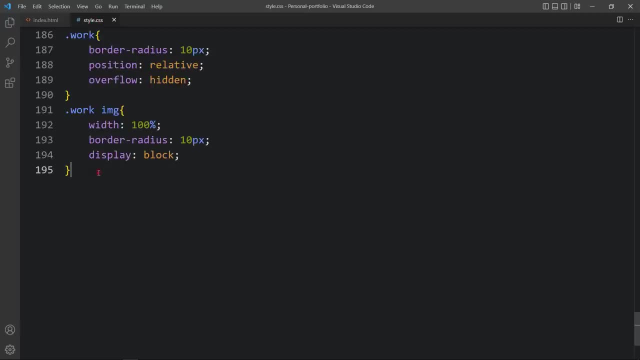 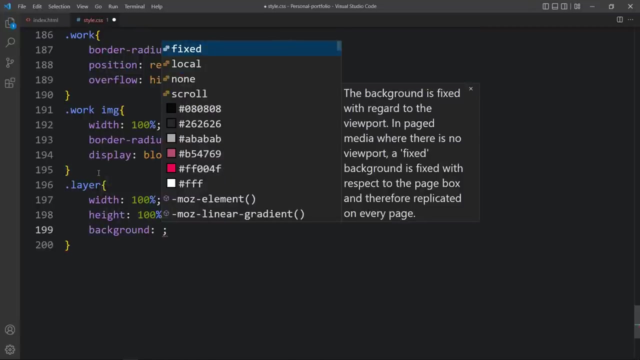 class name layer. so copy this, write it here in the css file. so for this layer we will add width. width will be 100 percent. then we will add height, height. also height, 50 percent. next we have to add the background. so in this background we will add gradient color. so let's. 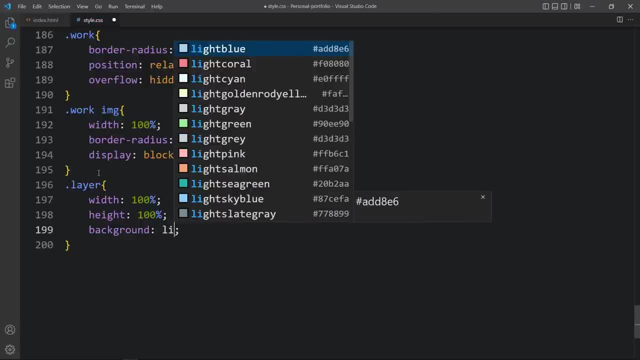 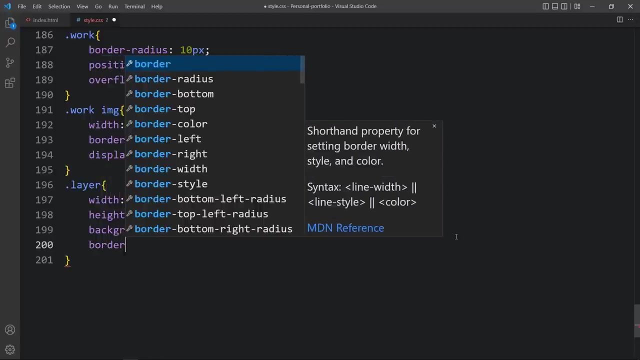 add linear gradient. first color code: it will be rgba: zero, zero point five. it will be black color with 60 opacity percent. then we will add this color code, then we will add the color code Zachary. After that we will add the border radius: It will be same: 10px. 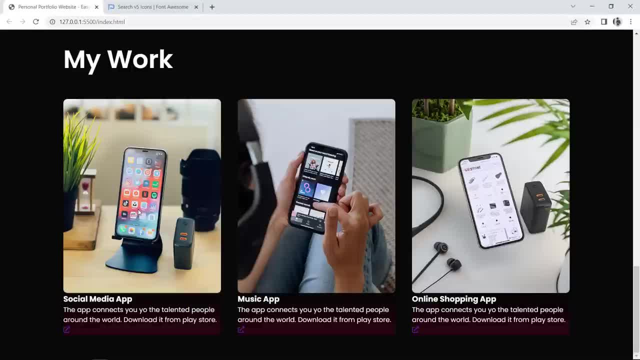 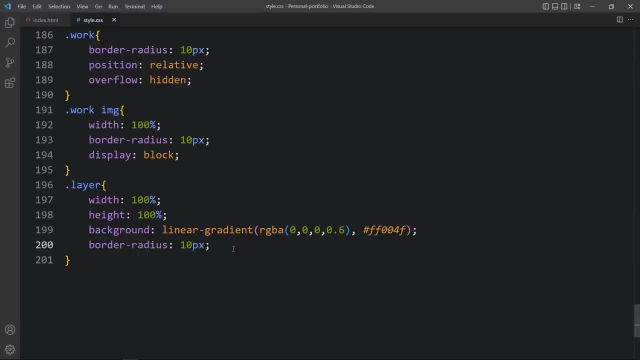 After adding this, let's see this on web page. So it is at this position. So we have to change its position. So let's come back Here. we will add position absolute, Then we will add left. It will be 0.. 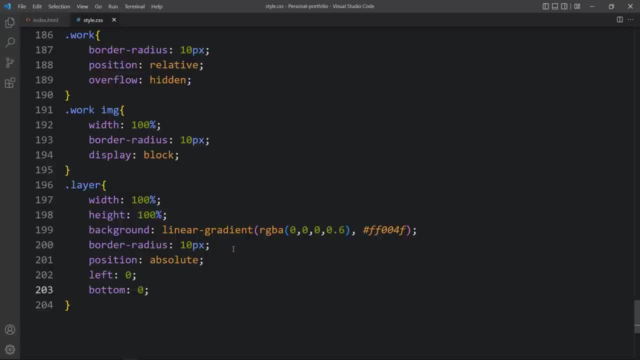 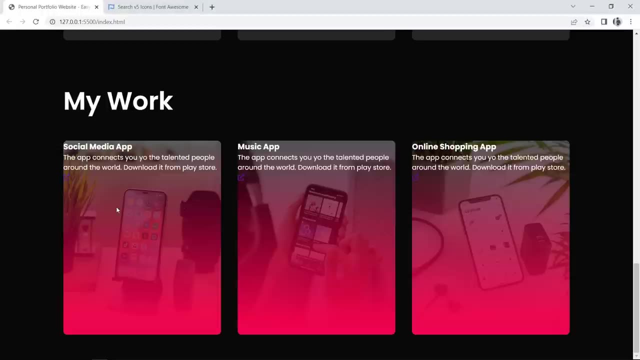 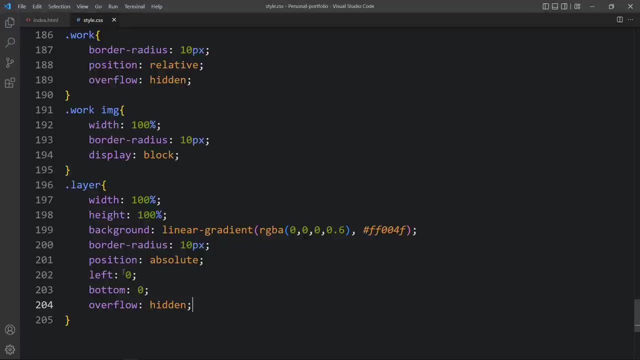 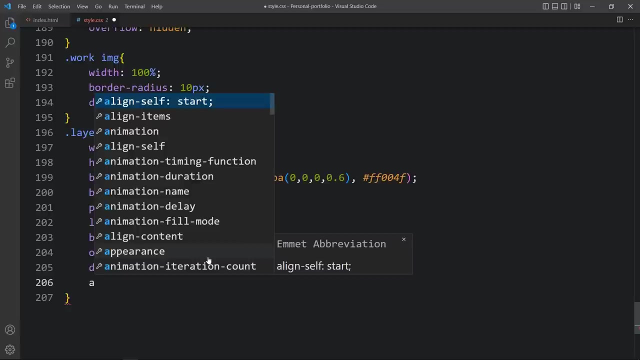 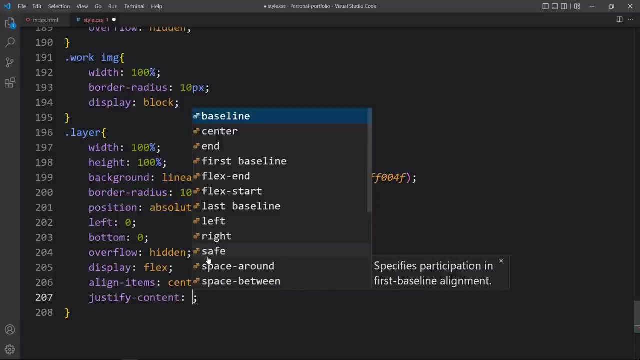 And bottom 0.. Now overflow hidden. You can see it is just over the image. We have to move these text in the center. So let's come back and here we will add display flex, align items center, justify content center and flex direction. 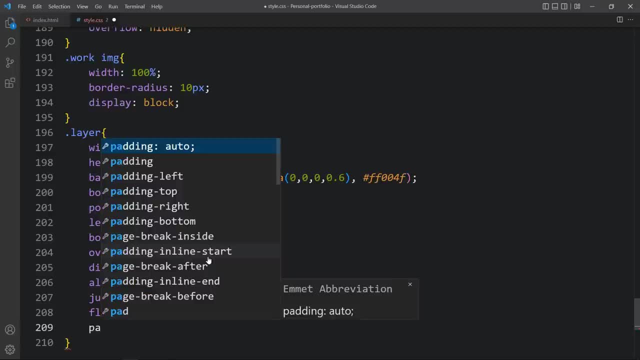 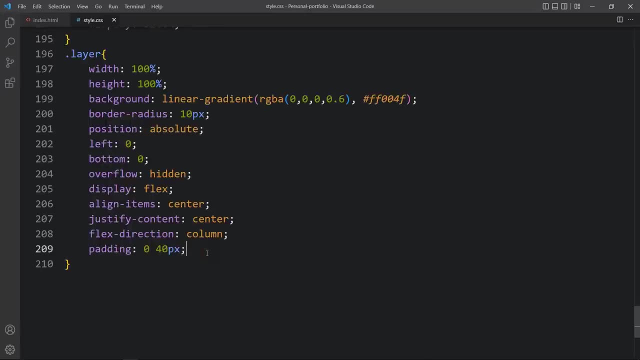 It will be column. Then we will add some padding- 0 and 40px, So we will add some space in left and right side. We will add text align center. After adding this again, come back to the website. You can see these text in the center. 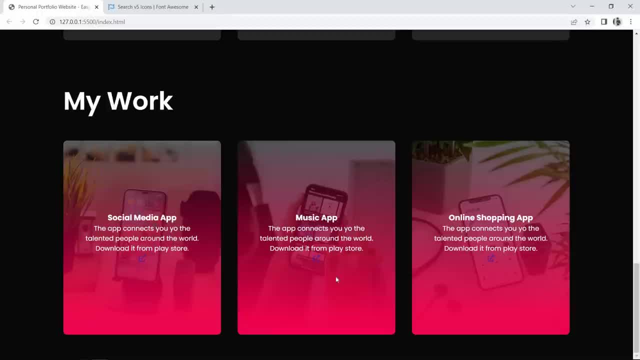 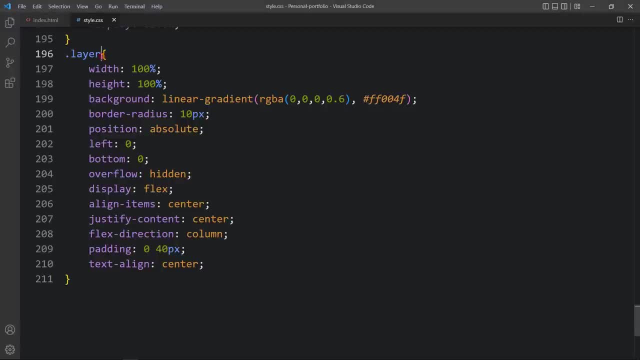 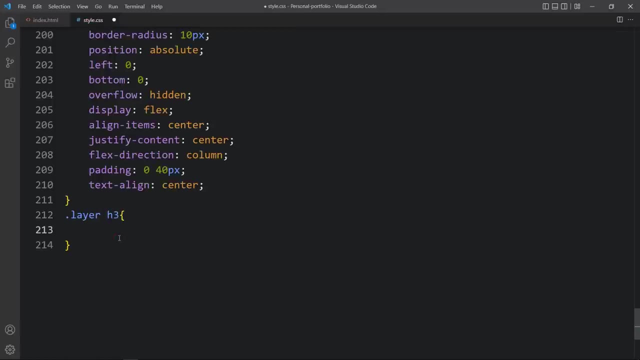 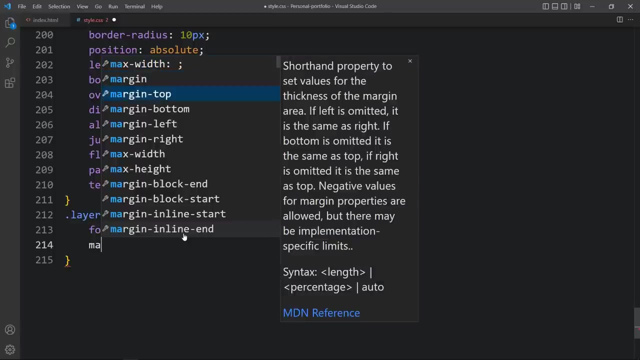 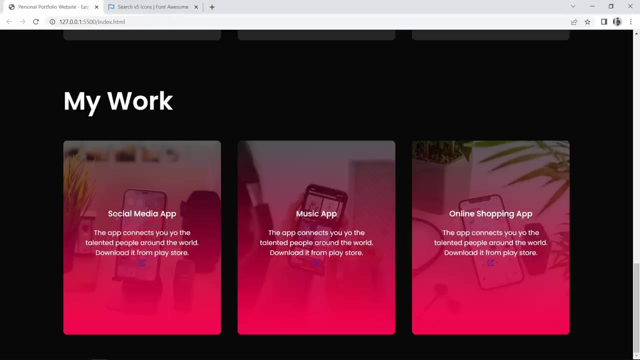 Next we have to change the font size and we will also decorate this icon. So let's come back and here we will add dot layer h3, because we have added the title in h3 tag. Let's add the font weight- It will be 500- and some space margin, bottom 20px. 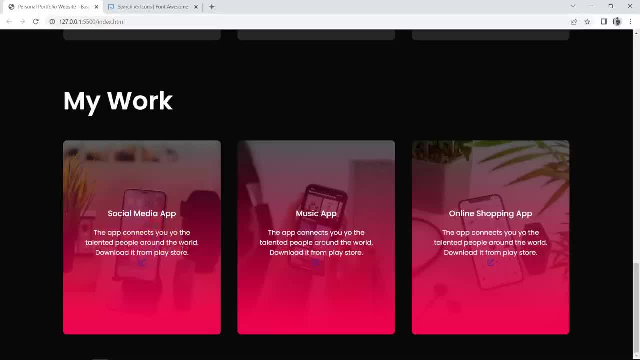 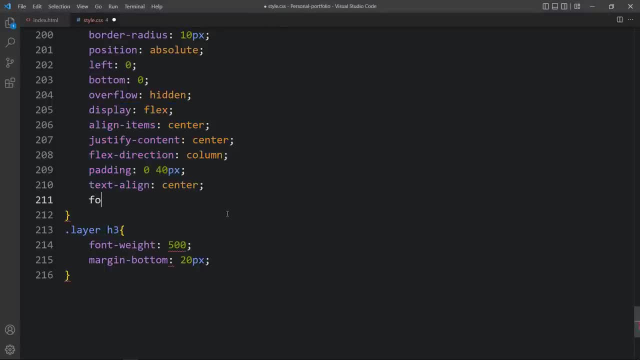 Now we have to decrease the size for this text, which is description text here. So let's come back and in this one, which is for the layer here, we will add the font size. font size will be 14px. Okay, So you can see decreased size for this text. 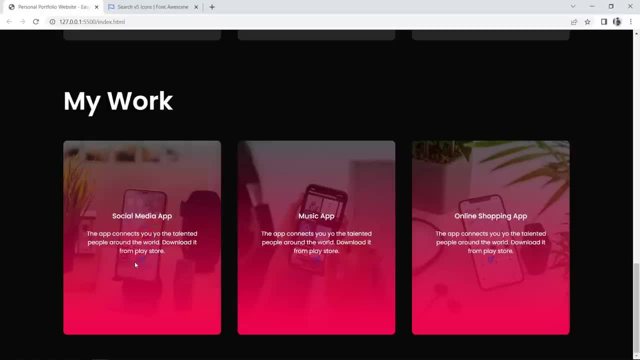 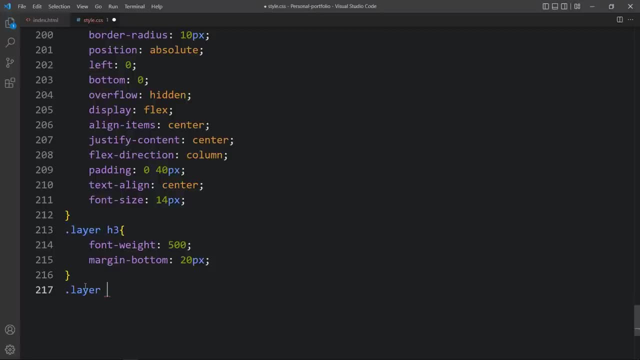 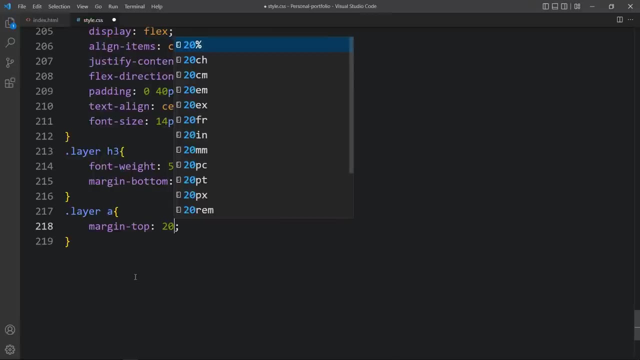 Next we will design this icon, which is the link icon. So again come back, copy this layer And in this layer we have the a tag. So in this a tag we will add the space margin top 20px. then we will change the color. 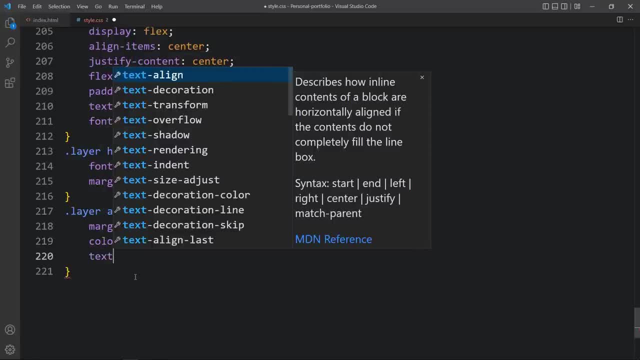 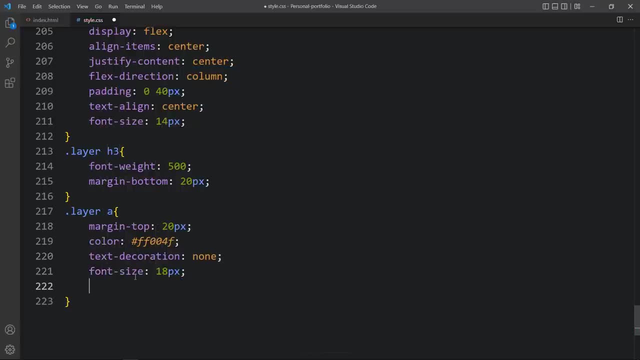 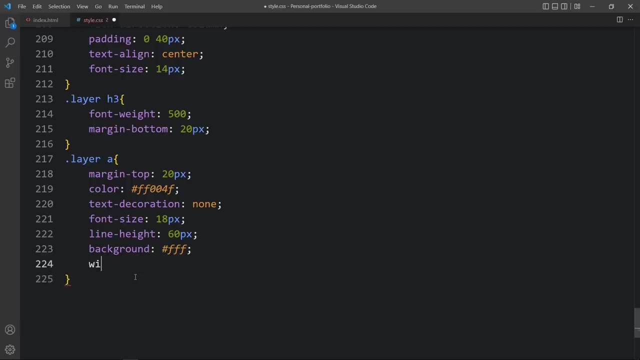 This color code. After that we will add text decoration: none. Then font size 18px and line height 60px. Then background background will be white color. Now we have to define the width and height. So width will be 60px and height also. 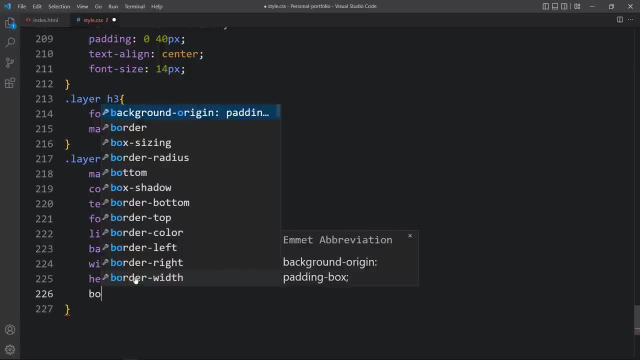 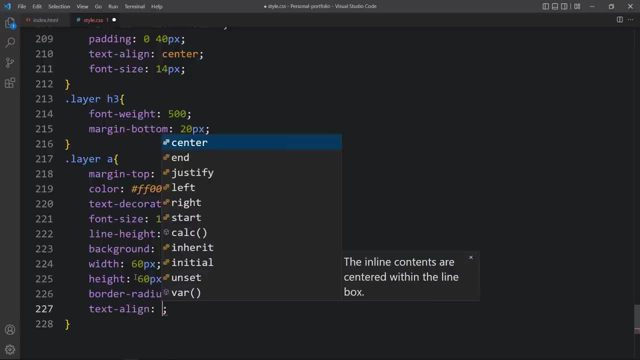 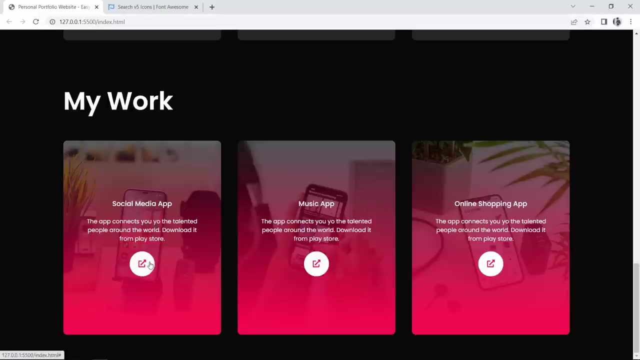 Okay, Then we will add border radius. Water radius will be 50%, so that it will be a circle, and text align center. After adding this, this external link icon looks good. So right now these contents are displaying by default, So we have to hide this one, and it will be visible whenever we will take cursor over. 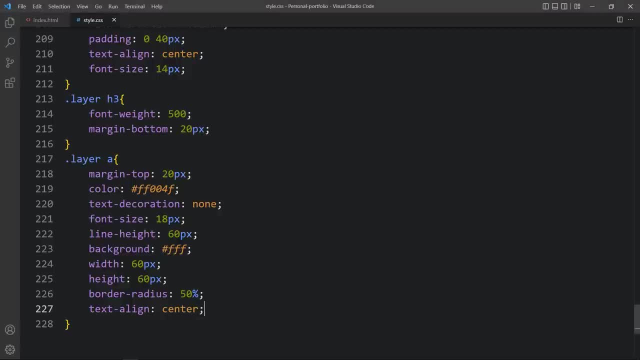 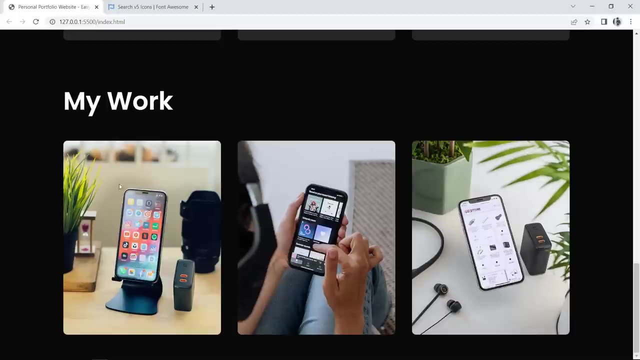 anyone. So to hide this one, let's come back here. We have added Height 100%, so we will make it zero And let's see it is hidden And whenever we will increase the height so it will again become visible. 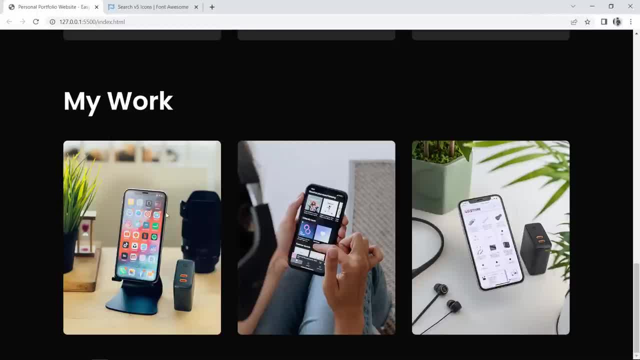 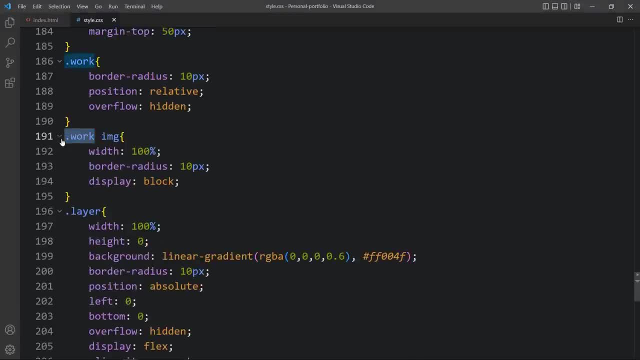 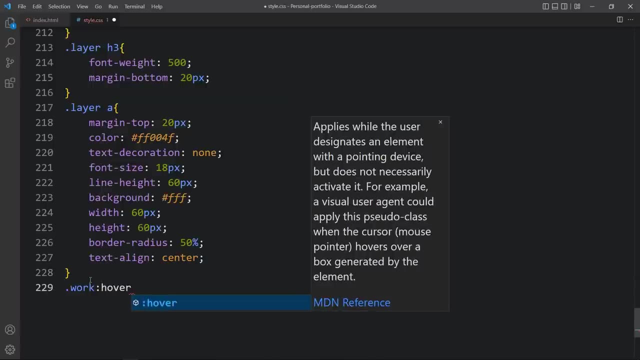 Before that, we have to add one more hover effect. If I take cursor over it, this image should zoom in. So let's come back and here we will add this work, Paste it here. Work Hover. Okay, And whenever we will take cursor on this one, it should increase the size for the image. 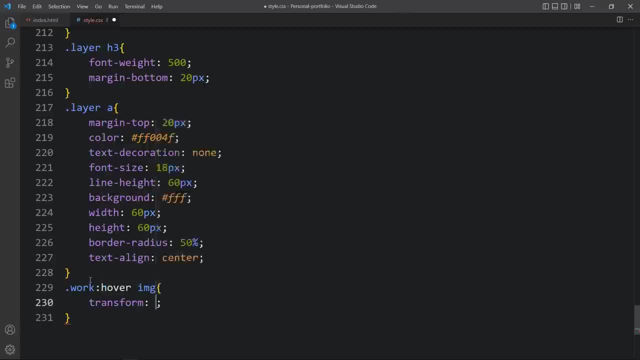 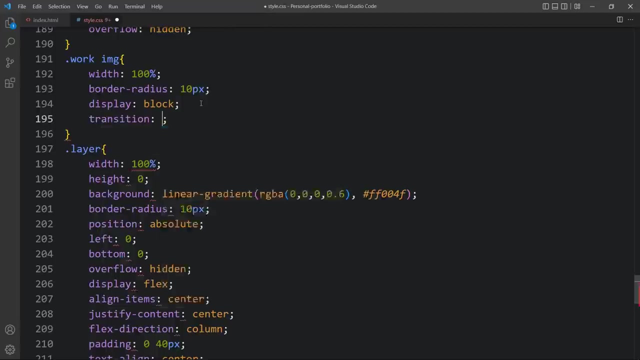 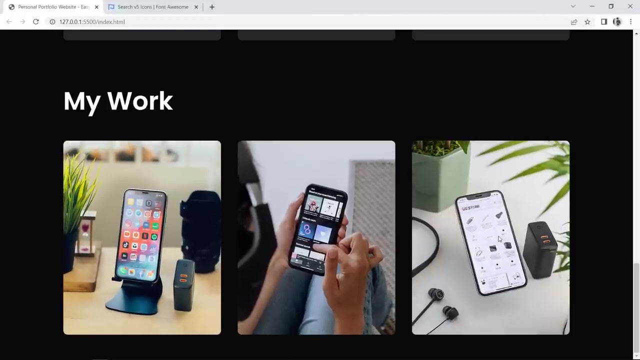 So we will add IMG and write transform scale 1.1 like this. And let's come to the top over here in this work: IMG, we will add transition transform. Okay, Okay, Okay, 0.5 seconds After adding this. you can see, if I take cursor, this image gets zoom in. 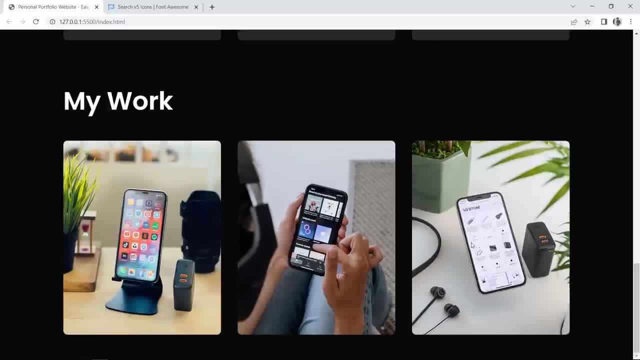 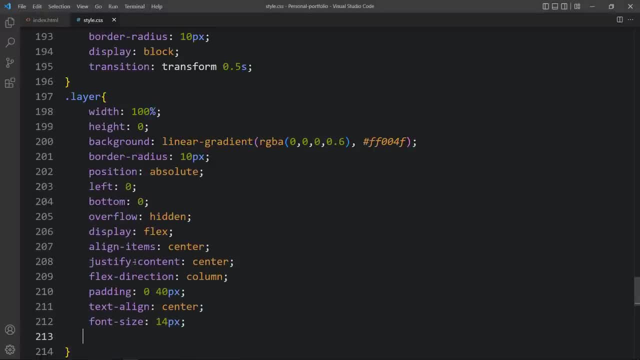 So this is the first effect on this work image. Next, we have to display the content that we have added over this image, which is hidden right now. So let's come back. You can see we have added height zero for this layer, So again, we will add this one. 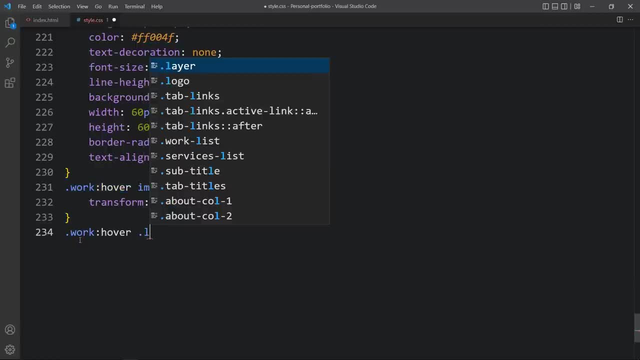 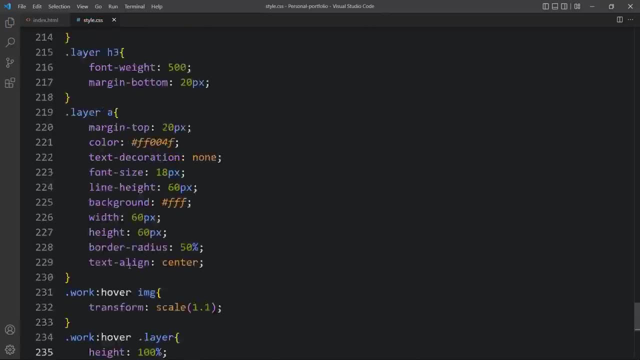 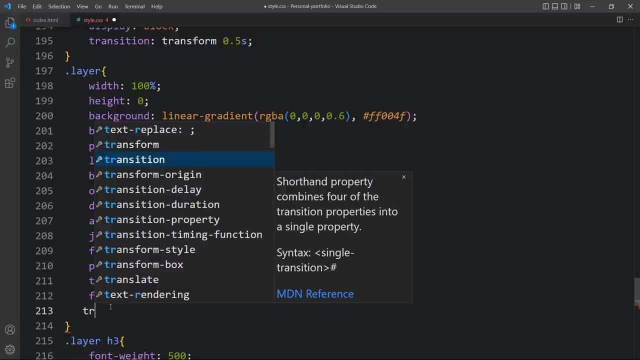 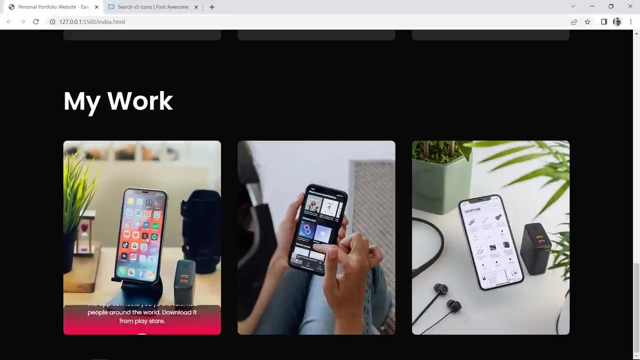 Then Right Dot Layer And right Height 100%, So it will increase the height. Let's come back to the layer which is here. So here we will add transition height: 0.5 seconds. You can see when I take cursor. this text is coming from the bottom. 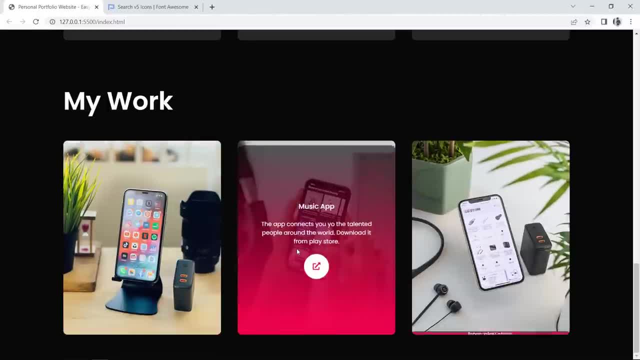 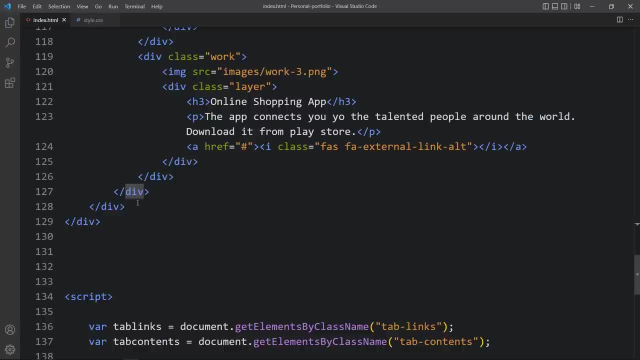 Okay, After adding this, we will add one button. So let's come back. come to the HTML file. You can see this div worklist is closing here, So here we will add a space and add one link with the a tag. 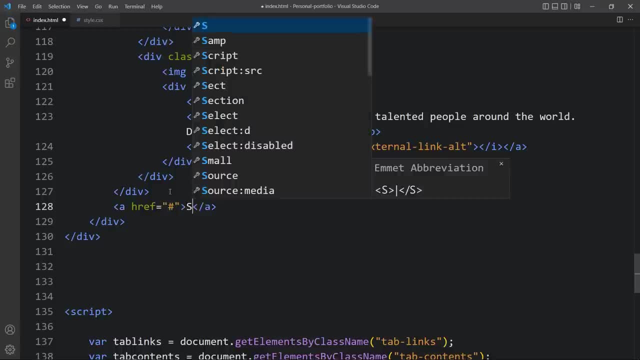 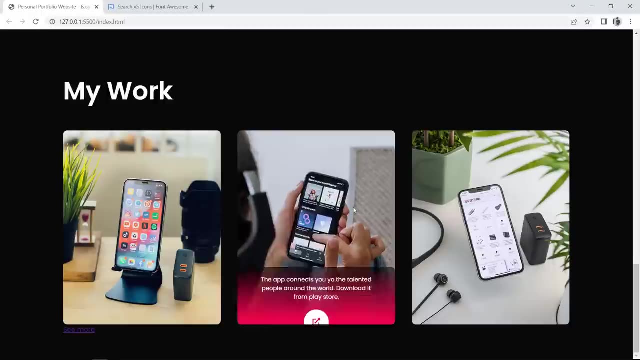 And in this one we will add the link text: See more. We will add one class name, So write the class name called BTN. You can see this link here at the bottom. See more. We have to move its position and we will decorate it as a button. 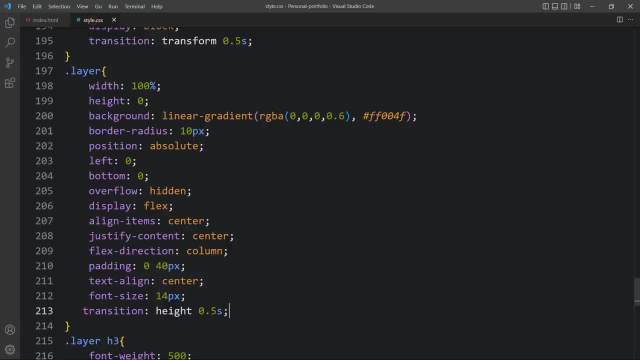 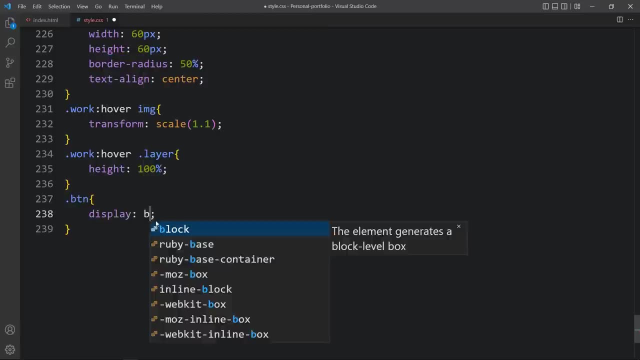 So let's come back and copy this class name BTN, Write it here in this CSS file right dot BTN. In this one we will add display. Display will be block, Then margin: We will add margin: 50 pixel from top and bottom left, right, auto. 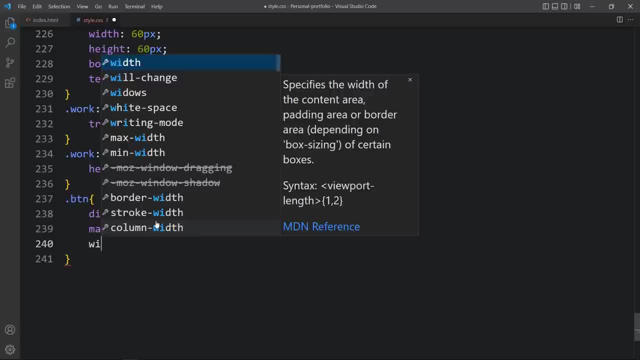 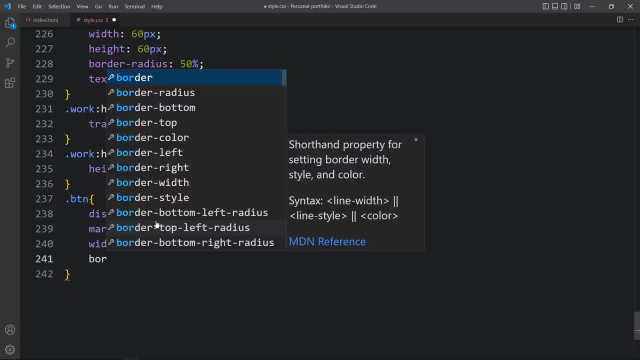 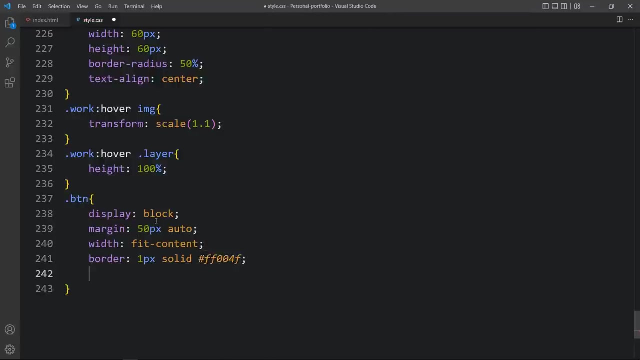 So it will be in the center. Then write width. Width will be fit content, Then border Border will be one pixel solid and this color. After that we will add some padding. that will be some space inside the button. Border radius will be six pixel. 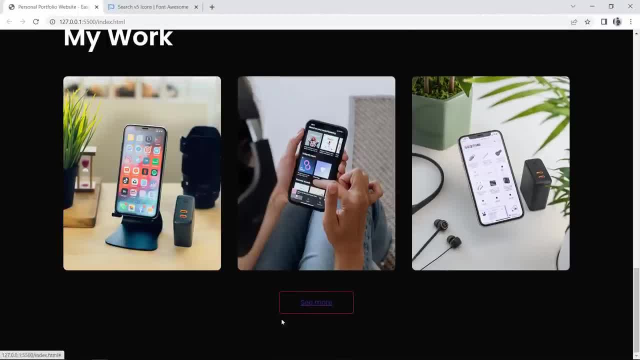 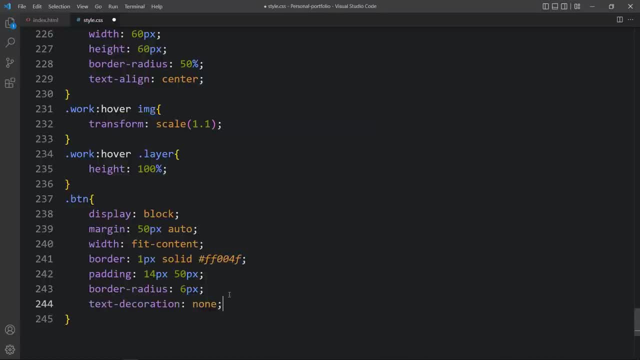 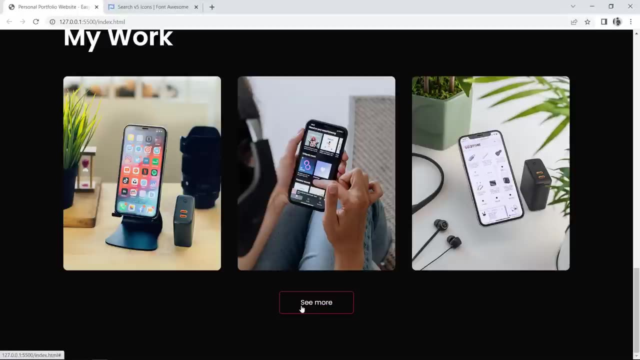 You can see it looks like a button. We have to change its color also and we will remove this underline. So here we will add text decoration none and color white. So it is looking good. Next we will add one hover effect on this button. 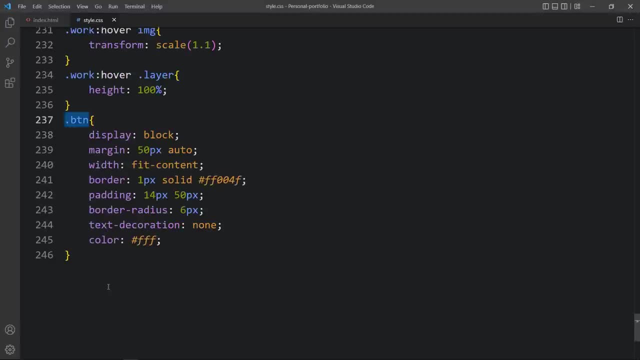 So let's come back and copy this button, Then write colon hover. Let's add the background. Background will be this color code: Very good, Whenever we will take cursor, the background will be changing And here in this one we will add transition, transition, transition for the background. 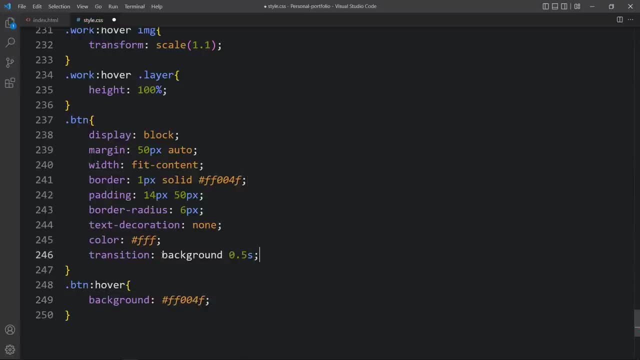 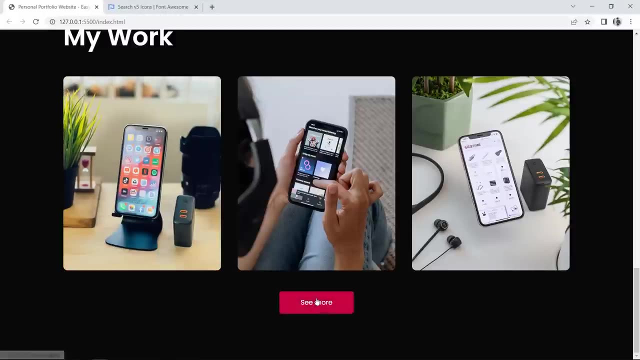 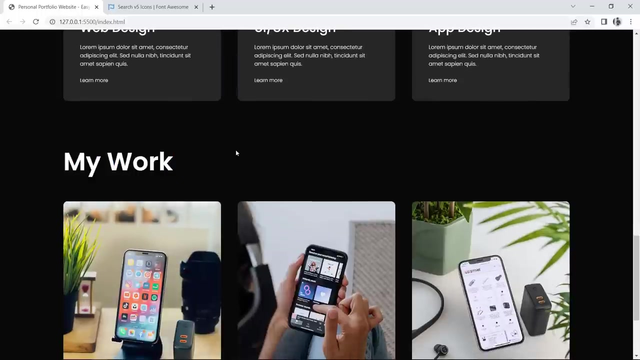 Let's add transition background: 0.5 seconds. You can see if I take cursor over this button, the background is changing. So finally, we have completed this portfolio or my work section also. Next we will create the contact section, where we will add the contact information, like phone. 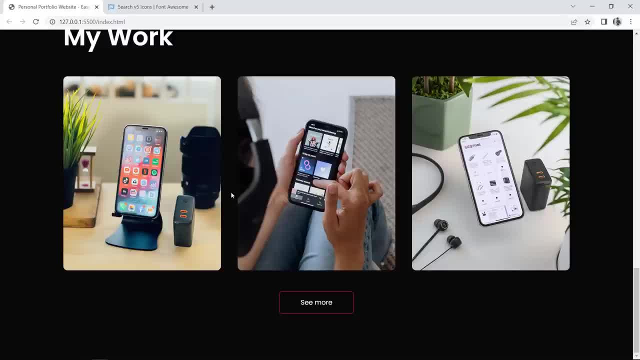 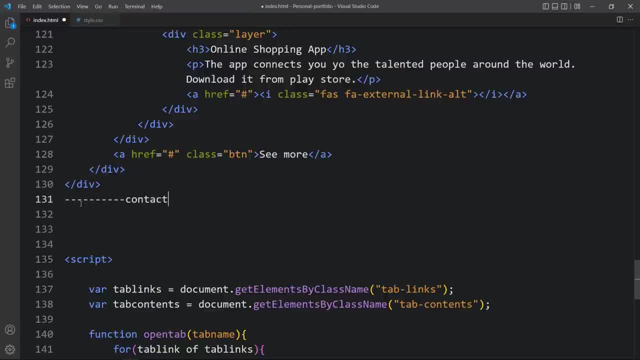 number, email ID- and we will also add one contact form For that. let's come back to the HTML file and here we will add one comment- contact- And let's create one div with the ID contact. So here we have one div with the ID contact. 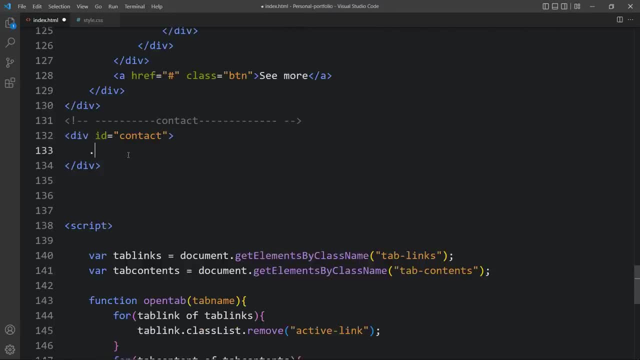 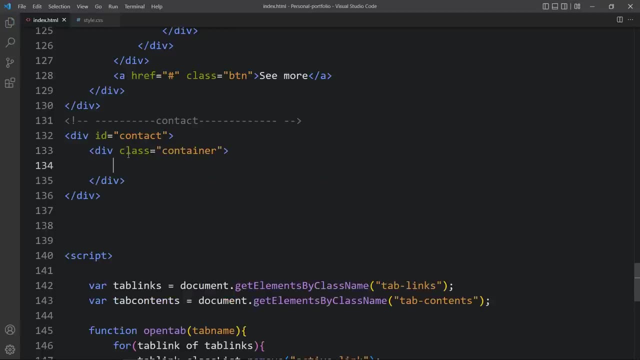 Okay, In this one again, we need one container And within this container we will add contents in two columns. In the first one we will add the contact information, like phone number, email ID and social media links, And in the right column we will add the contact form. 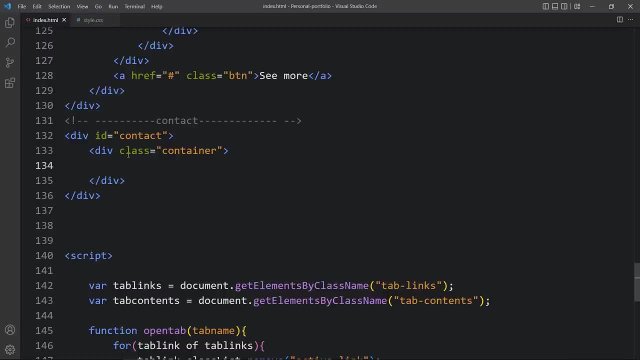 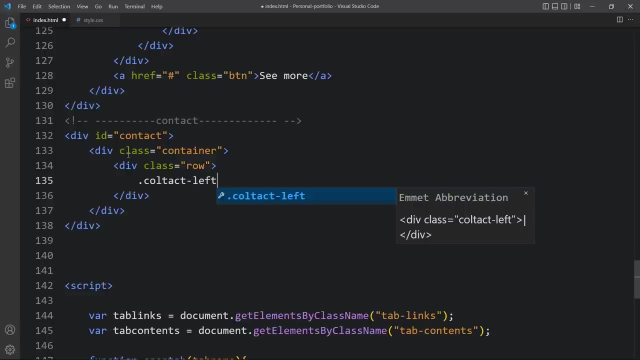 So here we have to create two columns. So first we will create one div with the class name row. Now in this row Let's create One div with the class name contact left. It will be for the left column, Just duplicate this one. 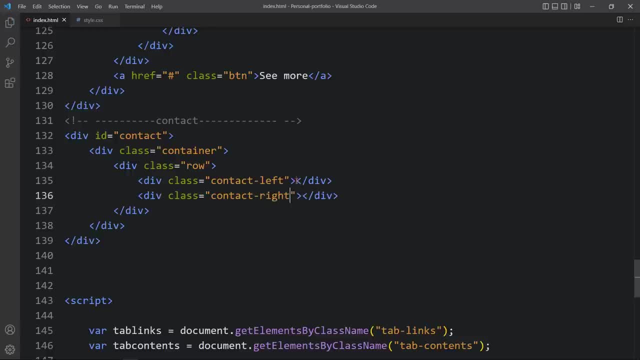 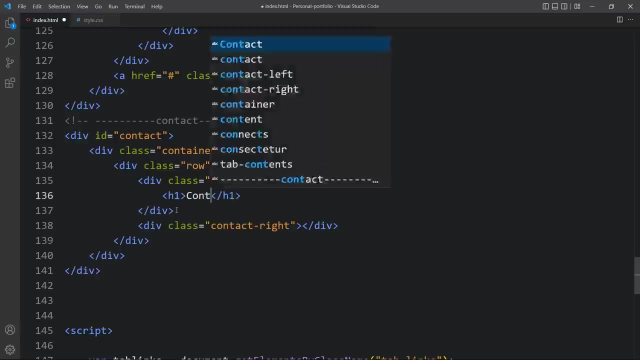 Here we will add contact right, So it is for the right column. Now, in the first one we will add one subtitle, So let's add one h1 tag. In this one we will add the text contact me and the class name that we have already. 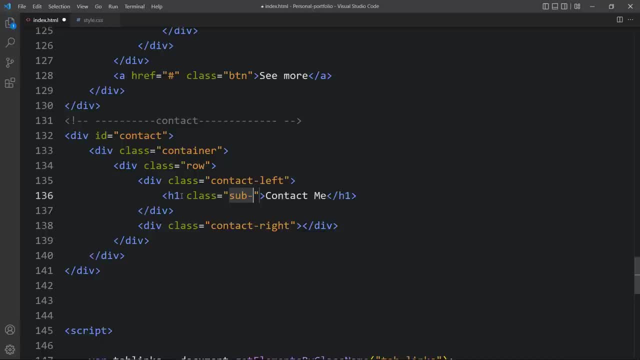 used subtitle And after that we have to add the email ID In p tag, Then we will add the phone number And next we will add the social media icons. So let's add the div With the class name Social icons. 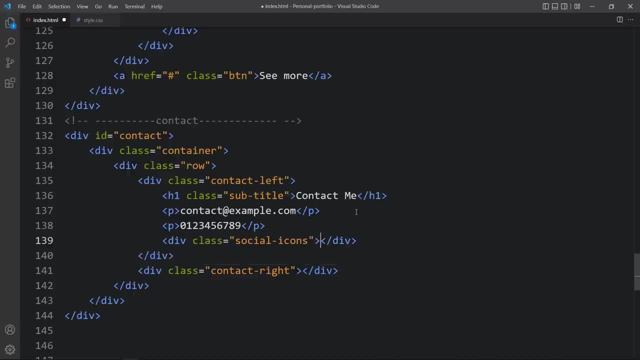 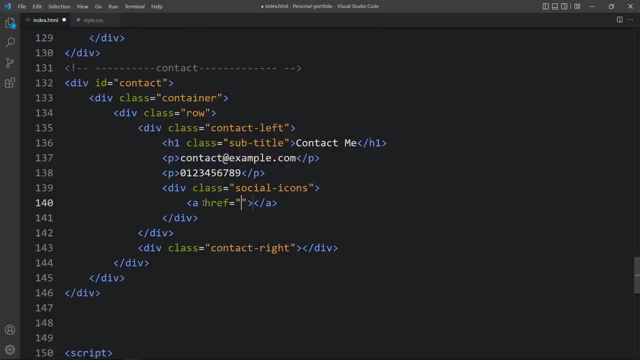 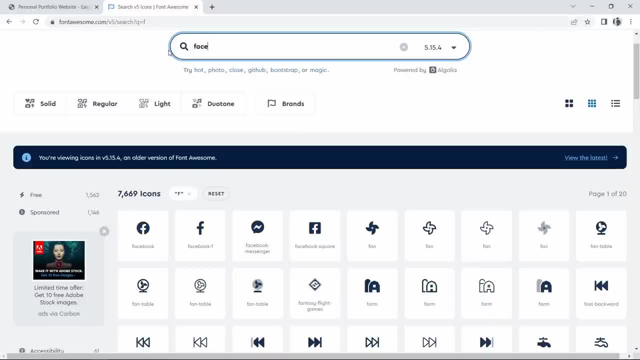 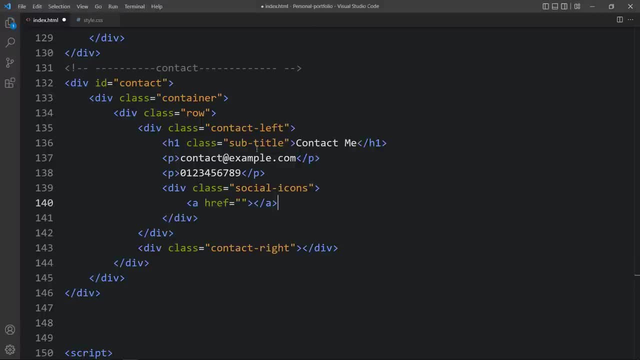 Here we will search for the icon Facebook. Let's click on this one. Copy this And paste it here. want to display the icon? let me duplicate it. you can go on the font awesome website and search for another icon code. i already know, so here i will write. 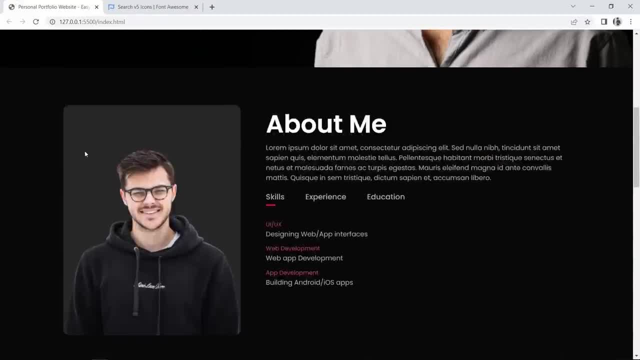 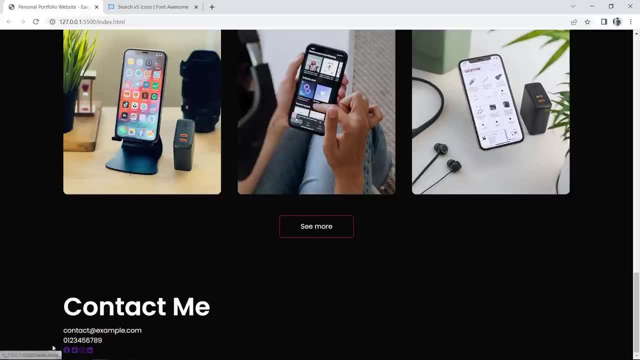 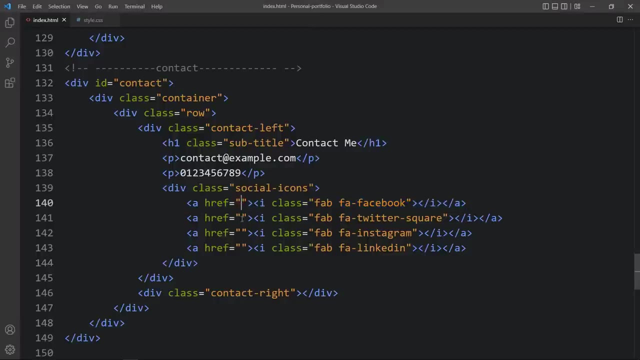 after adding this, let's come back to the website again. here you can see contact me this email id, phone number and social media links. suppose you want to add the profile link here, so let's come back and in this href here we will add the social media profile link like this one: 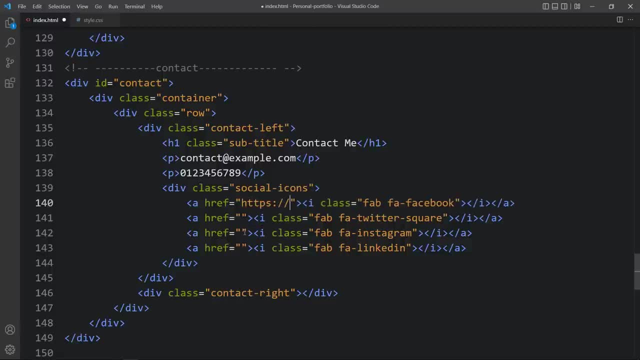 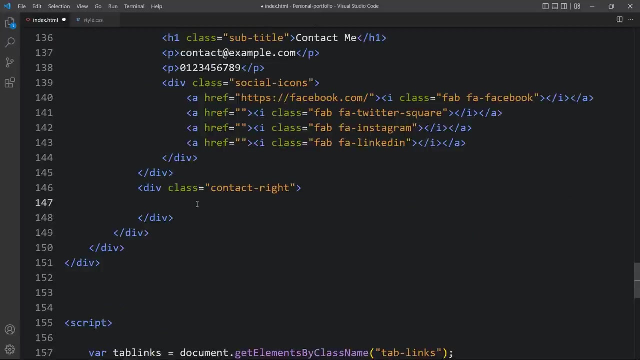 write the complete profile url here, and now we have to add some content in the right column, which is here here, and in this one we will create one form. so here we will add form tag and in this form there will be some input field for the name, email id and message. so first we will add: 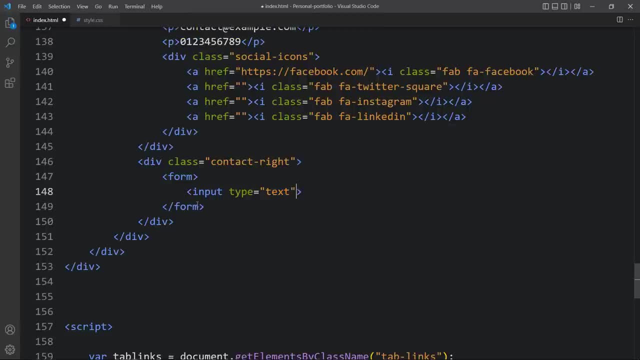 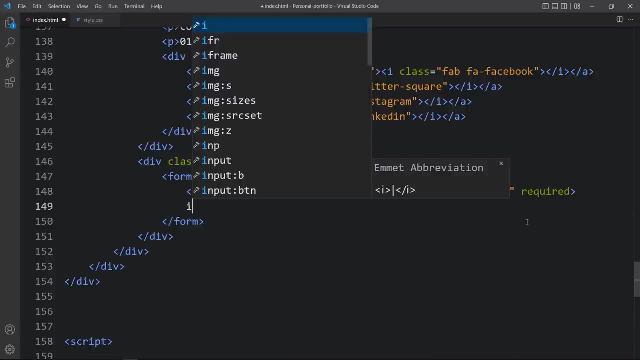 one input field for the name. input type will be text, name will be name, then placeholder it will be your name and this field will be required. next, we will add another input field which is for the email. name will be email placeholder- your email, and it is also required. 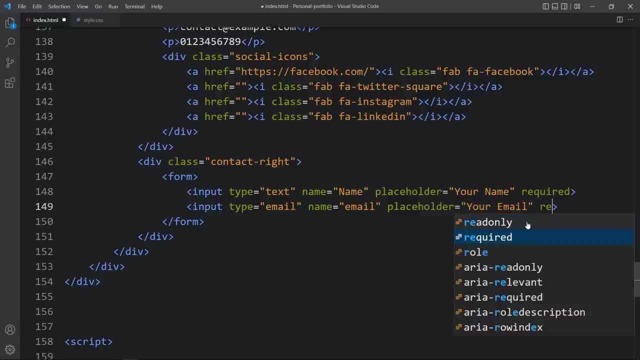 ok, then will add the text area. in this text area we will add the name called message: remove this id and columns row it will be 6, and then placeholder. in this placeholder we will add your message. ok, so this will be our message. ok, after this text area there will be one submit button, so we will add button. type will be: 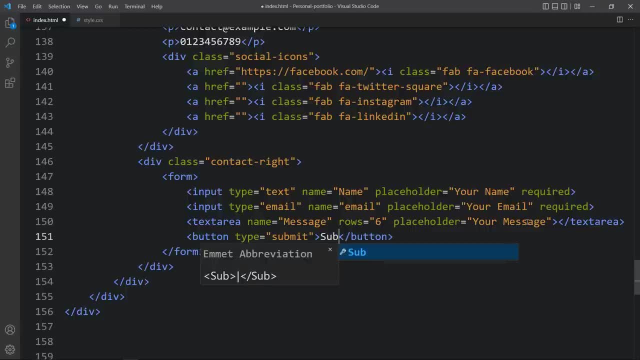 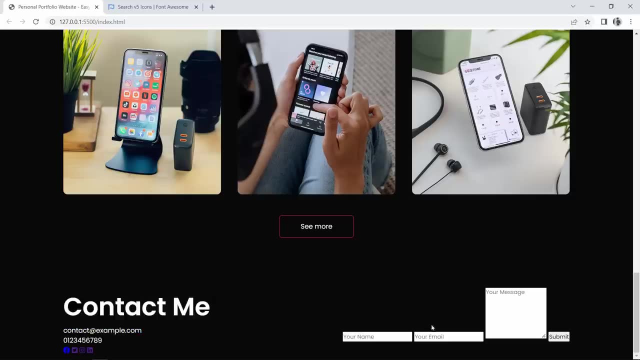 submit and button text will be submit. let's check this by page again. here you can see the contact information in the left side and this form input fields in the right side. next we have to define the width for left and right columns. so let's come back and here we have. 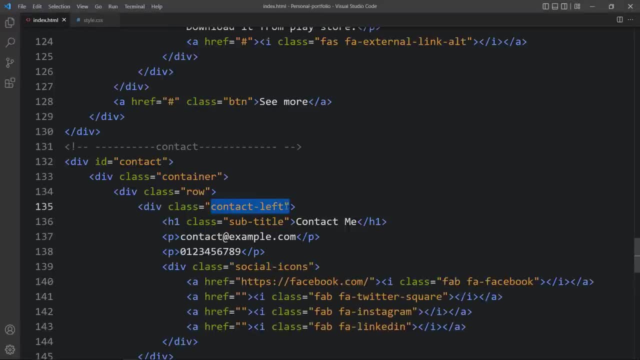 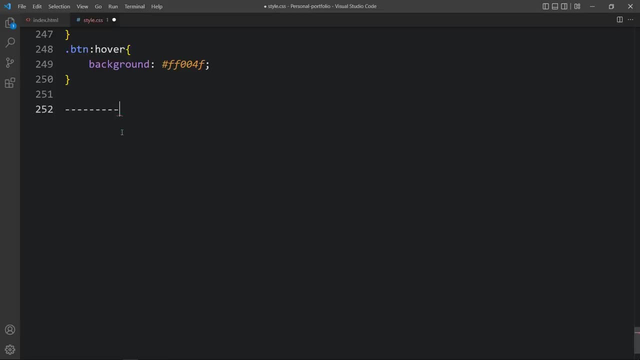 to add the css for this contact left, copy this one. come to the css file. first we will add comment here: contact. then write this class name: contact left for the left column. now for this left column we will add the width. so first we will add the flex basis. it will be 35 percent for the left side. now just duplicate. 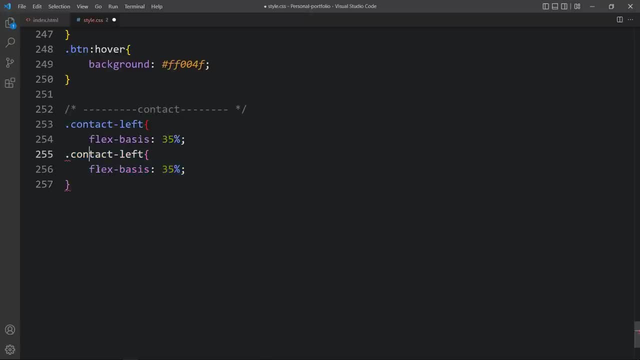 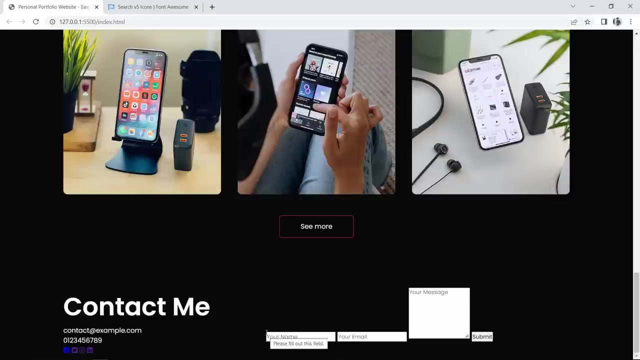 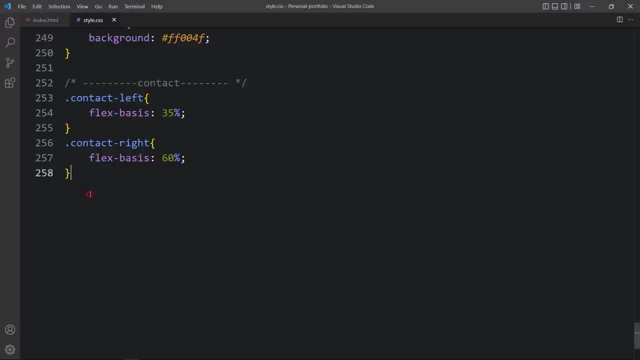 it and change the class name, it will be right, for the right one. width is 60 percent, so flex basis: 60 percent. now this form is starting from here. so first we will design the text and icons, which is in the left side. so let's come back and copy this class name, contact left, then write p. 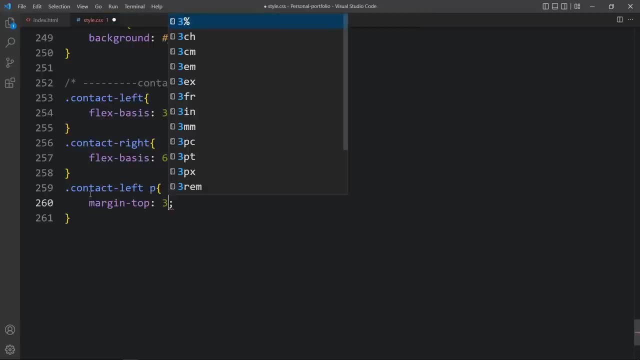 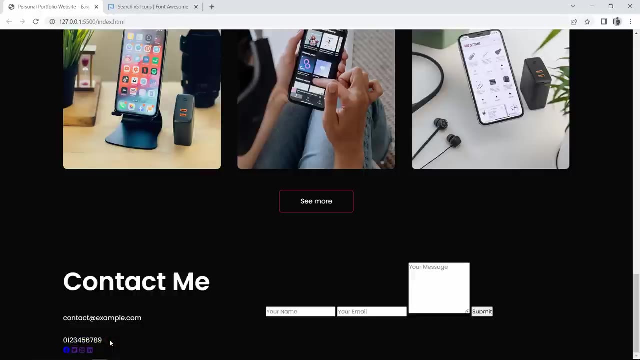 in this p we will add margin from top. it will be 30 pixel. we have some space here now for this email id and phone number. also, we will add one icon. so come back here and here we will search for one icon. search for one icon. 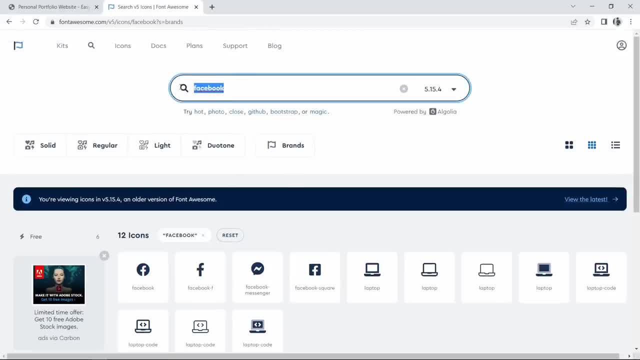 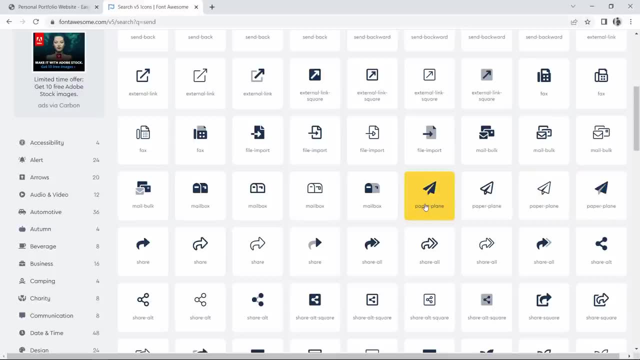 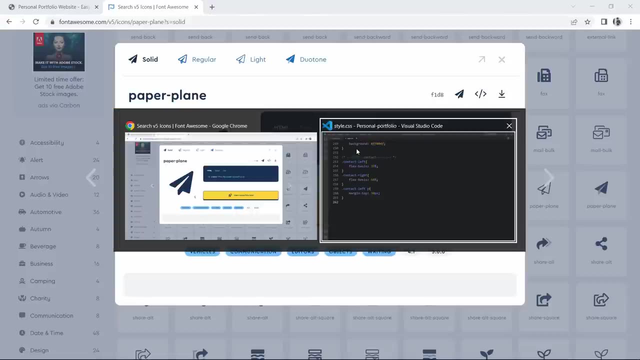 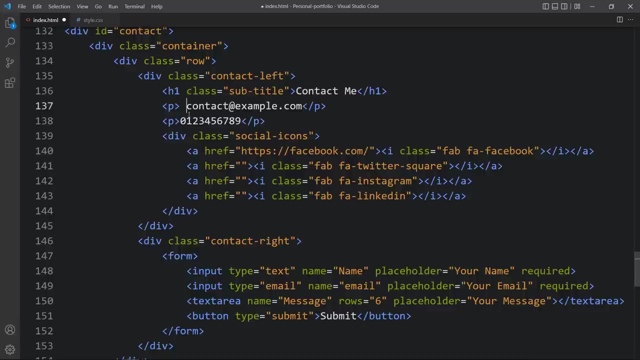 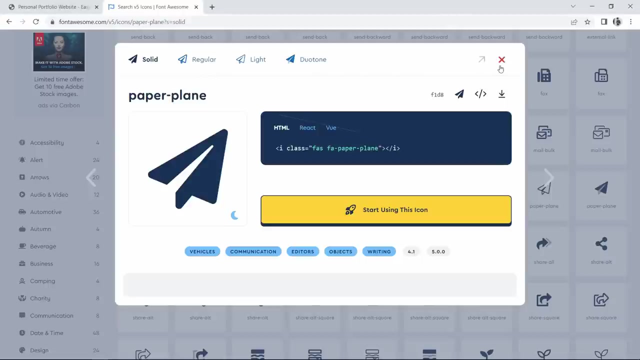 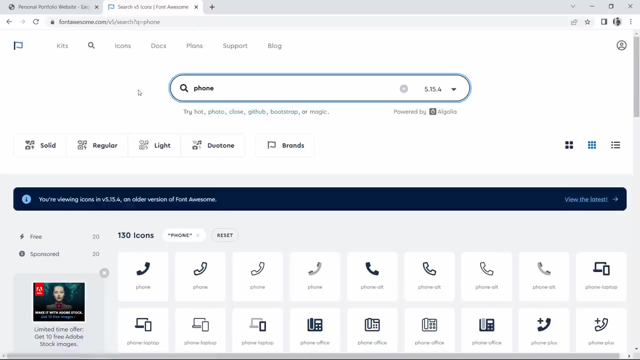 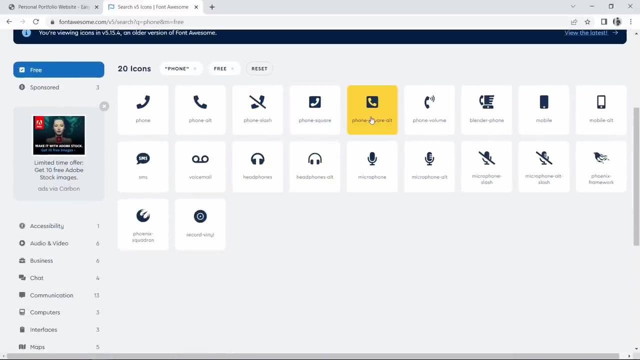 search for one icon. let me search send. let's click here and copy this one. add it here in this p tag this icon and email id. again come back and here we will search for phone icon. so let me search phone, then i will use this one. 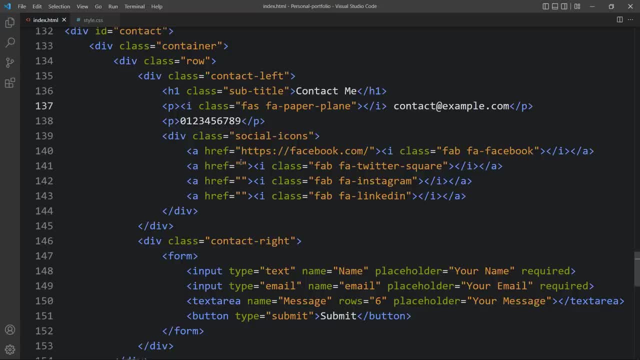 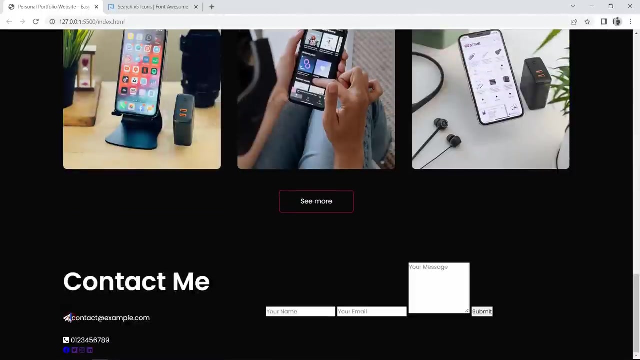 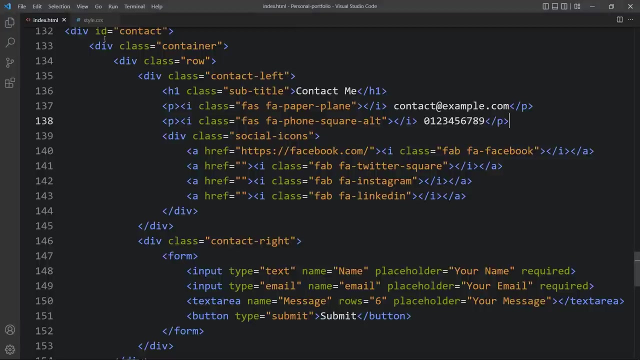 click and paste it here in front of the phone number. again refresh the website. so here you can see, we have the icon in front of email id and phone number. so we have to design these icons. so let me come back and in this css file we will add: 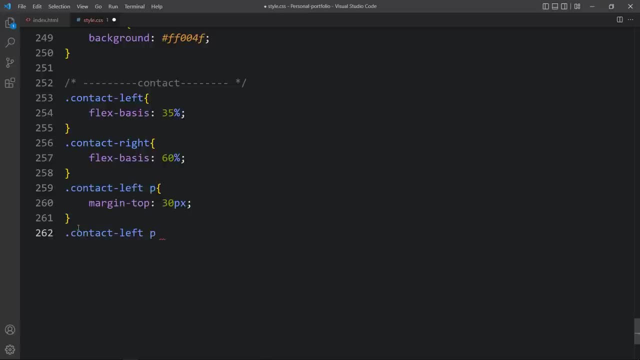 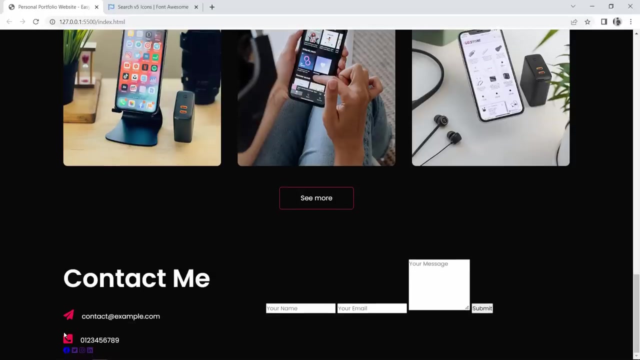 contact left p. and in this p we have added the icon with the i tag. so for this i we will add the color, then we will add the margin from the right side and font size. so this icon is looking good. next we will design the social icons. 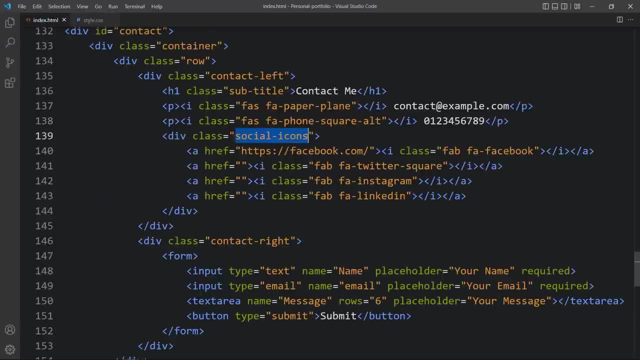 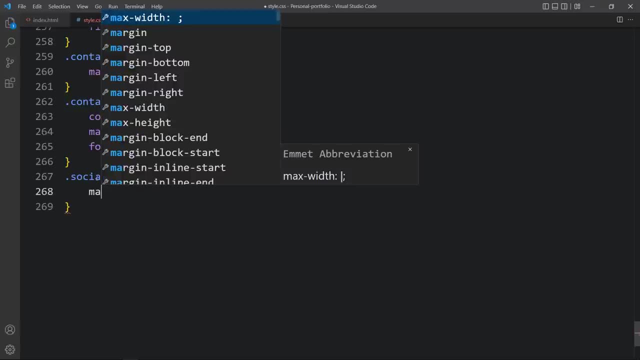 so here you can see the class name: social icons. copy this one. write it here in this css file. here we will add margin from the top. it will be 30 pixel. again, add this class name, then write a tag and here we will add text: decoration: none. 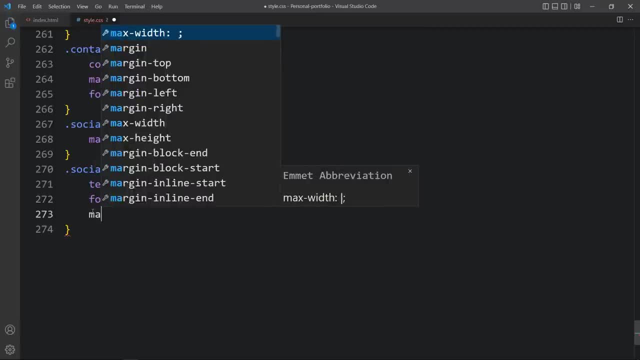 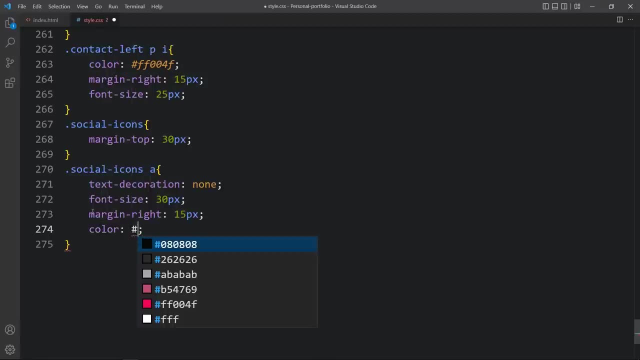 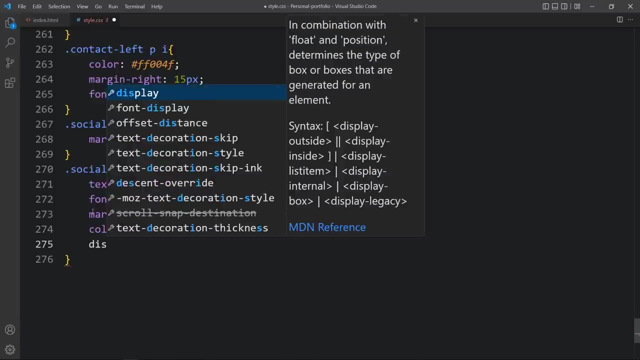 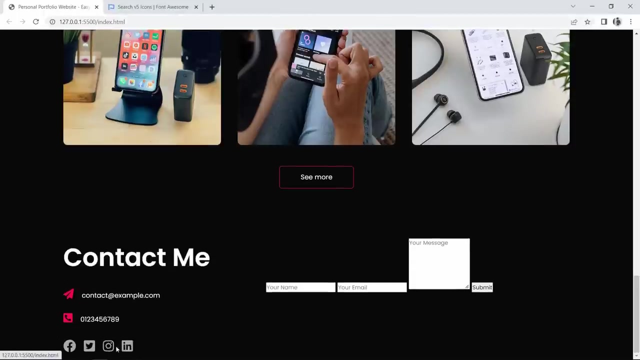 font size: 30 pixel, then margin from the right side it will be 15 pixel, then color, then color color will be this one and after that display display will be inline block. so this social media icons are looking good. next we will add the hover effect on these icons, so 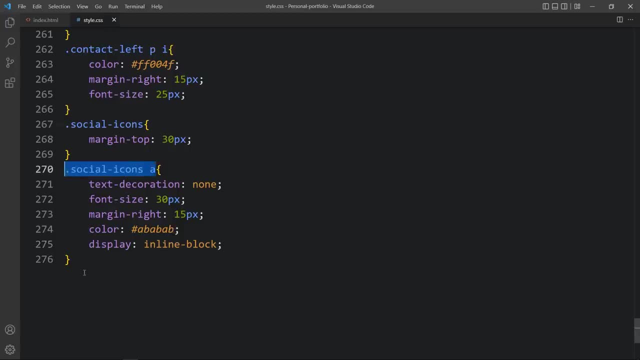 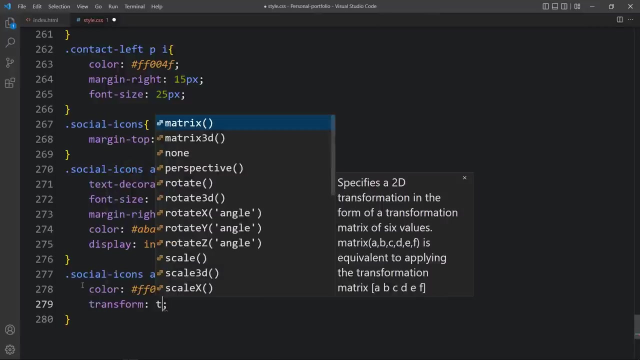 let's come back and copy this one, paste it here, so whenever we will take cursor it should change its color. so first we will add colon hover, then write color. this is the color code. after that we have to move this icon little bit up so we will add transform: translate y minus 5 pixel. so it 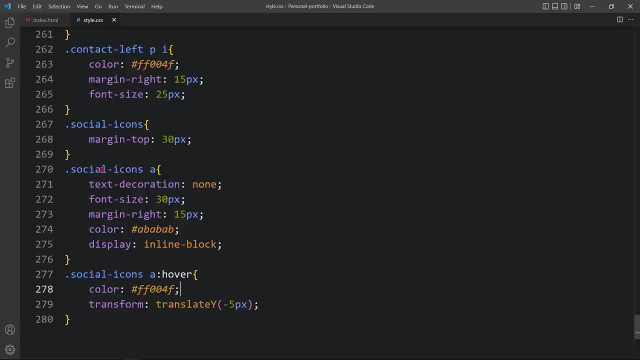 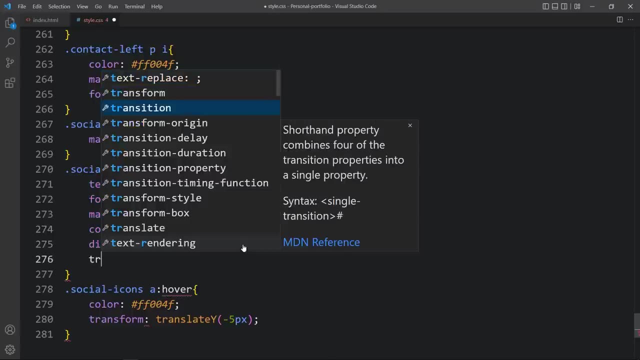 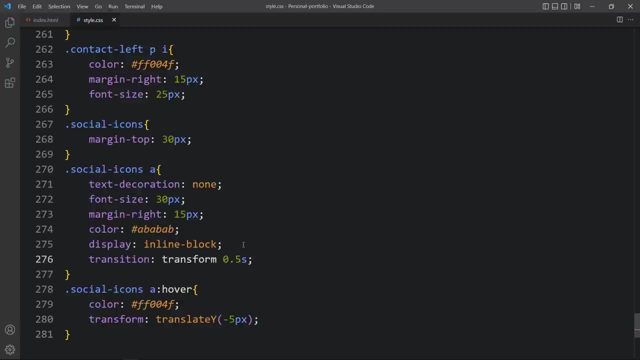 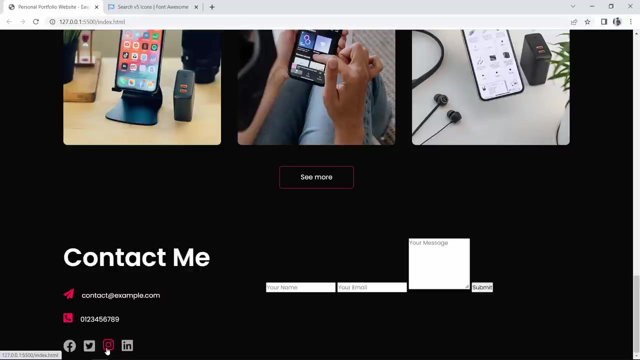 will move the icon up by 5 pixel and in this social icon, a, we will add transform transition transform 0.5 seconds. you can see, if i take cursor, it is moving up and the color is changing. after the social media icon i will add one download button where you can attach any. 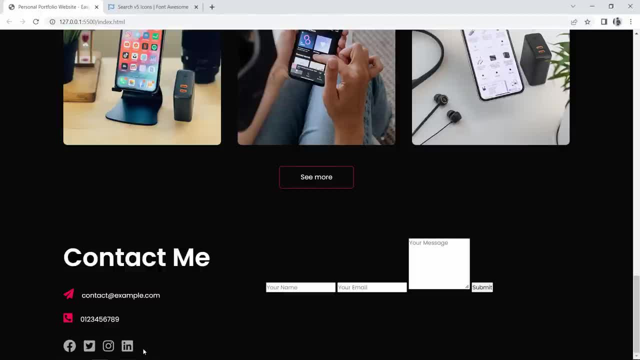 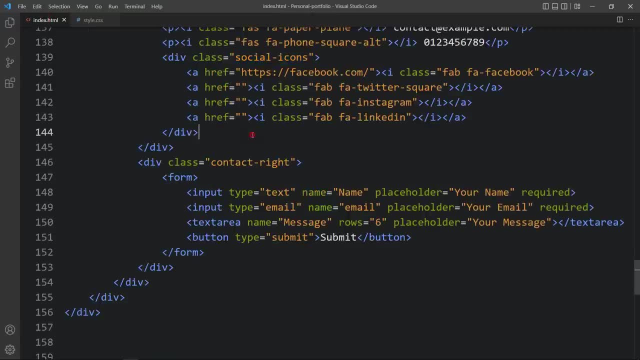 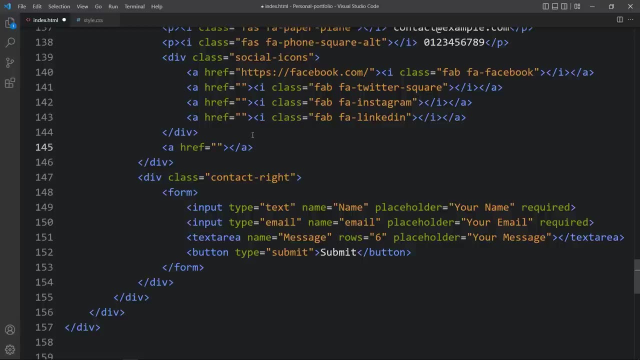 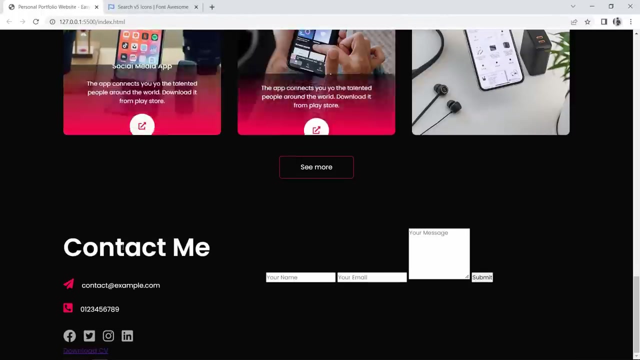 downloadable file, like your cv in pdf file or any other file. so let's come back and in this html file, after closing a this, which is for the social icon, here we will add one, a tag, then write the link text: download cv, so you can see this link here. next we have to decorate it. so let's come back and here we will. 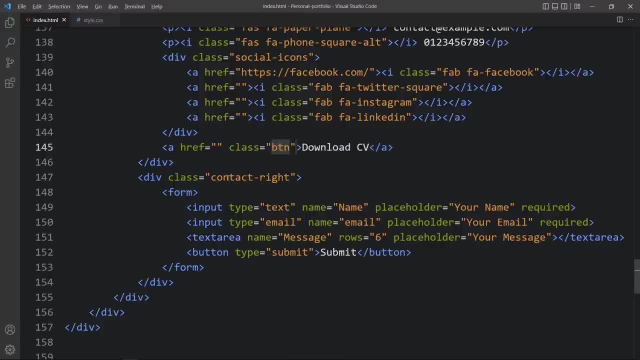 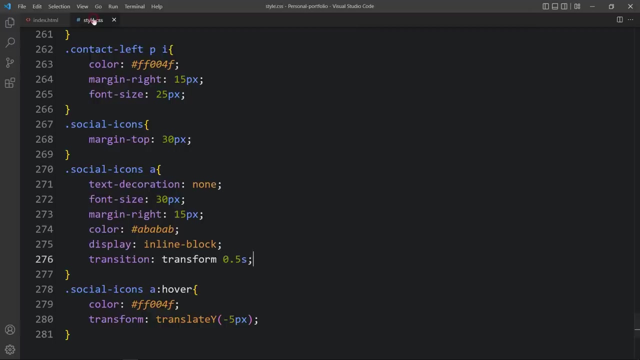 add one class name: btn, so you can see some changes here. now we have to move this button in the left side, so let's come back and we will add one more class name, btn2, like this: next copy this class name: btn2. come back to the css file here. 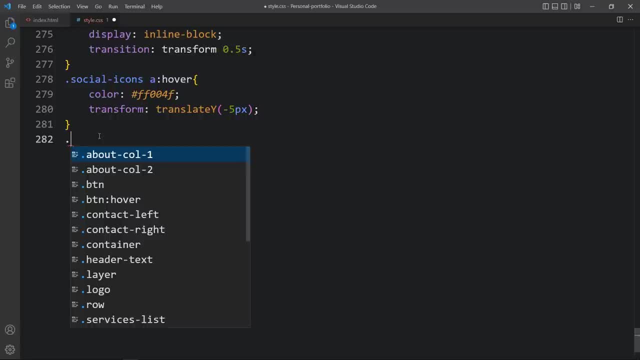 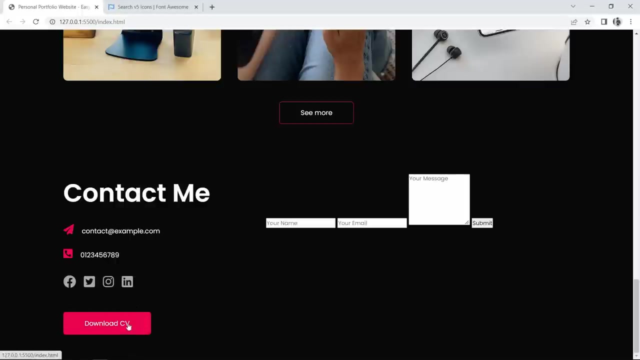 we will add btn. it will be dot btn, dot btn2. there is no space. so here we will add display, inline block and background, this color code so you can see the colored background for this button and you can see this button in the left side. but right now, if i click on this button, nothing will happen. 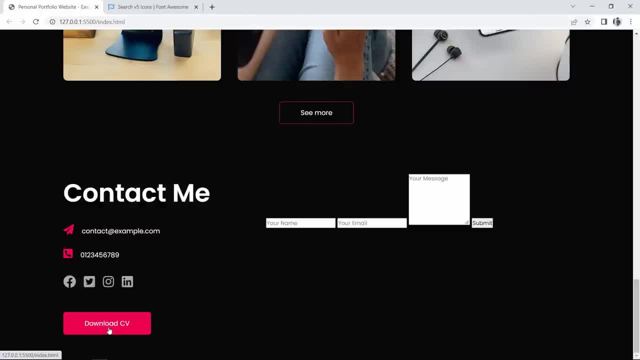 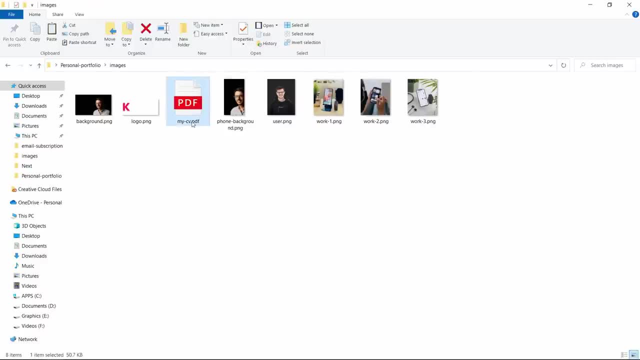 so next we have to attach one downloadable file in this button. for that you need any file that you want to attach in this folder. you can see i have added one file called mycvpdf, so we have to attach this file with the downloadable file. so we have to attach this file with the. 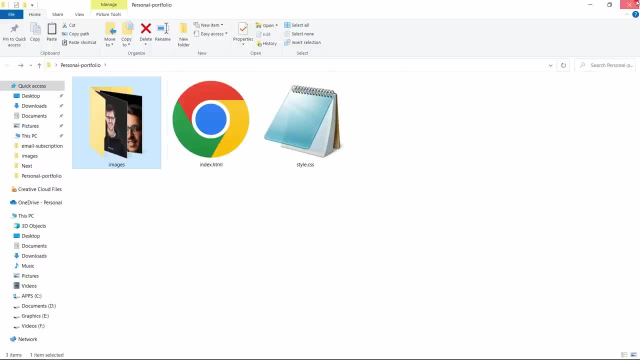 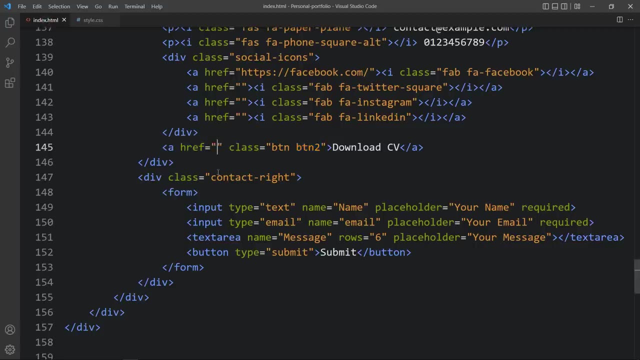 download button. it is in the images folder, so let's come back and in this html file, in this href, we will add the file path: images slash- mycvpdf. then we have to add download. that's it. so whenever we will click on this button, it will start downloading this attached. 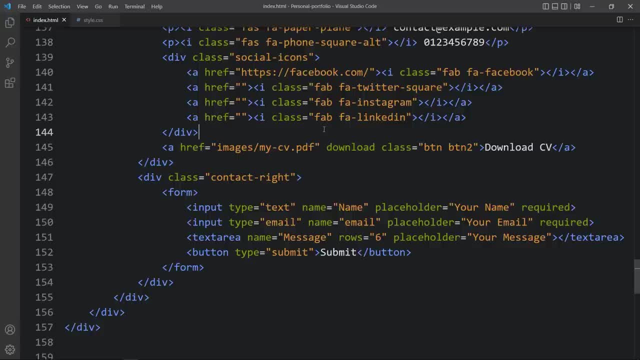 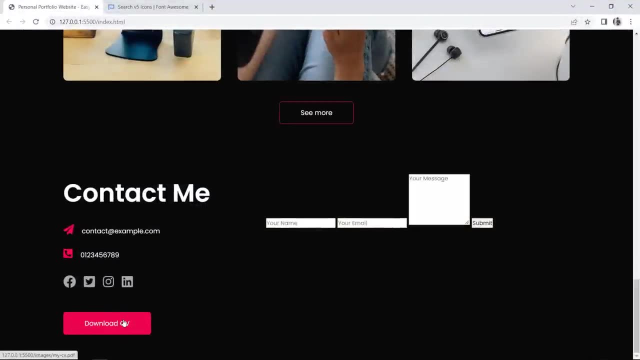 file in the browser. so let's come back to the website and you can see, if i click here on this button download cv, it will start downloading one file, which is mycvpdf. it has been downloaded, so this is how you can attach any downloadable file in this button. so after adding this button, 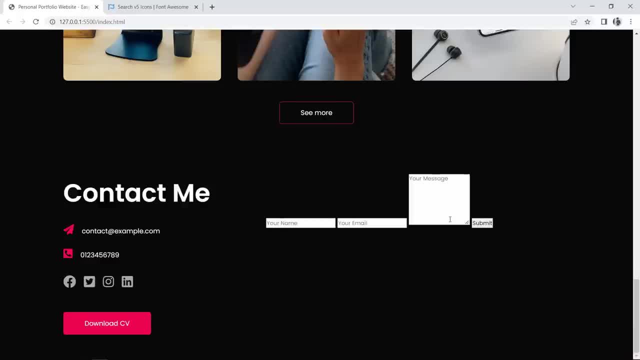 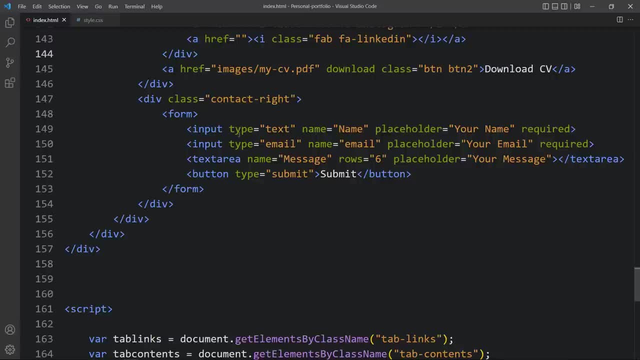 we will design this contact form which is in the right side. so let me come back and you can see we have added the form tag here and in this form we have added 3 input fields and one submit button. and in this button we will add one class name called btn and one. 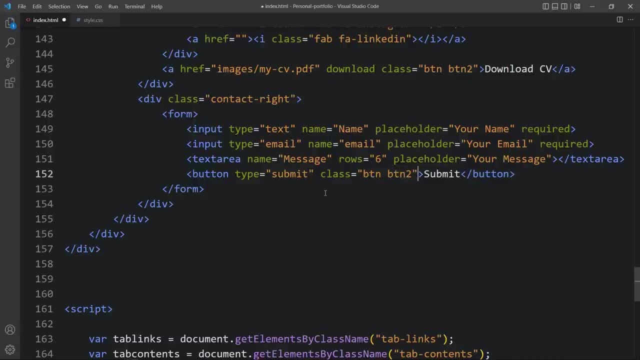 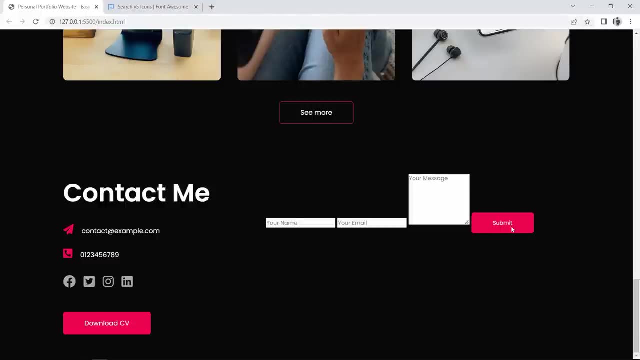 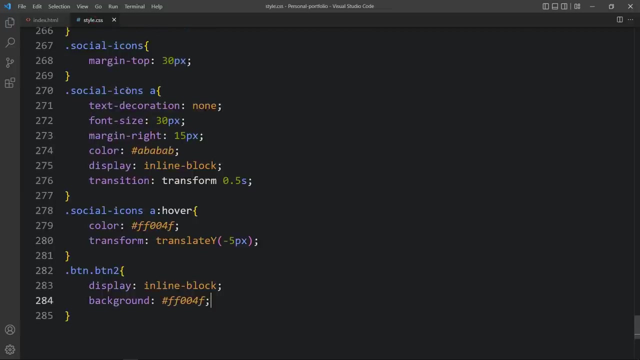 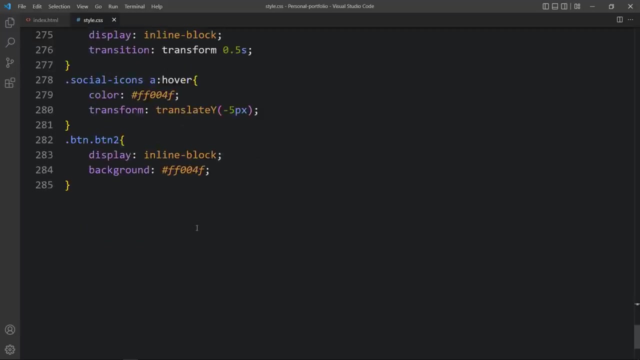 more class name: btn2. after adding this class name, you can see the submit button is also looking good. next… we will come back and and come to the css file. here we will add the second column class name, which is for the contact. write, copy this one, then write form. so for this form we will add the width. 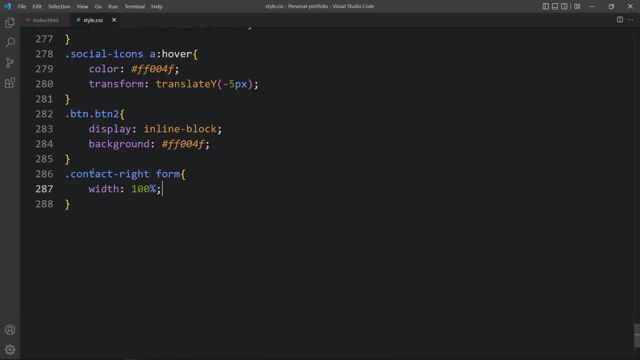 width will be 100%. now we will add form input because we have added input tag. lets add comma and write form textarea, textarea. so for this input and textarea we will add the css. so first we will add the width, width will be 100%, then border, border will be 0, then outline none. 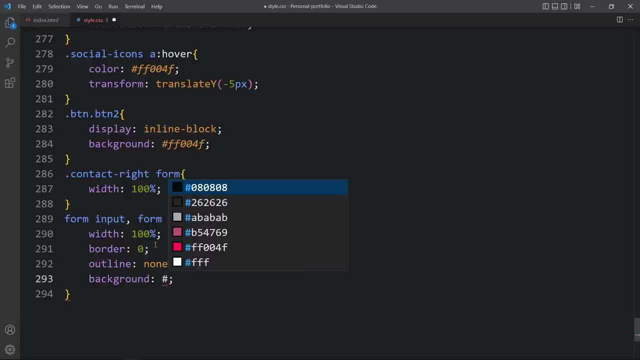 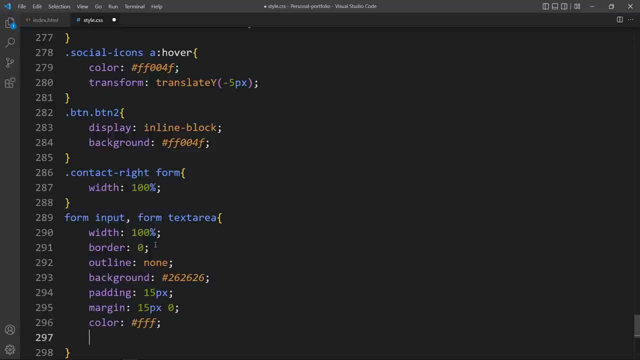 then background, then border radius. here we will add one color code. lets add space inside this input field. so we will add padding of15px, then some margin. some margin will be from top and bottom. then we will add color. it will be the text color. here will be written inside this input field. then we will add the. font size it will be 18px and border radius will be 16px. then we will add the Css co load what color we are all ready. then we will add the css co load the applying language to this을, and we come to final part of this class. here we 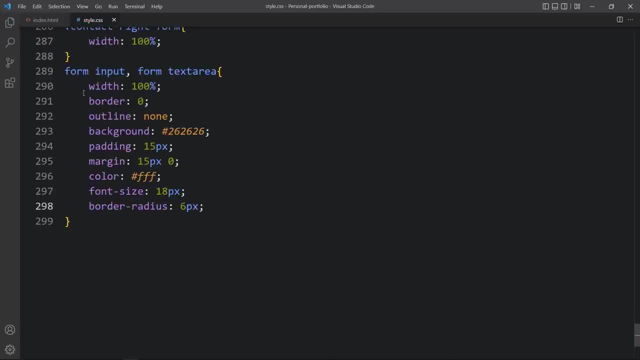 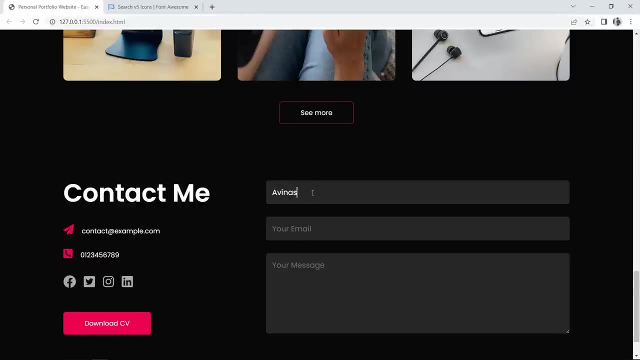 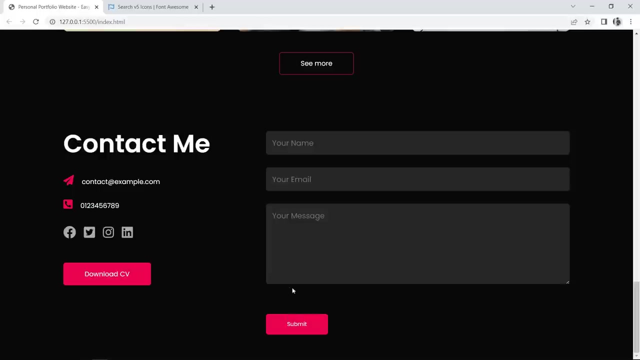 6 pixel. after adding this for the input fields, you can see this input field looks good. we can write anything, we can type any message in these input fields: your name, your email and your message. now we will change the size for this button and we will reduce this space which is between the input box and the 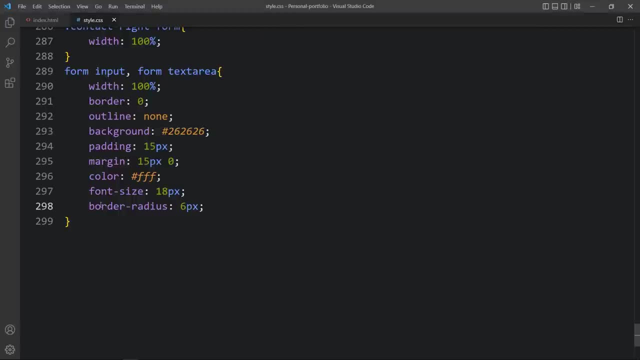 submit button and we will add cursor pointer. so let's come back, and here we will add form btn2. so for the btn2 we will add another padding. it will be 14 pixel and 60 pixel, so the width will be large, and then we will add the font size. 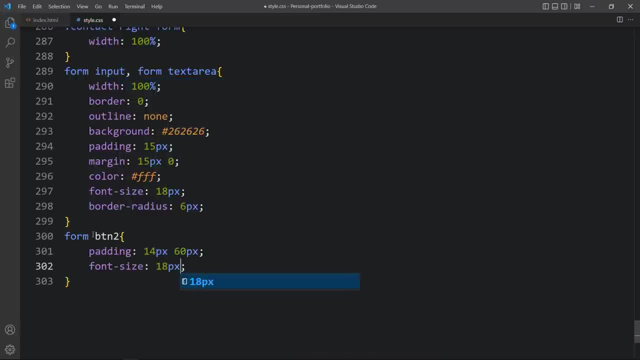 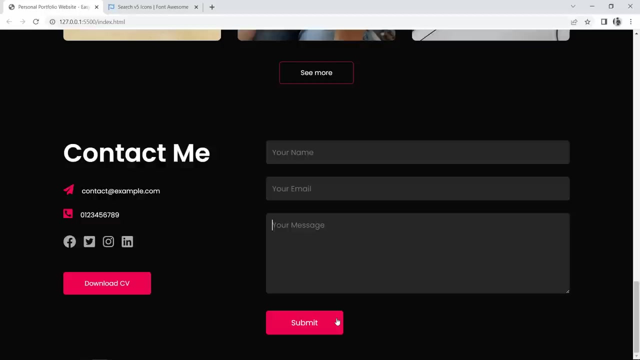 it will be 18 pixel, then margin from the top it will be 20 pixel and then we will add cursor pointer here. we will add dot btn form- dot btn2. now you can see this submit button is also looking good. if i click here it is saying: please fill out this form because 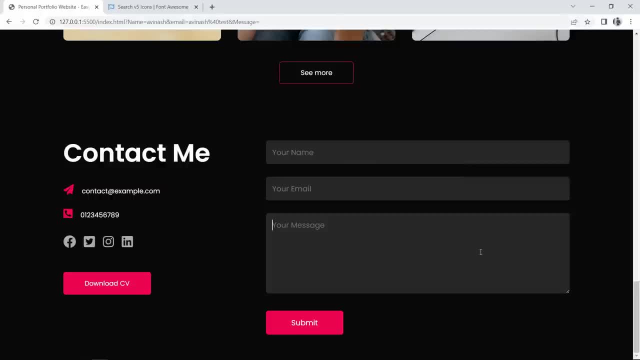 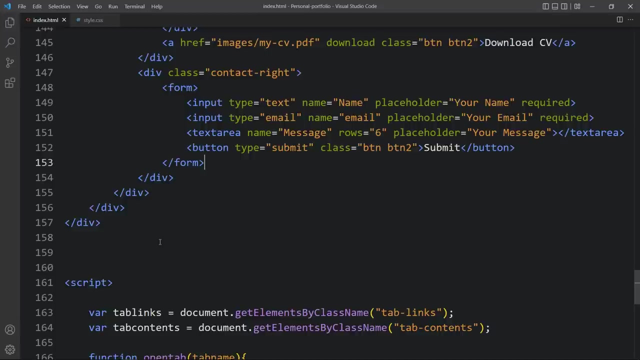 it is required after completing this website. i will teach you how to connect this form with the google sheet, where you can receive the contact form inquiries on your google sheet. so for now, we will create the bottom section, which is for the copyright section. so let's come back and come to the html file just above this closing div. it is here. so 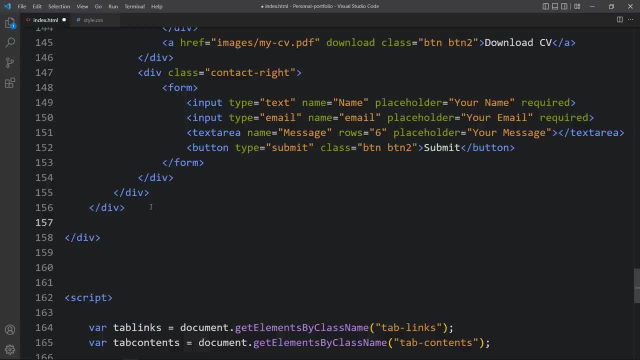 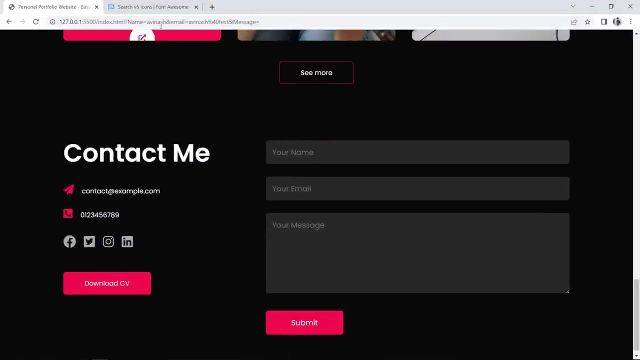 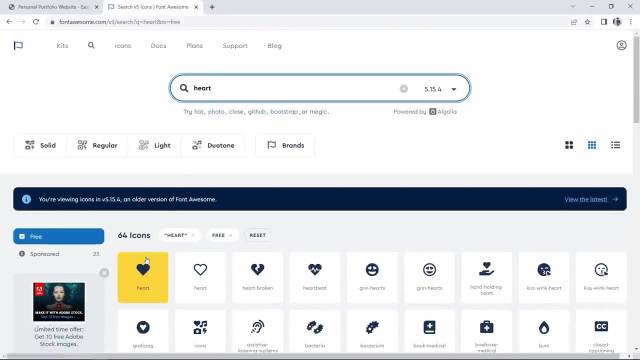 here we will add another div with the class name copyright. in this one we will add the text in p tag. so this is the text. in this one we will add one heart icon also. so come back to the second website. here we will search for heart, click here, copy this one, then paste it here. 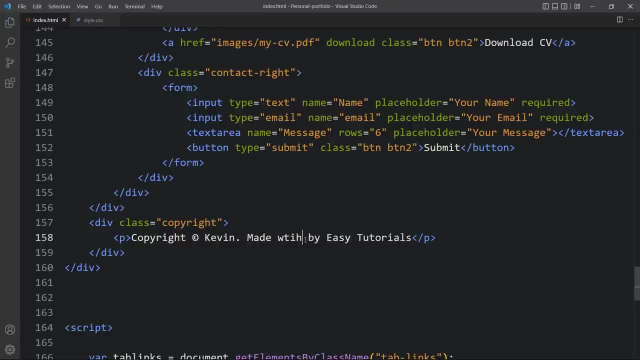 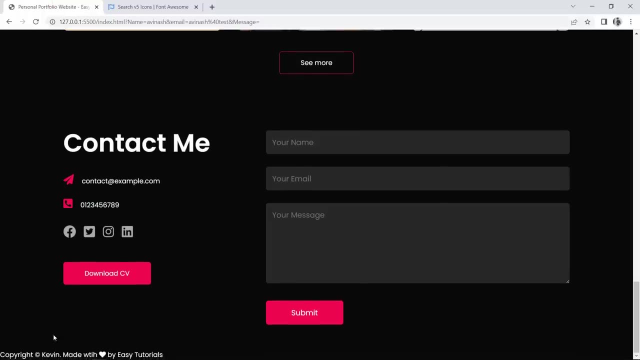 after adding this again, refresh the website. here. you can see this message at the bottom. next we have to change its position. it will be in the center and we will add the background color also. so lets come back and fill it out. and here we have. itůI created the background. we will charity. it is attached to the last. 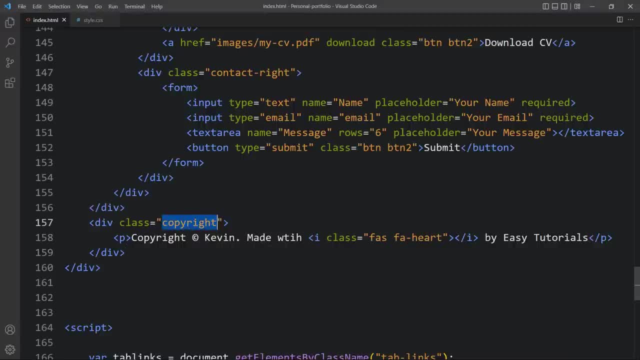 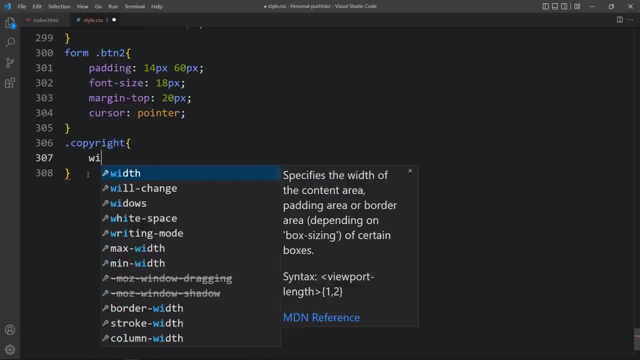 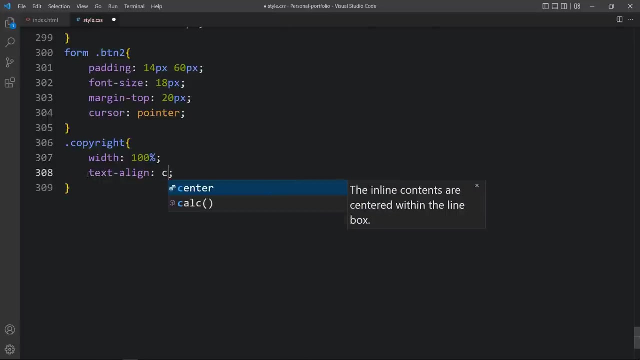 and copy this class name copyright and write it here in this css file: copyright. in this one we will add the width. width will be 100%, then text align will be center, some padding and background, font weight will be 300 and summer space from the top margin: top will. 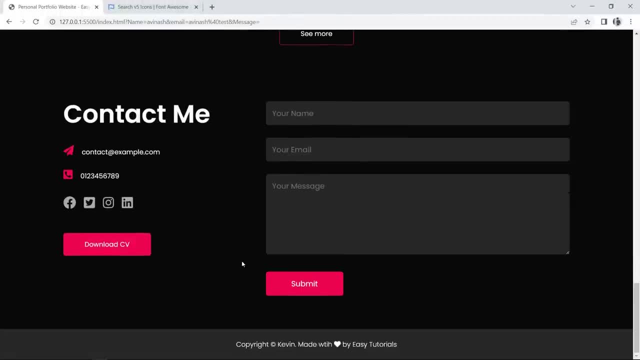 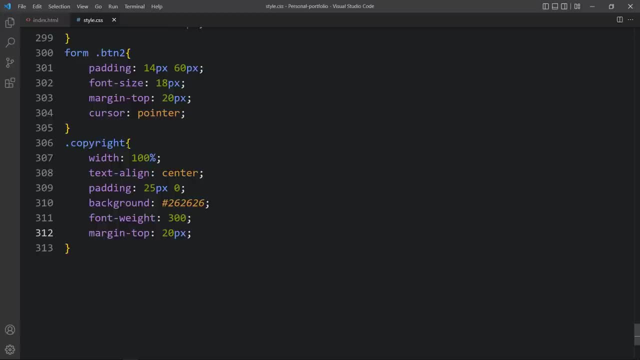 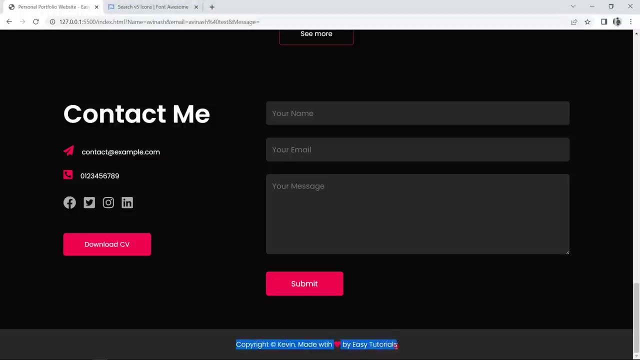 be 20px. you can see this bottom copyright area is looking good. next we have to change the color of this heart icon. so lets come back and copy this one copyright, then write itag for the icon. here we will add the color. thats it. you can see color in this heart icon. so we have added all the contents on. 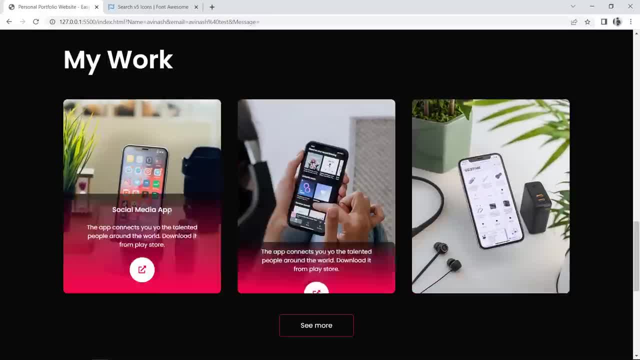 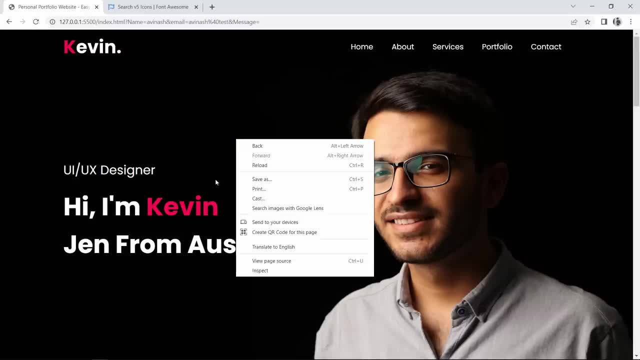 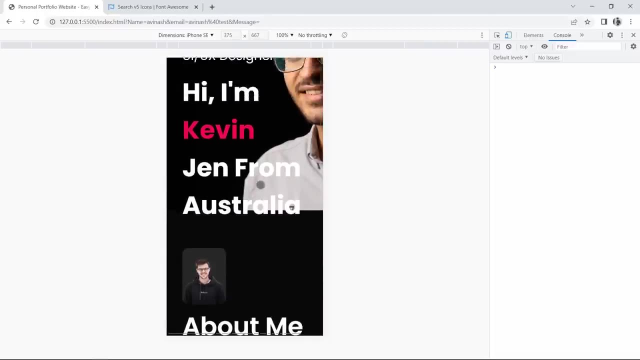 this website and you can see this hover effect is working fine. next we have to check this website on a smaller screen and lets see how it looks. if i change the screen size, you can see the header part is not looking good. then this image is very small. these text are large. 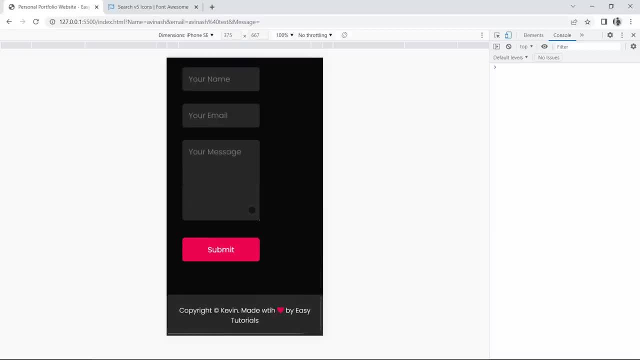 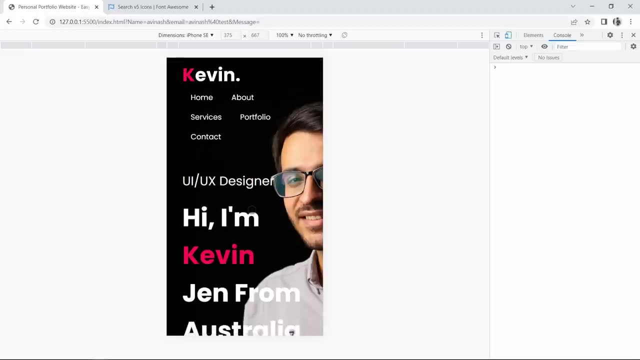 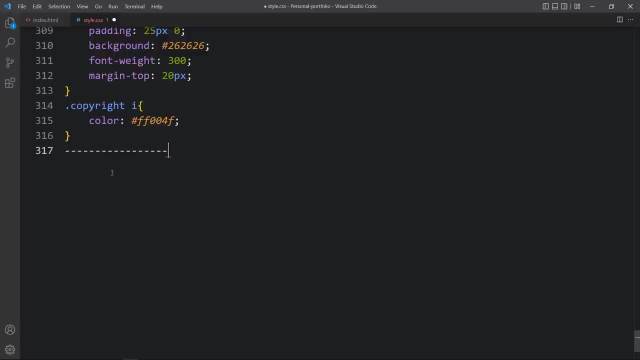 here at the rate media only screen and max width: 600px. now we will add the css properties within this one. so whatever css properties we will add here that will be applicable for the small screens. the screen width will be minimum 0 or maximum 600px. so lets come to the website. 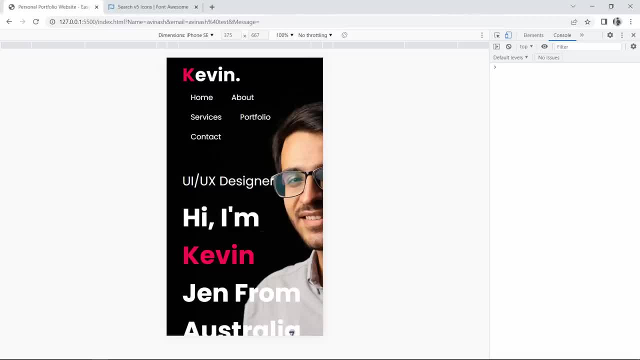 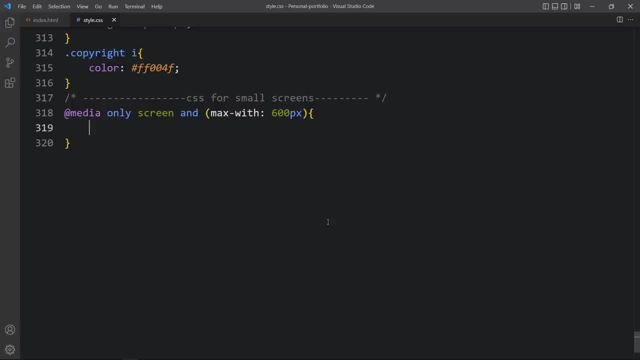 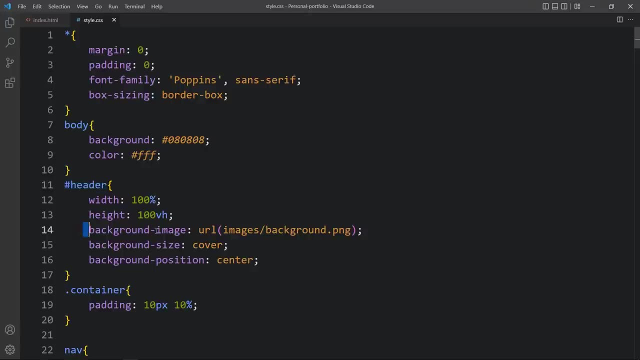 and here you can see, we have the image in the background, which is not in the perfect position, so we have to replace this image with the another one. so lets come back to the css file. here you can see we have added the image in this header and background image. 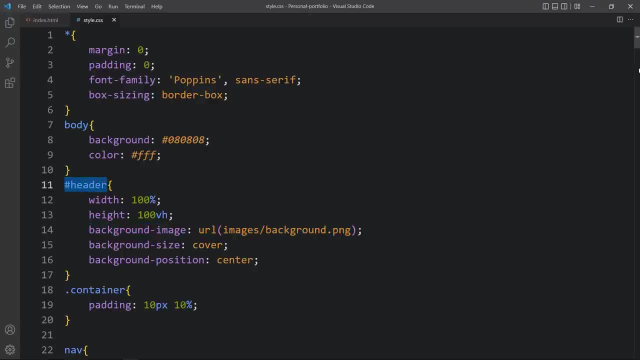 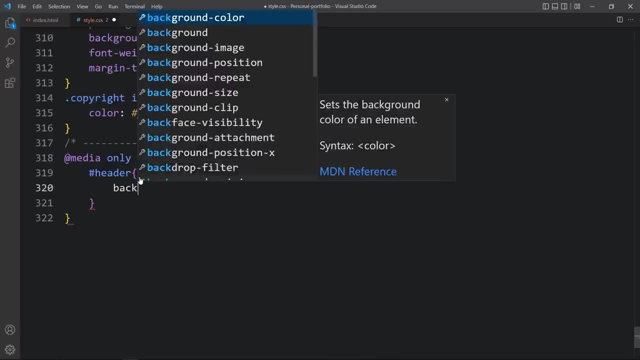 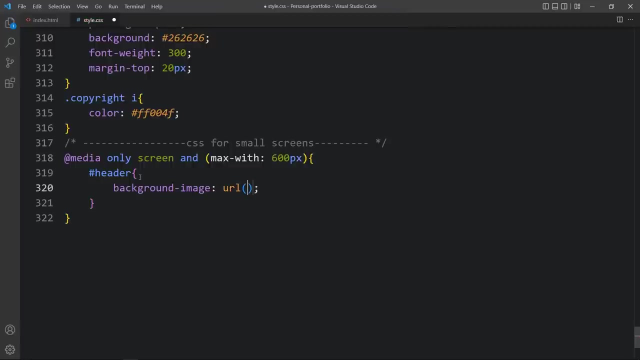 so we have to replace this one. so lets copy header header, header. write it here in this media query: dot header: background image url. and in this url we will add the another image file path. so in this folder you can see i have another image. 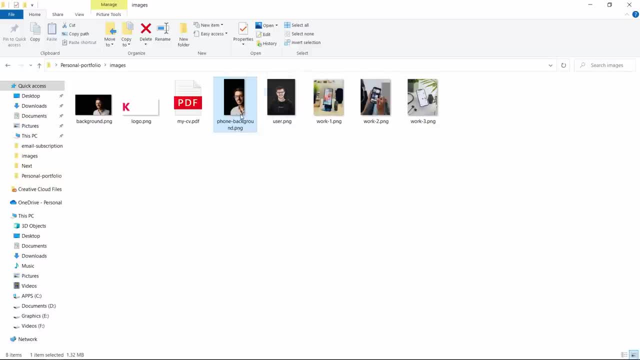 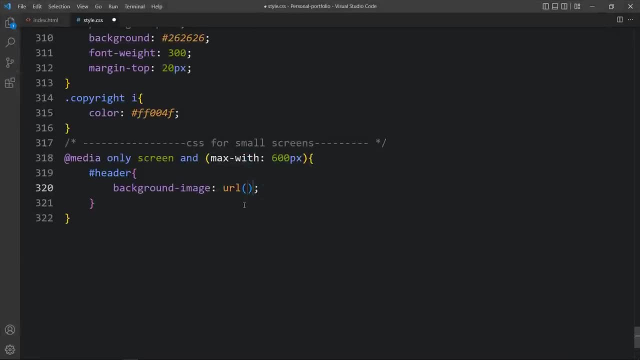 which is phone background dot png. so we will use this image: phone background dot png. copy this one, add it here. images slash- phone background dot png. after adding this, let's come back to the web page. this image is still same, so let's come back. yes, here we have to correct this one. w i d t h width. 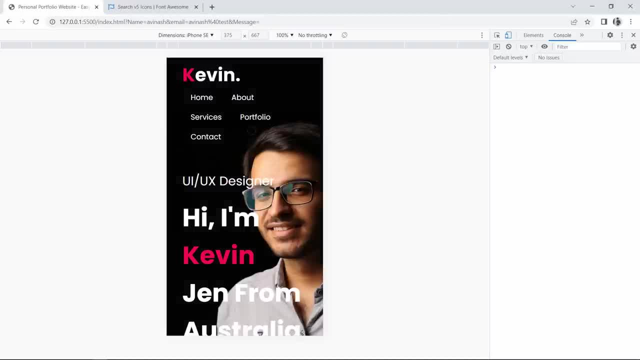 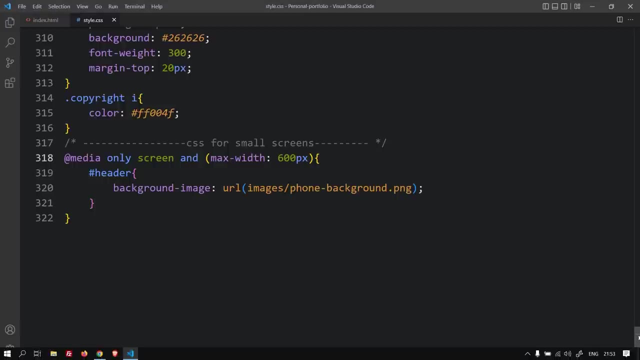 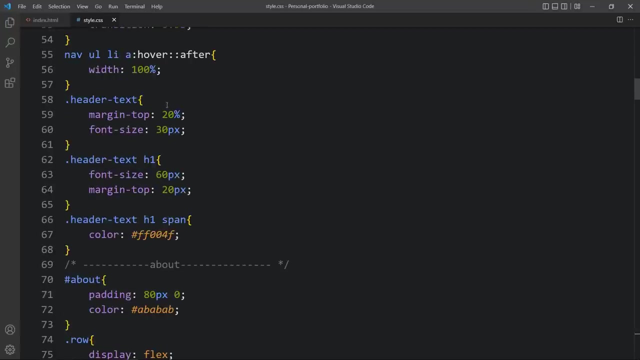 max width: 600 pixel. after that you can see this image has been changed. now it is in good position. next, we will decrease the font size for this text, which is ui ux designer and this main title. so let's come back and you can see we have added the titles in this one, which is header text and header text h1, so we have to replace 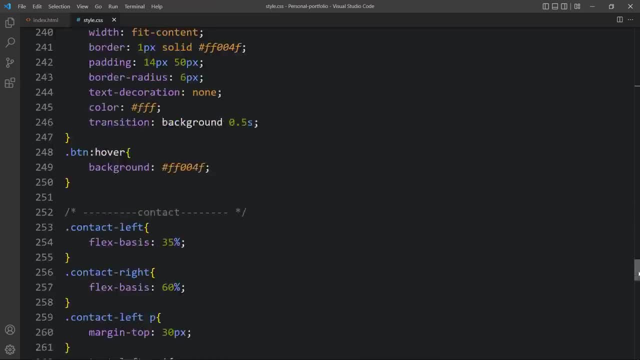 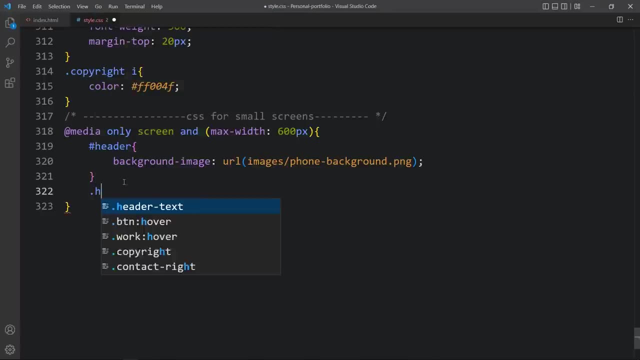 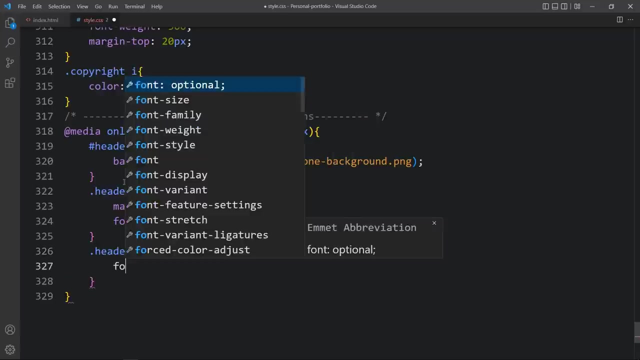 these font size. let's come back to the bottom, where we have added media query and in this one we will add dot header text. here we will add margin, top 100 and font size. let's add small font size, which is 16 pixel. again write edit text and h1 for the main title. here we will decrease the font size. it will be only 30 pixel. 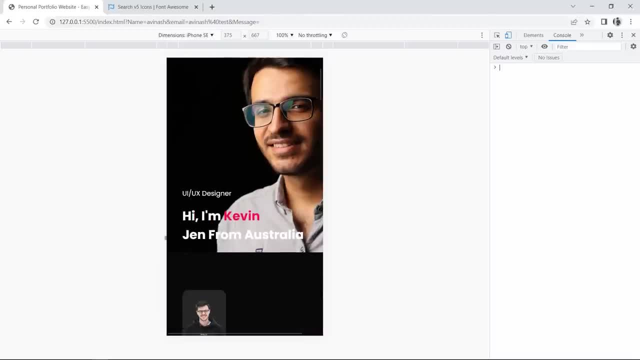 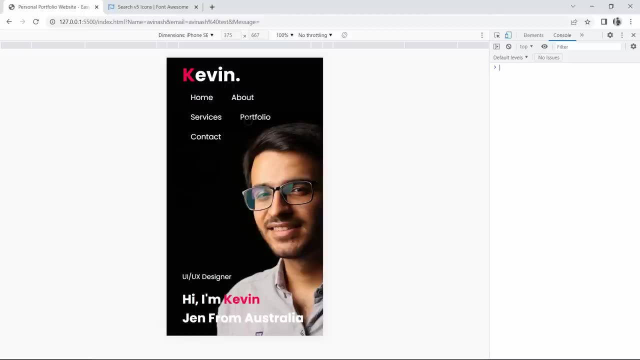 so you can see this text over here. it will move up whenever we will fix this navigation bar. in this navigation bar you can see this menu is visible by default, so we have to hide this one and it will be visible whenever we will click on any menu icon. so first we have 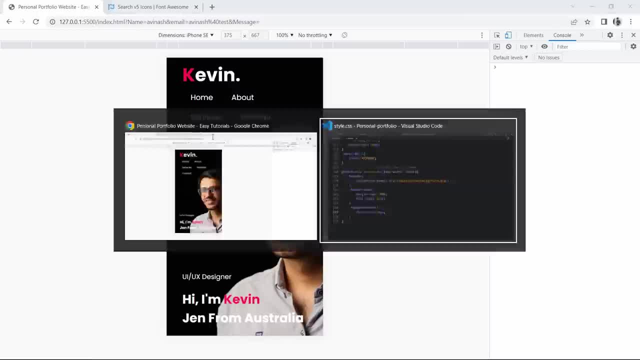 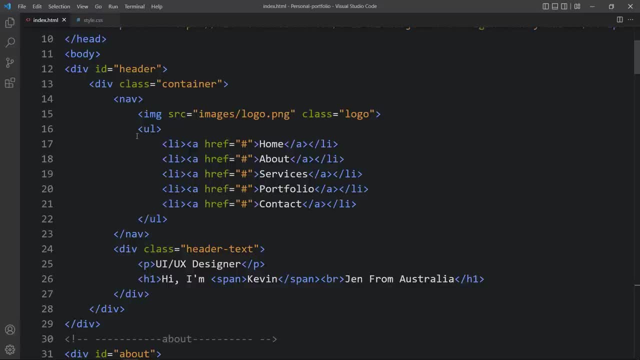 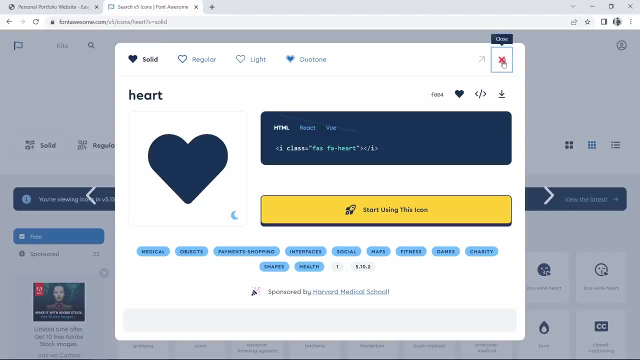 to add one menu icon here. so lets come back, come to the html file, come to the top, where we have added the menu links. it is here. so here we have to add icons. so lets come back to the website, which is fontawesome, and here we will search for menu icon. so lets add menu. 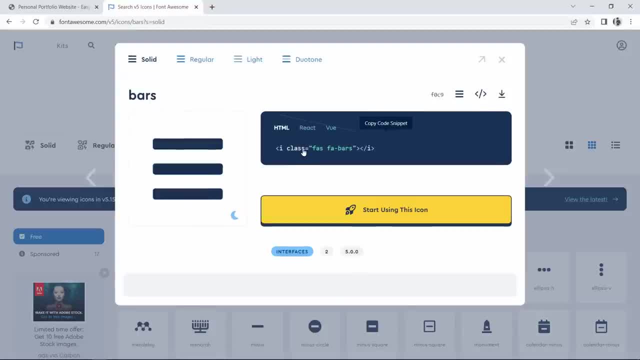 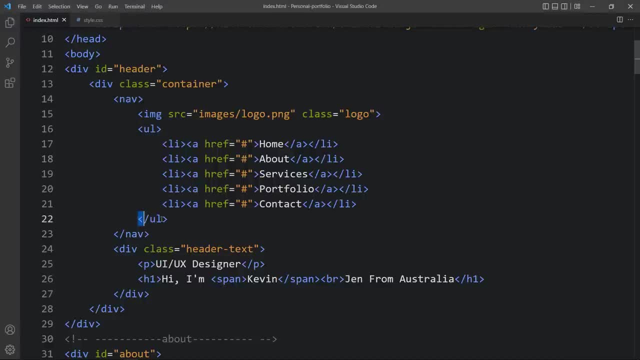 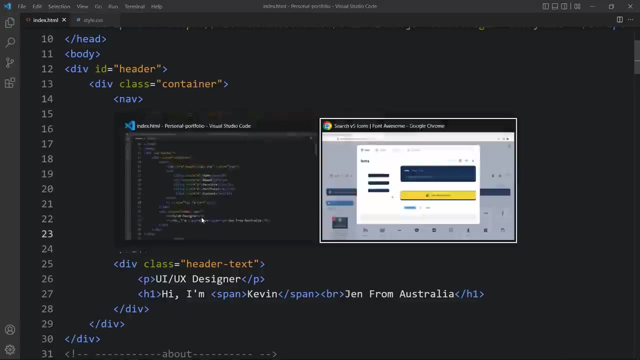 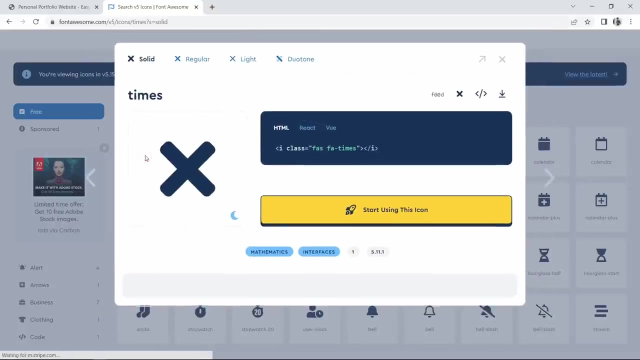 click here. copy this one. so it is for the menu icon. come back to the html file and we will add it here just after this closing ul tag. paste it here. next we will add one close icon. so here again, search for another icon. i will add times. click here and click to copy this one, then add it. 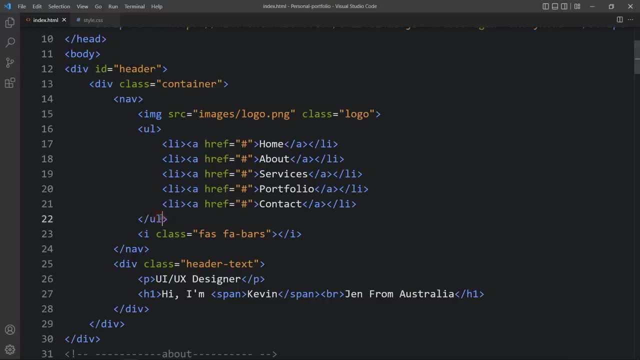 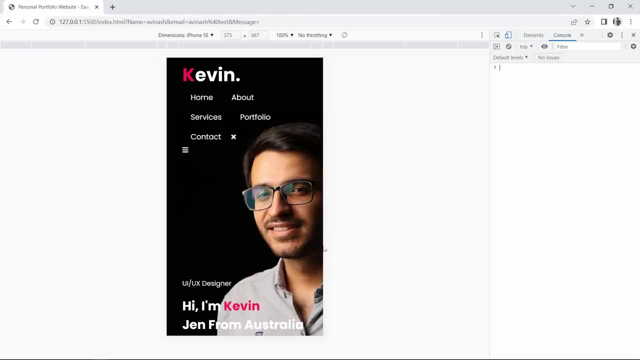 here, just above this closing ul tag, add a space and add it here. so we have added one cross icon and one menu icon. let's see, on this web page you can see this menu icon and this cross icon. let me open this web page in full screen. here also you can see this. 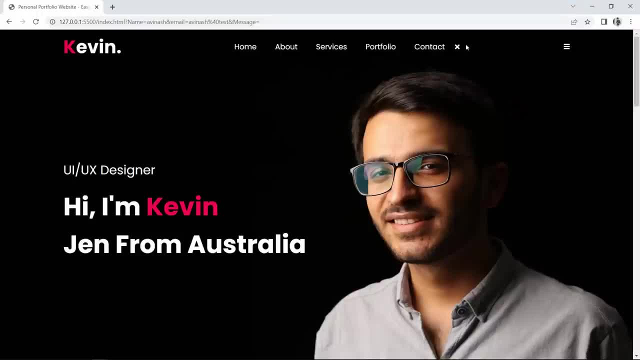 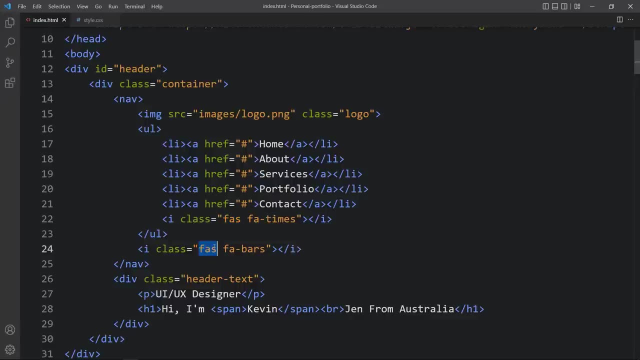 cross icon and this menu icon. so we have to hide these icons by default and it will be visible whenever we will open this web page in a smaller screen. to hide this one, let's come back and here you can see we have these icons with the class name FAS, FAS. so here 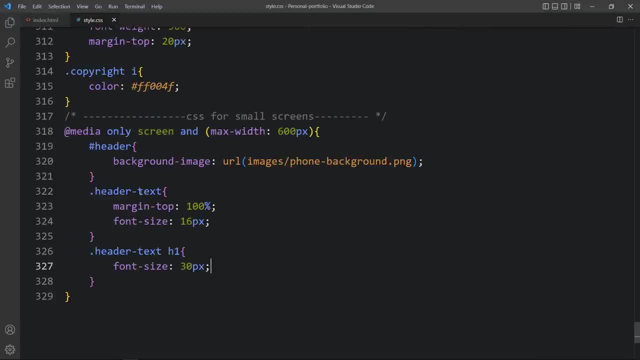 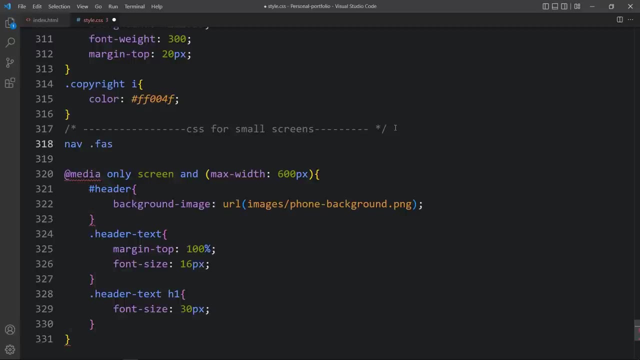 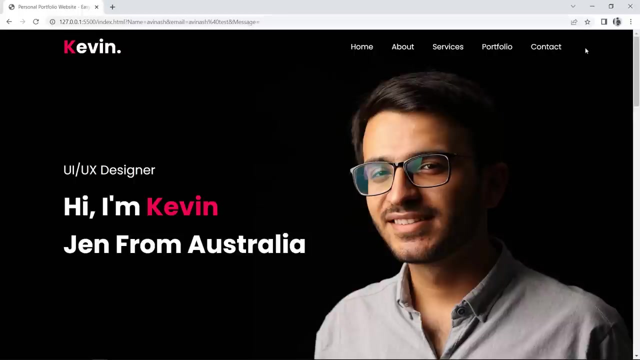 let's come back to the css file. just outside of this media query we will add a space and here we will add navfas for the icon display. none, so it will be hidden. you can see these icons are hidden, and if i open this web page in a smaller screen still, it is hidden. so 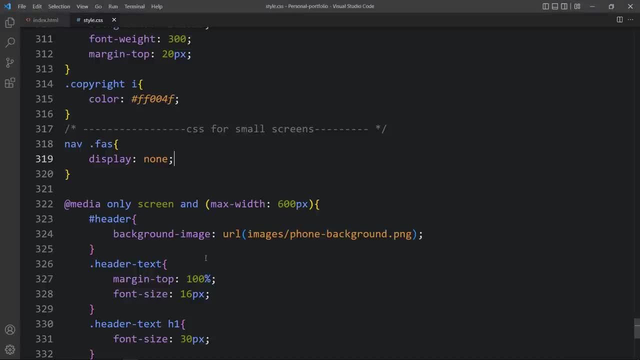 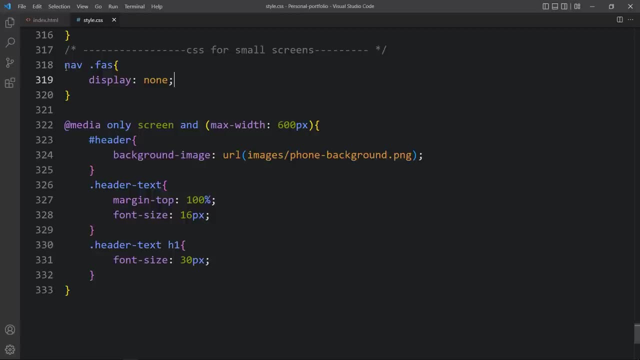 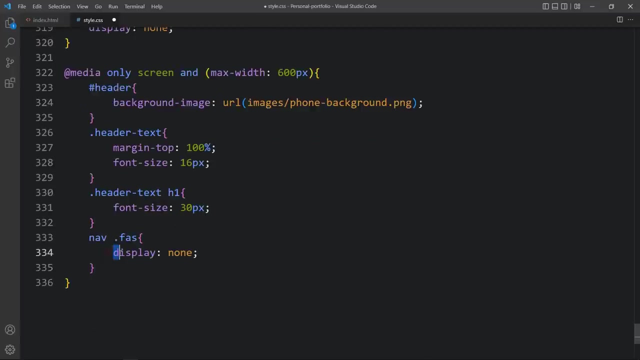 we have to display these icons on a smaller screen. so let's come back and in this media query again, we will add the same thing, navfas, in this media query, and we will add display block, so it will be visible. and we have to change the font size also, so we will add font. 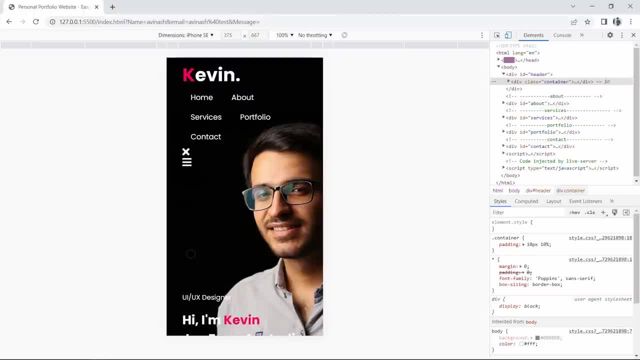 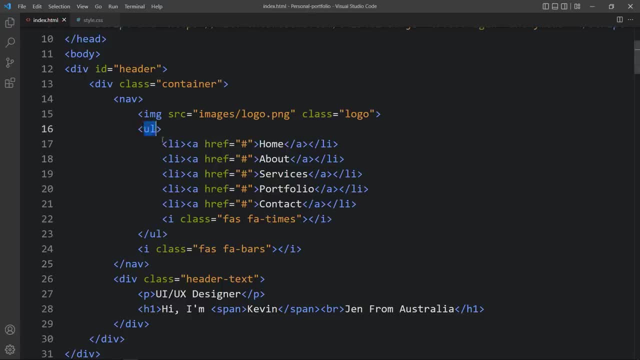 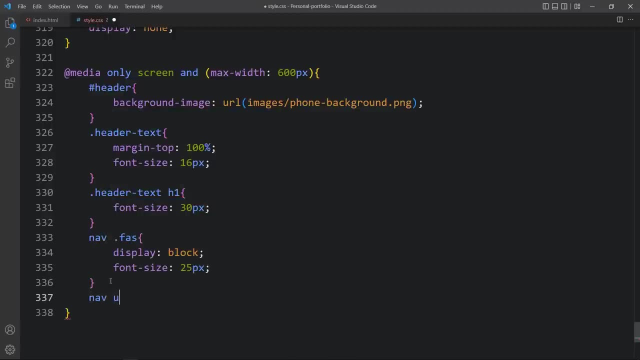 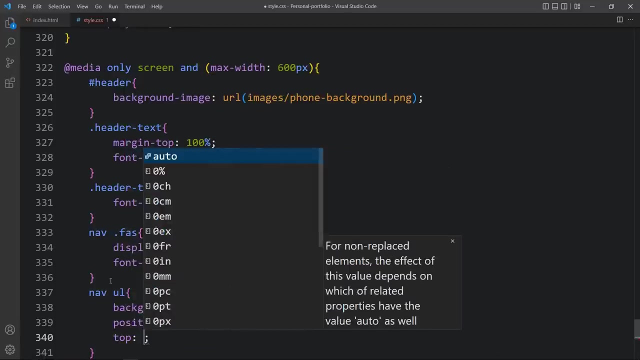 back. you can see we have these menu with this ul and li tag. so come back to the css. in this media query we will add nav ul- background. let's add this color code in the background. then position position will be fixed top zero and background position will be fixed top zero and. 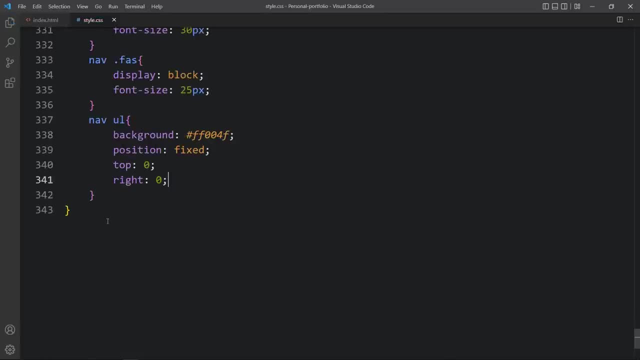 then position. position will be fixed: top zero and right zero, right zero. then we will add the width. width will be 200 pixel and height 100 vh. padding from top: it will be 50 pixels, so there will be some space on top. now you can see this side navigation menu. 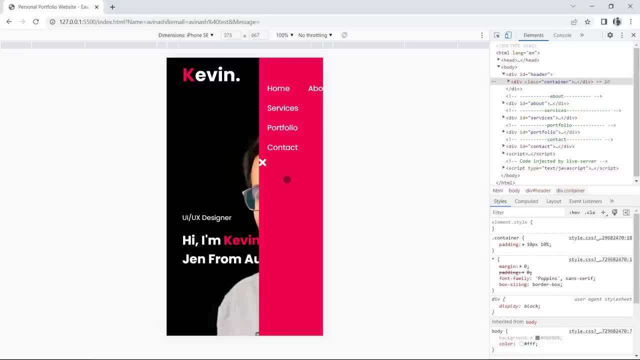 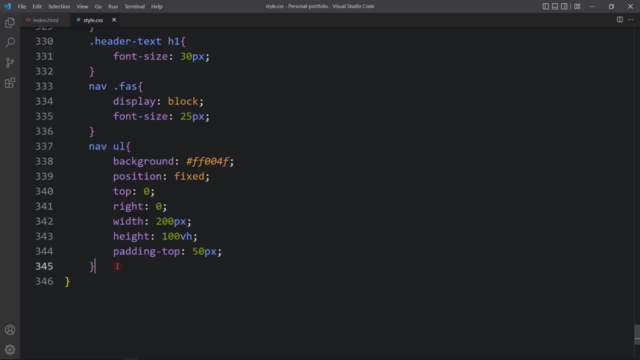 now you can see this side navigation map. you can see this side navigation and this side navigation is available also as the banner looks not good, but it will be compared there. all the pixels here are all time, all time. on this page. we have these menu all key with 0, 1, 0 p icatxr slo. 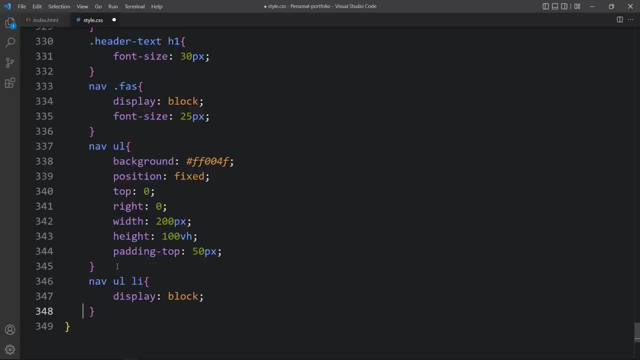 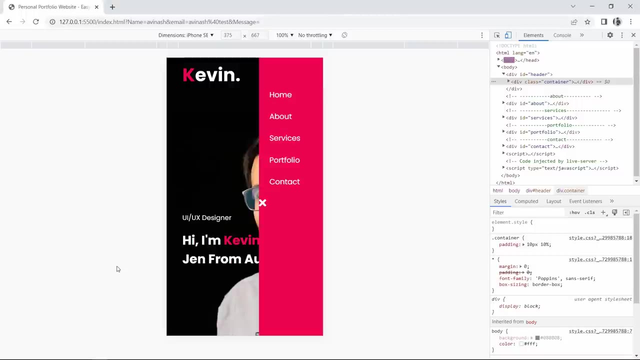 and we will look under our eyes and click on. go to the menu on this part. values on these list you can see here. let's name these. enter hundred and first. people without entering a storm color tip law are arranged vertically. next we have to set position for this cross icon. so let's come. 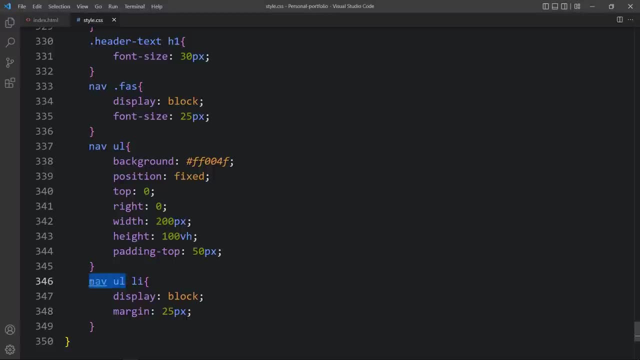 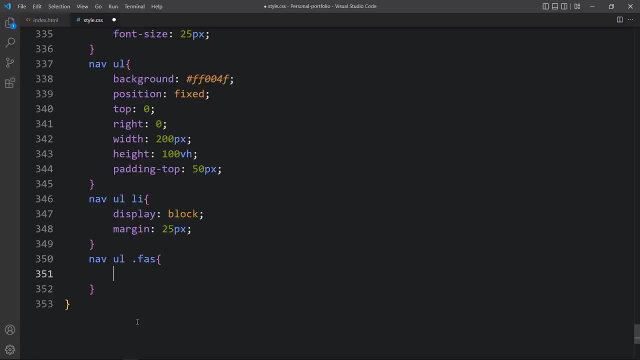 back. here we will add nav ul and in this ul we have the icon with the fas class name. so here we will add position. position will be absolute. then we will add top, it will be at 25 pixel and left 25 pixel, then cursor it will be pointer. after adding this, you can. 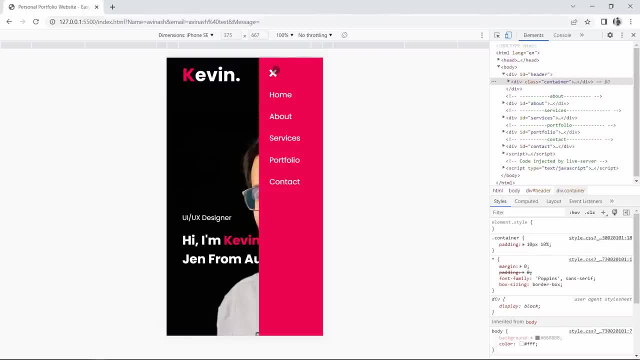 see this icon here. now we have to add the click feature on this icon. whenever we will click here, this side menu will be hidden, and when we will click on the menu icon, this side menu will be displayed. right now, this menu is visible by default if i refresh the website. 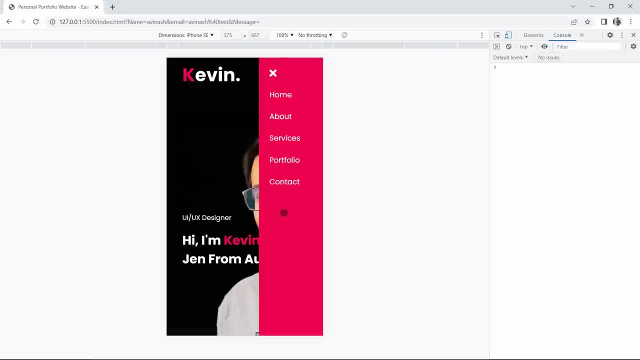 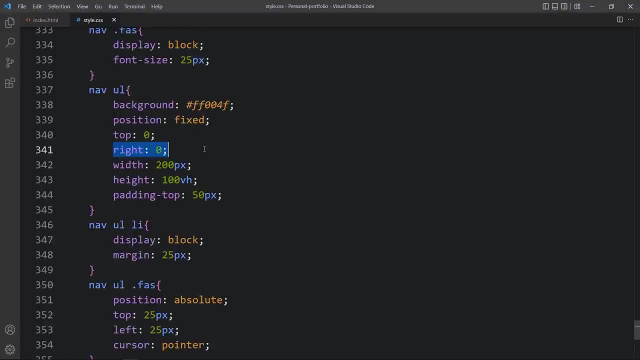 you can see, this side menu is visible, so by default we have to hide this side menu for that. let's come back. and here we have added right zero. so instead of this right zero, we will add right minus 200 pixel. why i am adding minus 200? because the width is 200, so it will move. 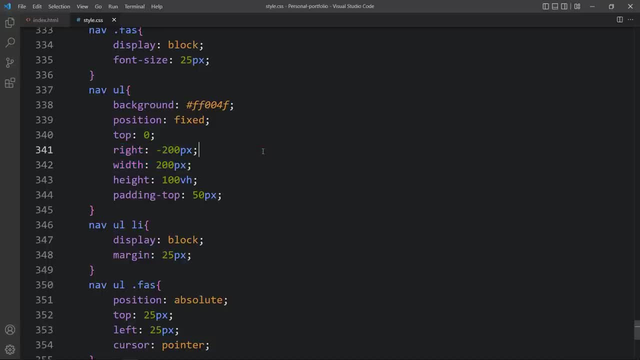 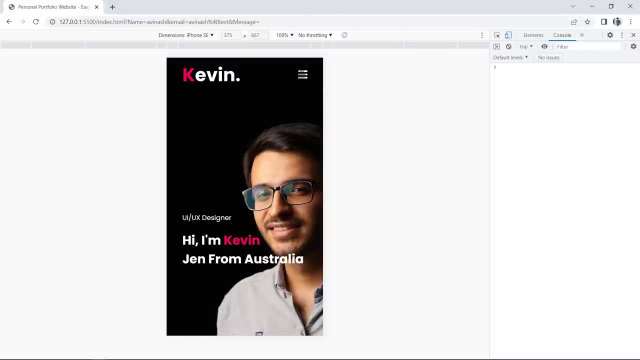 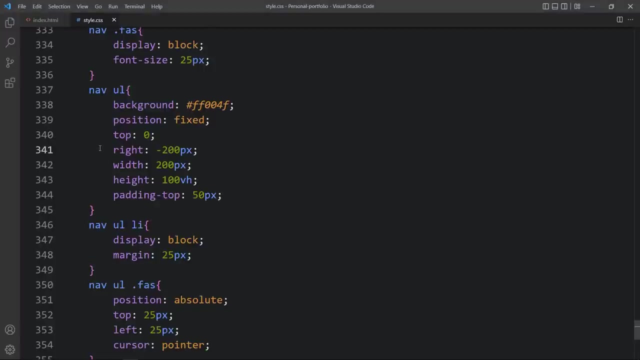 on the right side by 200 pixel and it will become hidden. so you can see this side navigation bar is hidden and we have added the menu icon. if i click here, this menu icon is not working right now because we have to add the click functionality using javascript, so let me come back here in this ul we will 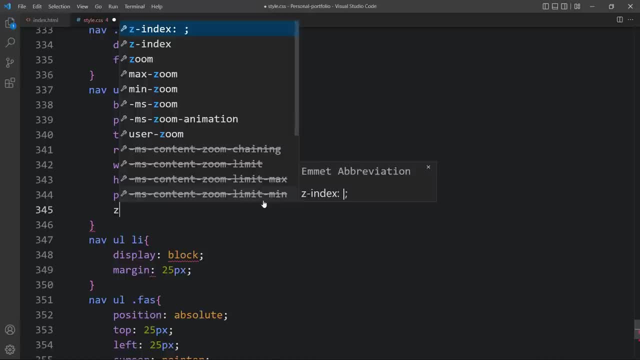 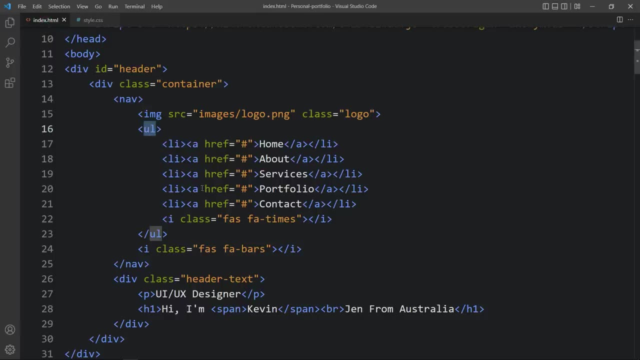 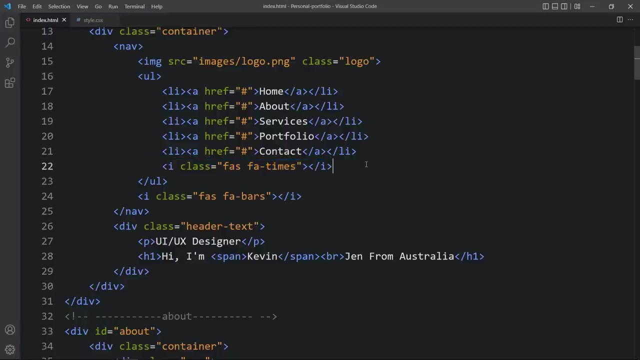 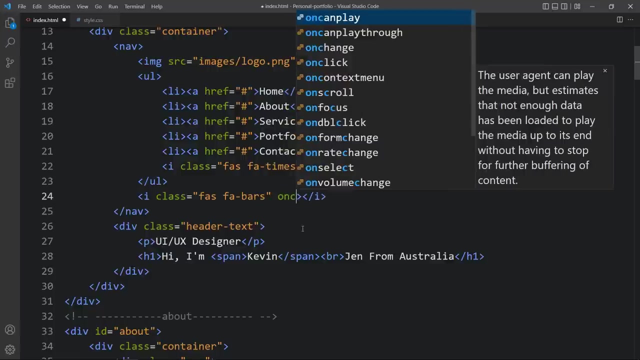 add one more thing, which is zindex 2. so let's come back to the html file and we will add in this icon, which is for the cross icon and menu icon. we will add two functions. so let's add on click on click equal to close menu, so it will close the menu, and in this icon we will add on click equal to open. 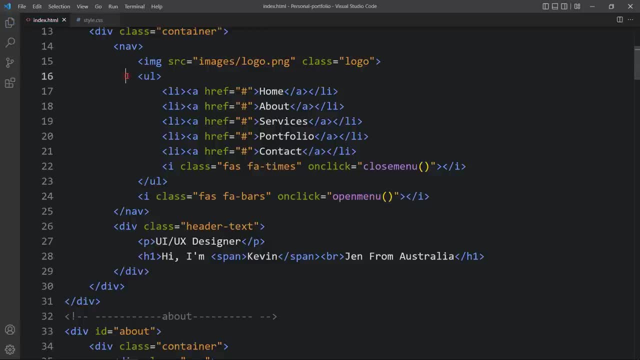 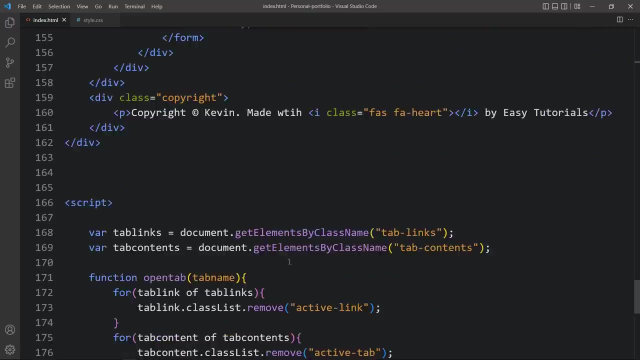 menu. so it will open the menu. in this ul we have to add one id, so we will add the id. so add the id called side menu like this: after adding this id, this on click close menu and on click open menu, let's come back at the bottom and here we will add the javascript. 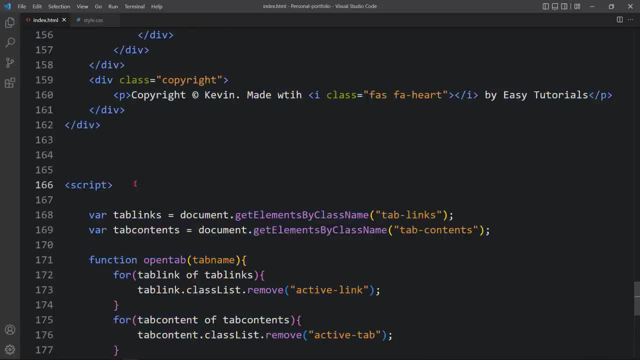 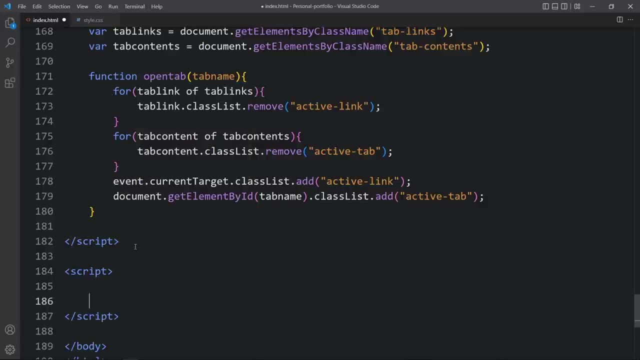 so we have added one script here we can add in the same script type but i will add it separately. i will add script and in this one we will add variable for the side menu. here we will add side menu equal to document dot. get element by id and write the id that we have just added, which is here. 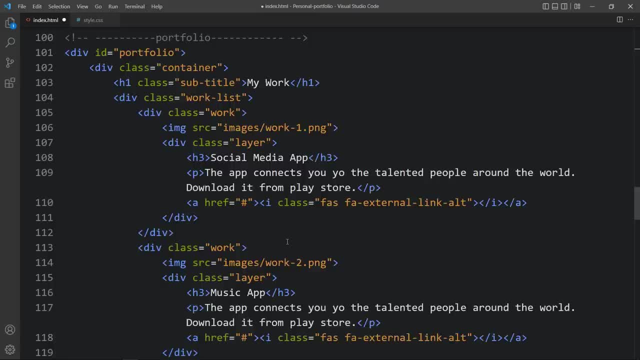 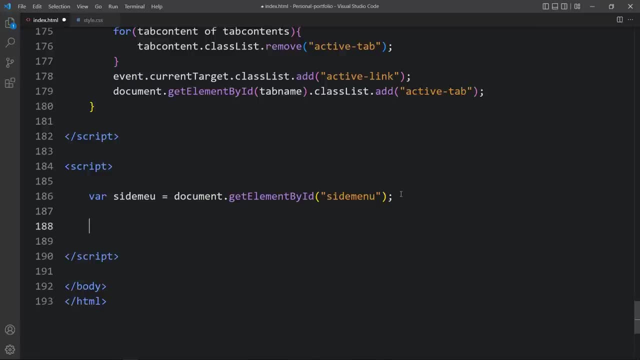 side menu, copy this one and add it here. after that we have to add the functions that we have added in the icons. so here we will add function open menu: define this function. so whenever we will click on this menu icon, that will call this function, called open menu, and when this open menu. 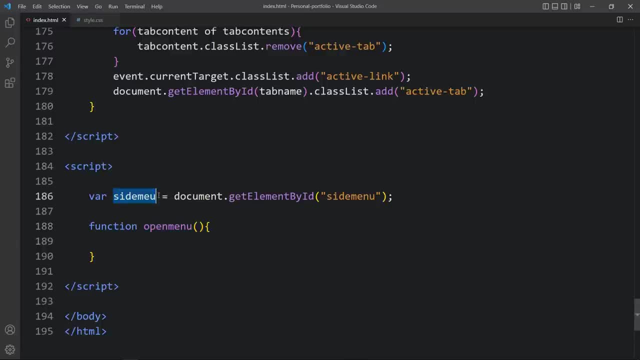 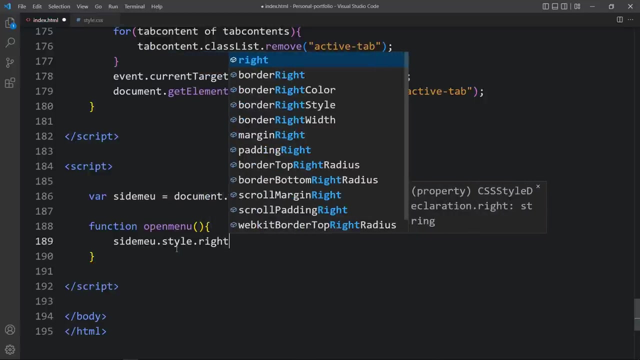 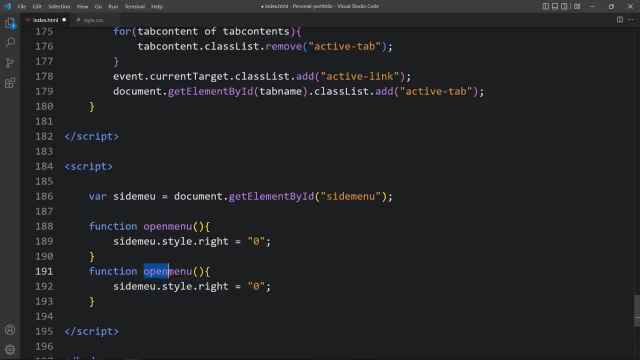 will be called here. we will add this side menu: dot style, dot right equal to 0.. so whenever the right will be 0, it will be visible. let's duplicate it. it will be close menu and when we will run this function- close menu- it will become 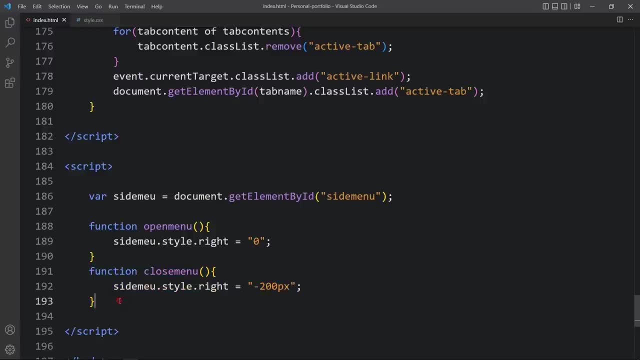 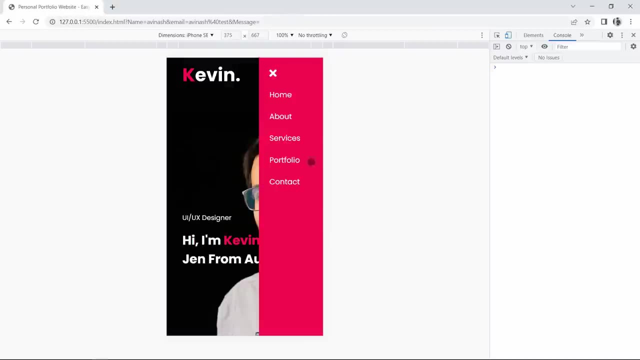 minus 200 pixel. that's it. after adding this, again refresh the website. and here you can see: if i click on this menu icon, this side menu is visible, and if i click on this cross icon, it is hidden. so this side menu is coming and moving instantly. so we need some time delay. so let's come back. 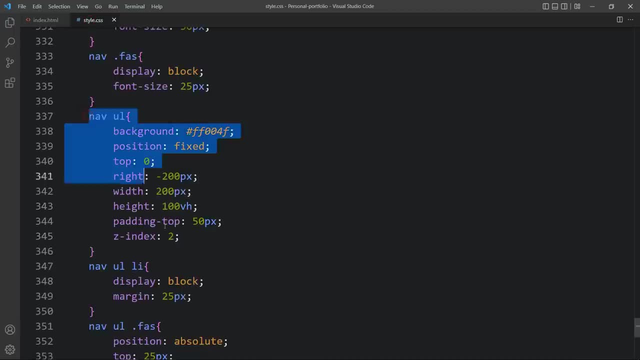 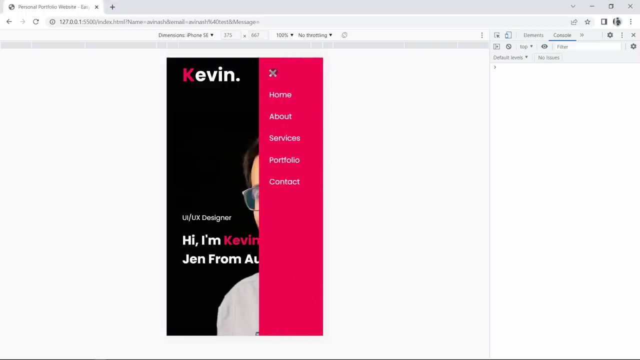 in this css file and here we have added nav ul. so in this one we will add transition write 0.5 seconds. that's it. if i click here, you can see it is smoothly coming from the right side. and if i click on this cross icon again, it will go on the right side and it will become hidden. 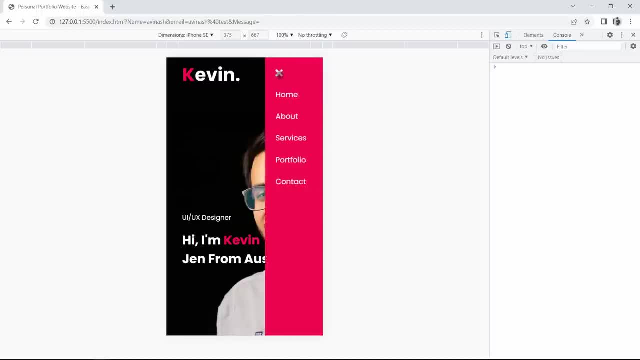 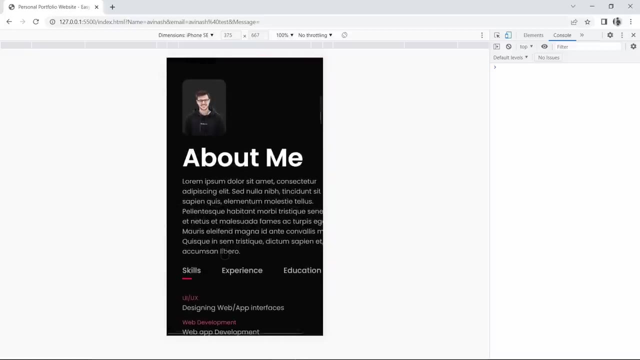 so this one is working fine and other things, which is this type of title is looking good. now let's scroll this and come to the next section, which is for the about in this about, the size for this image is small and this text is going to the right side, so we have to. 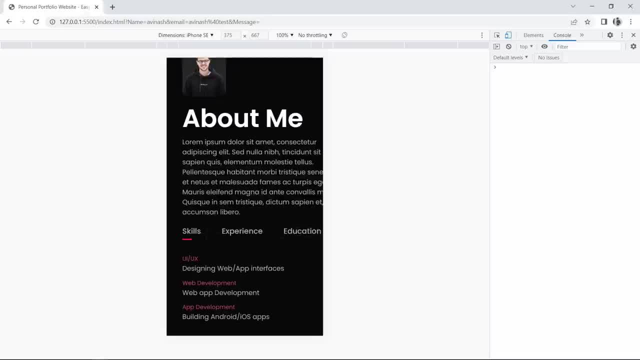 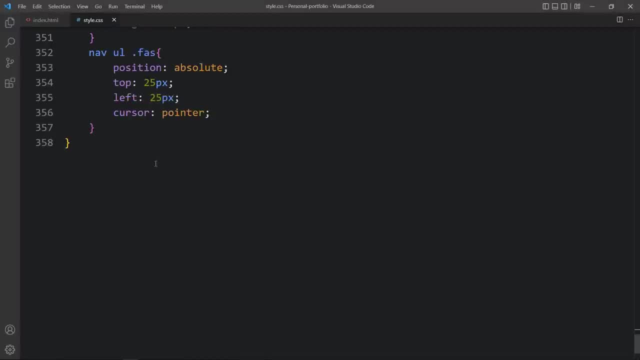 decrease the space between these text and we will decrease the font size also. so first we will decrease the size for this text, which is about me. so let's come back, come to this media query. in this media query here we will add the class name that we have added for the subtitle. so write subtitle and decrease the font size. font size will. 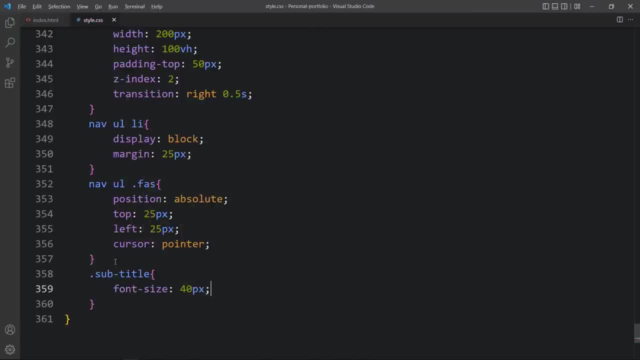 be 40 pixel, so the size has been reduced. next we will increase the size for this image. for that here we will add the class name for the left and right column, which is for the about call 1 and comma about call 2. for this one we will add: 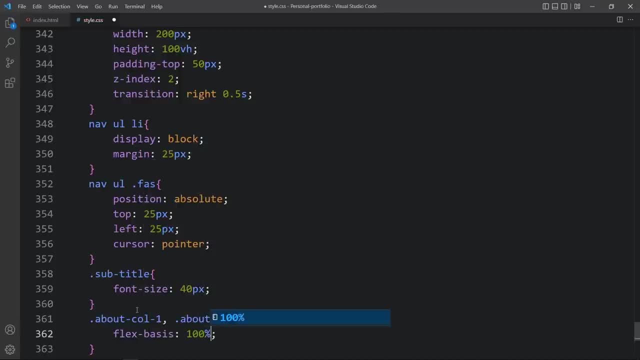 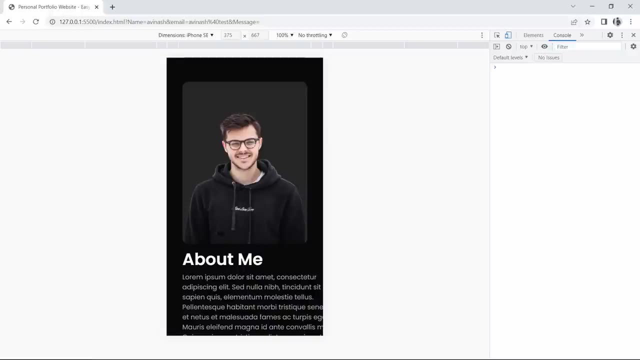 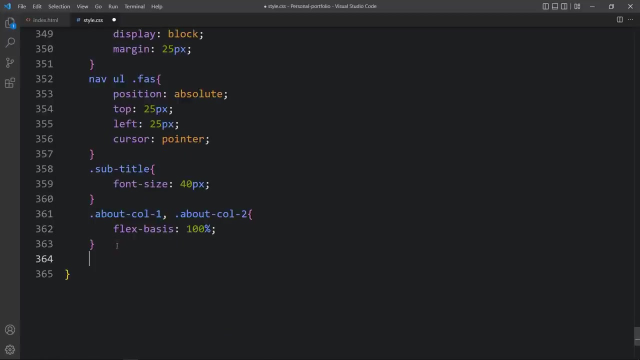 flex basis. it will be 100. now you can see the increased size for this image. next we need some space between this image and this text, so let's come back and again write this class name, then write margin from the bottom, so we have some space just below this image. next we have to decrease the font size for this text. 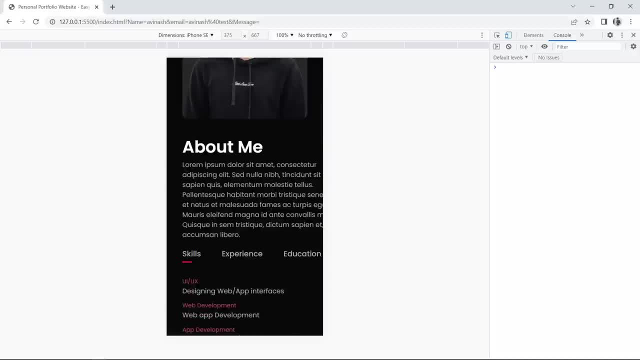 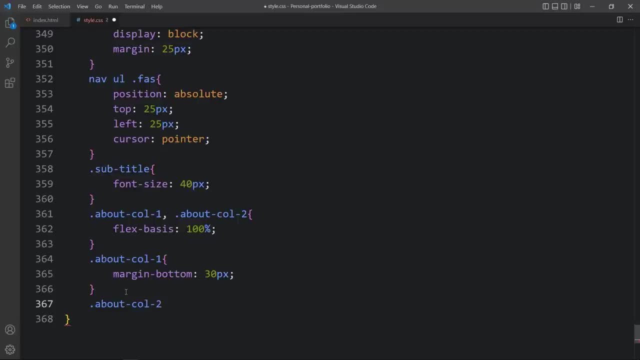 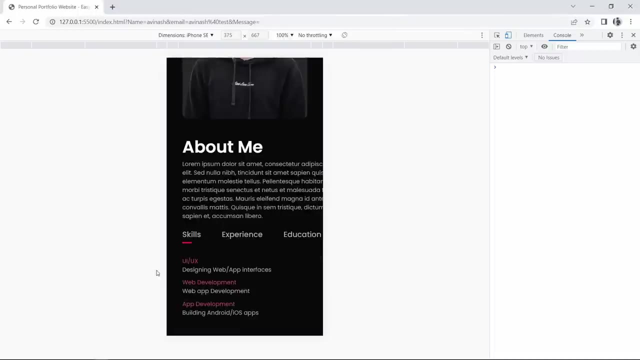 which is here. so let's come back and write the second class name for the second column about call 2, and here in this one, we will add the font size 14 pixel, so the font size has been reduced. next, we will decrease the space between this skills, experience and education, and we will also decrease 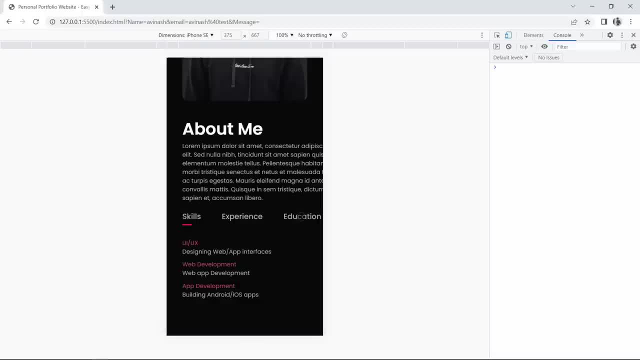 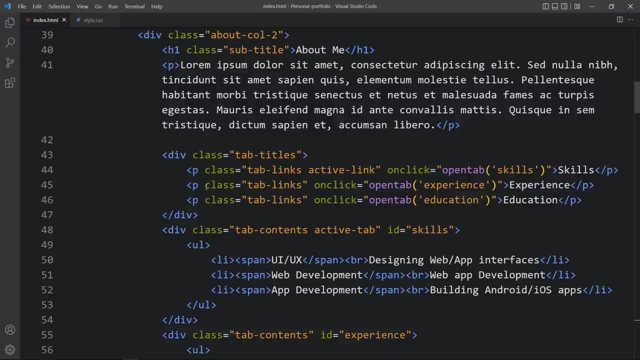 the font size for this text. so we will add the font size 14 pixel. so the font size has been reduced font size. so let's come back and here you can see we have added the link title, which is tab titles and tab links. so let's copy this one tab links for this one. here we will add the css. 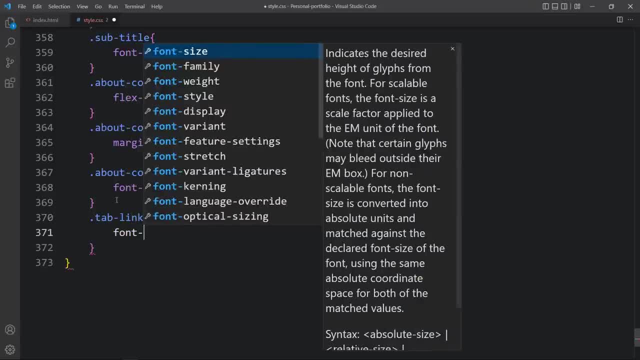 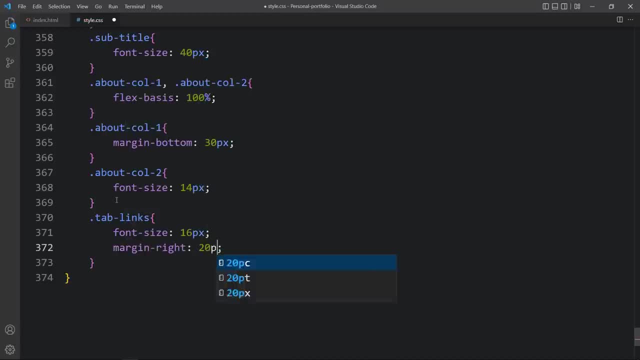 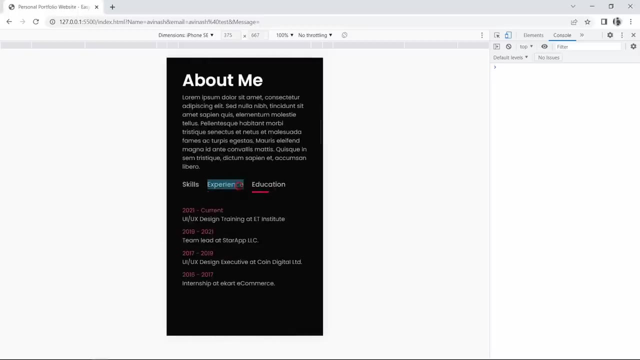 in the media query. let's add the font size: it will be 16 pixel and margin from the right side 20 pixel. so it is looking good. if i click on experience, it is working. if i click on education, it is working. so this about section is also good for the smaller screen and this. 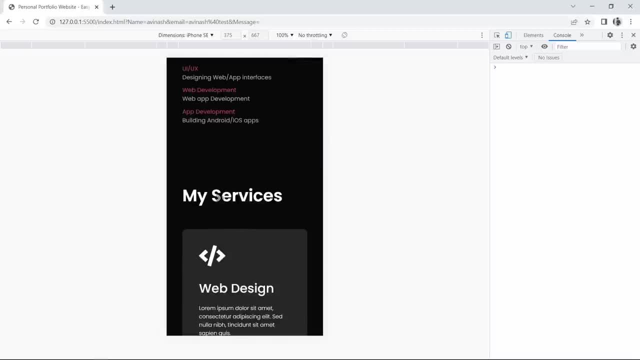 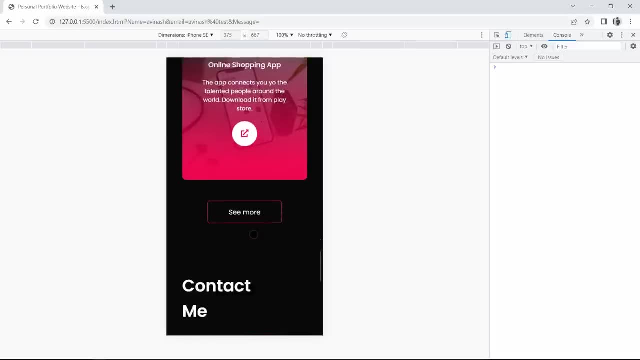 header section also let me scroll down and this, my services section is looking good and this work section is also fine. here and now in this contact section we need to increase the width: contact left column and contact right column. so let's come back to the css file and in this media query we will add: 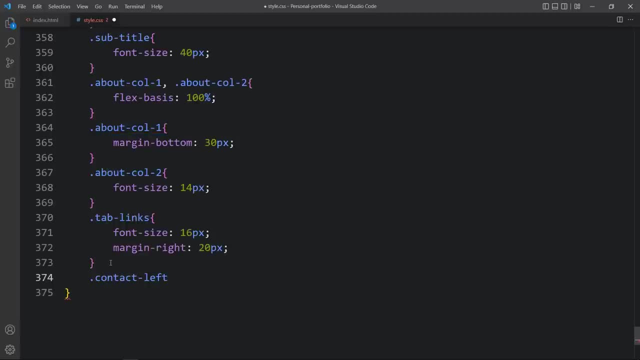 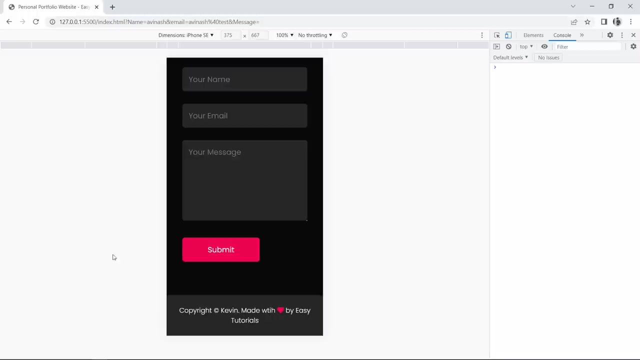 dot contact left and the second class name, comma dot contact right. for this left and right column we will add flex basis 100, so you can see this form is looking good and this button is also good. here and next we will add the css for this copyright text and we will reduce the font size for this. 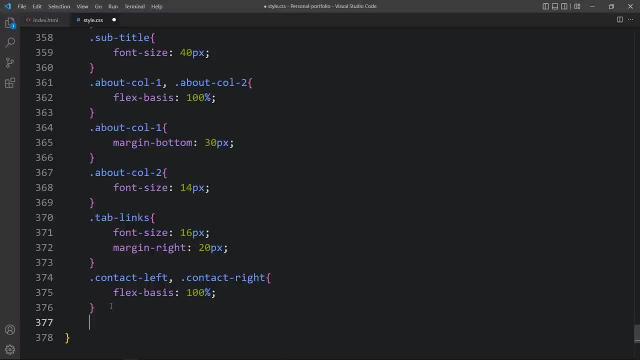 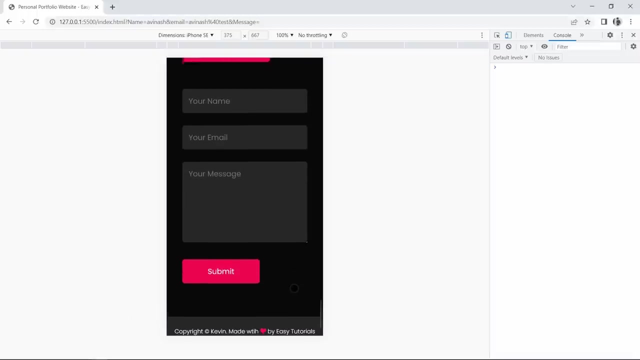 one. so let's come back and write the class, name, dot, copy, type, font size. it will be 14 pixel. so this copyright text is also fine for smaller screen. so let's scroll this website up and you can see all the sections on. this website is looking good for a smaller screen device. 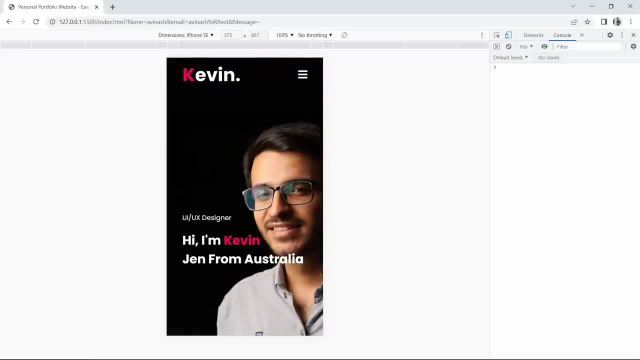 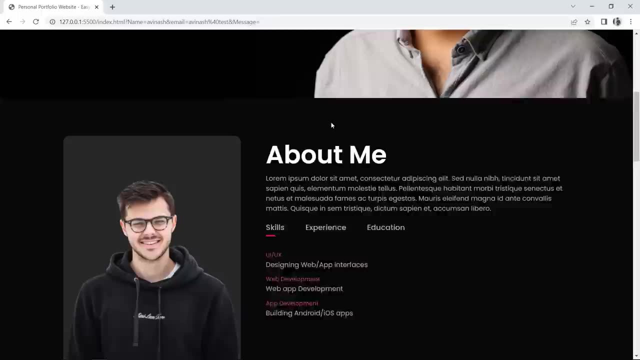 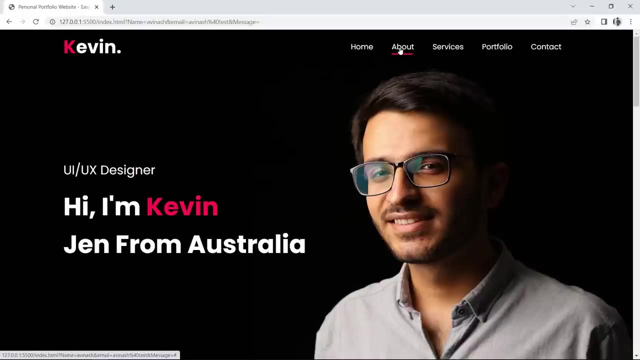 and now we are done. let me open this website in full screen here also. it is fine. next we have to add the click features in these menu links. if i click on about, it should scroll the webpage to the about section. if i click on services, it should display the services section. if i click on portfolio, it will open the portfolio. 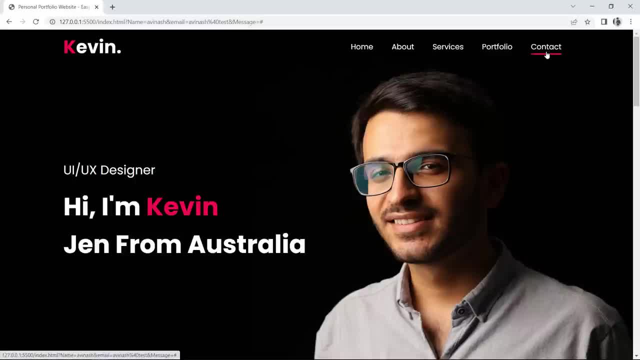 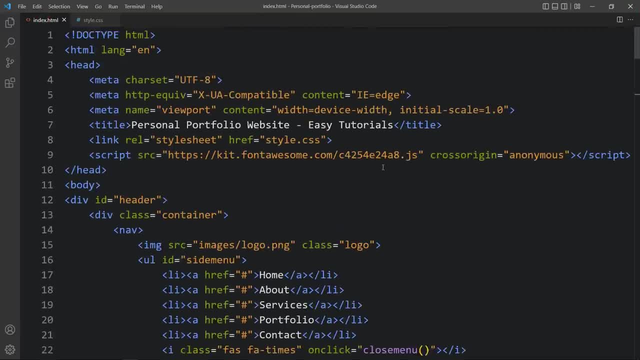 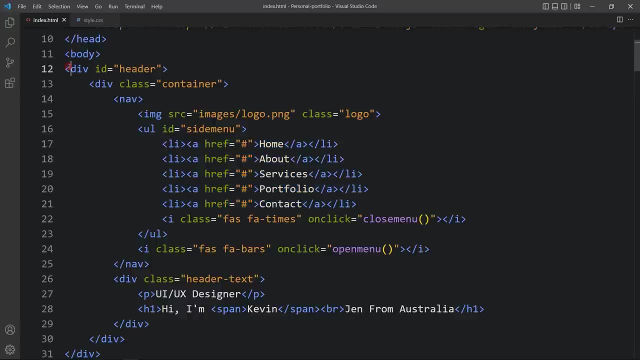 section and if i click on contact it should scroll the webpage to the contact section. so let's come back and in this html file, just come here- where we have added the navigation links here. so in this one we will add the id of this section. so here in this header you can see we have added 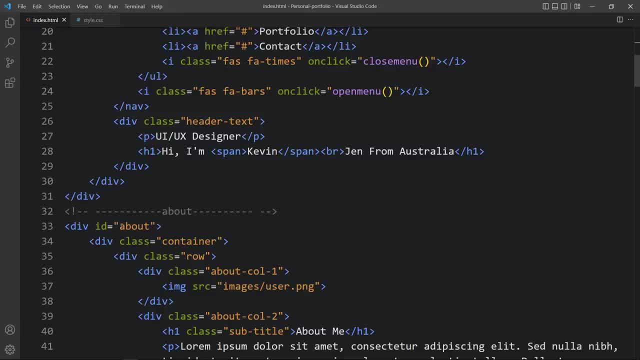 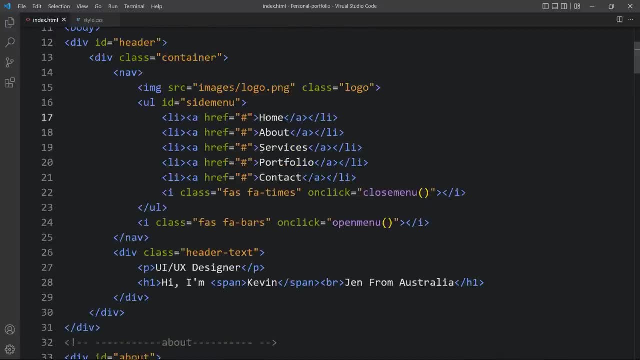 the id header. now in the second one we have added the id about. in the third one we have added the id services, like that. so here we have to add these id. so first we will add header, hashtag, header in in this href, then we will add hashtag about, then services, then portfolio, then contact. 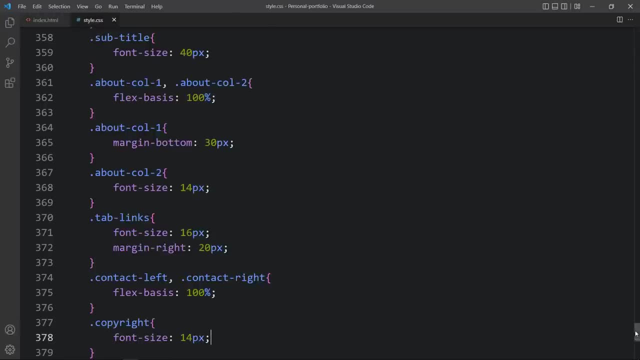 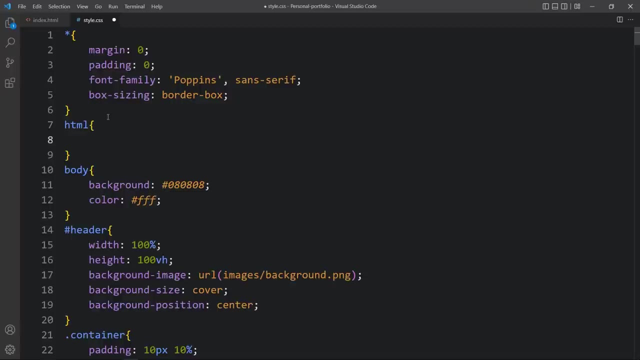 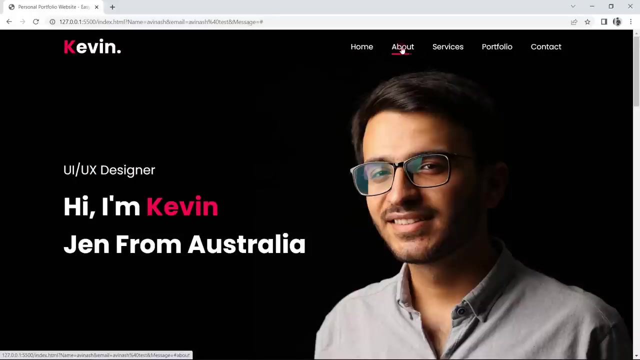 after adding this, come back to the css file and just come to the top. here we will add html and in this html we will add the scroll behavior. scroll behavior will be smooth. that's it. after adding this again, refresh the website and let's click on the about. it will scroll. 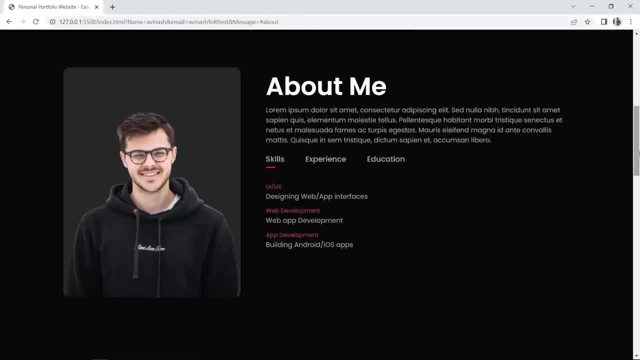 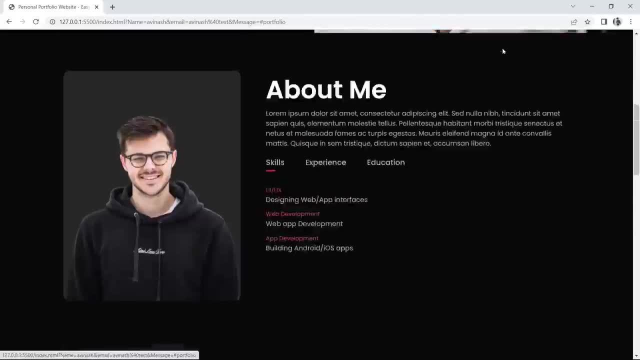 the website to the about section very smoothly. let's come to the top and click on contact. it is a scrolling the website to the contact section. let's come to the top, click on portfolio. it is a scrolling the website to the portfolio section, or my work. let's come here, click on. 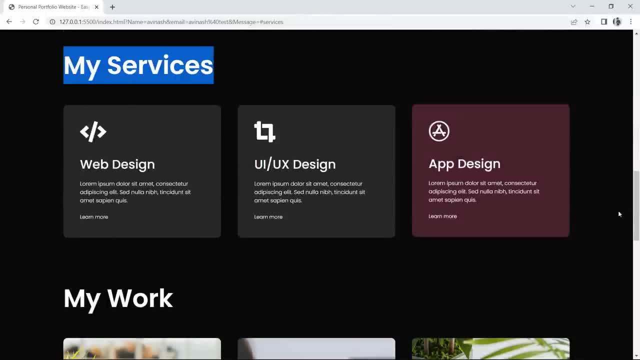 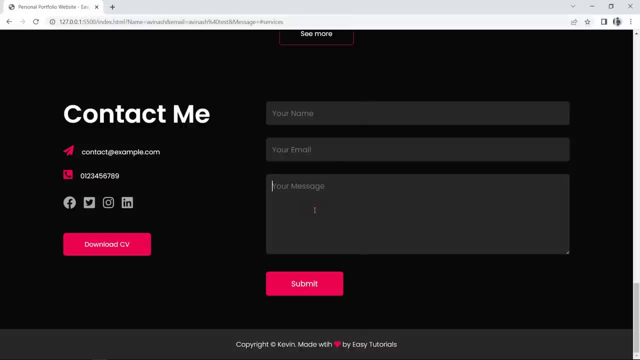 services. it is a scrolling the website to the services section, so this is working fine. so now we have designed this website. next we have to make this contact form working. whenever people will enter any data in this contact form and click on this submit button, you will receive the information on your google sheet to make this contact form working, just 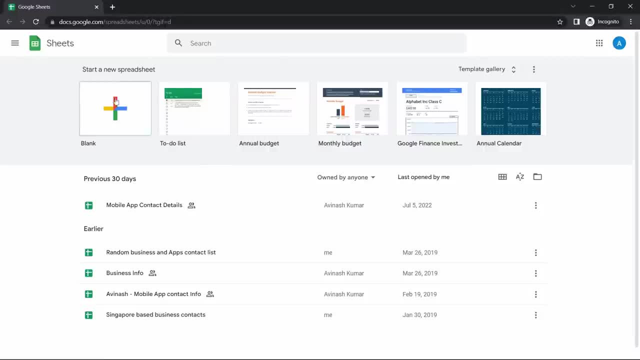 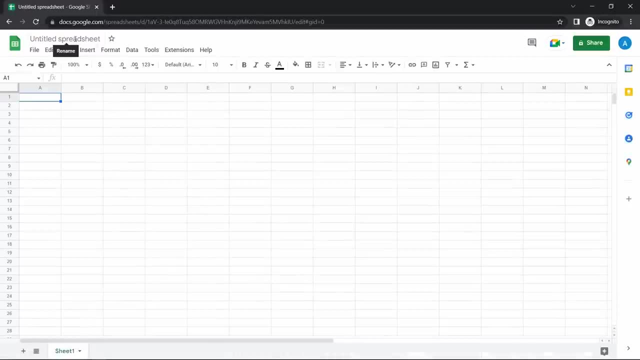 open your google sheet and here you have to create a new sheet. click here and write any title for this sheet. i will write contact form and in this field we have to add the name that we have added in the input field of the form. so let's come back to the code. 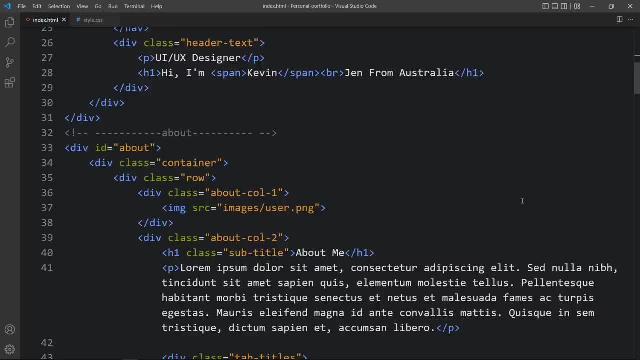 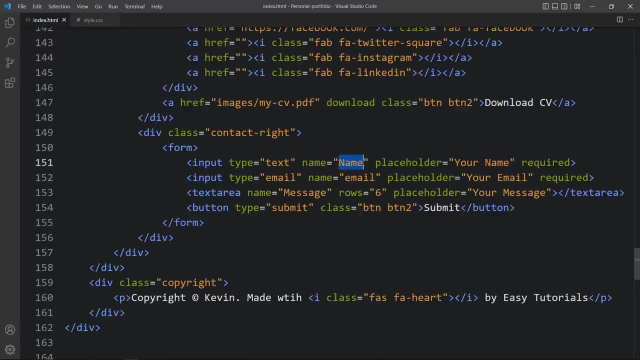 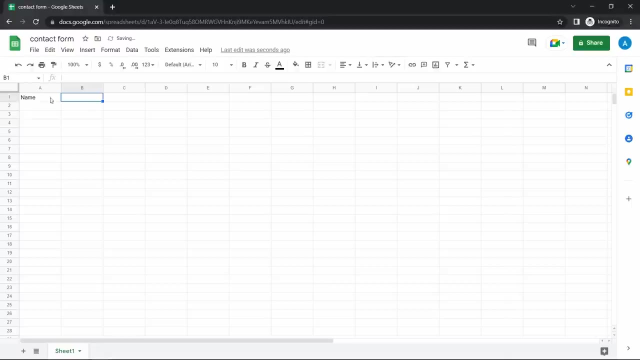 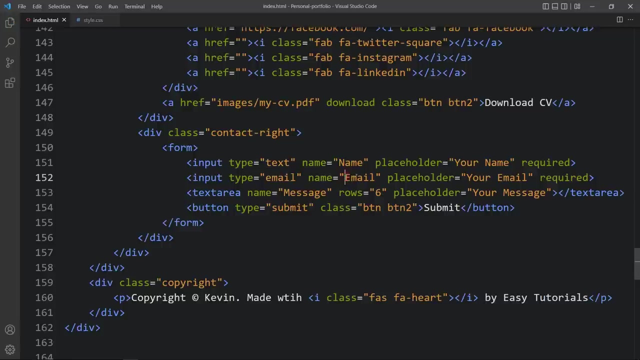 file, in this html file, come to the form, and in this form you can see we have added the name. copy this one and add it here. name. now in this second column we will add this one, which is email right capital e. it should be same like if you are using the small case. 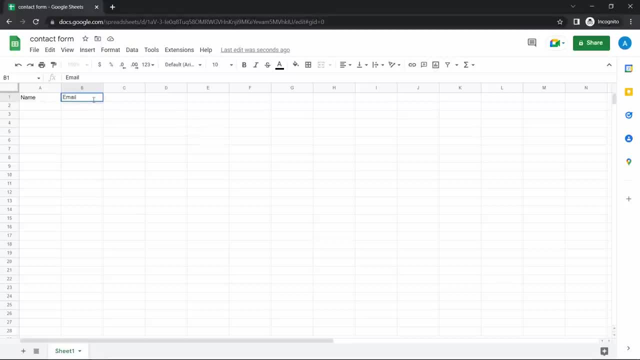 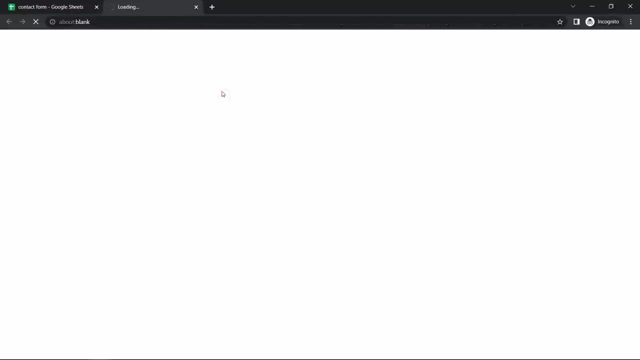 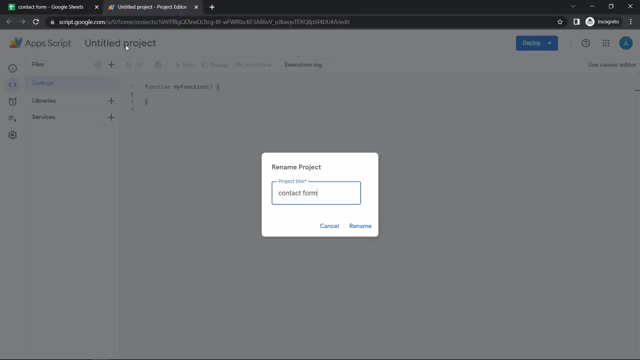 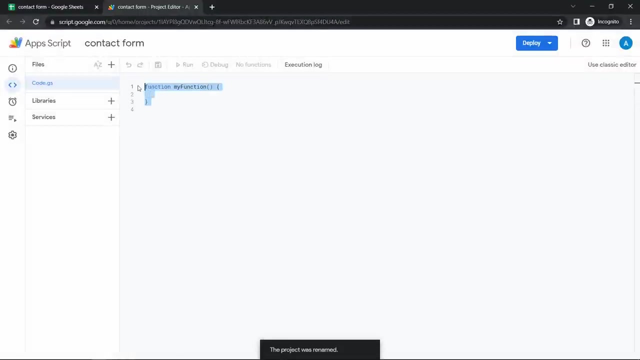 then it will be small case here- email. then we have the message like this: so we have added this one. next we have to click on this extensions, then click on a script. for this script we will add one title- it will be same as contact form- and remove this function, which is written in this, a script file, and here we will add: 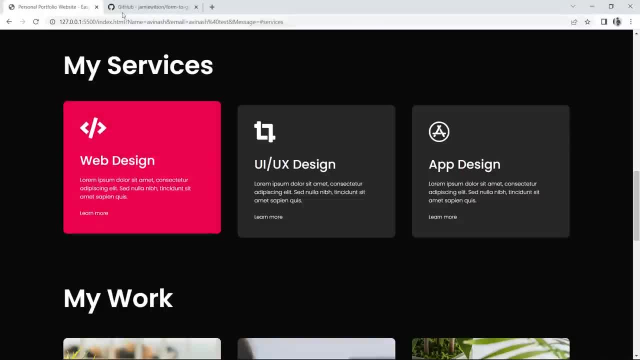 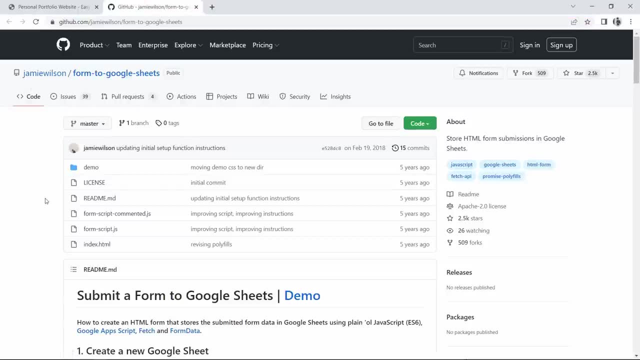 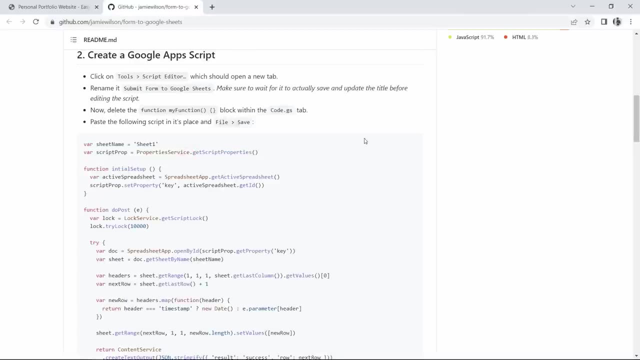 one script for that. let me come back to a, a github link. you can find this github link in the description. you can see the name of the creator for this code. let's scroll down here and here you will find this script. so just copy this one. click here to copy and come back to the form: a script which is app. 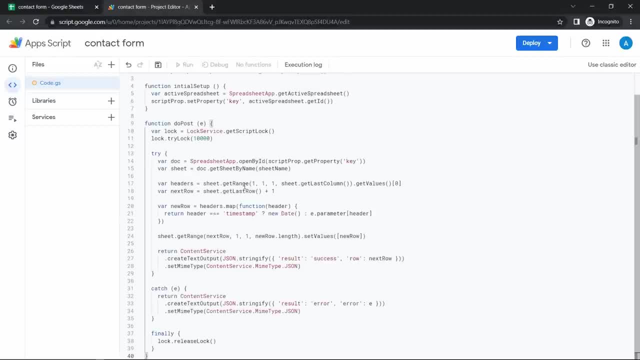 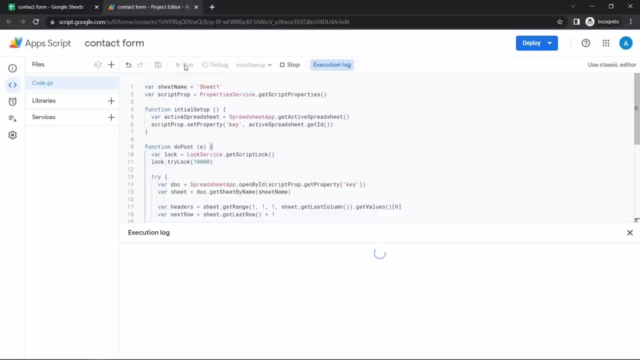 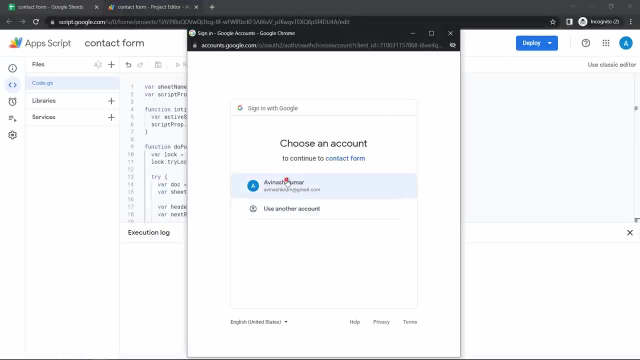 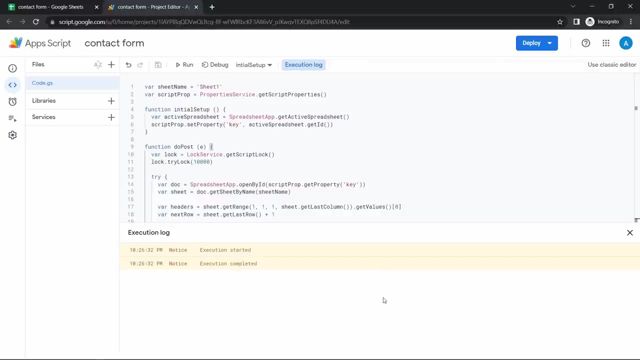 script here. paste this one and click on this save icon, which is here. and after save, click on run and it is asking to review the permission. click here and confirm your account. click on advance and click on goto contact form and save. click on allow. now you can see this message: execution started and execution completed. that's it after that. 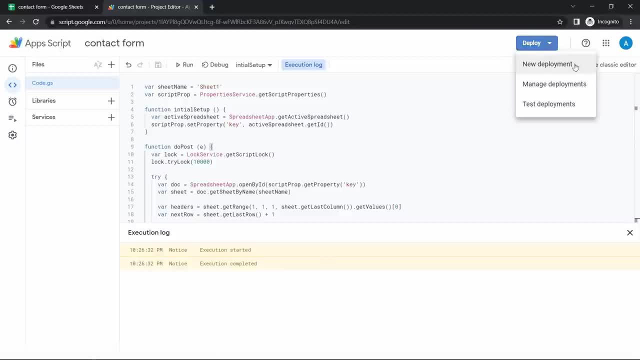 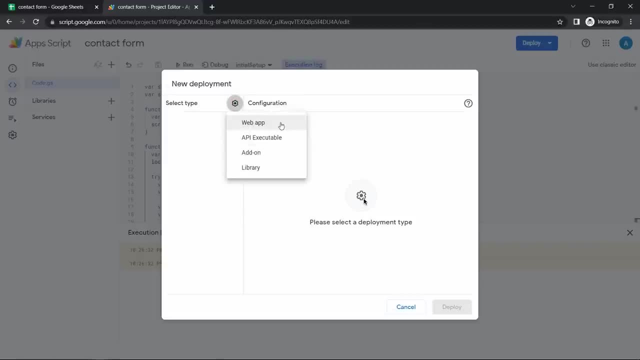 you can see this button here: deploy- click here. click on new deployment, click on this setting icon, click on web app and here you have to add any description. i will add contact form. it will be your email id. there is no need to change anything. and in this third, 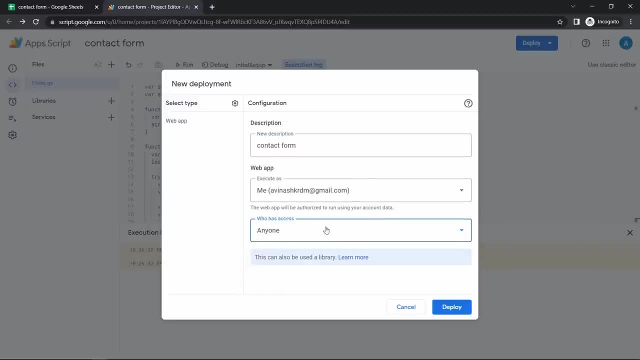 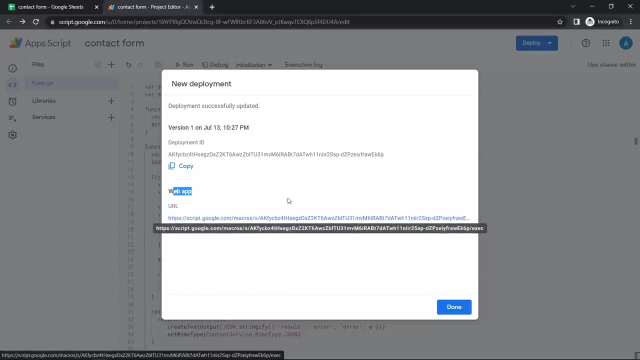 one. select anyone. it is important select anyone, then click on deploy. after clicking on this deploy, you will get an url. you can see we got an webapp url that we will be using on our html file. so now again, come back to the github link and scroll down, and you can see. 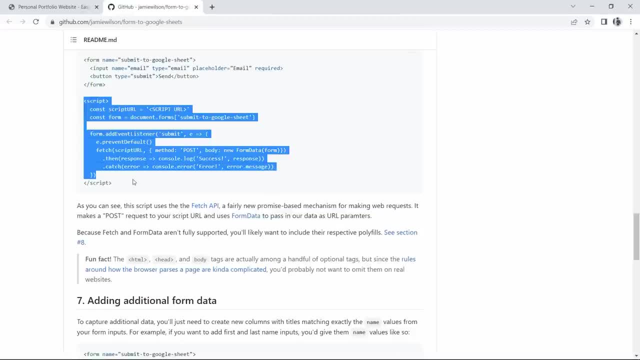 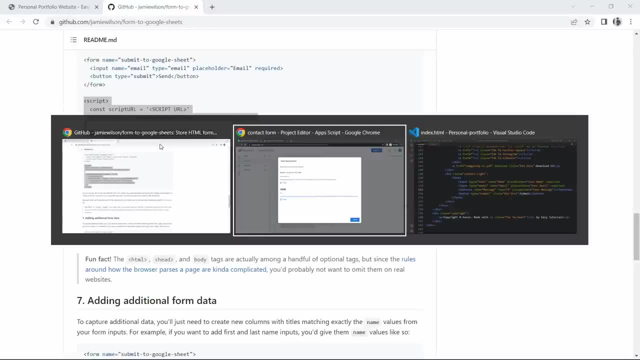 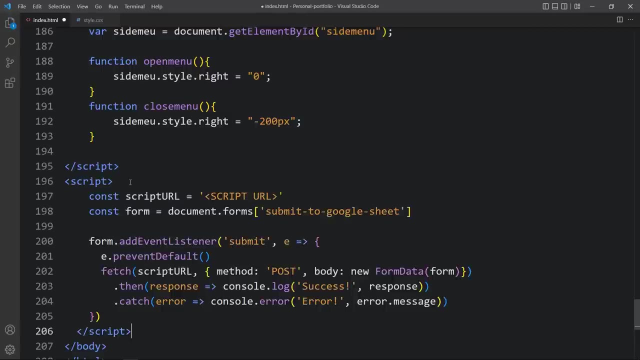 and here you will find the suscript. just copy this suscript from this web page and add it in your html file. let's come back and in this html file, just at the bottom above this closing body tag, i will add the suscript like this: and here you can see the script. 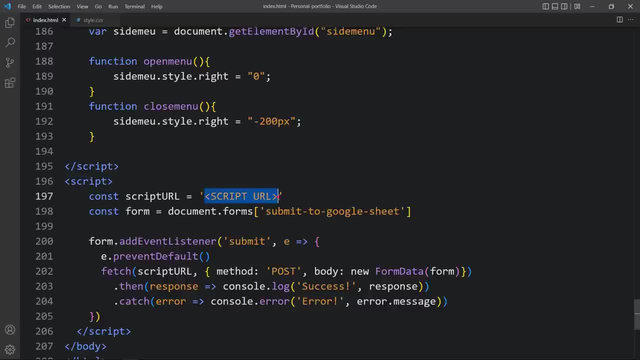 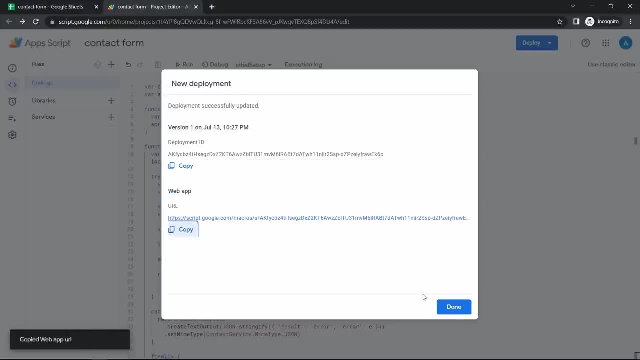 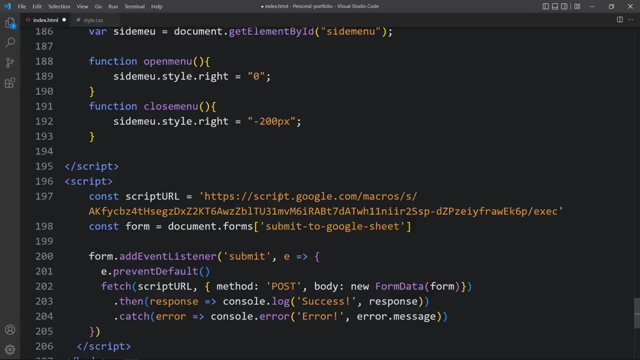 url here. only you have to add the url that we got from the app script. just copy this url and paste it here like this: after adding this here, you can see submit to google sheet. just copy this and come back to the form where it is here in this form: 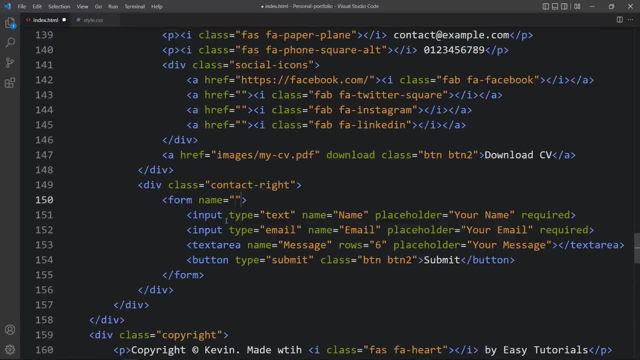 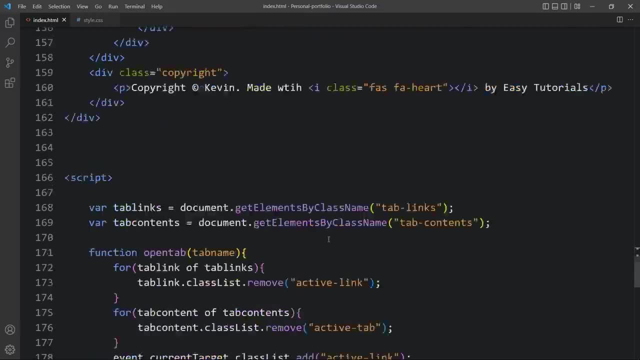 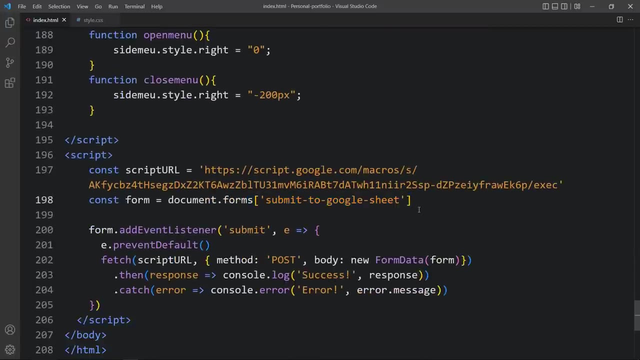 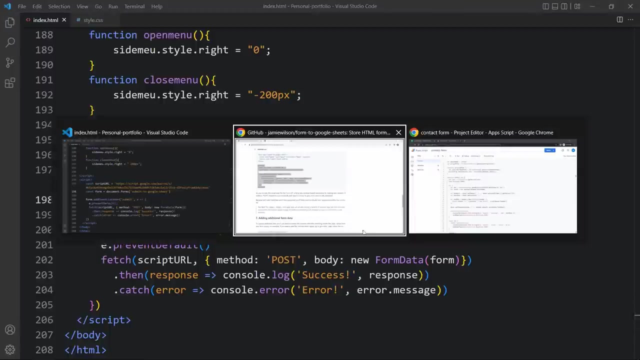 we will add name. this one submit to google. it will be same here: submit to google. form name is submit to google and here also it is same. after that, if we will submit this form, we will receive the information. let's see, come back to the website and let's write. 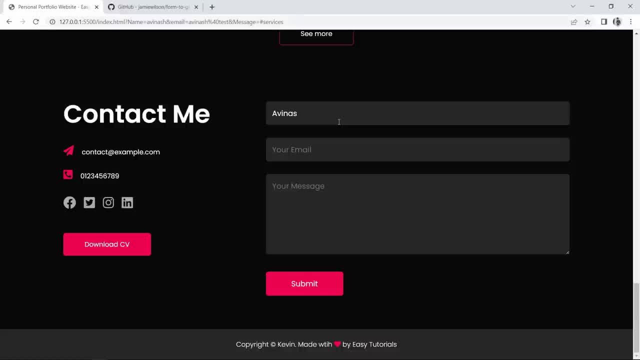 anything here. i will add avinas1. then write one email id here- test1 at gmailcom- and write the test1. this is the message. this is the name, email id and message. click on submit and you can see. this page is as it is. there is no change. 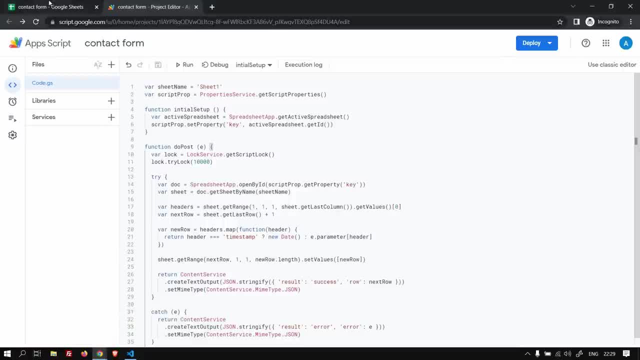 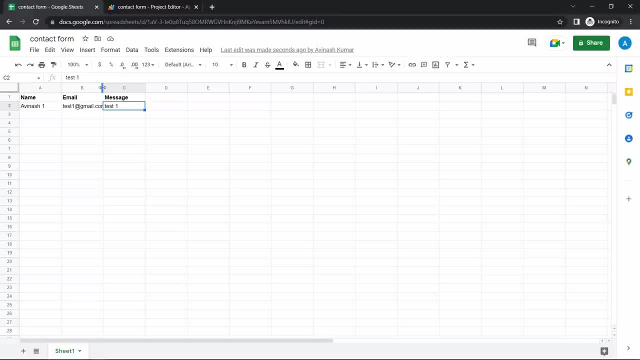 but if i go to the google sheet you can see we got the information here: avinas1, test1 and test1. we got the name, email id and message. so this is how you can receive the information on your google sheet whenever people will enter any data in the contact form. next we 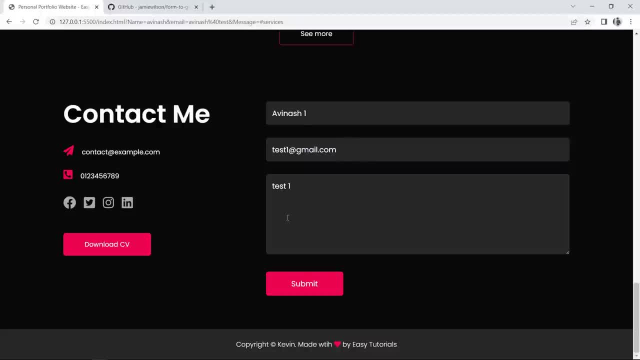 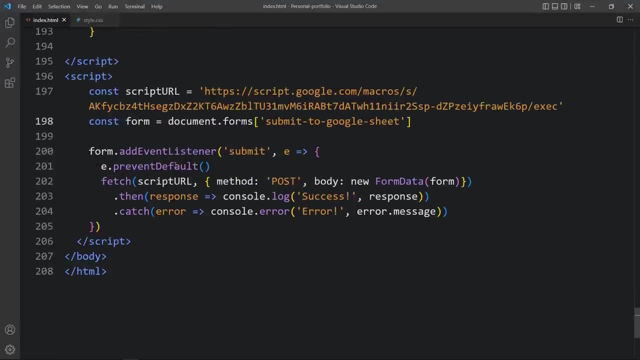 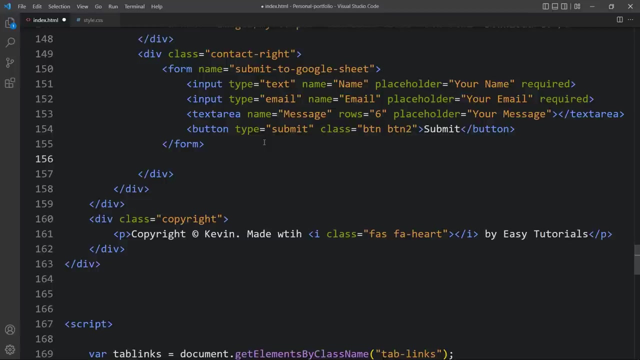 have to make this form reset after submitting the form, and we will get the contact form page confirmation message here that the message had been sent successfully. like that? for that let's come back. and here we have the form. so after this form we will display one message. 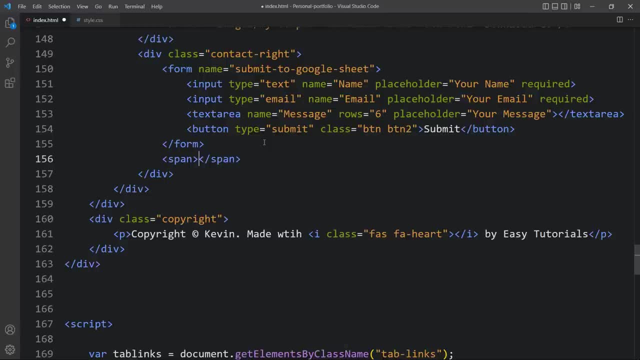 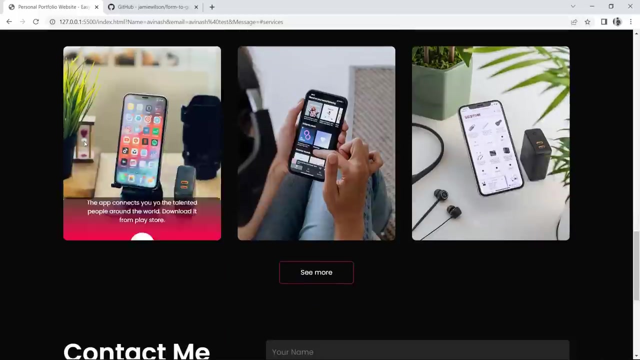 so let's add one span tag here and in this span we will add one id and write the id msg. and in this msg let's add anything: hello. and let's come to the website and see where it is displaying. it is displaying here, hello, like this. so next we have to design this one. 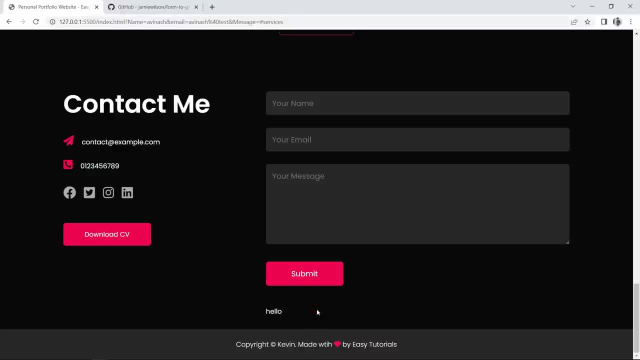 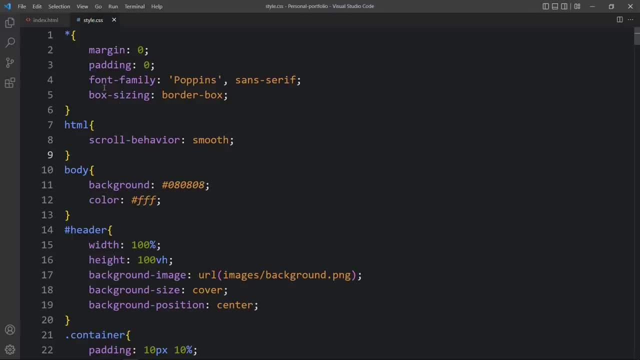 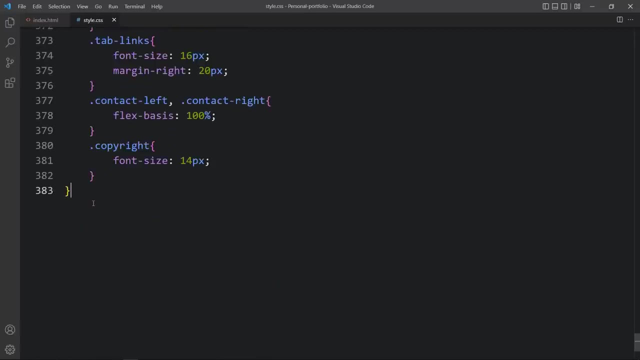 so we will change the color and some space we will add. so let's come back and come to the css file at the bottom we will add: after closing of this bracket, we will add hashtag span because its an id for this span. we will change the color. it will be this color code. 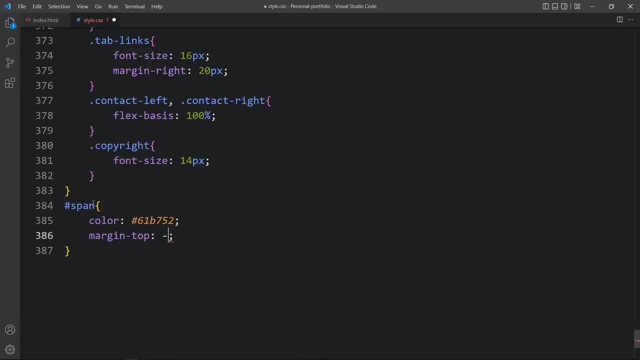 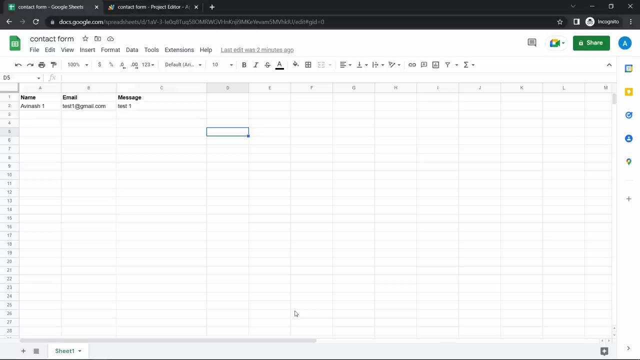 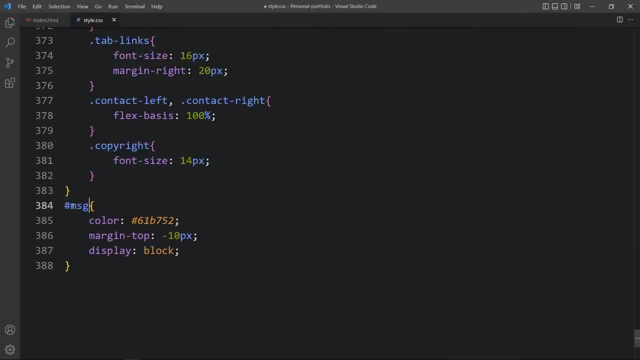 then remove a space from the top, so margin top minus 10px and after that display it will be block. there is no changes here, so lets see here we will add msg. this is the id right hashtag: msg. now you can see the color has been changed. 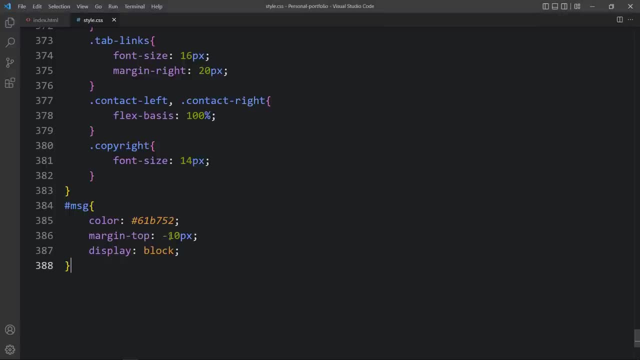 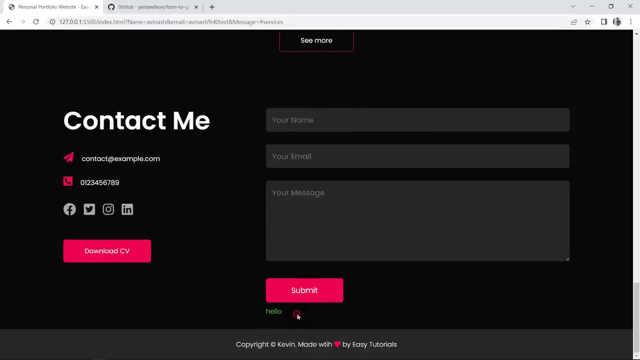 we will move it up. so again, come back. and here we will add minus 20px. it is here if i write minus 40px. yeah, this position is good. so next we have to replace this message, and it will be only displayed whenever we will click on the submit button. so lets come back. 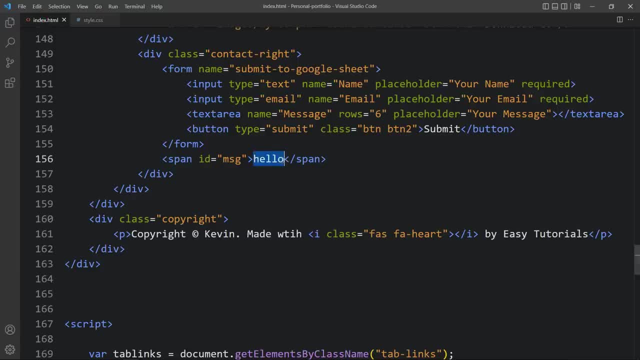 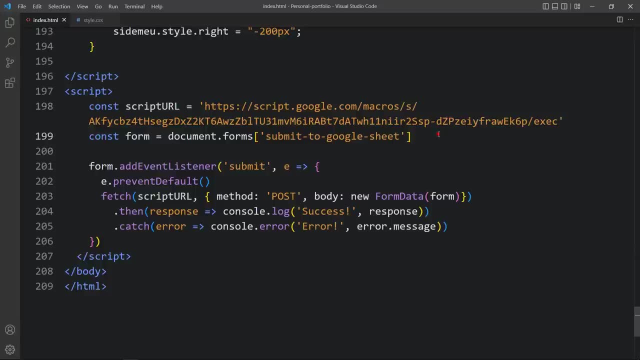 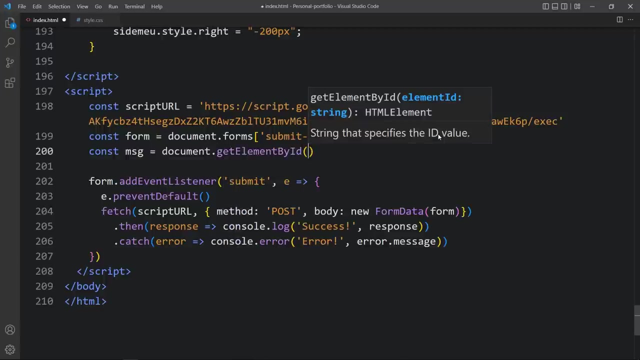 and here hide this one. so just remove this hello and come to the bottom and this one. we have added this const, this const, so let's add one more. here we will add const msg equal to document dot. get element by id and in this id we will add msg like this: now in this, then we have: 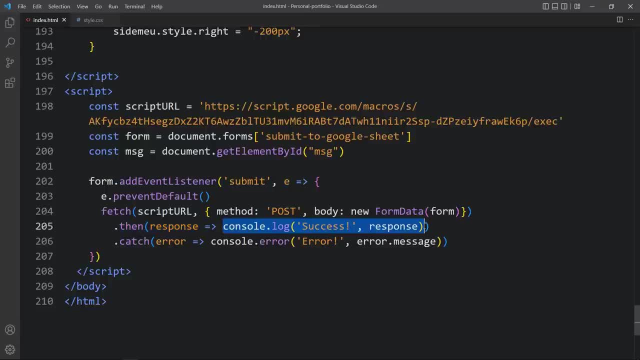 the success. so we have to remove this one and instead of this we will add our own message. so, after this one, remove these things and here we will add curly braces, then write msg dot, inner html equal to here. we will add this message sent successfully. so whenever we will click on the submit button, it will 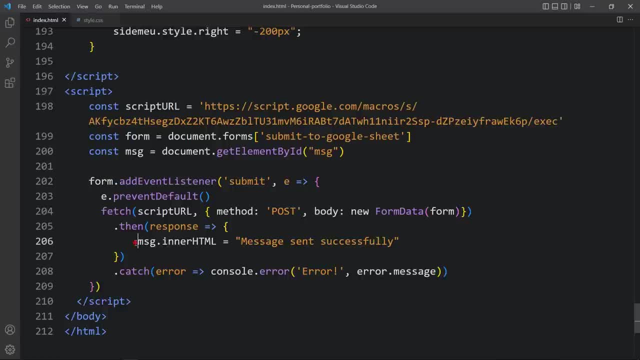 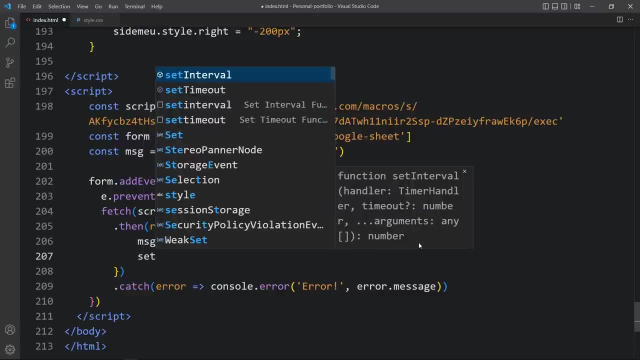 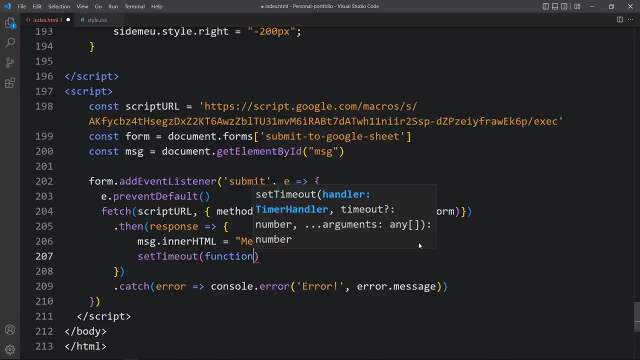 send the data and then it will display this message. but this message will be displayed continuously, so we have to hide this one after few seconds. so here we will add set time out, then write function and in this one write msg dot. inner html equal to this quote. it will be blank, and here add comma 5000. so it is 5000. 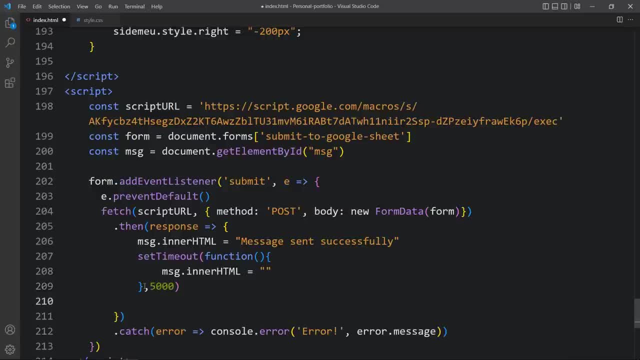 milliseconds, so after five second the message will be removed and then we will add form dot reset. so it will reset the input form and we will personally first self set the code. so we will get this one and we will publish update item. update data will set this. thanks, go ahead many. there are thousands of. 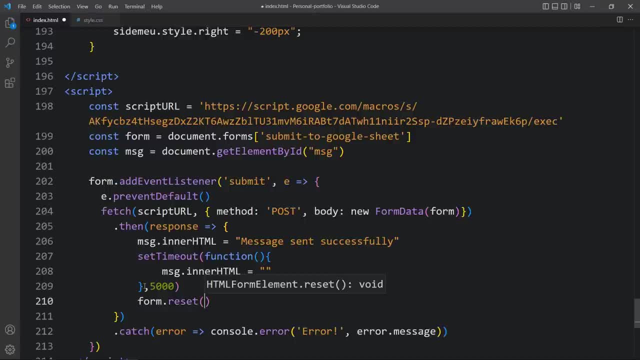 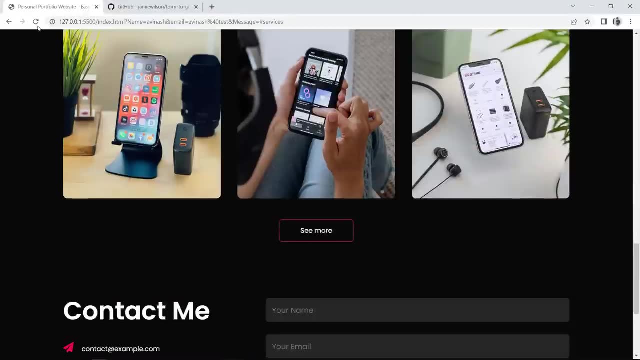 fishköpping, send many of these toesy and every one of these messages will work the same yet. so let's add community, as we stones everything we has to identify the folder absolute entry and let's change the field in the form that's it. after adding this again, refresh the website and let's add any. 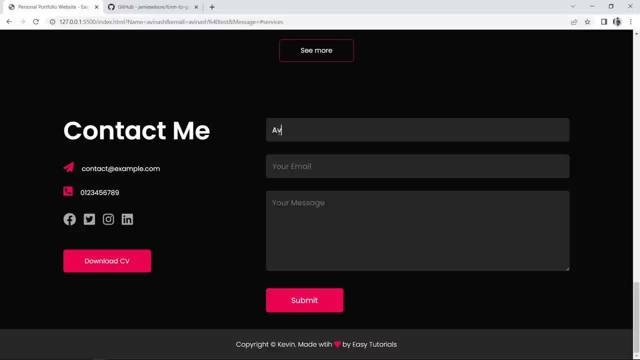 other data in this form. here we will add the name, email id, then message. this is second test message. let's click on this submit button and here you can see this message. message sent successfully and it will be removed after five seconds. done and you can see the form has been reset. let's check our google sheet. here you can see we.